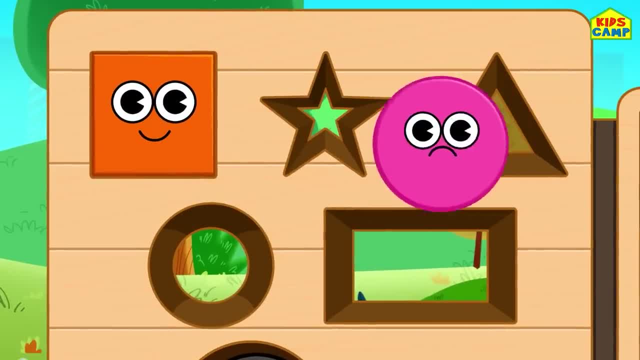 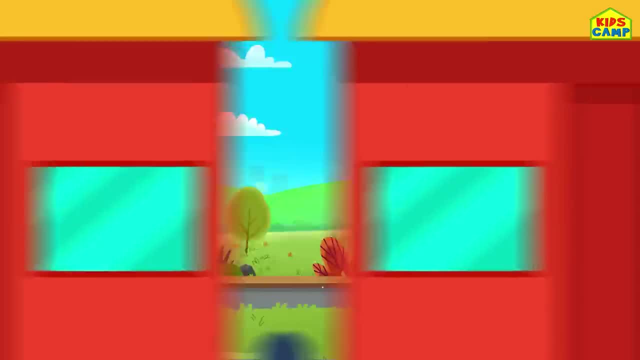 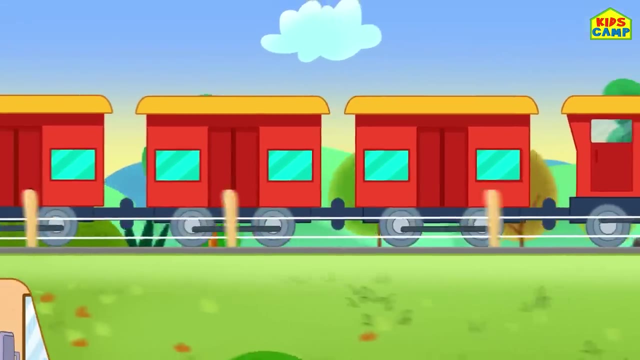 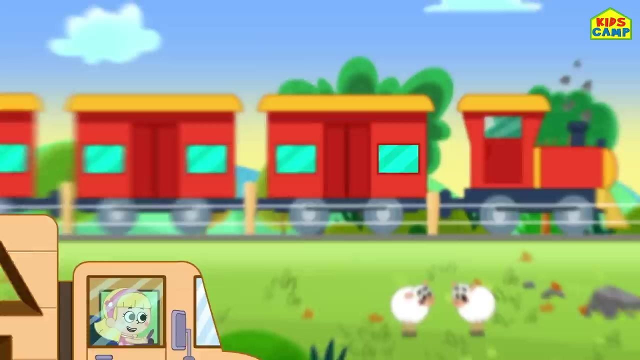 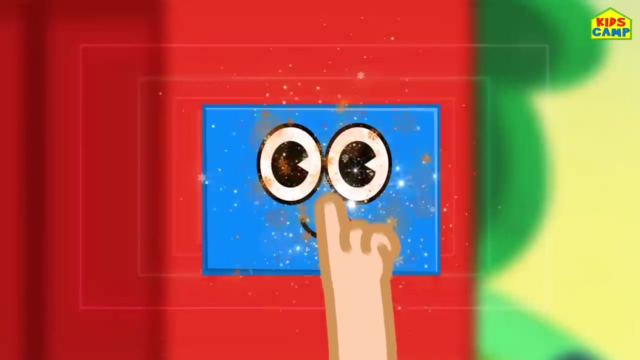 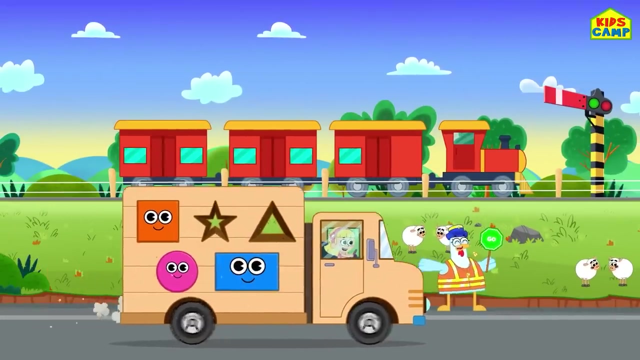 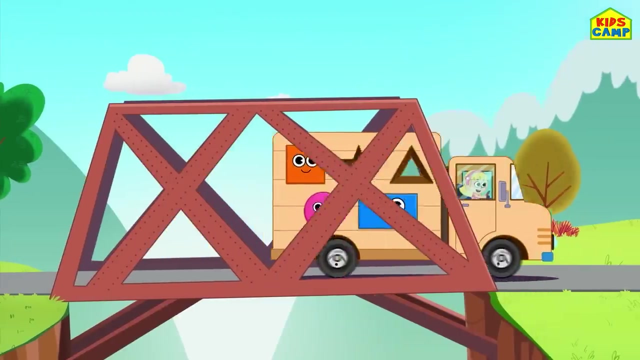 Uh-oh, Not there. No, Aha, It fits correctly, Let's go ahead. Wow, A train. Aha, Do you see what I see Our next shape: Rectangle. Amazing, It fits correctly. Woohoo, Over the bridge, Here I go. Honk, honk, honk, Here I go. 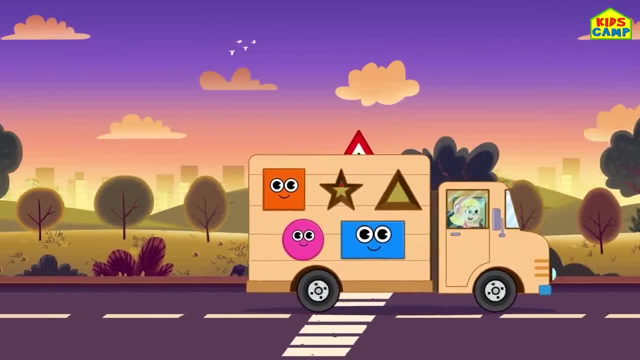 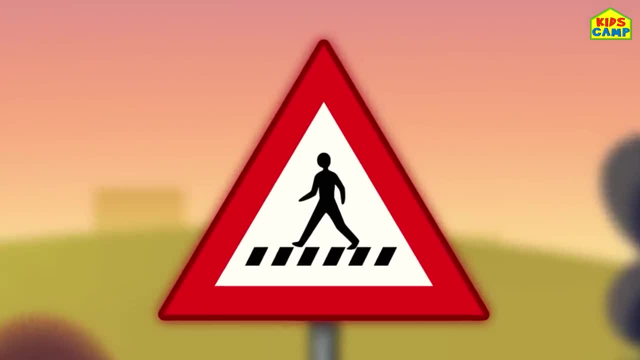 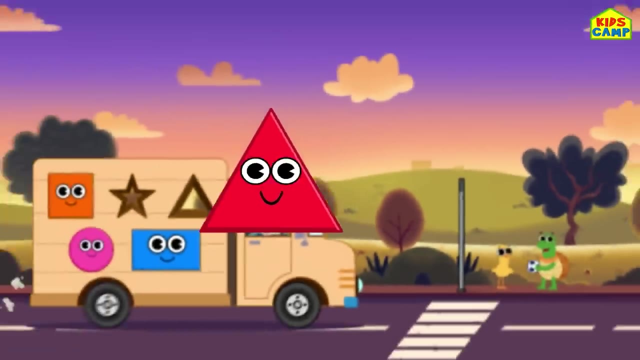 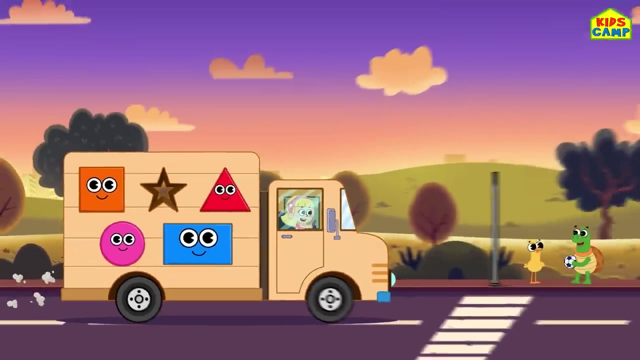 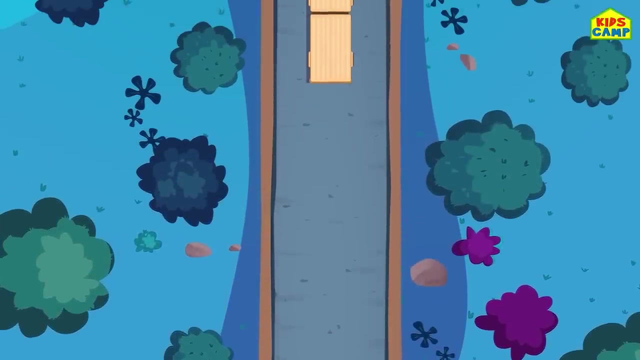 Oh, we almost missed that. Hmm, Is that a triangle? Yes, it is. Wow, Let's place it on my wooden truck. No, Aha, It fits. Let's look for another shape. Where could it be? Wow. 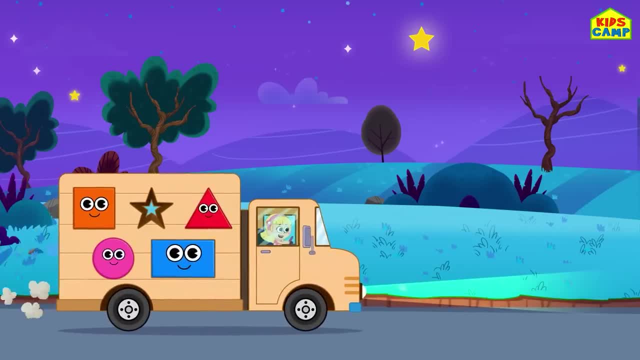 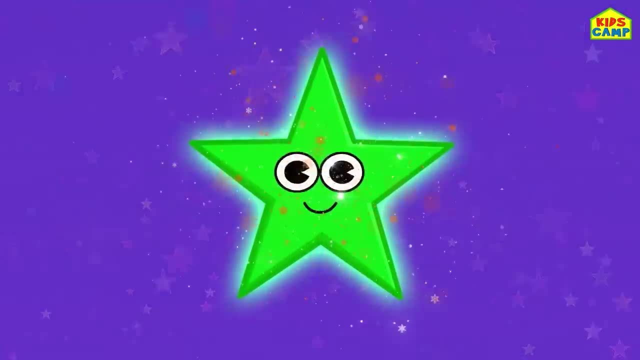 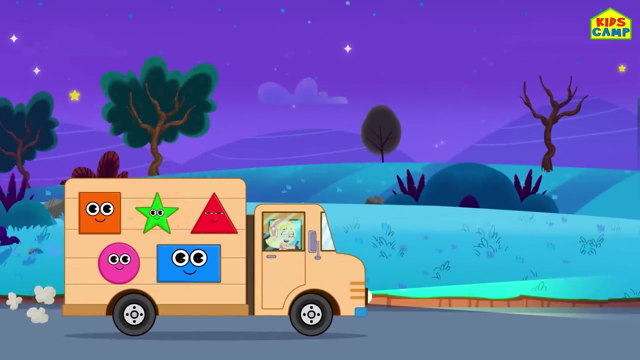 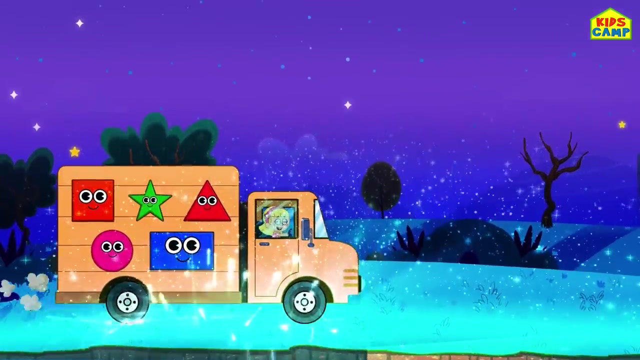 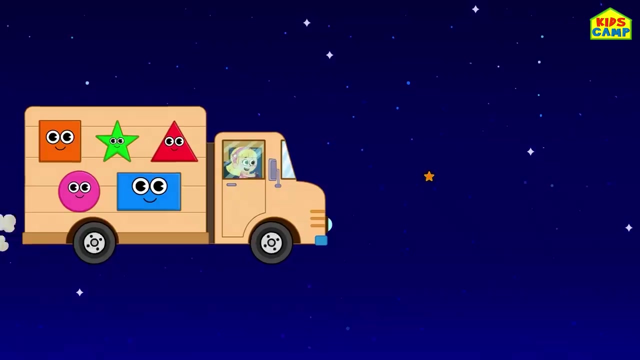 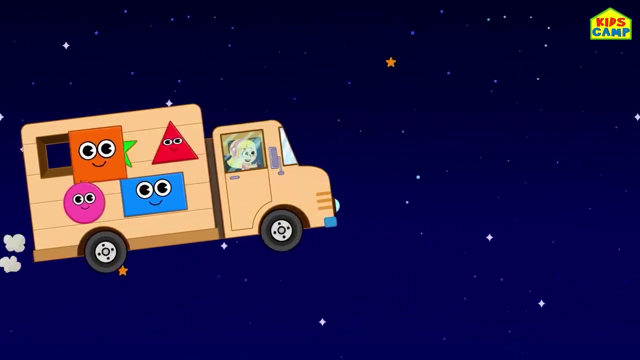 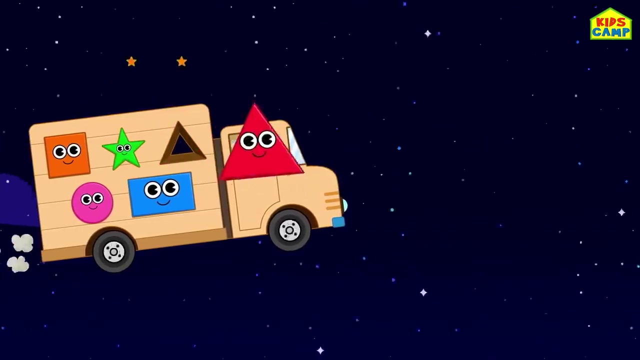 I see it, It's a star Wonderful. Let's place the star on my wooden truck. We've done it. We've collected all the shapes. Oh magic, Wow, Wow, Here I go. Square Star Triangle. 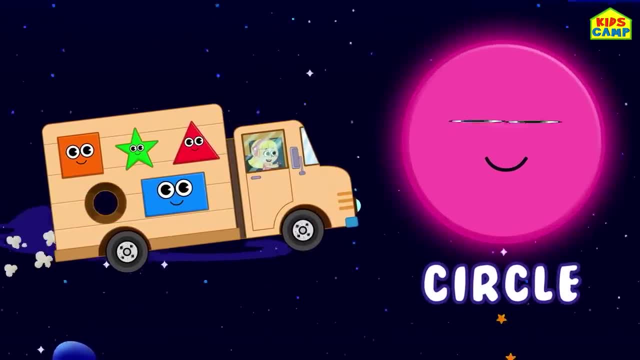 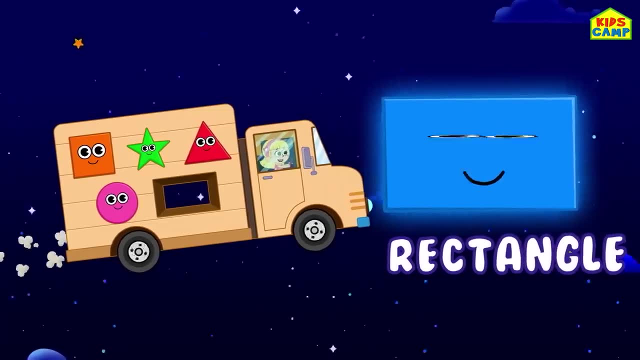 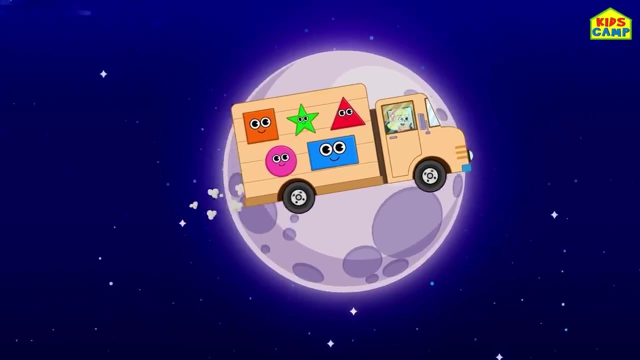 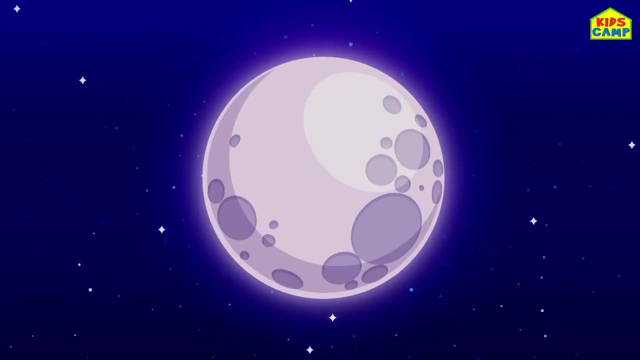 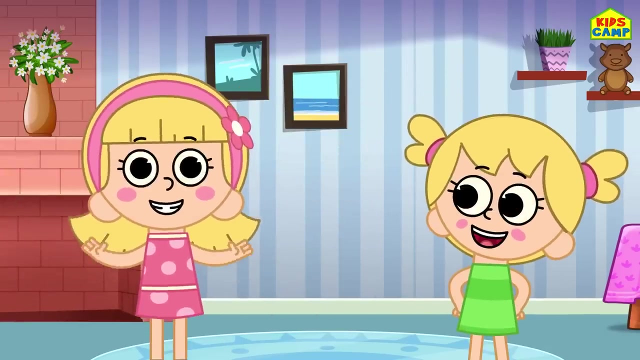 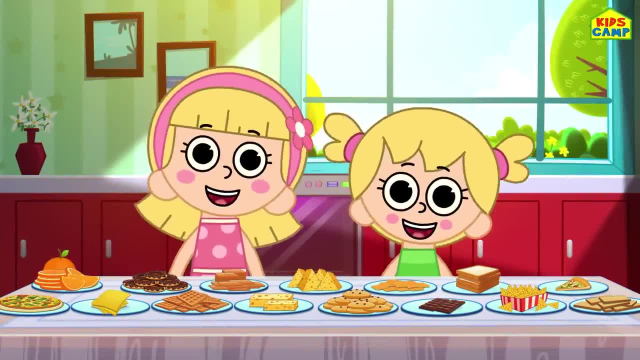 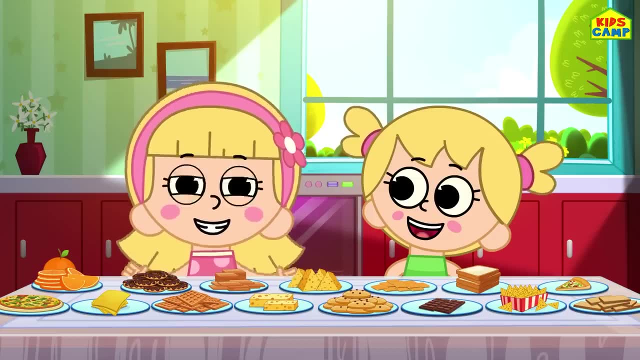 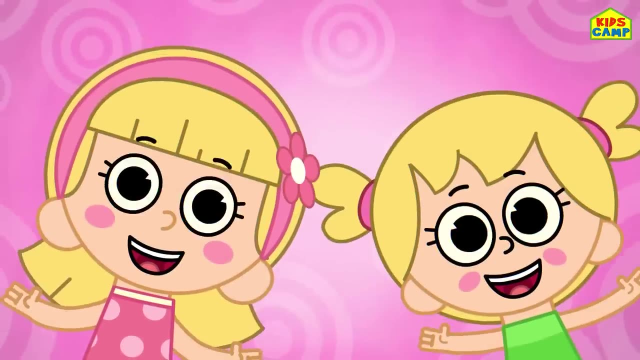 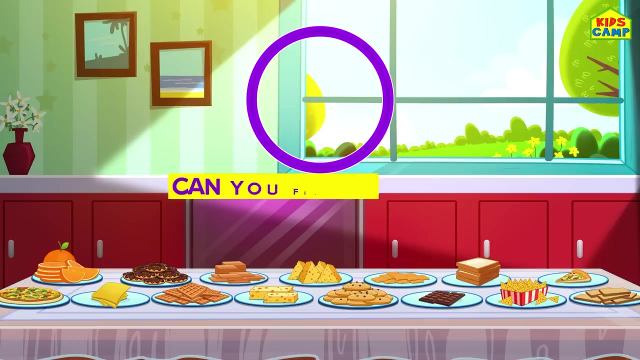 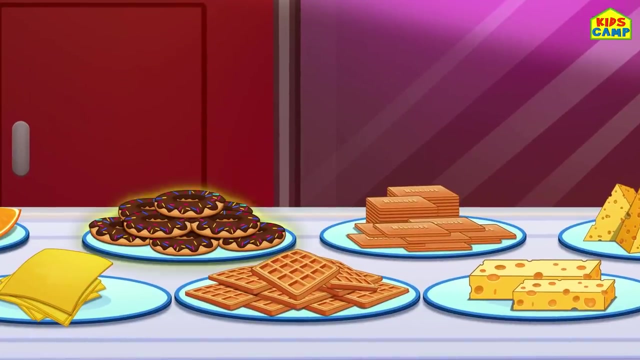 Yay Ooh, Look at all this food- So delicious. We are also going to learn our shapes. Ready Eva. Let's match the shapes with the food Circle. Can you find a circle? Where's a circle? What food is the shape of a circle? 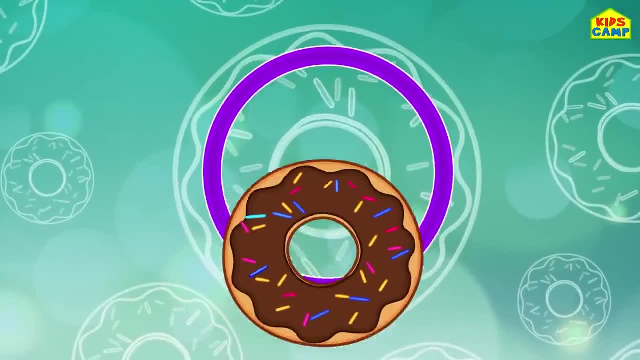 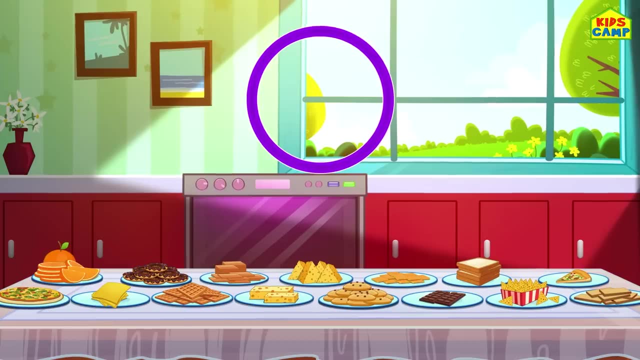 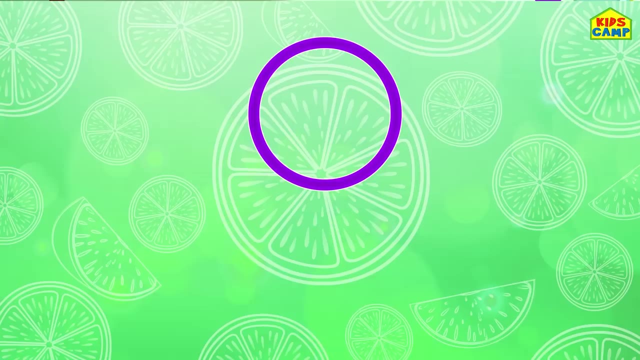 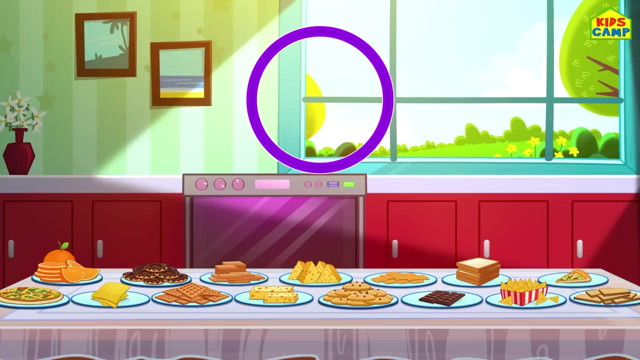 That's right, A doughnut. A doughnut is in the shape of a circle. What else? Hmm, That's right, An orange slice. Woohoo, An orange slice is also a circle. What else can we find? That's a circle. 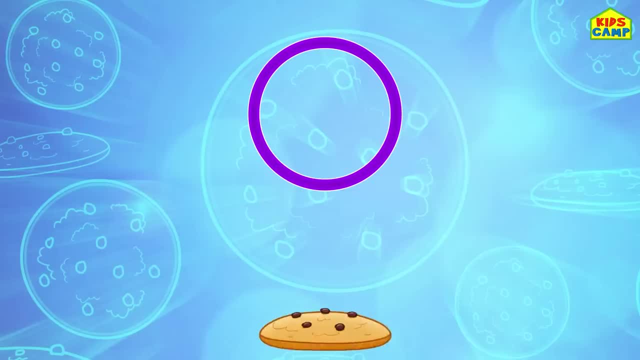 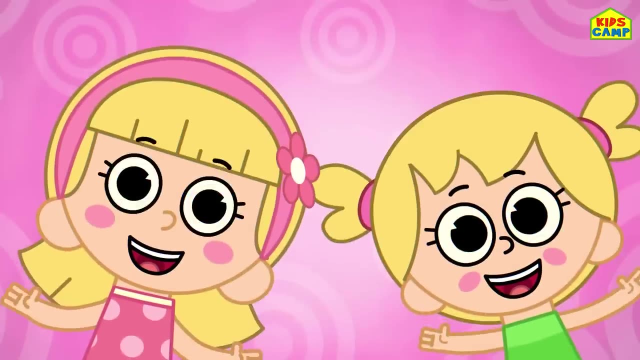 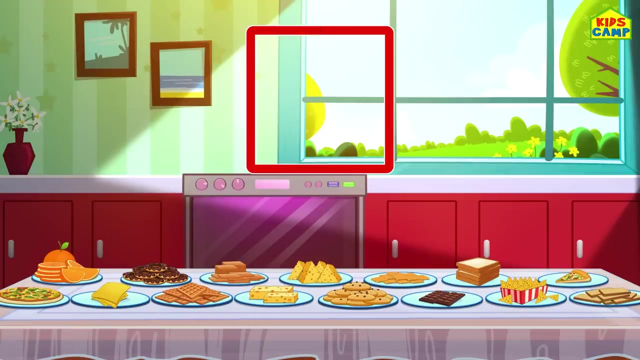 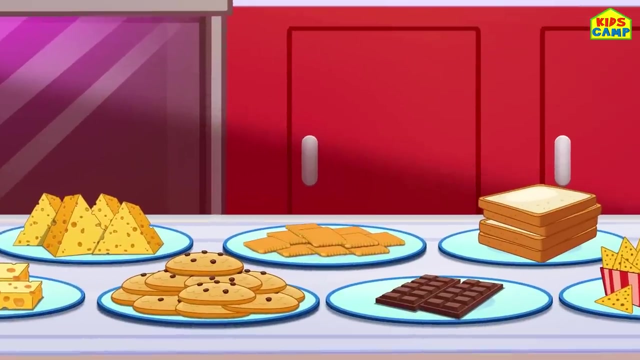 Hmm, A cookie. Yummy, A cookie is also a circle. Yay, What's the next shape? A square. Hmm, Can you find a square? kids, What food is in the shape of a square? Hmm, That's right, A craggle. 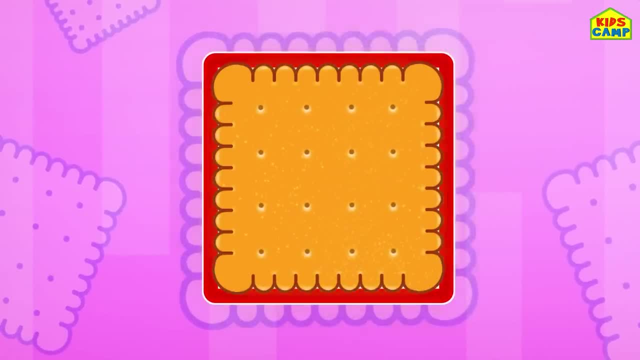 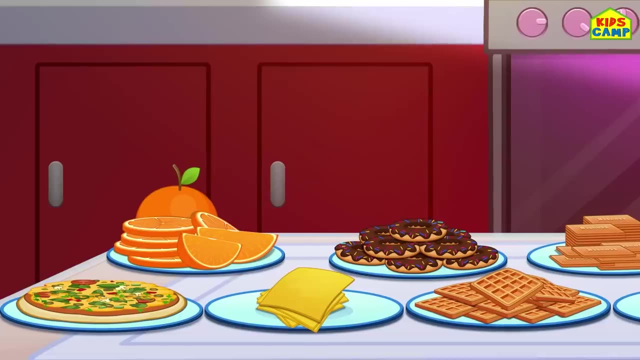 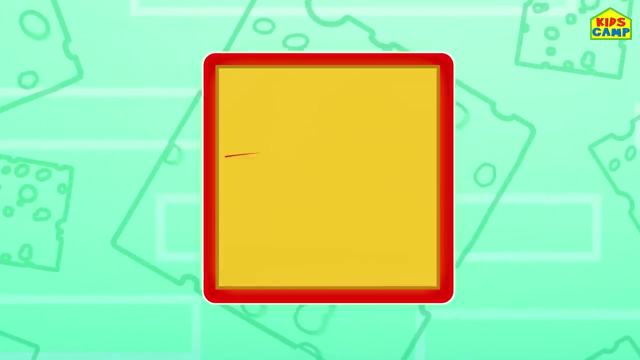 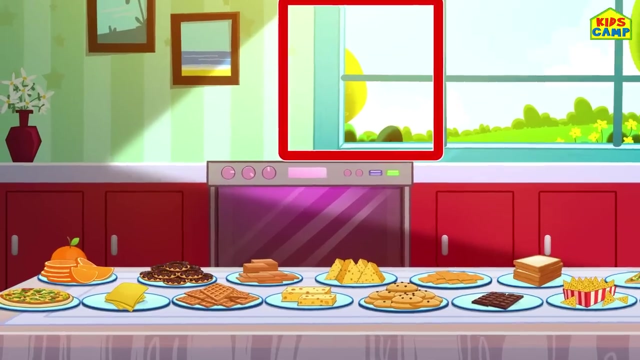 Yummy, That's the shape of a square. What else can we find that's a square? Aha, A slice of cheese. That's right, A slice of cheese is also a square. What else is a square? Aha, I see it. 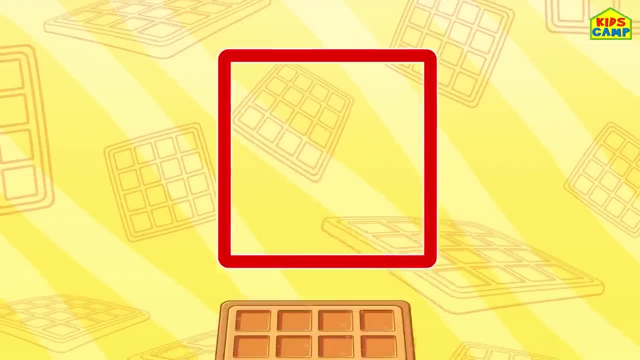 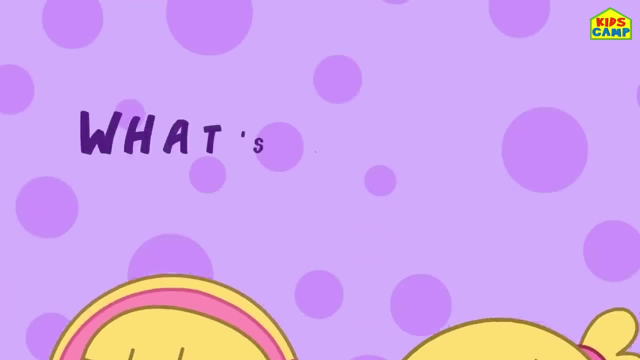 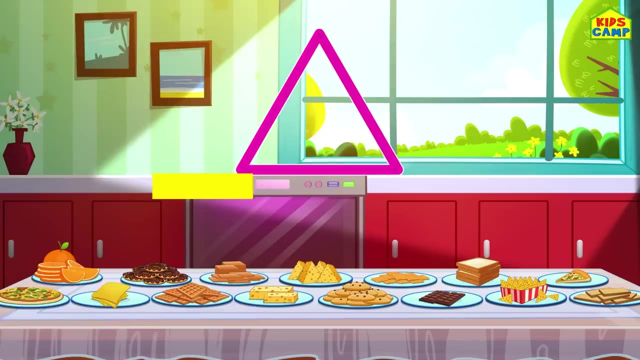 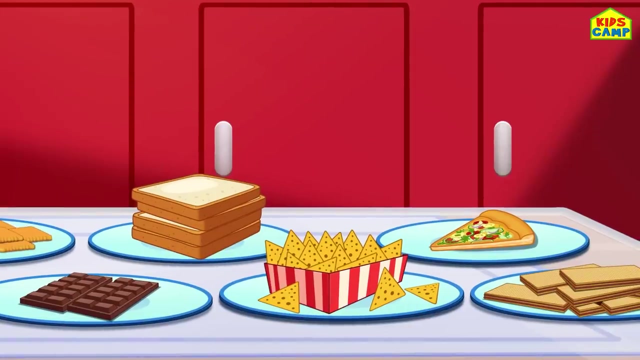 A waffle. A waffle is in the shape of a square, Yay. What's the next shape? A triangle. What's the next shape? A triangle. Can you find a triangle? Hmm, Do you see it? I see it too. 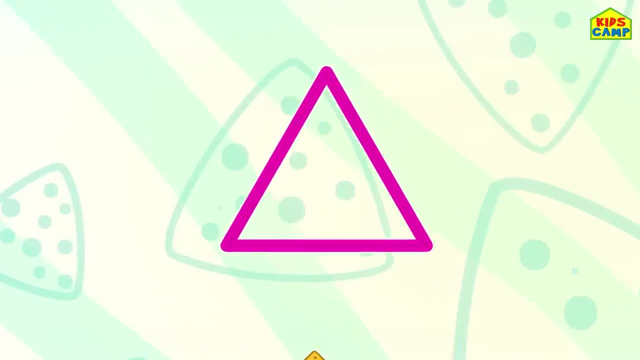 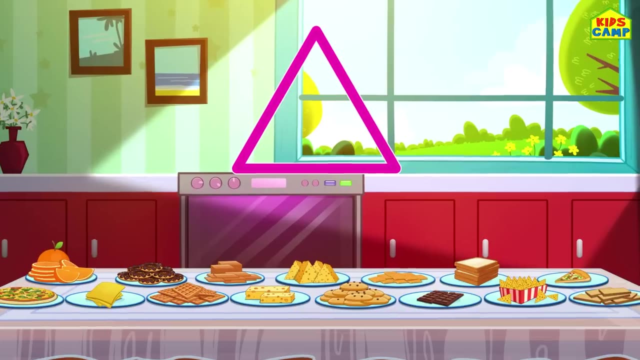 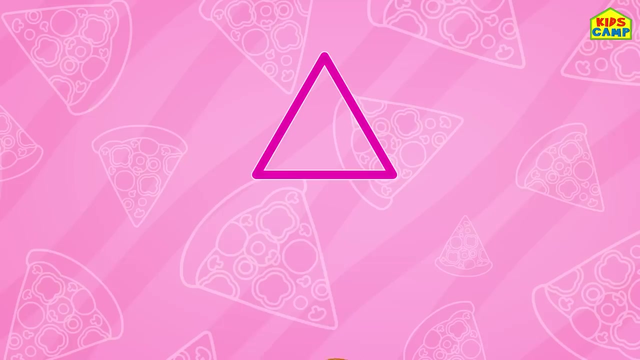 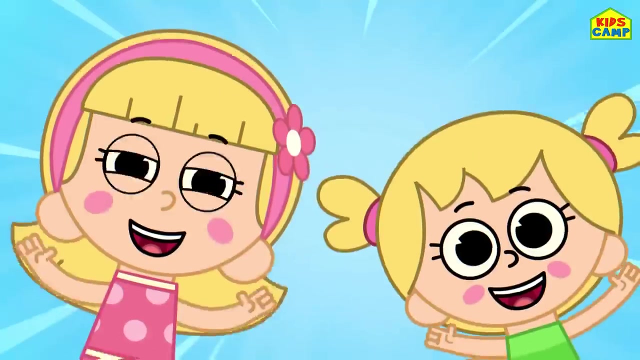 Nachos. A nacho is in the shape of a triangle. What else That's right? Everyone's favourite, A slice of pizza? Woohoo, That sure is a triangle. Yay, What's the next shape? A rectangle. 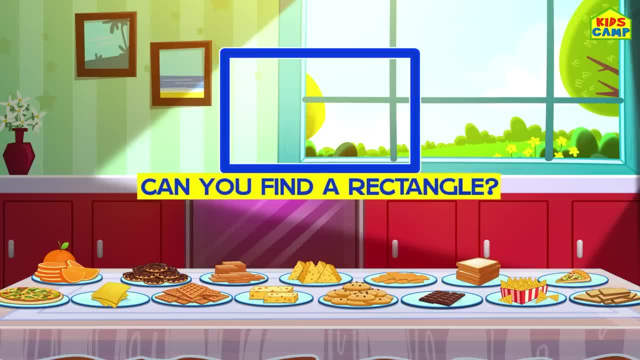 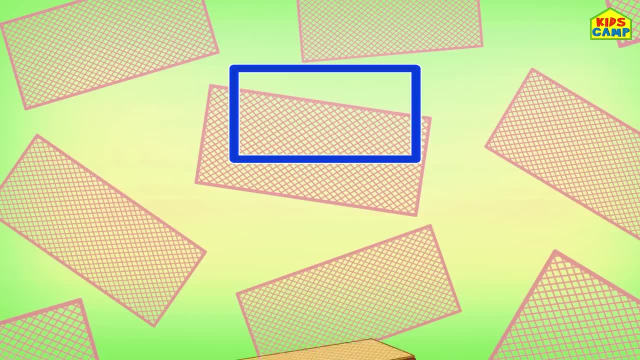 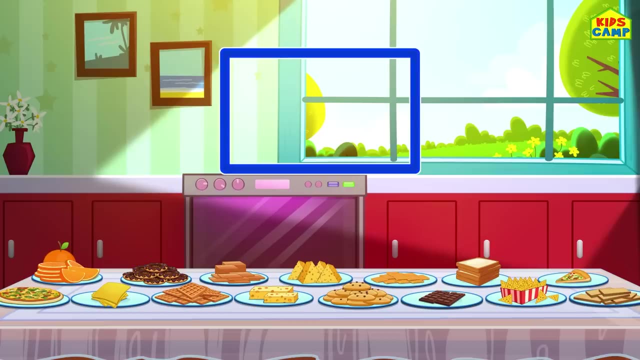 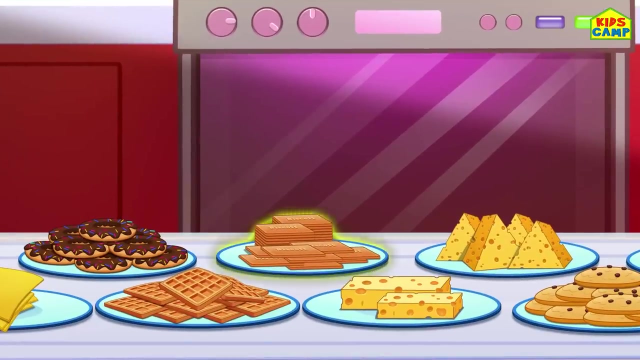 Can you find a rectangle, kids? Hmm, Ah, I see it too: A chocolate wafer. That's right, That also is a rectangle. Yay, What else? Hmmm, What's that? Yummy Biscuit. 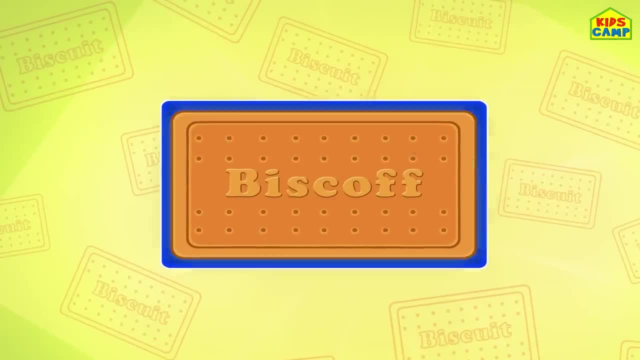 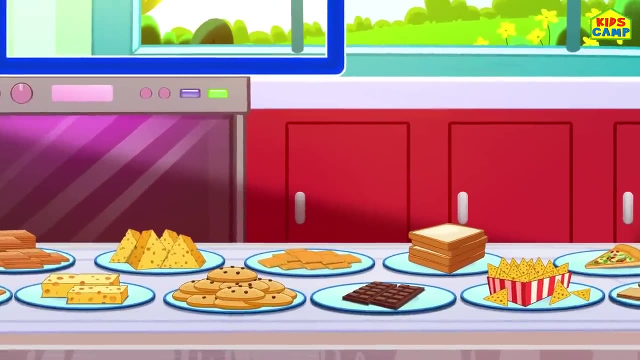 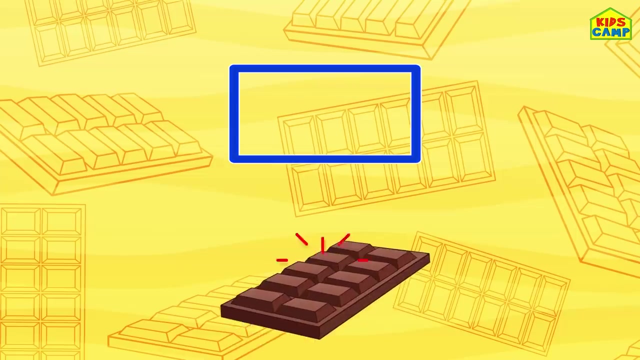 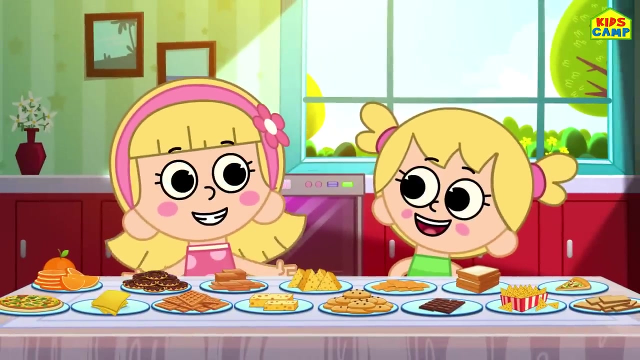 That sure is the shape of a rectangle. Anything else. Aha Chocolate, Woohoo, A bar of chocolate. That's right, kids, We did it. This all looks so good and we found all the shapes. Good job, Eva. 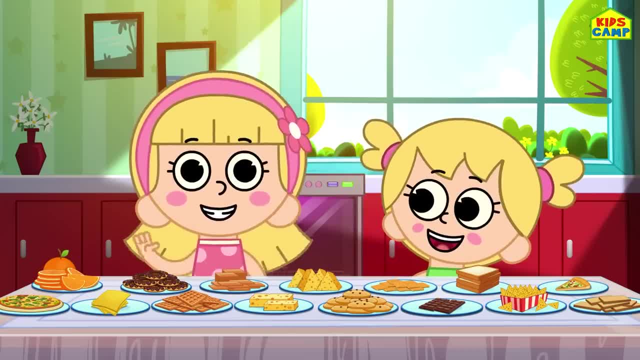 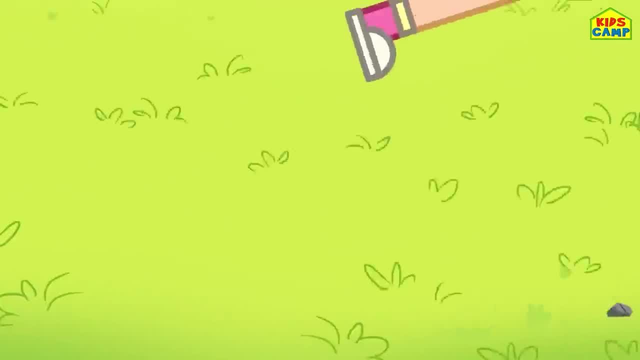 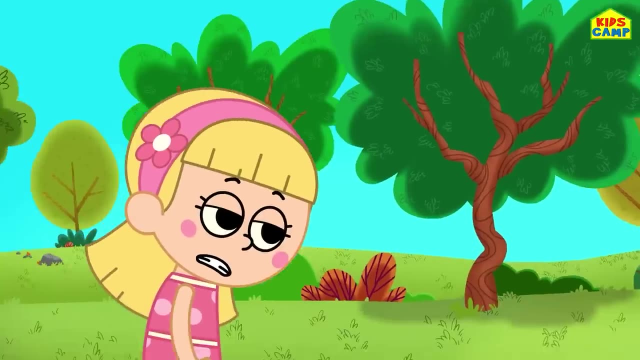 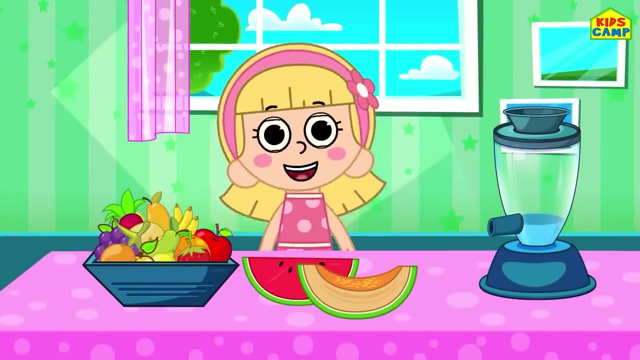 Good job, kids. Bye, bye. What a perfect sunny day to play outside, Oh yay. What should we do to beat this heat? I know Let's make summer coolers. Hey friends, what fruit should we pick first? A scrumptious apple. 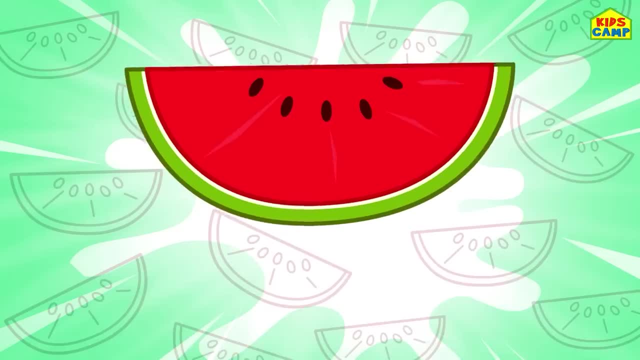 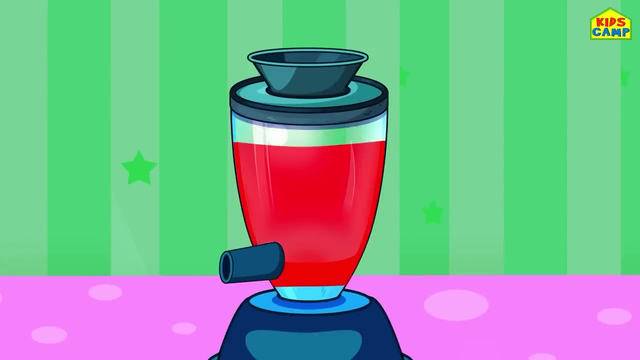 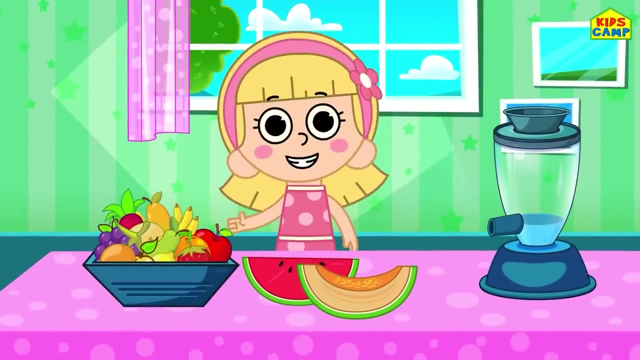 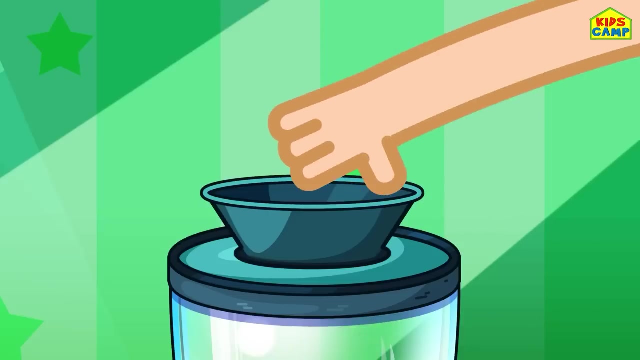 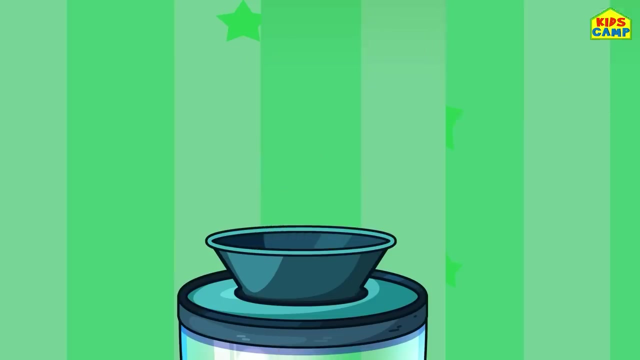 A yummy strawberry And a juicy watermelon. Let's blend them up. Yay, A red cooler. Let us give them another go. I'm going to take a yummy papaya, an orange and a juicy melon: In they go. 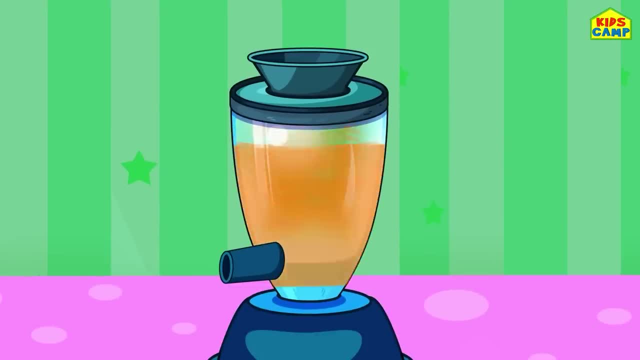 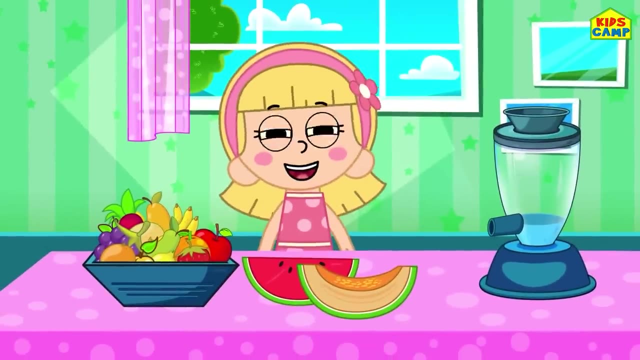 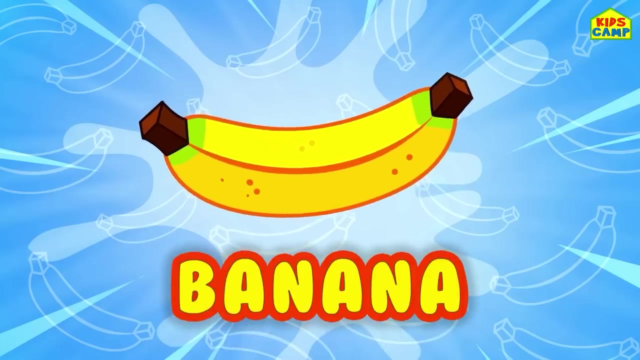 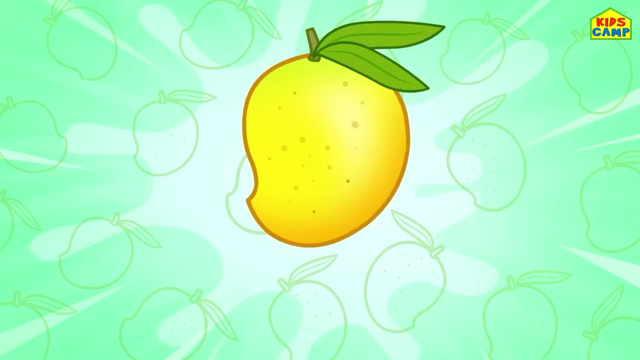 Let's mix them up. Woohoo, An orange cooler. Yay, Let's try another one. This time I'm going to take a banana and a pineapple and a yummy mango. Woohoo, In they go. 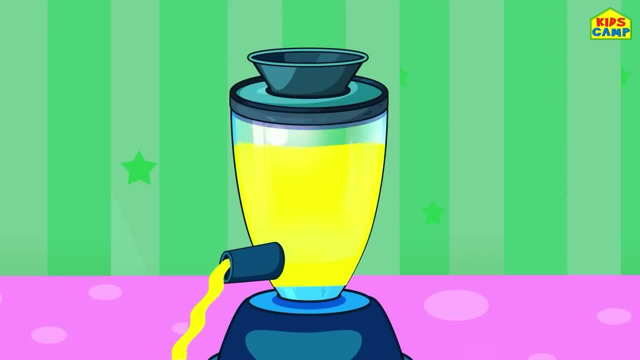 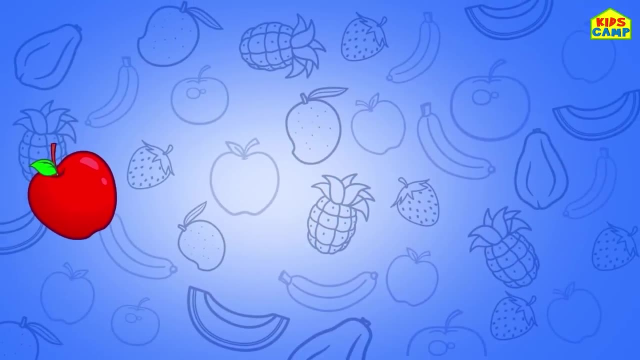 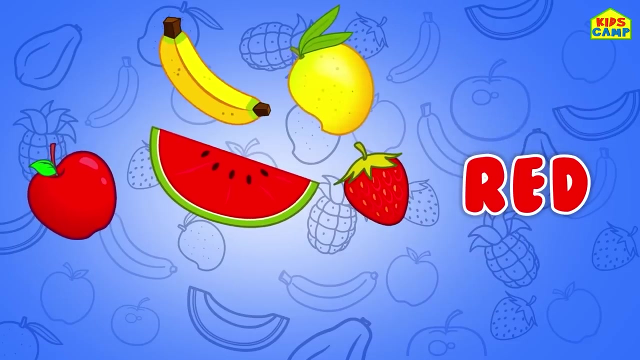 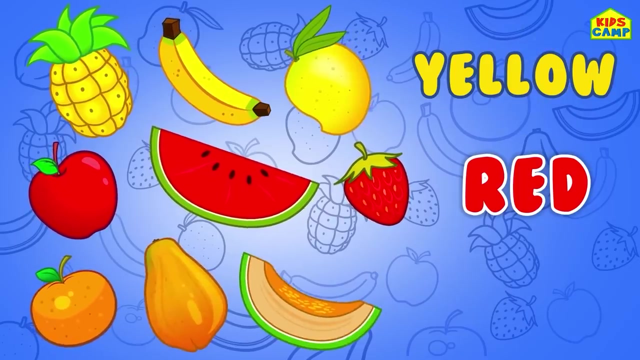 Let's mix them up. A yellow cooler. Wow. Today we learned that apples, watermelons and strawberries are red Mangoes, bananas and pineapples are yellow Oranges, papayas and melons are orange in color. 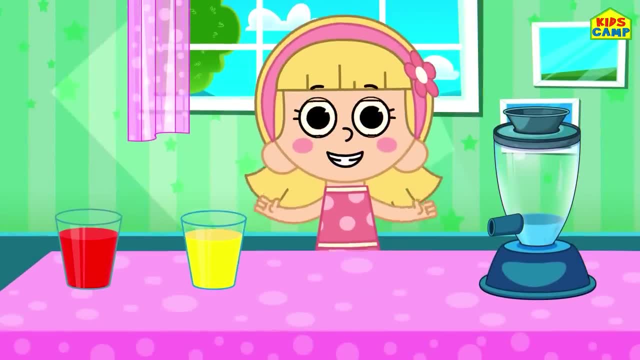 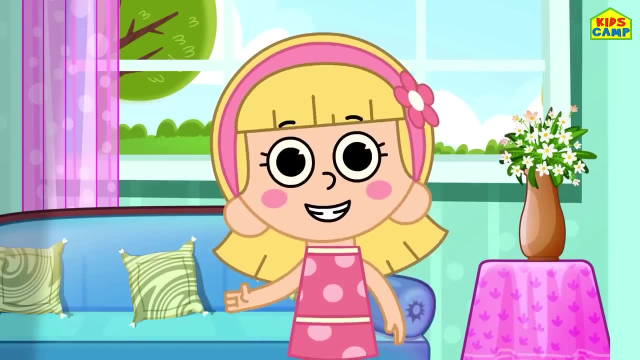 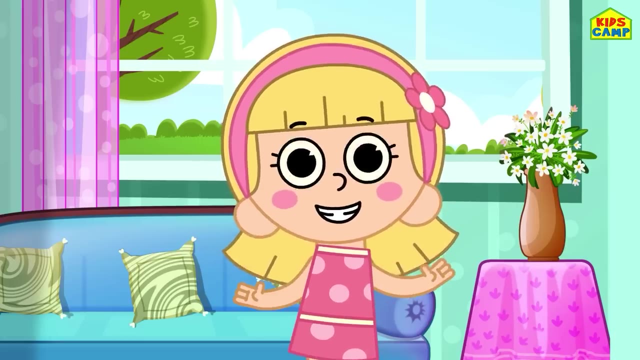 We had a fun learning day And delicious summer coolers to drink. Yay Hi, I'm Ellie, And today we're going to play a fun game with colors. That's right, We all love colors, Don't we? We have to find all the different types of colors. 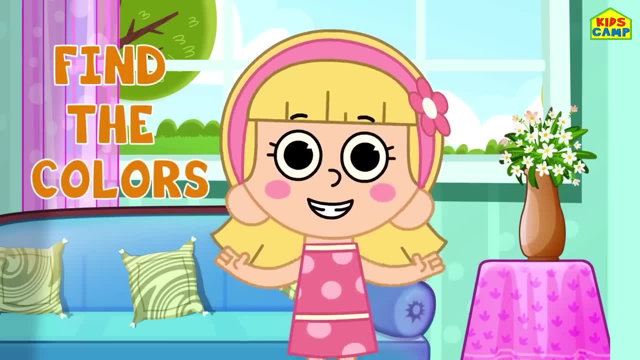 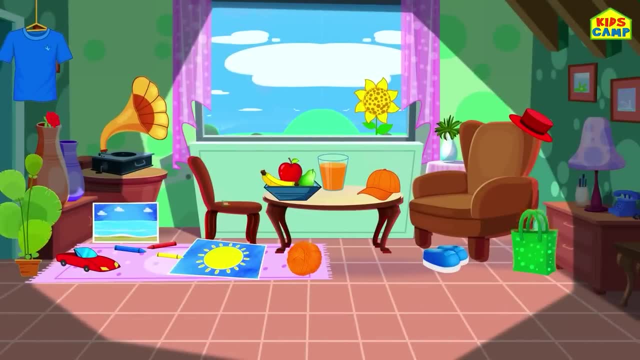 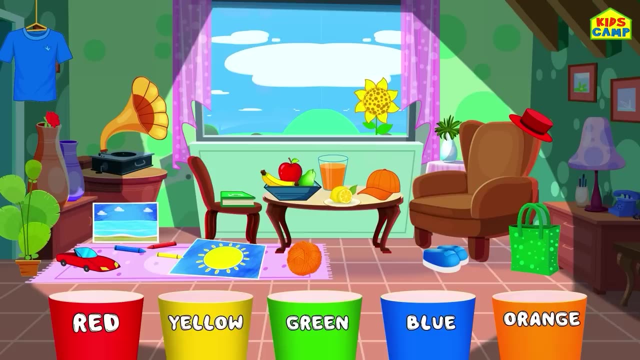 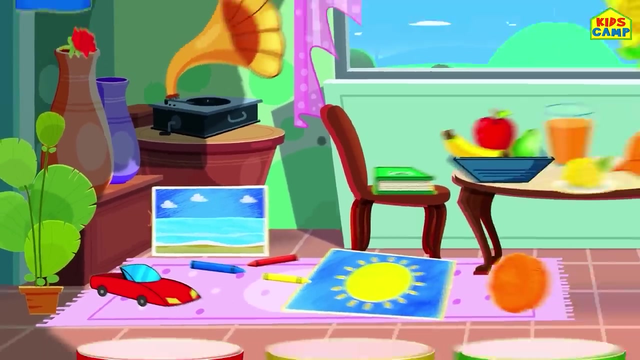 as mentioned on the buckets. The first color that we have to find is Red, Red, Red. Can you spot everything red? Let's get started. Can you find anything red? Umm, That's right, A toy car. Yes, It's red. 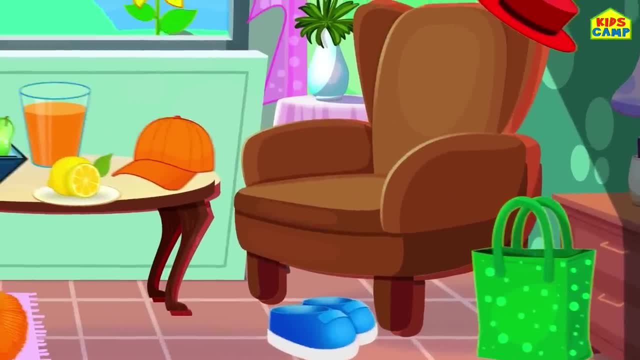 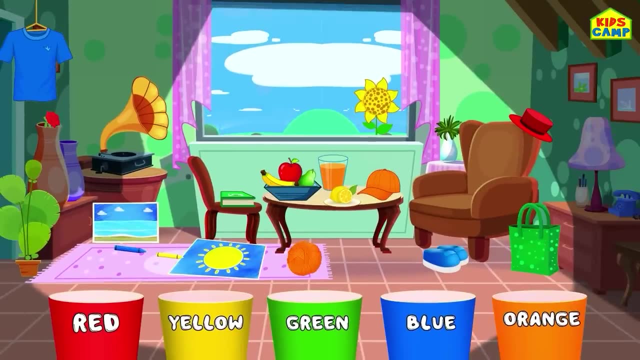 Let's add it to the red bucket. What next? What else is red? Uh-huh, I see a red crayon. That's right. Wow, A red rose. What else is red? An apple. We'll add that to our red bucket. 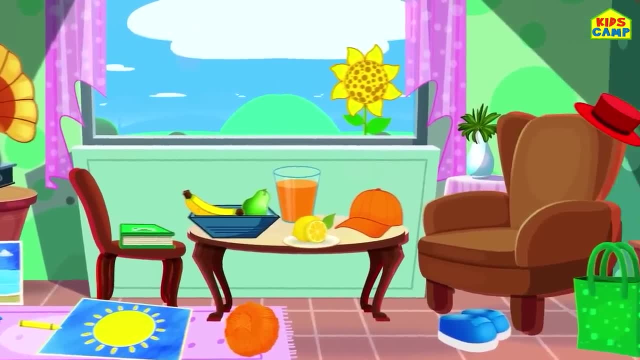 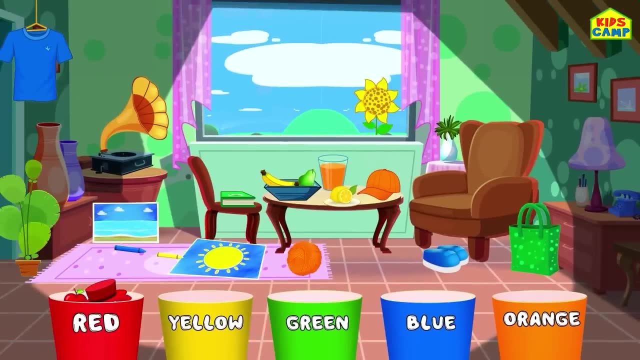 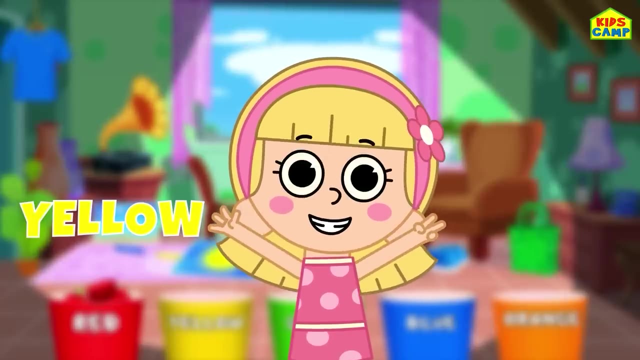 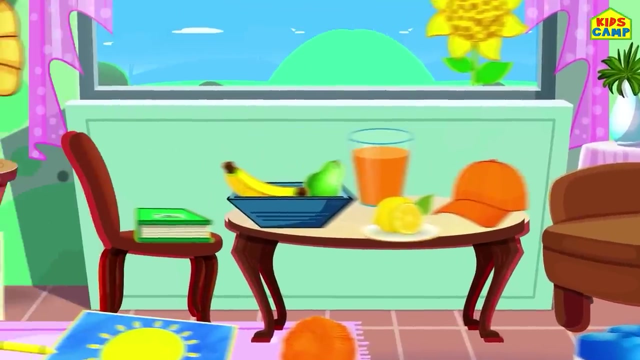 Keep looking for something else that's red. That's right, A red hat. Woohoo, We found everything that was red. What's the next color? Yellow, My favorite. What do you see that's yellow? Uh-huh, My drawing of the sun. 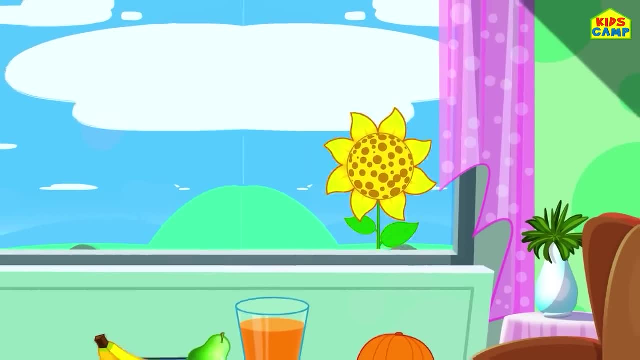 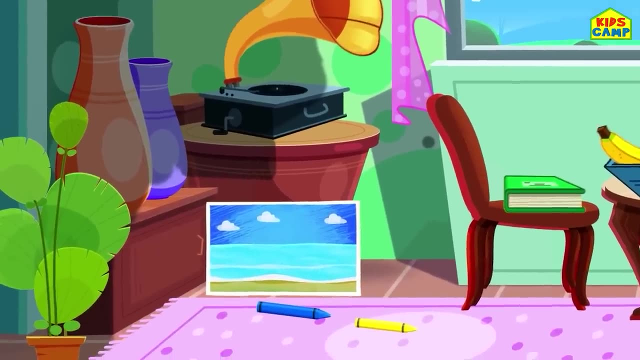 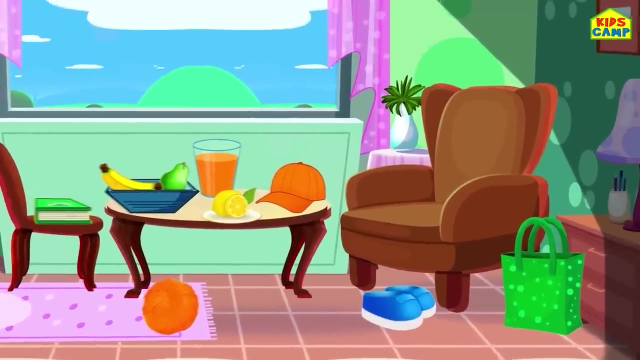 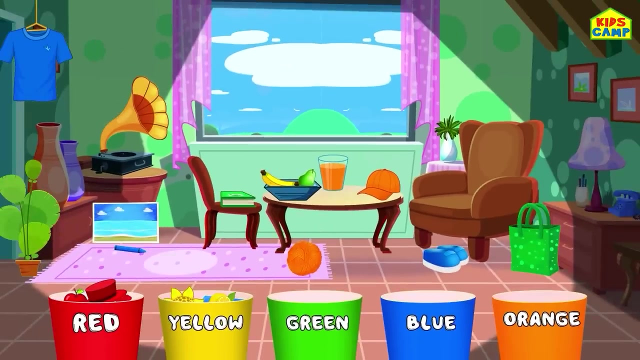 The sunflower, That's yellow too, Into the bucket. Good job, friends. What else is yellow? A yellow crayon, That's right. What else do you see? Uh-huh, Lemons, Wonderful, What else? Uh-huh, A banana. 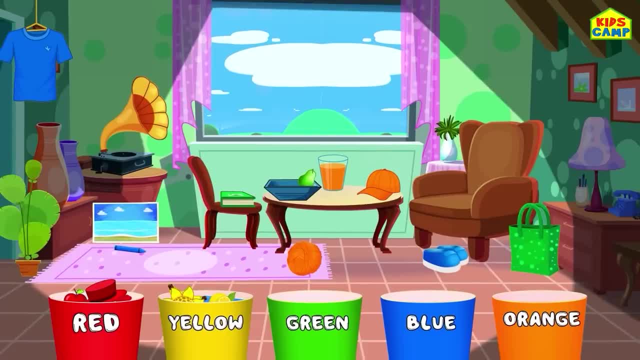 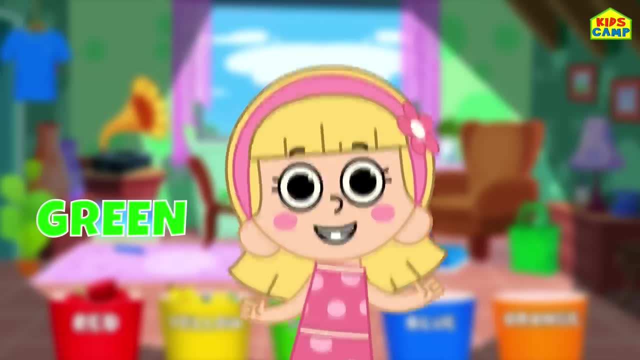 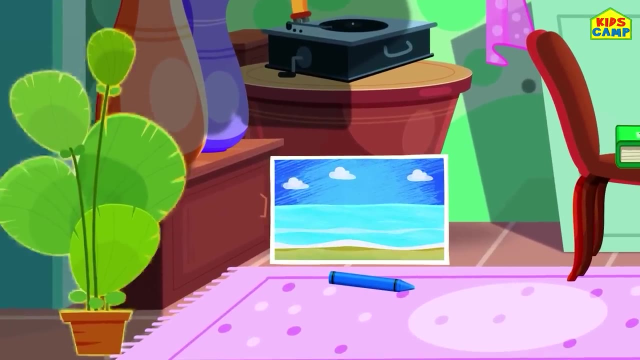 The banana is yellow. Into the yellow bucket, it goes. Let's go to the next color, Which is Green. Can you look for something that is green in my room? Uh-huh, I see it. The plant Into the bucket, it goes. 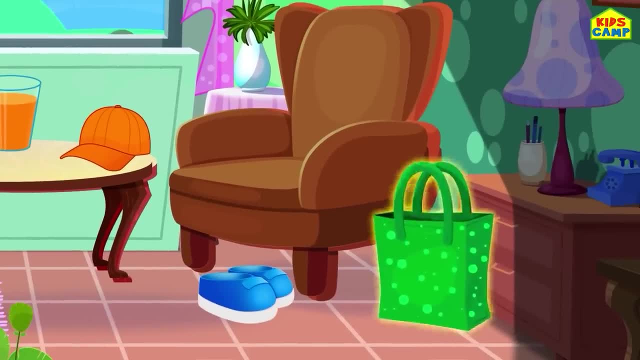 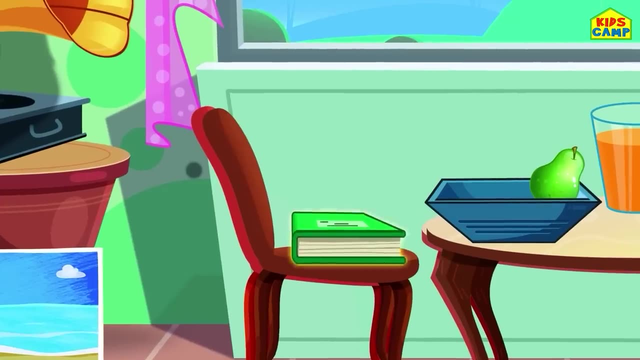 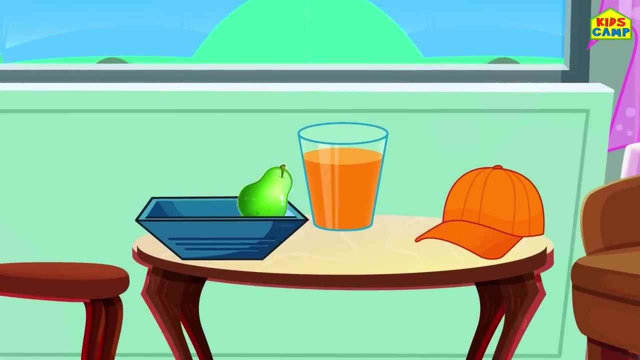 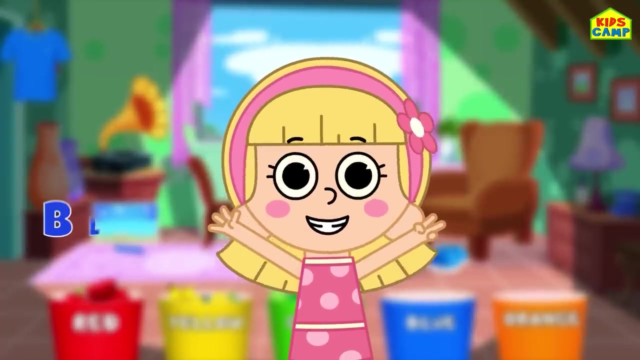 What else is green? That's right, The green bag, Anything else? I see it too. The green book, Woohoo, What else? The pear? That's green too. Into the green bucket. Yay, Let's move on to the next color. 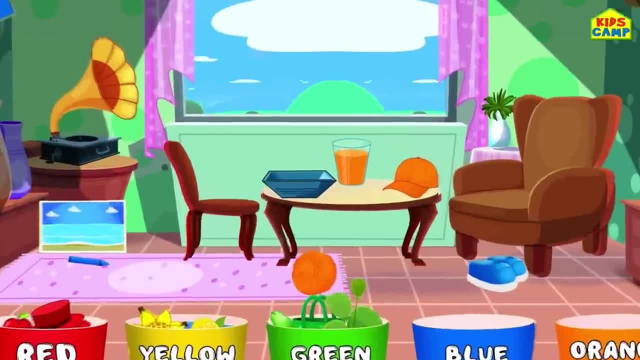 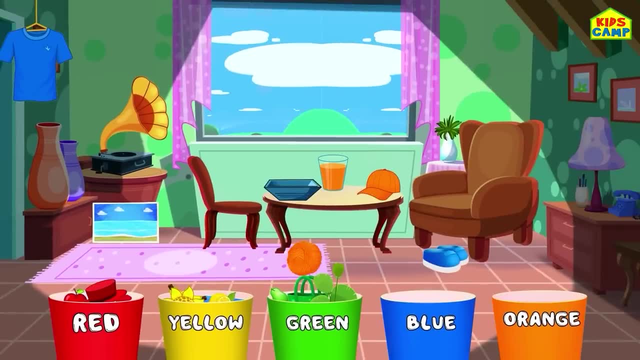 It's blue. Woohoo. What's blue colored here? The blue crayon, Anything else? My drawing of the blue sky, What else? The blue t-shirt Into the bucket. Uh-huh, I see My pair of blue shoes. 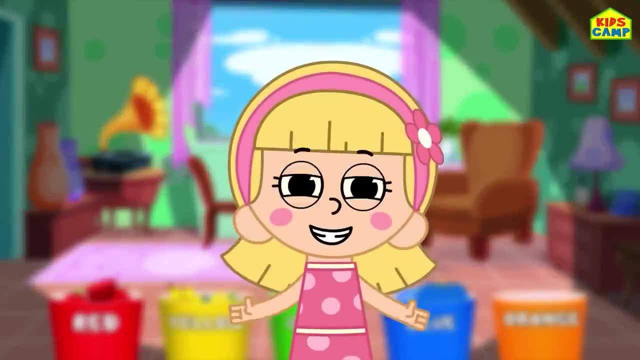 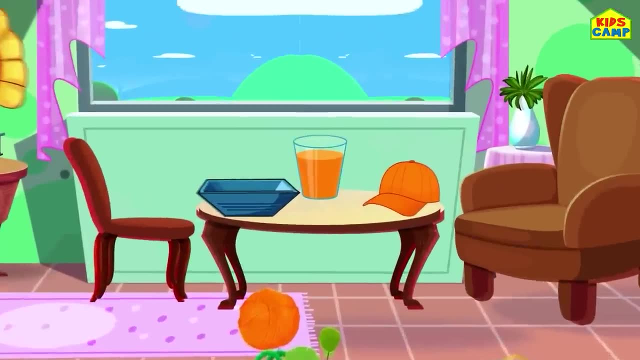 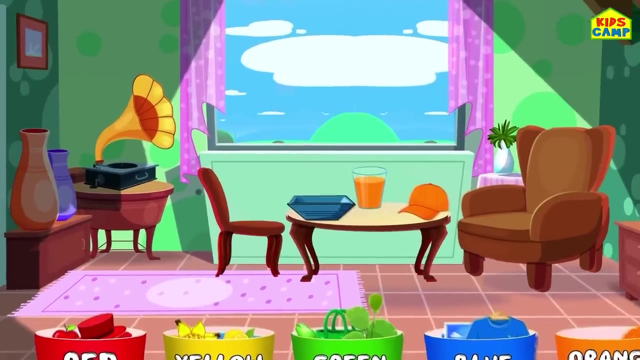 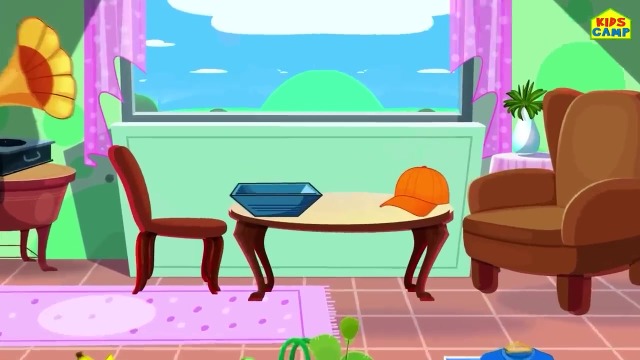 We found everything blue. What's next? It's orange. That's right. Can you spot something orange? An orange yarn of wool, That's right. What next? I see it: A glass of orange juice And an orange cap. 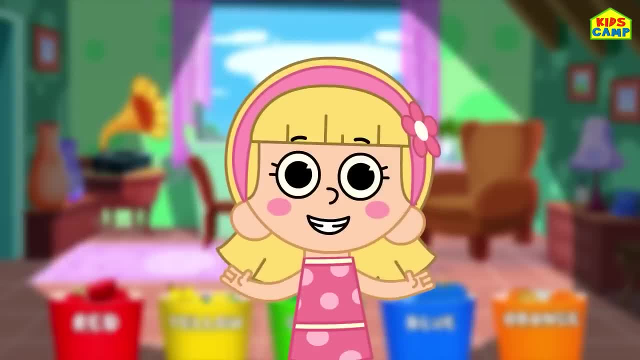 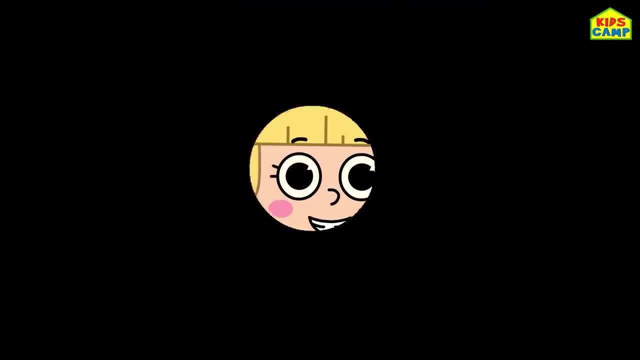 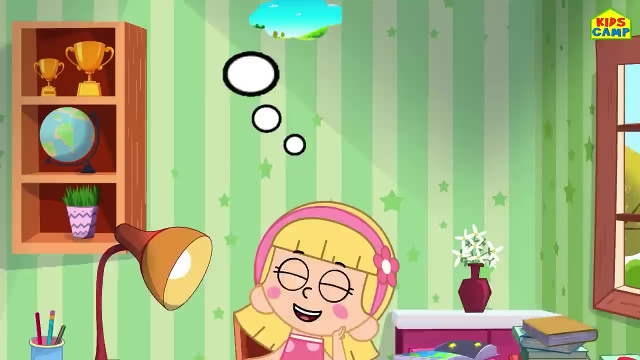 Yay, Into the orange bucket it goes. Wonderful kids, We found all the colors. Bye, Hi friends, I'm Ellie. Let's play a fun game where we match the pairs. Let's match the professions to their vehicles. What vehicle? 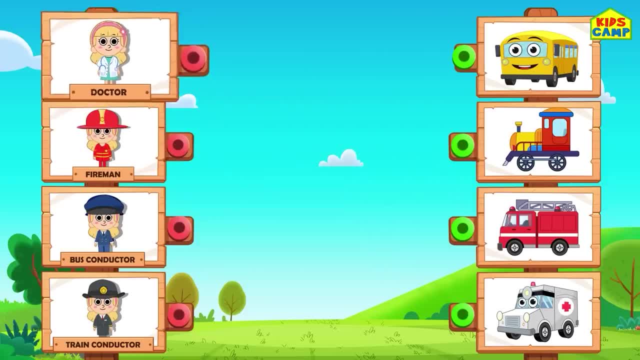 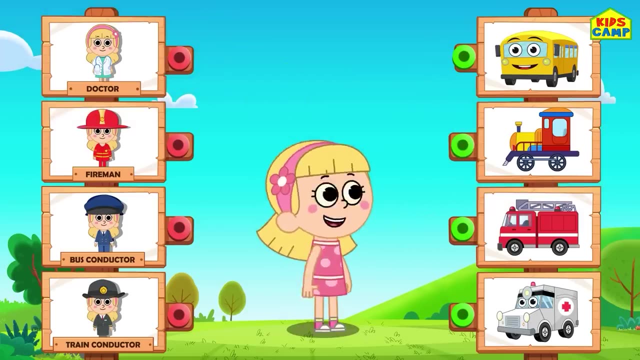 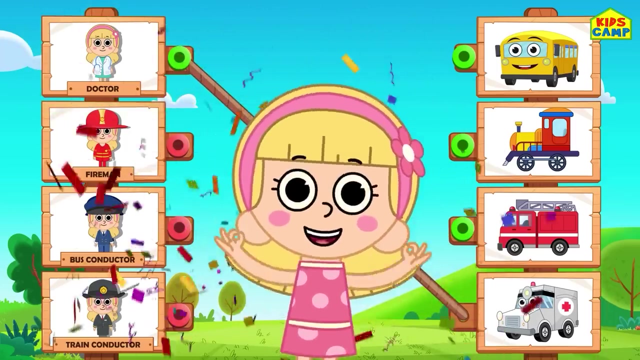 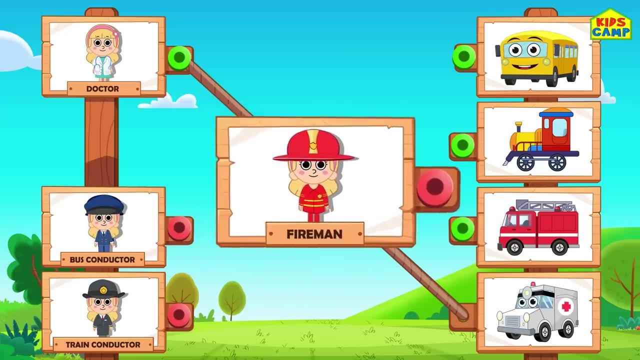 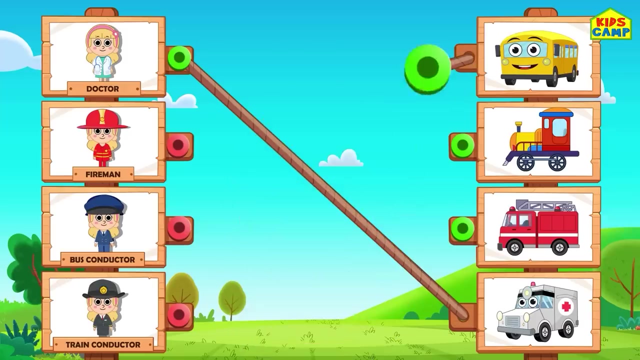 What vehicle will a doctor use? A fire truck? No, A train. No, I know The doctor will use an ambulance. That's right, Yay. A fire fighter will use Which vehicle? Hmm, A bus? No, no. 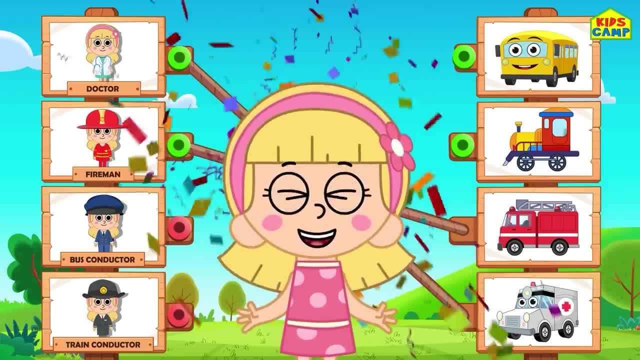 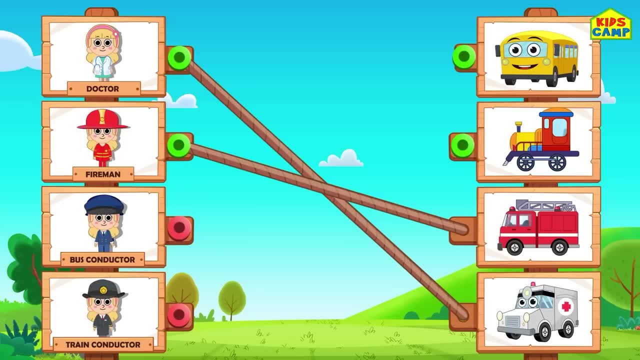 A fire truck, That's right. Yay, A bus driver will use a train, That's right. Yay, A bus driver will use a train, No A bus, That's right. Good job, friends. Yay, What's next? 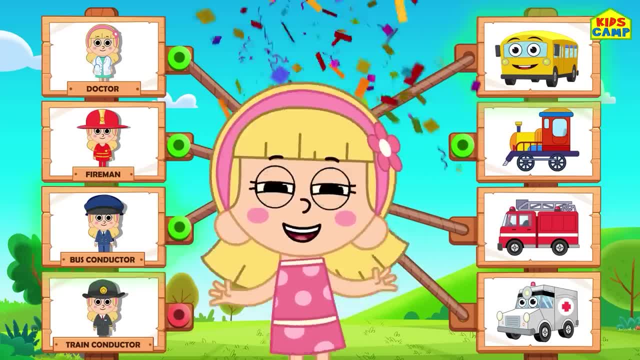 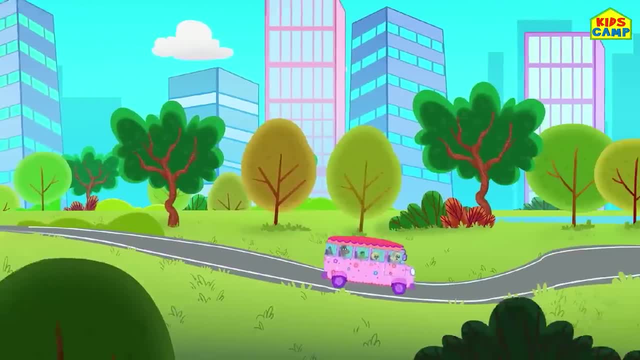 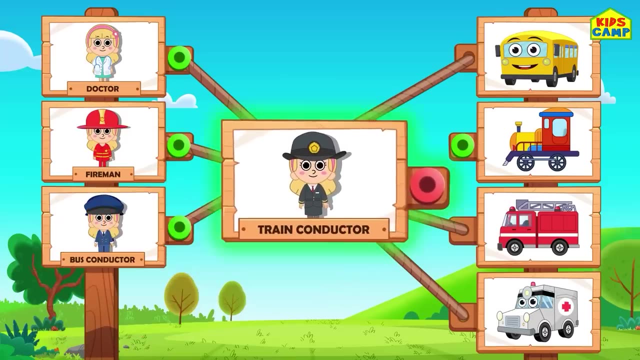 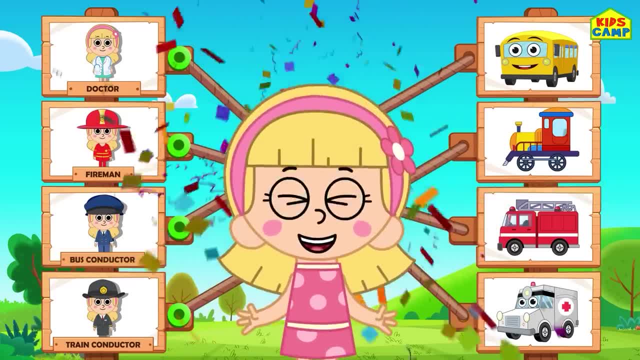 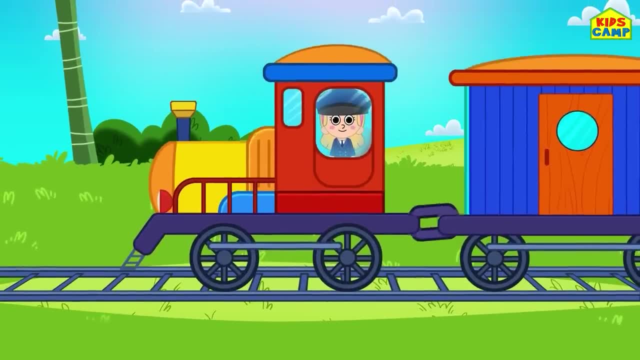 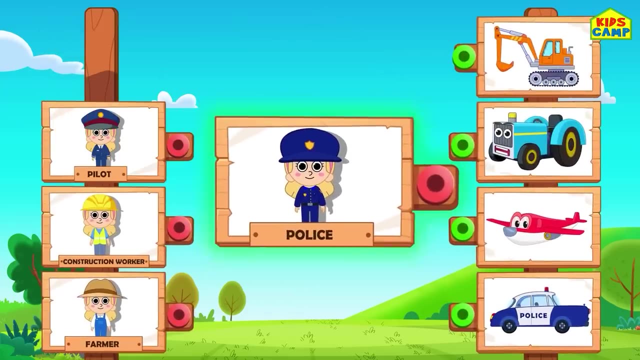 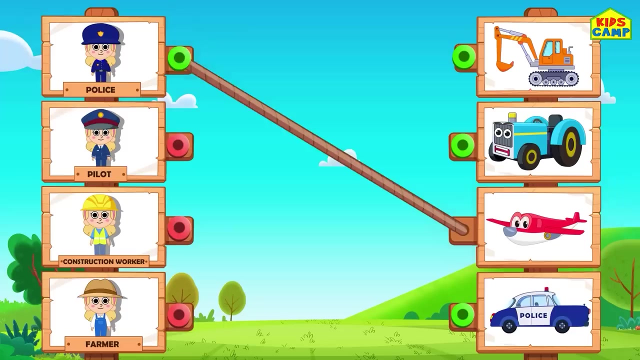 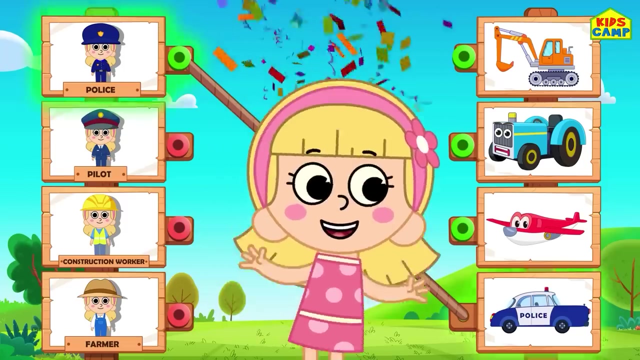 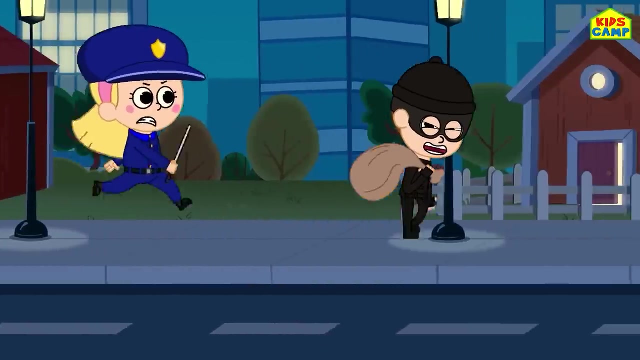 No, The trains, That's right, All aboard. Uuuh, Which vehicle will the police use? An airplane: No. A tractor, No Way. Hmm, I know A police car, That's right. Yay, A pilot will use. 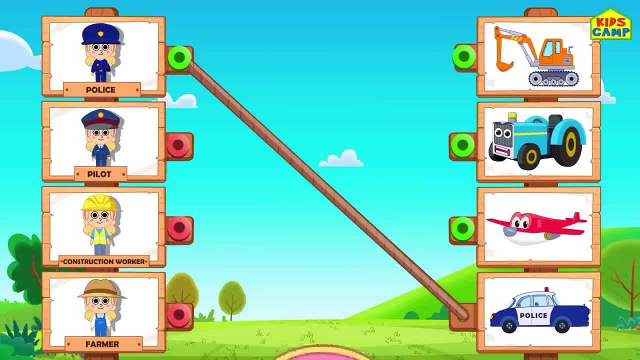 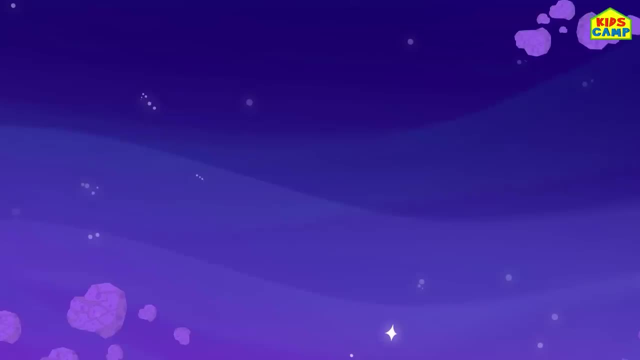 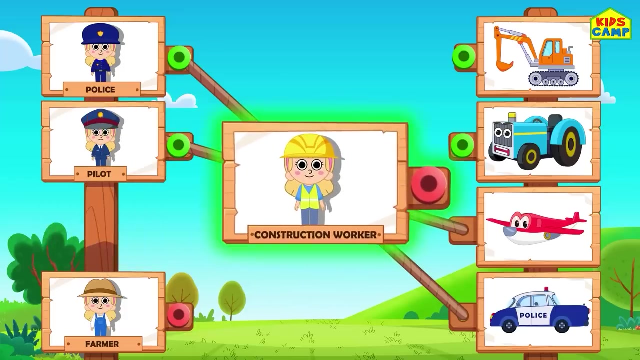 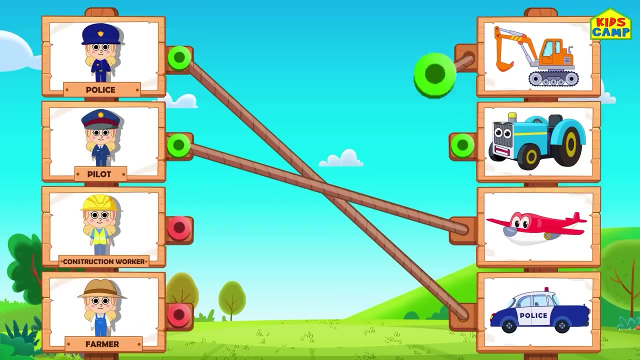 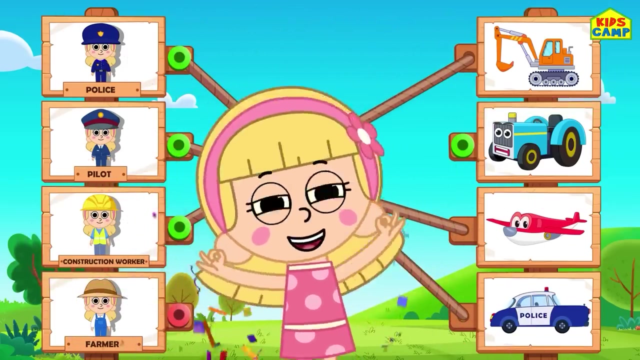 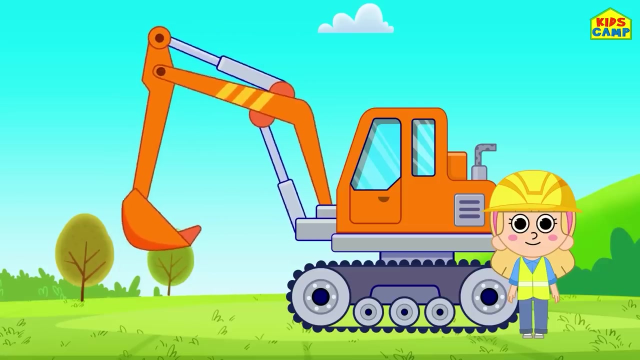 Which vehicle? Hmm, A digger. No, An airplane- Yes, Fly away. Yay. A construction worker will use. Which vehicle? A tractor? No, A digger, That's right, Yay. What vehicle will a farmer use? 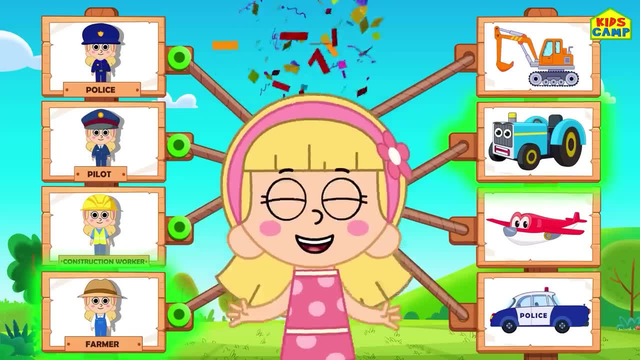 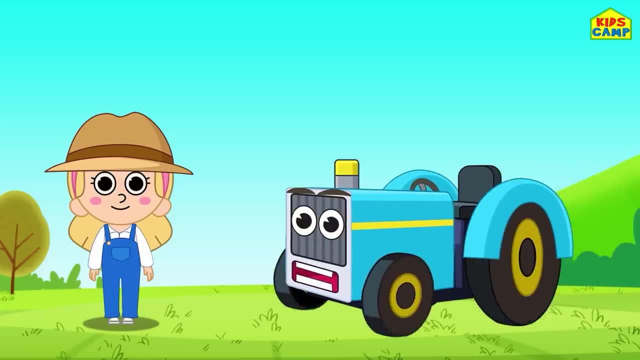 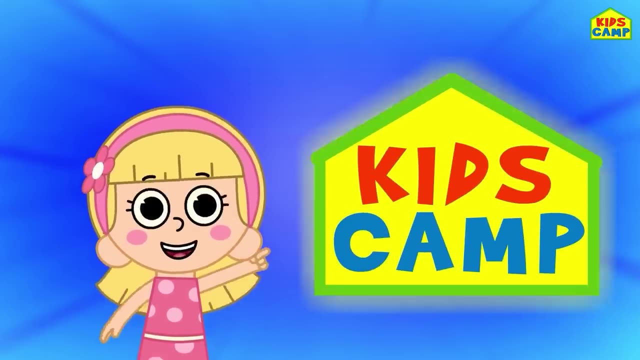 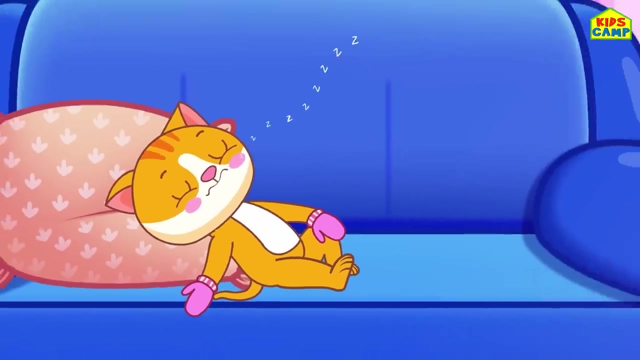 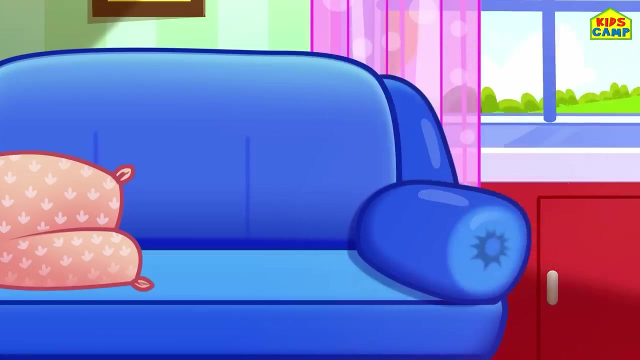 A tractor. That's right. Yay Superb. That was so much fun. Keep watching Kids' Camp. Bye, Good morning Kitty. Wake up, Let's brush your teeth Ready. What do we brush your teeth with? 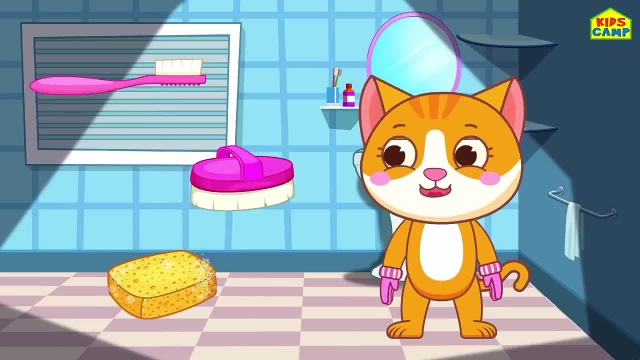 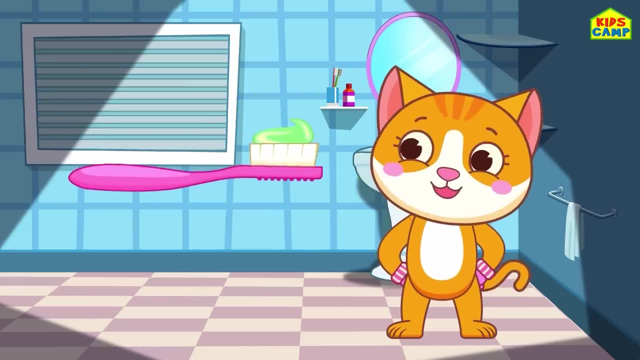 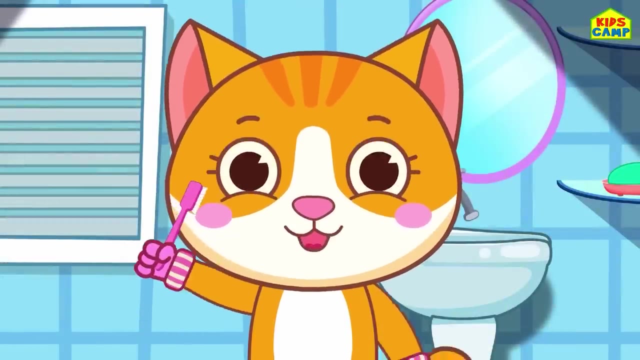 Is this a toothbrush? No, Is this a toothbrush? No, no. Is this a toothbrush? Yes, it is Yay, Yay, Wow. Your teeth are sparkling white. Now let's have a bath. What do we have a bath with? 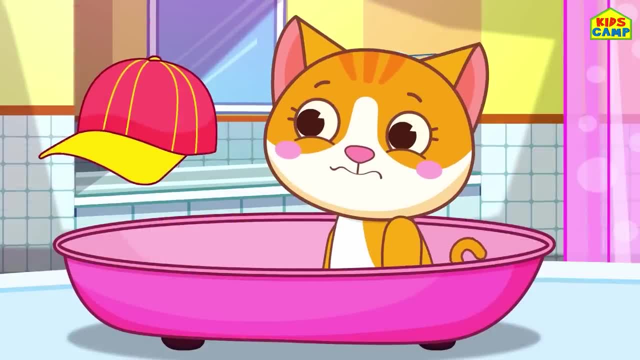 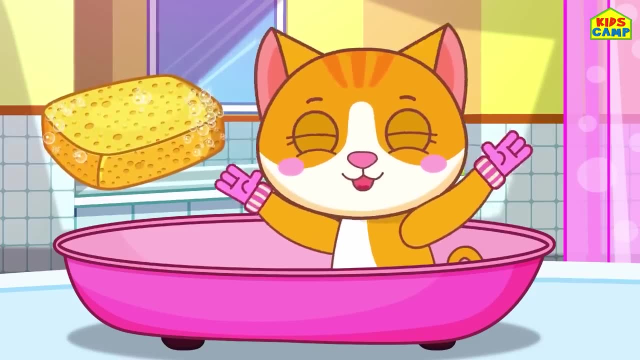 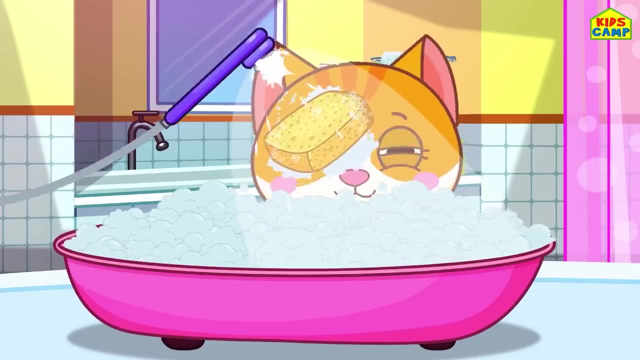 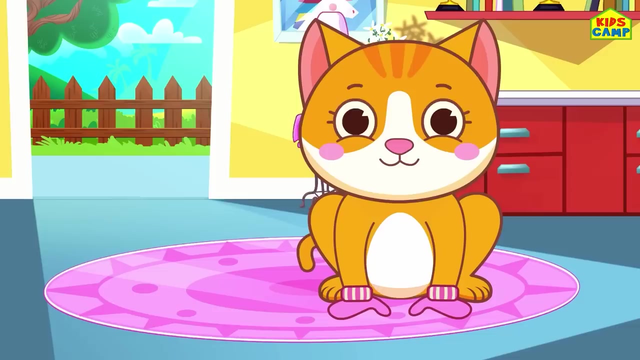 This one, No, This one, Definitely not This one. Yes, Don't you love taking a bath? Wow, You're neat and clean, Kitty. Now let's have breakfast. What do we have for breakfast? This one, No. 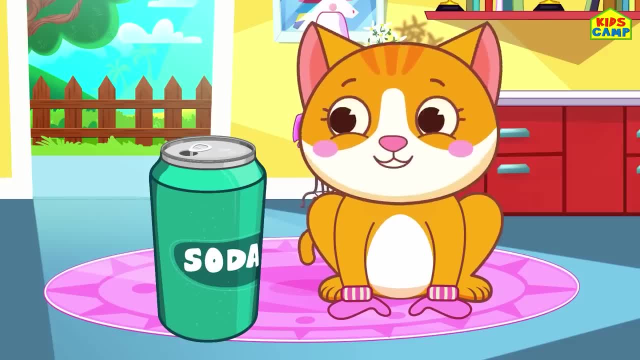 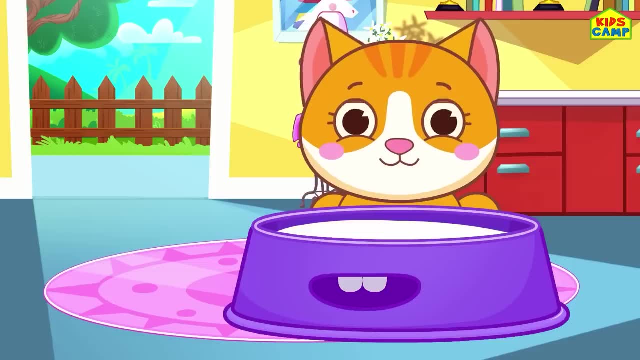 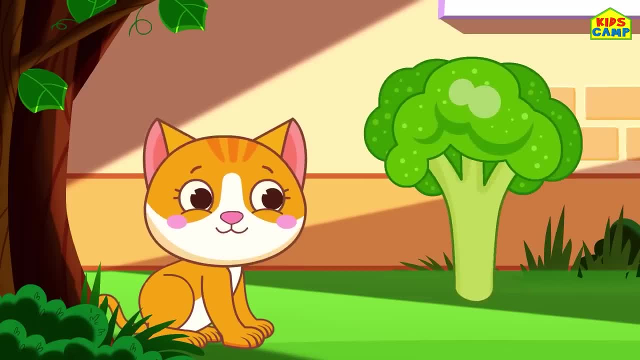 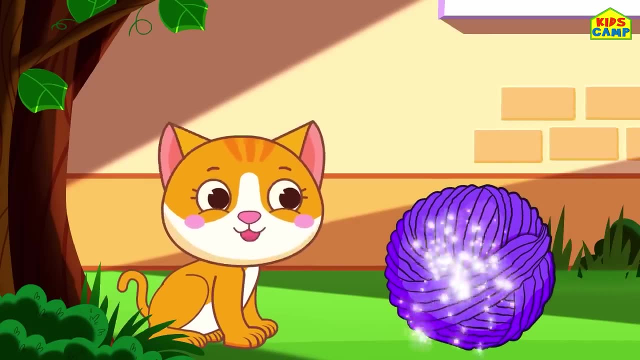 This, This, This, This. No, It's a broccoli. No, We can't play with this. It's a candy. Yes, We can play with this, It's a ball of string. Wow, So much fun. Now let's eat something. 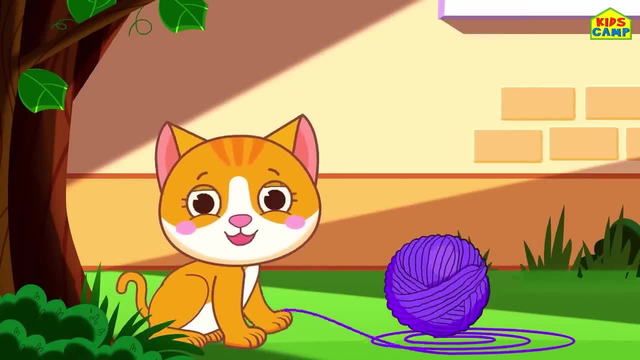 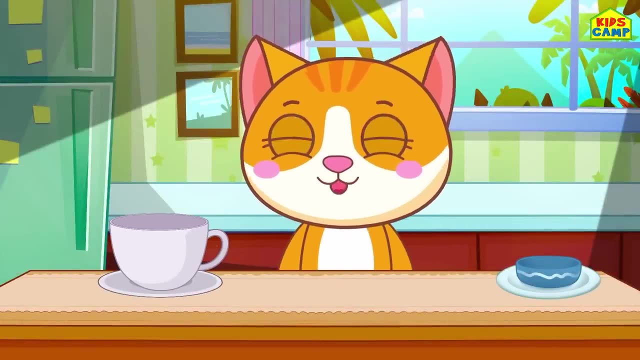 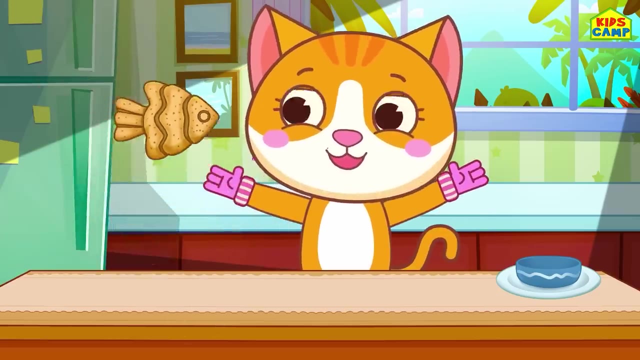 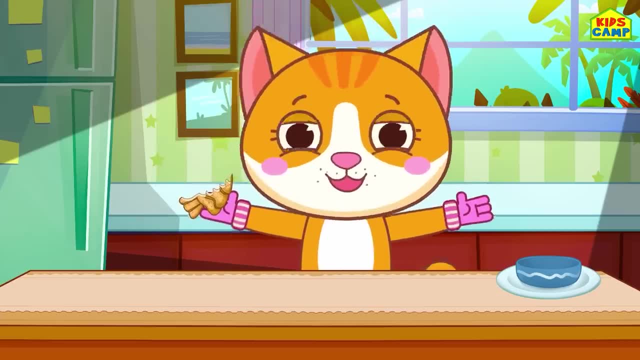 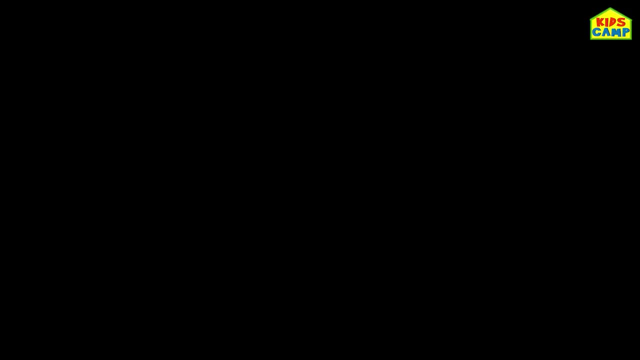 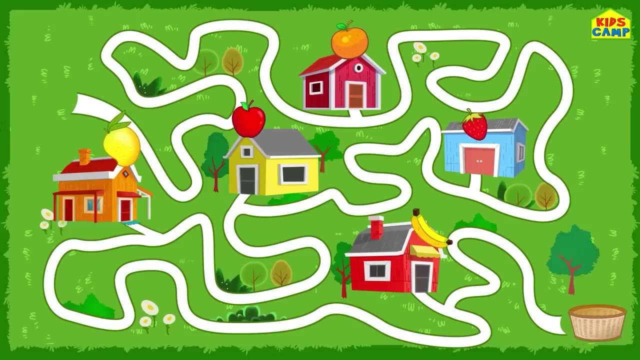 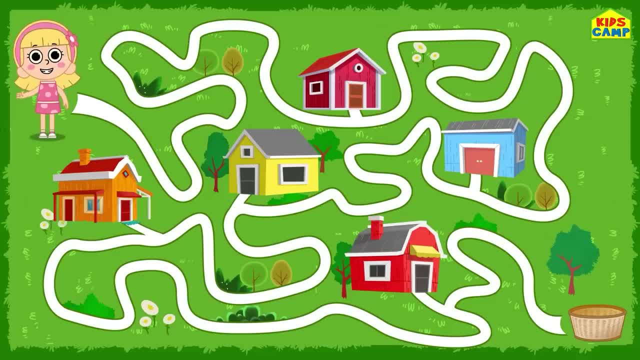 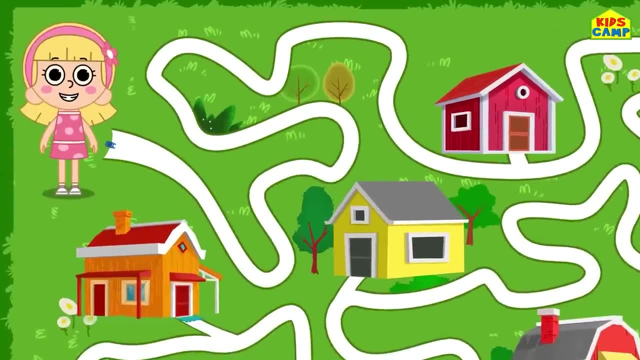 See you soon, Bye, Bye, Hi. I am Elli And I have to collect all the fruits into the basket. That's right, Feel free to help me out the door. No thanks, Come on. Here goes my cart. Let's collect fruits. 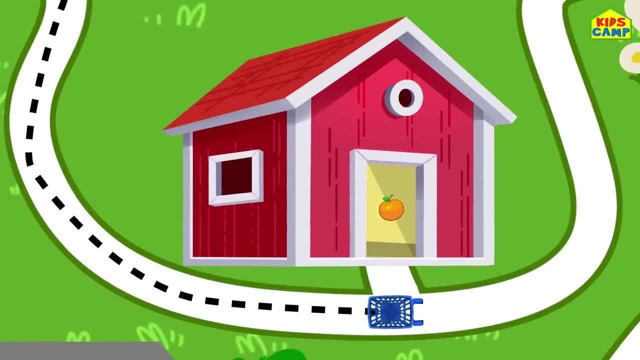 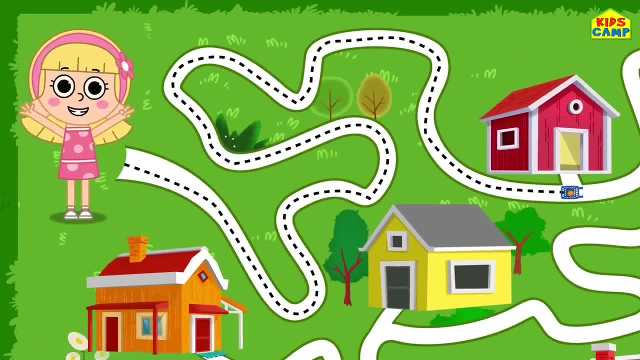 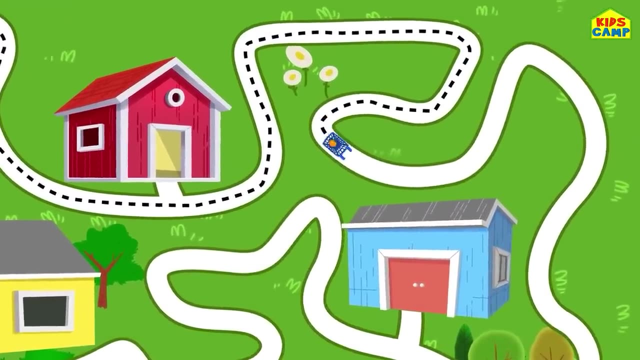 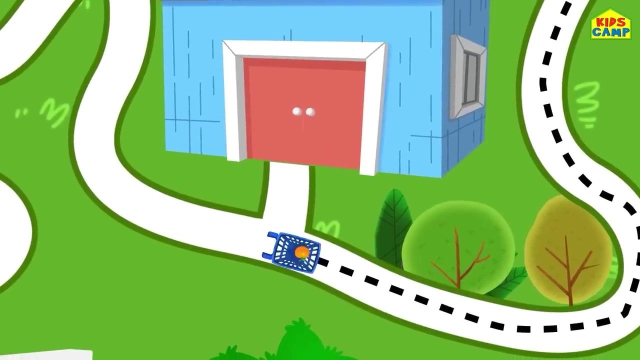 Knock knock, Hi. Do you have any fruit? Ooh, An orange Into my cart. Wonderful, Wonderful, Let's keep going. Ooh, Knock knock. Do you have any fruit? Aha, A strawberry Into the cart. 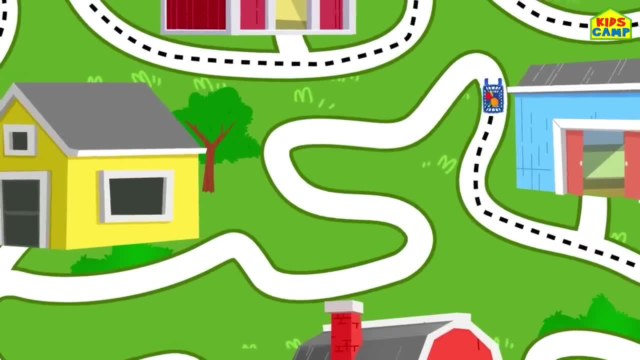 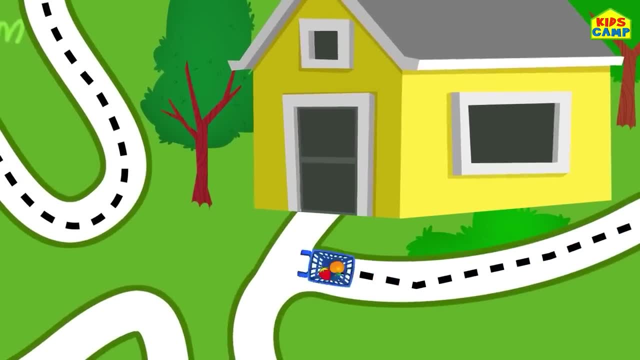 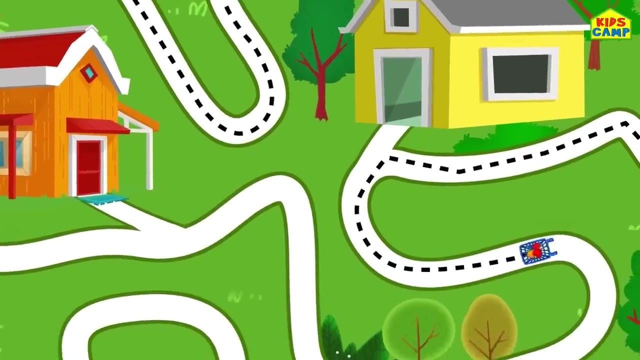 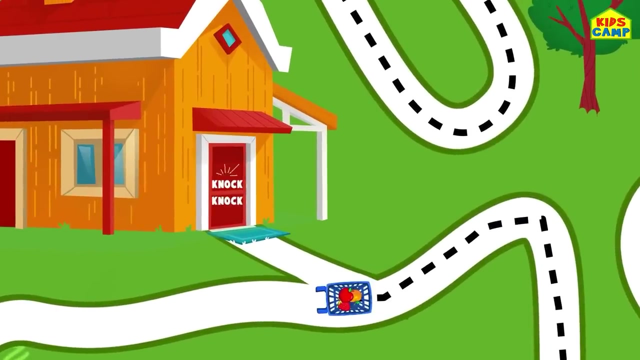 Wonderful, Let's get going. Knock knock. Hi, Do you have any fruit? Ooh, My favorite, An apple Into the cart. Yay, Let's keep going. Knock knock. Do you have some fruit? Ooh, A mango. 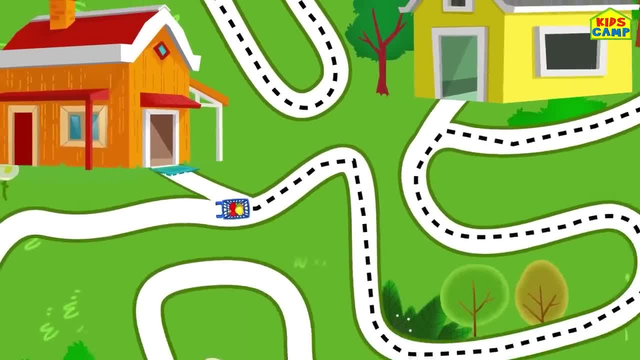 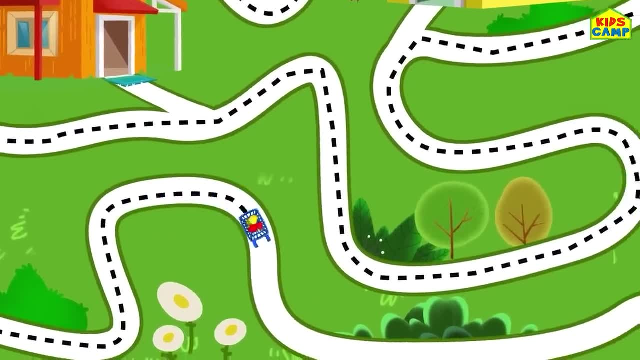 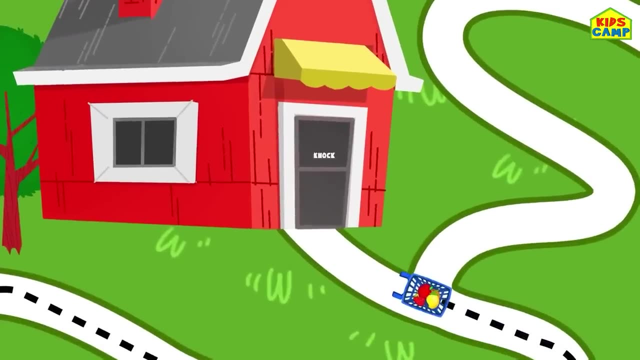 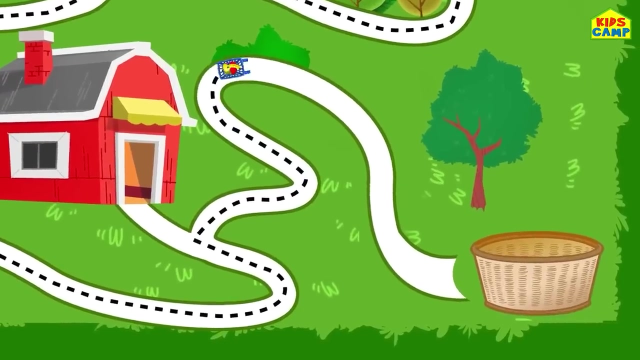 Into the cart, Let's get some more. Keep going, Knock knock, Knock knock. Hi, Do you have some fruit? A banana? Yay, Into the cart, Let's keep going. Yay, We've collected all our fruits. 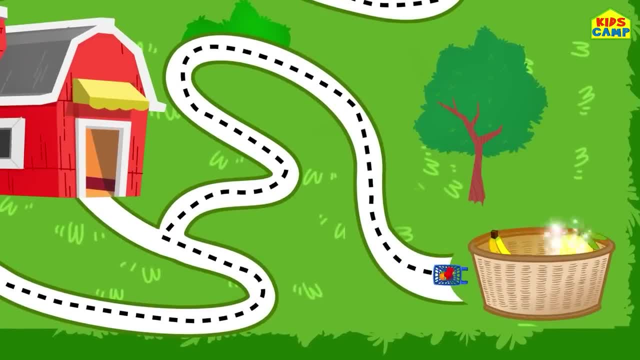 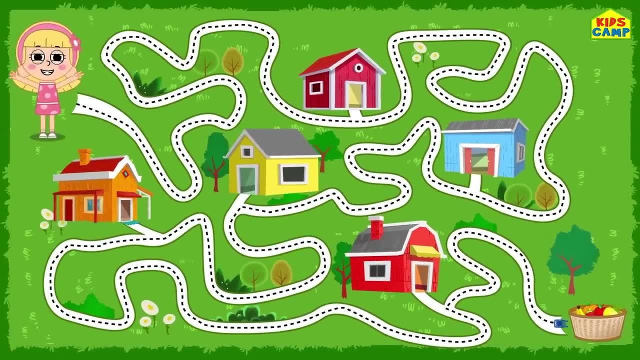 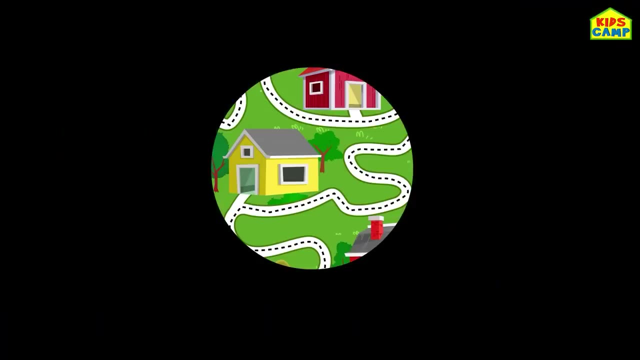 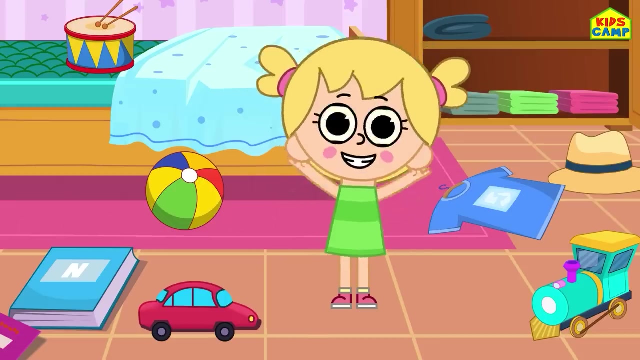 What did we get? A banana, a mango, an apple, a strawberry and an orange. Good job, Thank you so much for helping me find my fruits and collecting them in my basket. Thank you, Hi friends, I'm Ellie and this is Eva. 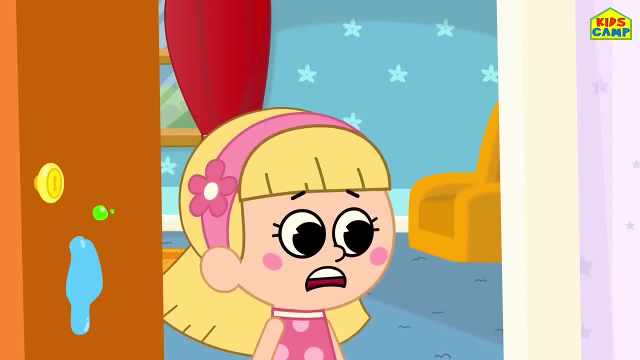 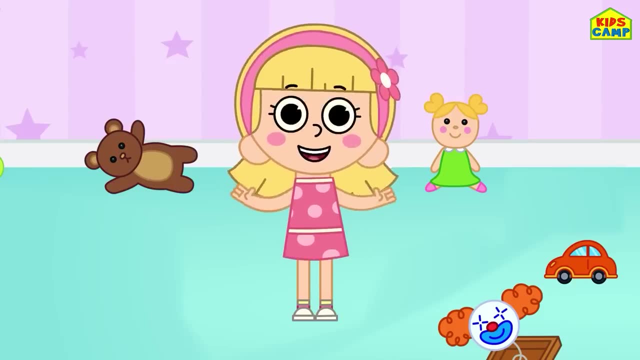 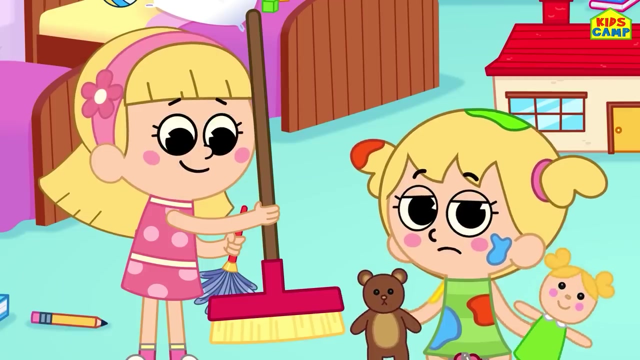 Eva, Look at your room. You have to clean the room now. I know a fun way to clean our room: Let's find the objects and put them where they belong. Eva, Let's clean our room. Let's do this, friends Ready. 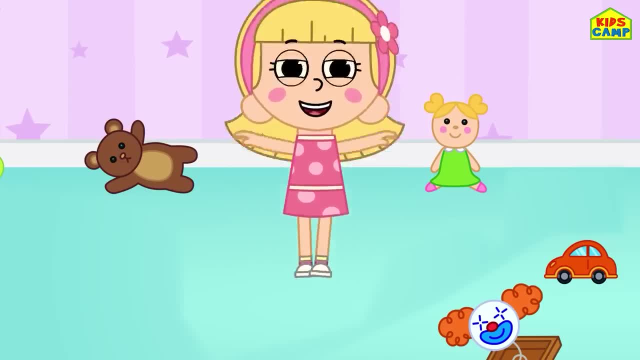 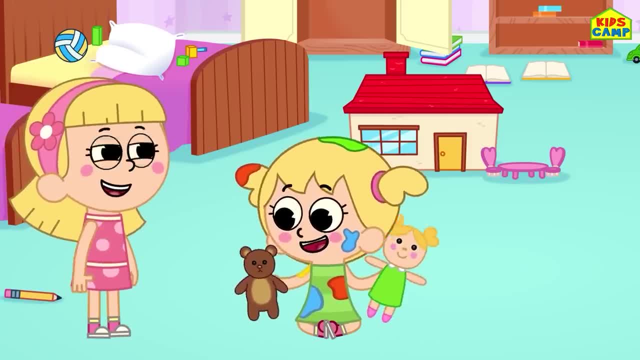 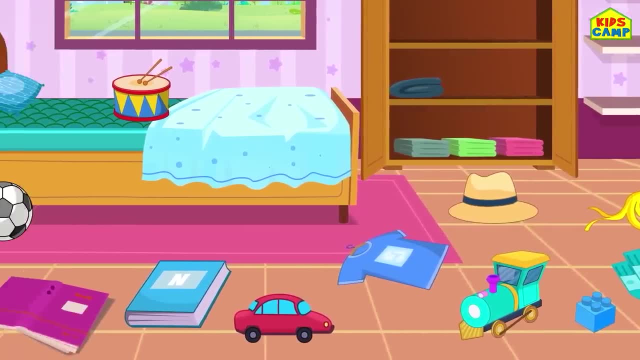 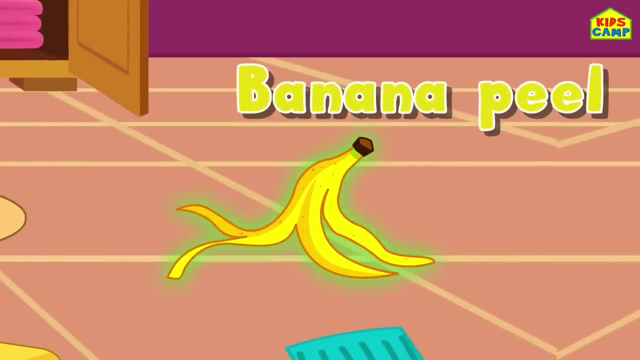 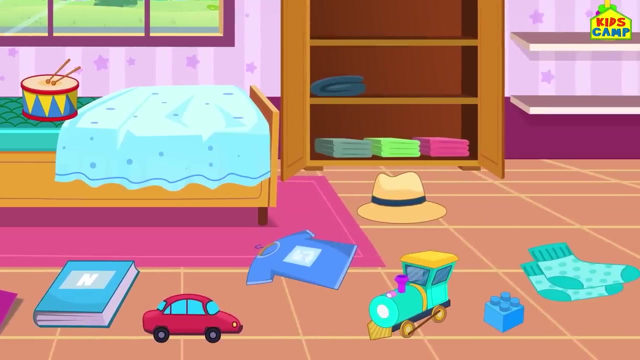 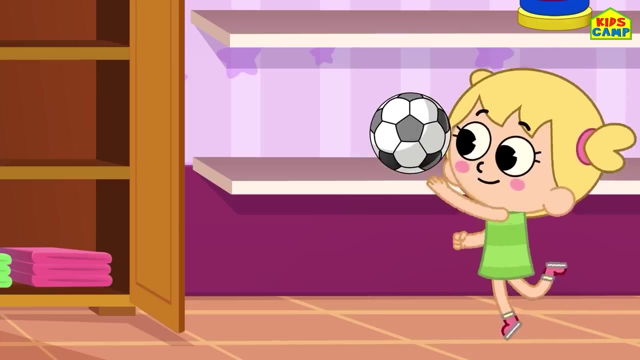 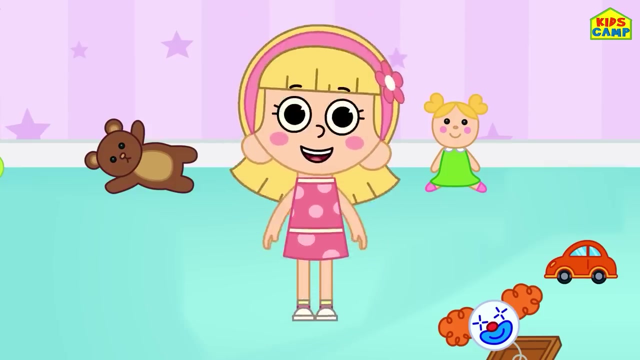 Come on, You can do this, Eva. you know what you have to do. that's right. let's first pick up the banana peel into the dustbin- good job. now let's pick up the soccer ball and keep it on our shelves. good job, Eva. very good, let's clean some more. 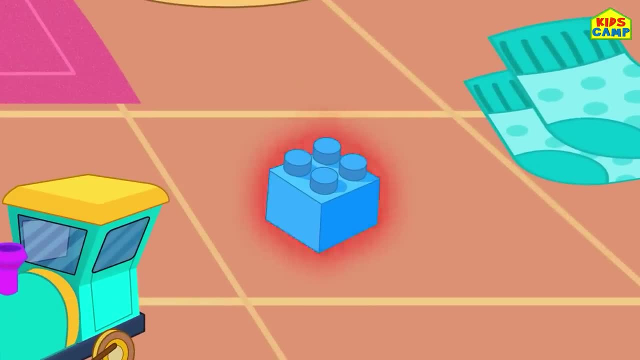 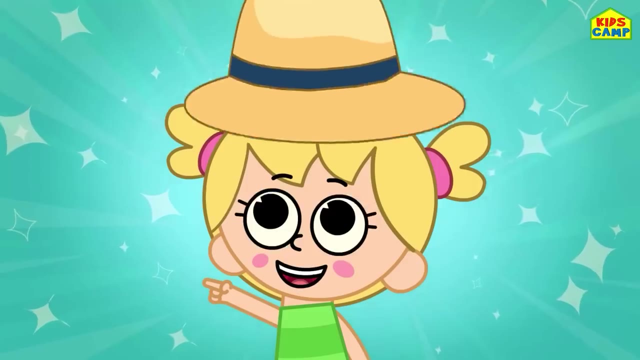 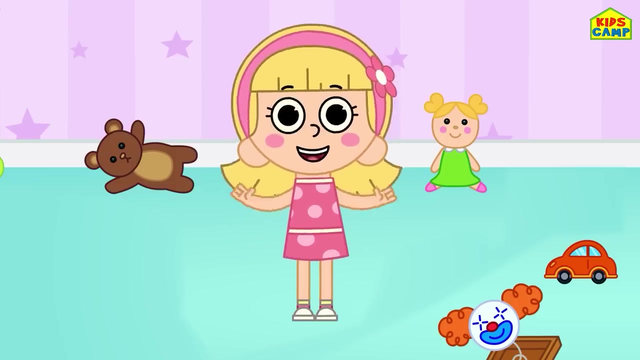 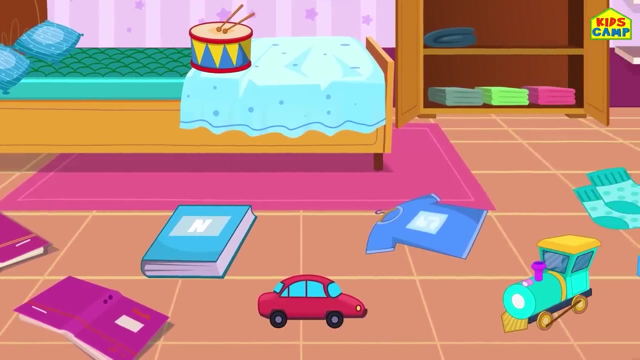 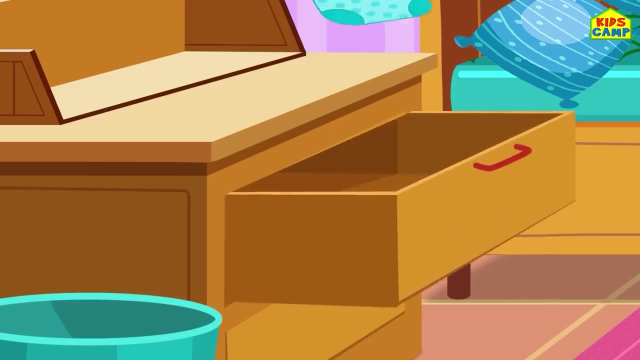 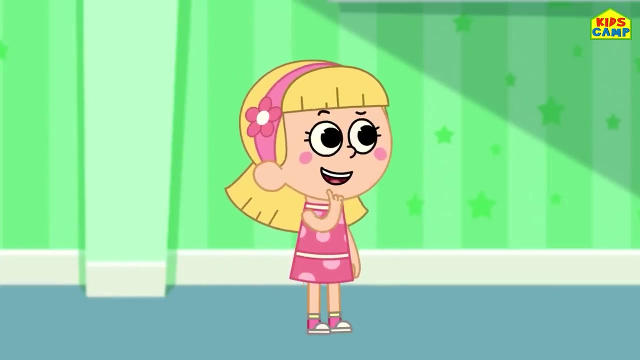 let's look for the hat. where is it? no, that's not a hat. no, that's a hat that's right on to the shelves. good job, let's clean some more now. let's look for the socks. that's right into the drawer. wonderful, very good, Eva. where are your books? look for them, that's right. 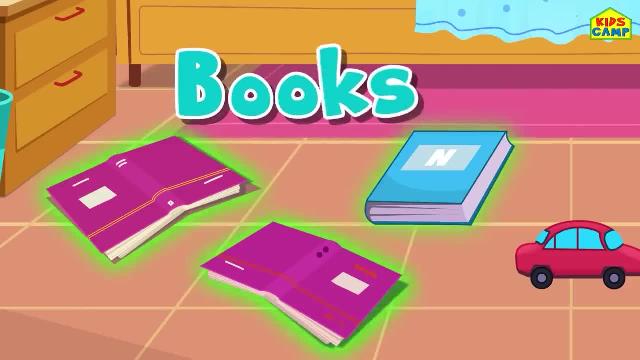 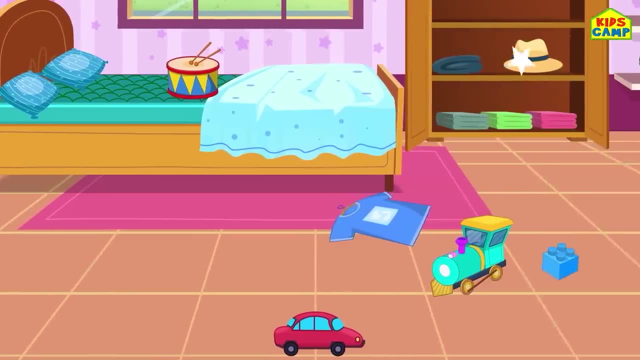 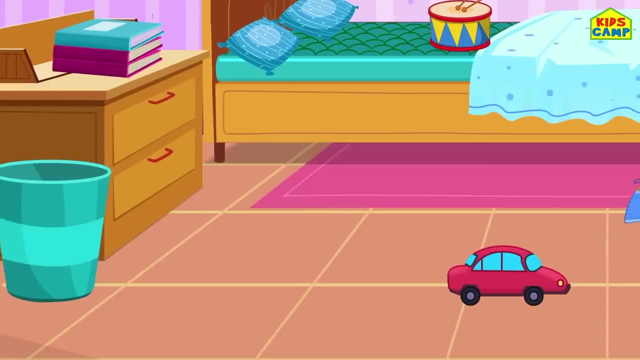 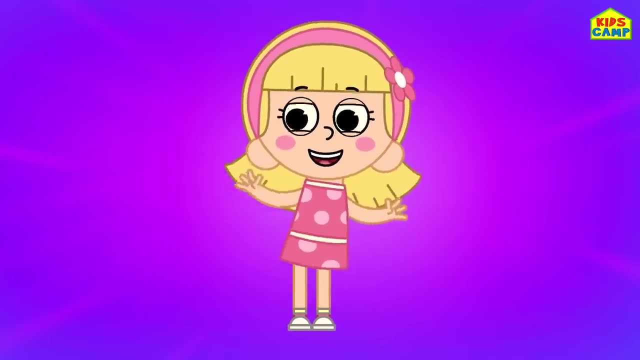 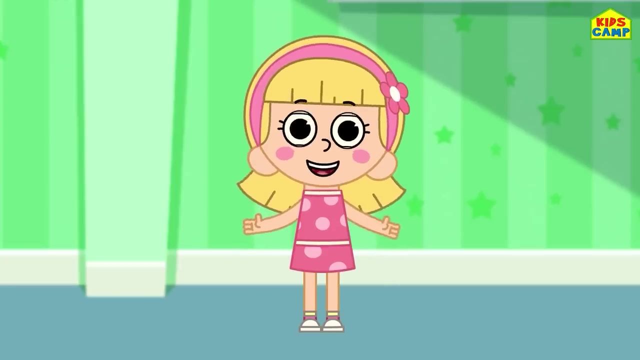 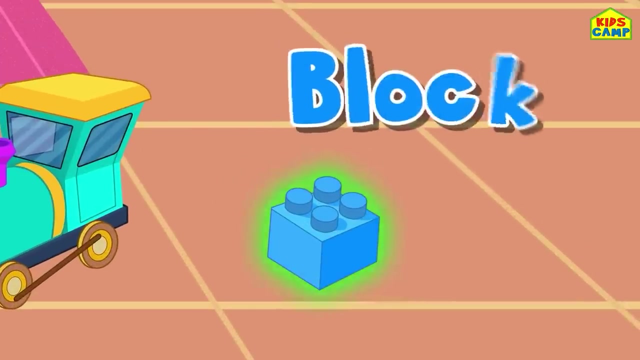 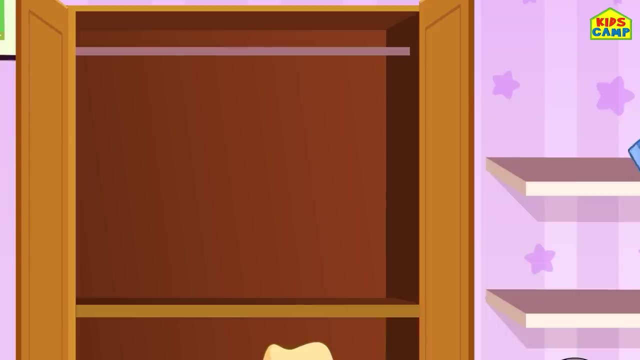 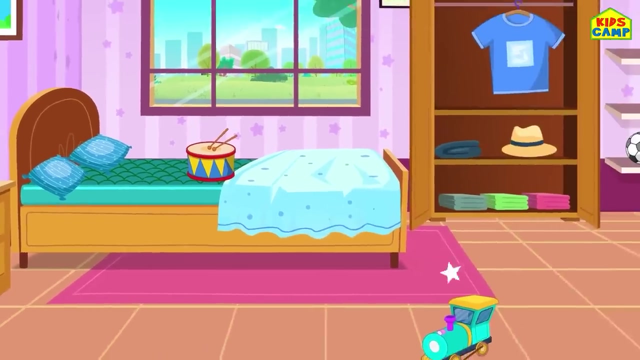 here are the books. let's pick them up. very good, stack them together. the room already looks clean, wonderful. now let's look for the toy car- that's right, amazing. onto the shelf. good job, Eva. let's clean some more. the block and the t-shirt, Eva. let's pick them up into the cupboard and on the shelf. good girl, wonderful. 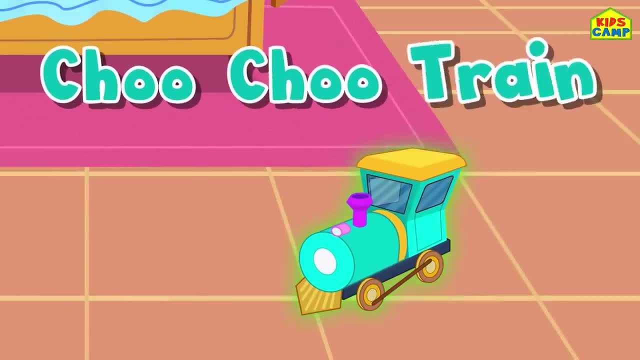 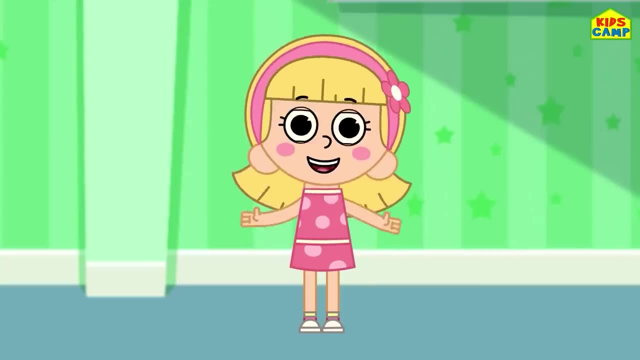 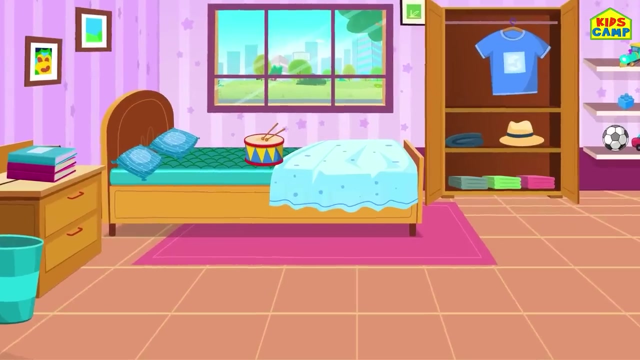 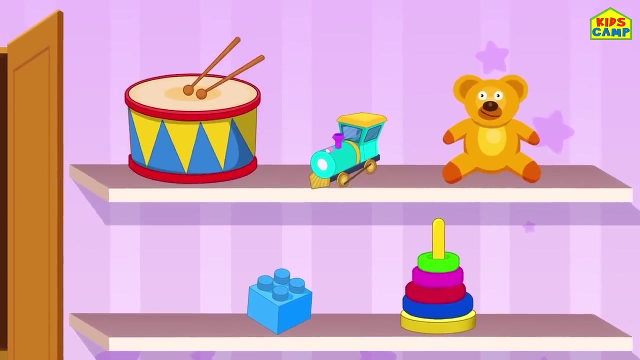 let's clean some more. the juju drain onto the shelf. we did it, we're almost there. good job, friends. wonderful the toy drum. let's pick it up and put it on the shelf. that's right, our room looks clean. yay, good job, Eva. let's pick it up and put it on the shelf. that's right, our room looks clean. yay, good job, Eva. yay, good job Eva. 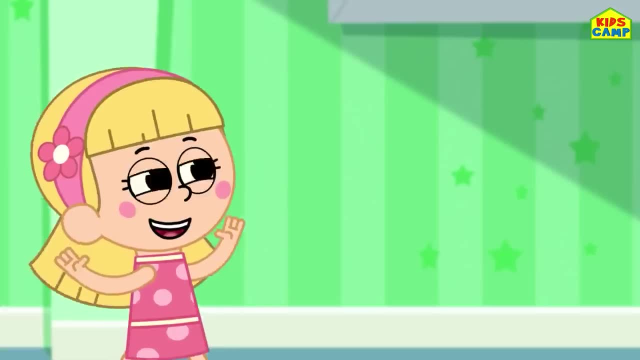 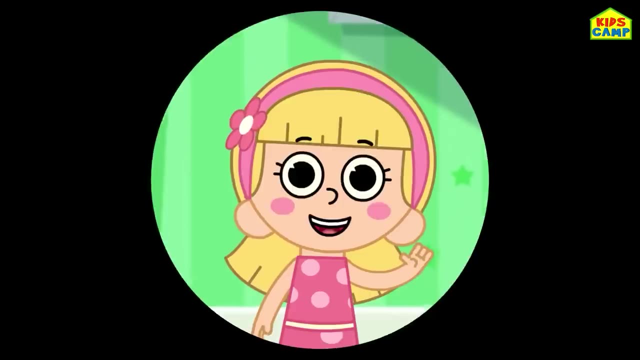 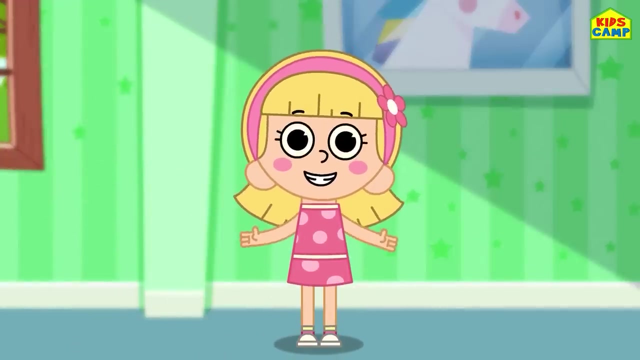 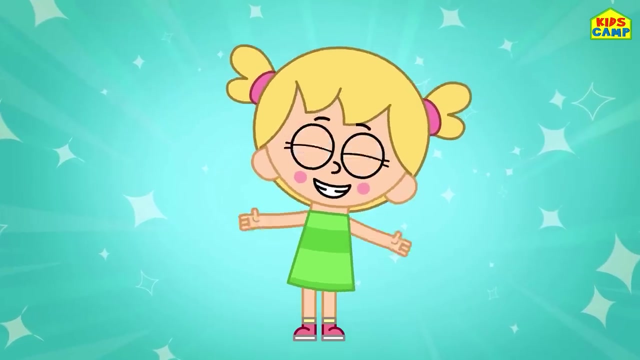 the back studied way. good job, Eva. wonderful, that's how you clean your room. wasn't that fun kids? hi friends, i'm ellie, but i can't find my cat. i don't know where she's gone. can youhhelp melook for her? hi, Eva, where's our cat? 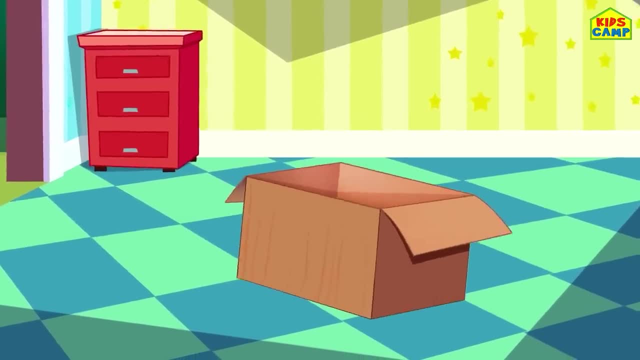 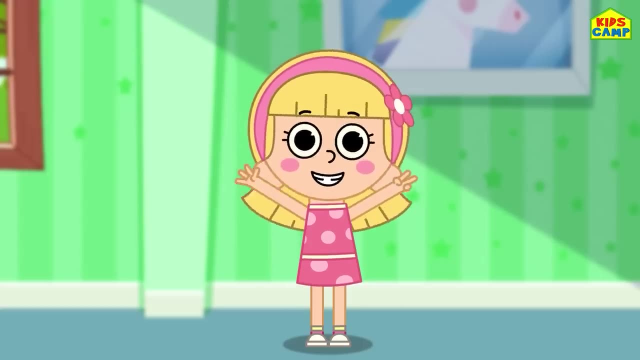 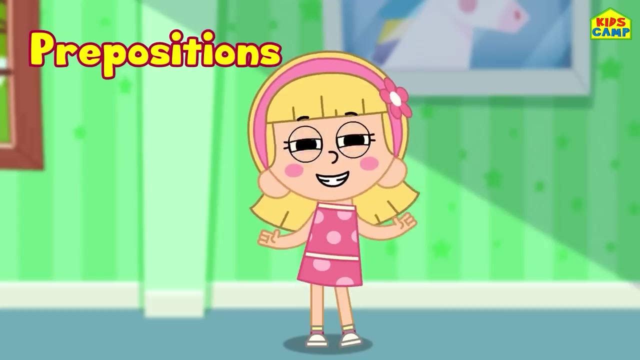 don't-how. That's right, She's in the box. HmmEva seems to be confused. Don't worry, Today we are going to learn prepositions and how and where to use them. Ready, Let's start. The first preposition is IN. 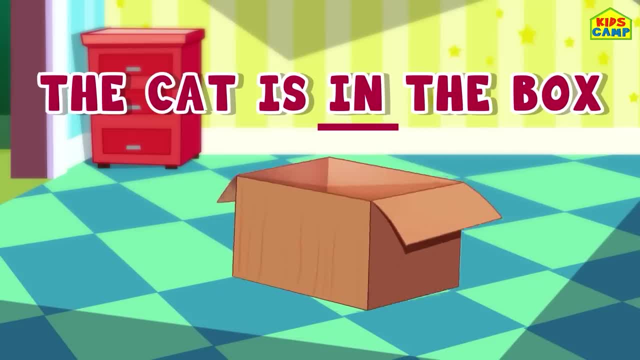 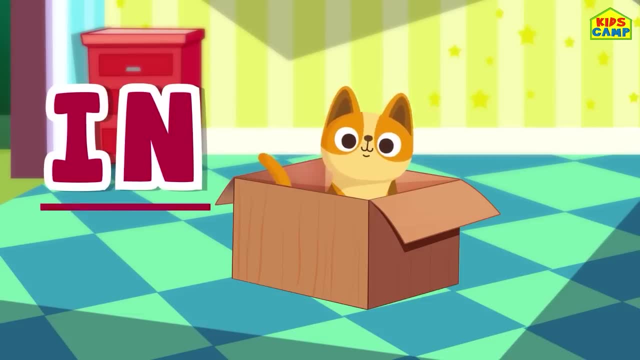 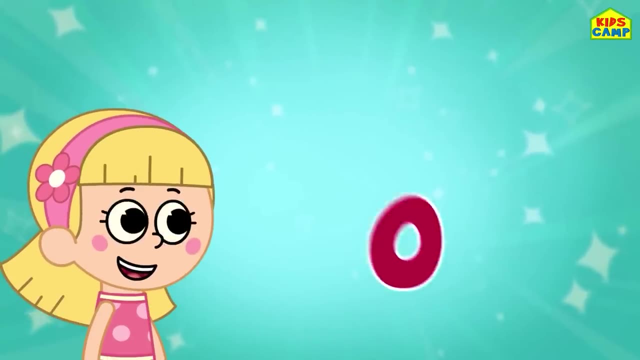 The cat is in the box. Do you see that, Eva? She's in it. IN is the preposition and this is how we use it To show the position. The next one is ON. That's right, The cat is on the box. 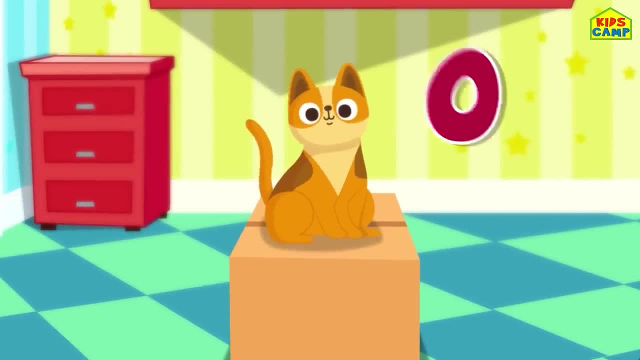 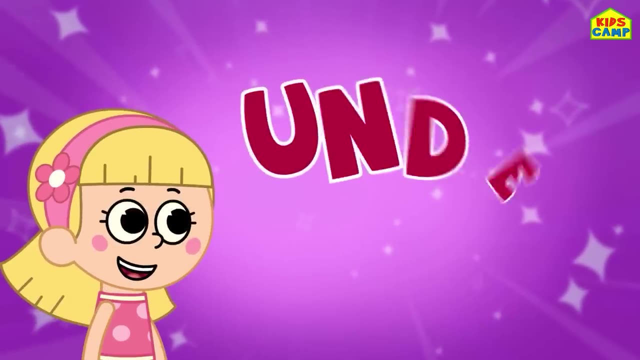 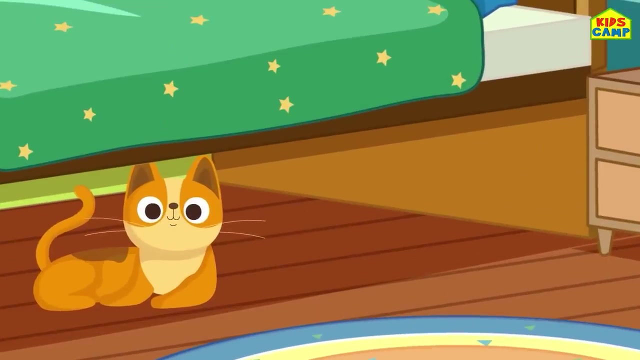 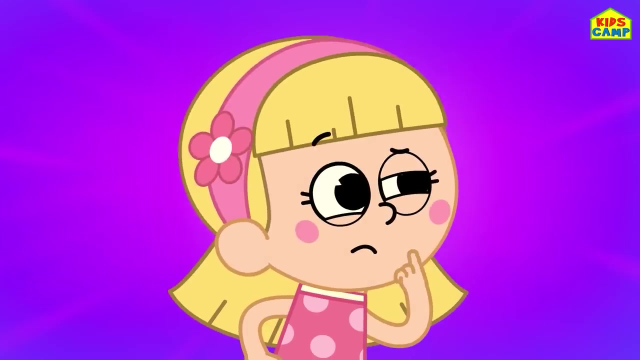 Yay, This is easy, isn't it? This is how we use the preposition ON. Next is UNDER or BENEATH. The cat is UNDER the bed. There she is. We found her. Good job, friends. Where is the cat now? 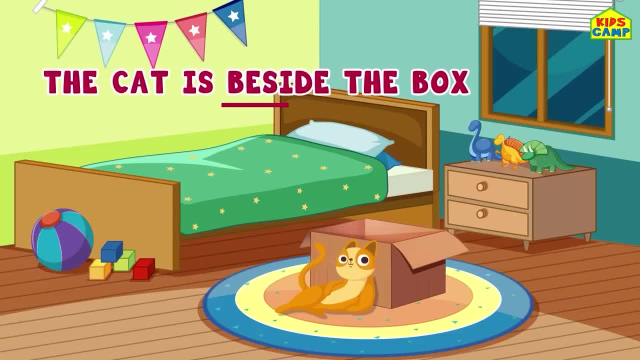 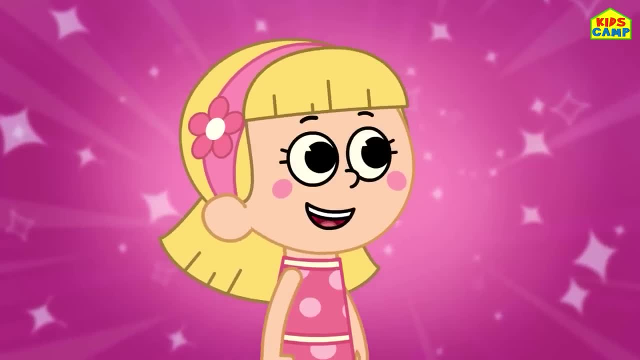 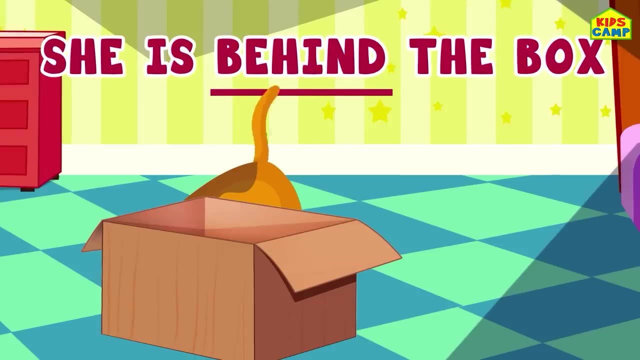 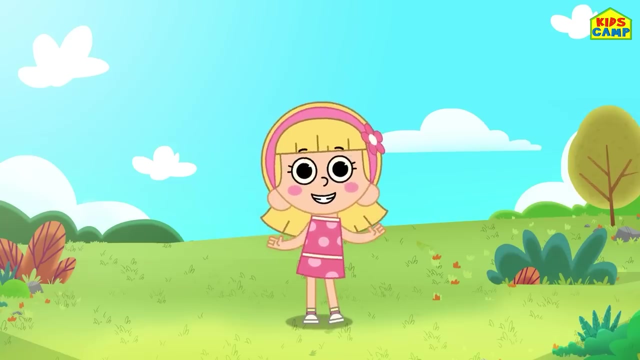 The cat is BESIDES the box. She's beside it, Right. Where is the cat now? She is BEHIND the box. There she is. Yay, Come back for more games and keep watching Kids Cam. Until then, bye, bye. 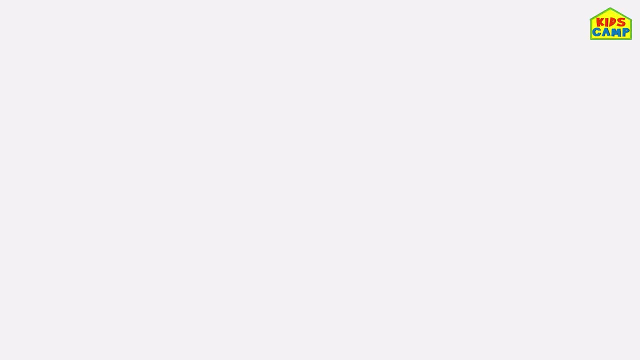 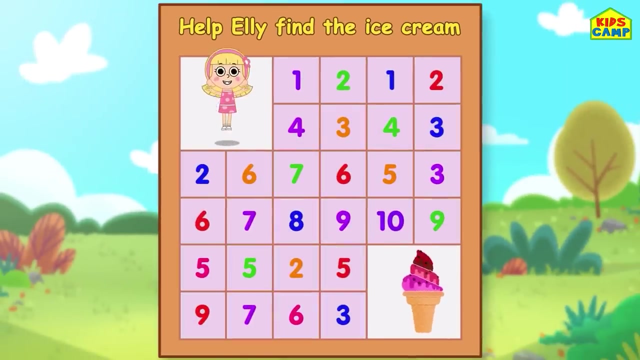 Bye, Hi friends. I am Ellie. Would you like to help me reach the ice cream? Yes, Then let's get started with this amazing number maze. Yay, Let's get started. Let's start with the number 1.. Let's start with the number 1.. 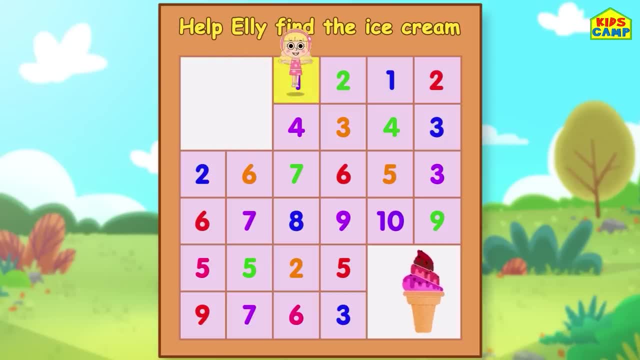 Yes, I am on number 1.. Let's go to the next number 2.. Yay, Oh, That's not right. Aha, That's right, That's 3.. Let's go to the next one. Let's go to the next one. 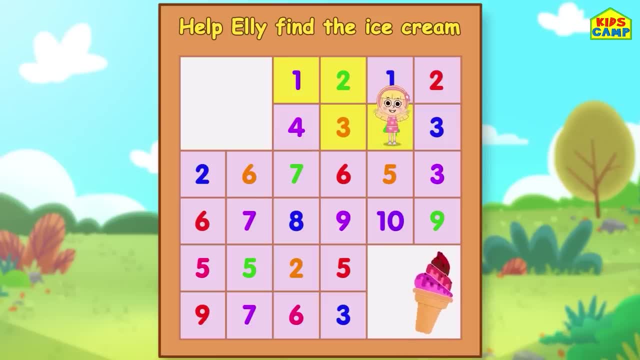 Number 4.. Yay, Aha, Number 5.. Good job friends. Good job friends. Oops, That's not right. The next number is 6.. That's right, Wonderful. Next, 7. We are almost there. 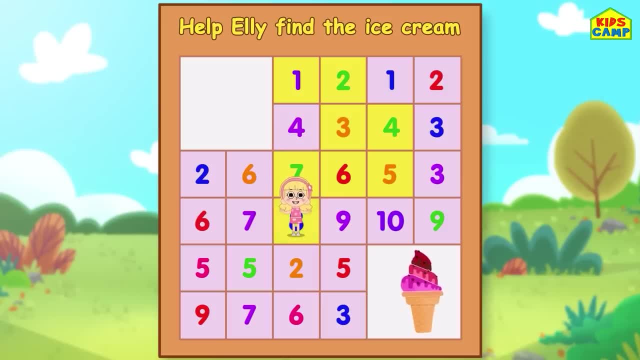 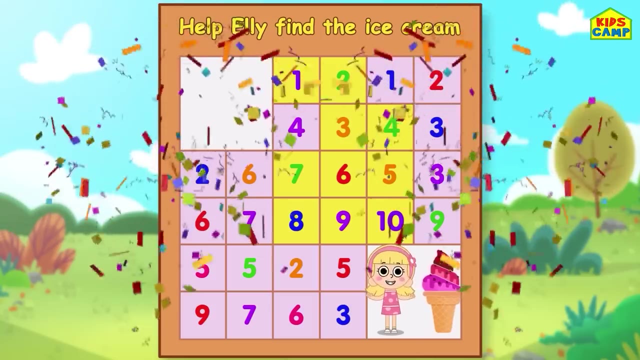 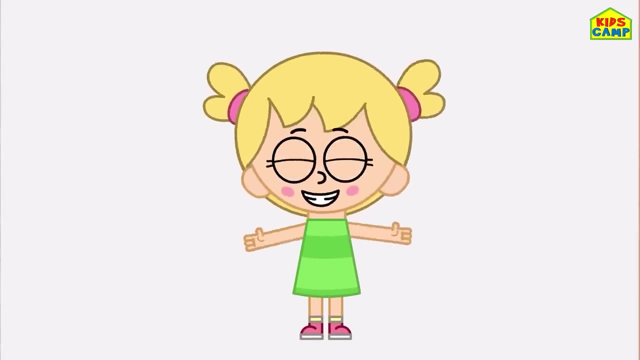 And 8.. Yay, Uh-oh, No, That's right. 9! And 10!. Yay, We did it. You helped me reach the ice cream. Thank you, Oh, It's Eva's turn now. 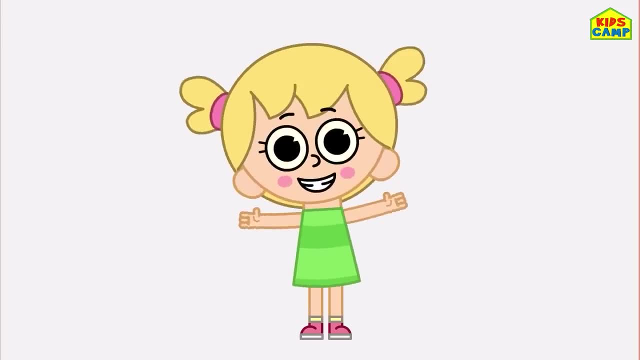 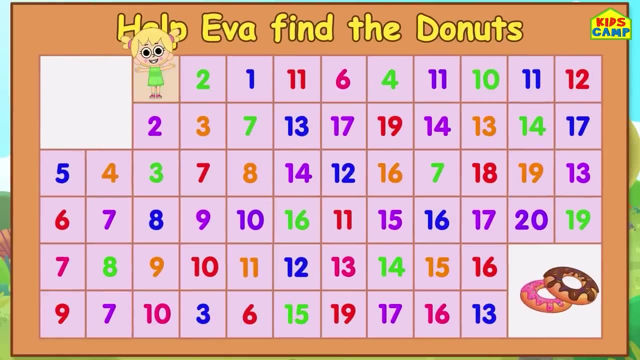 Can you help her reach the donuts? Let's get started. Yay, Let's start with number 1.. 1., 2., 3. Good, 4.. Uh-oh, No, no, no, That's right. 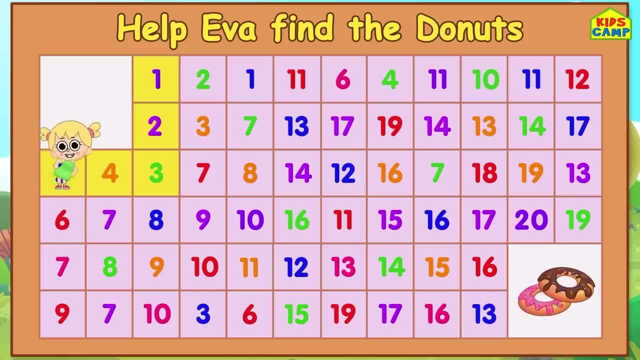 Number 5. Good, 6. Keep going. 7.. 8. Yay, Oops, That's not right, That's right. 9. And 10! 11. Keep going. Yay, We are on 12.. 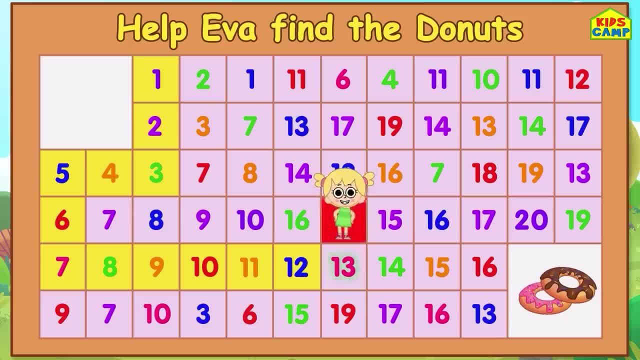 What comes after 12?? Uh-oh, No, not that one, That's right. 13! And 14!. Next is 15!. Woohoo, Only 5 more to go. 16!, That's right. 17!. 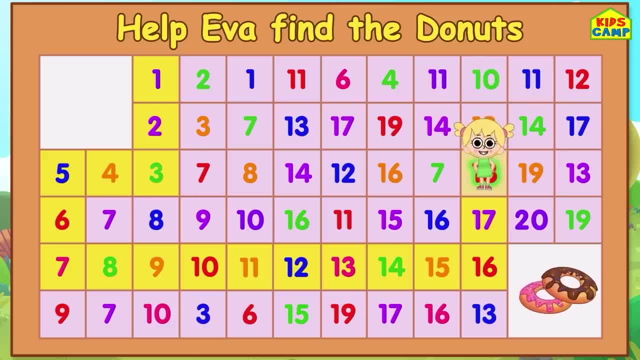 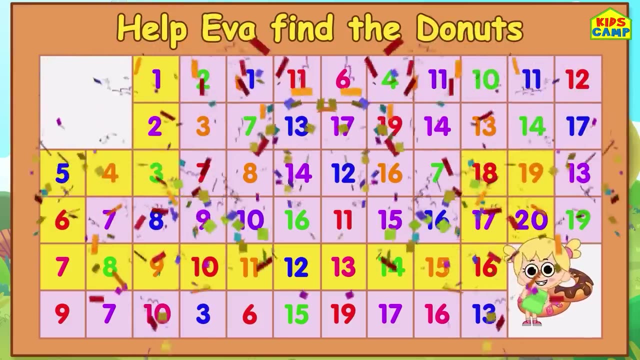 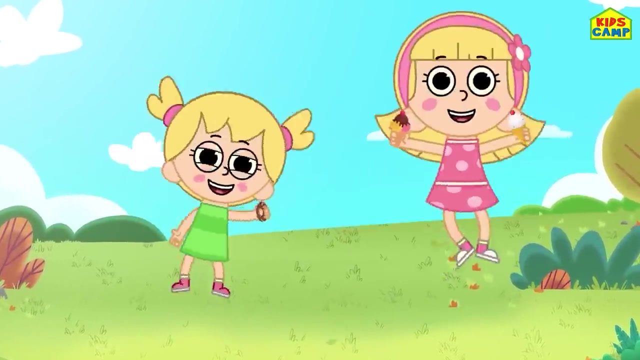 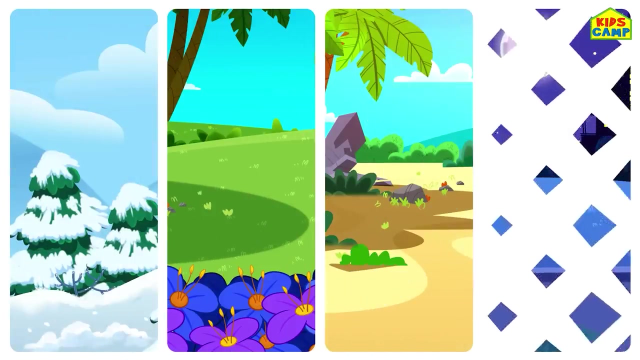 Next is 18!- That's right. 19!- We're almost there. And 20!- That's right, We did it. Woohoo, We helped Eva find the donuts. Good job, friends. Bye Seasons with Elli. 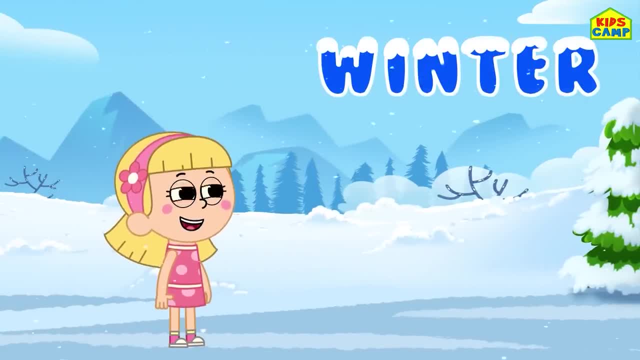 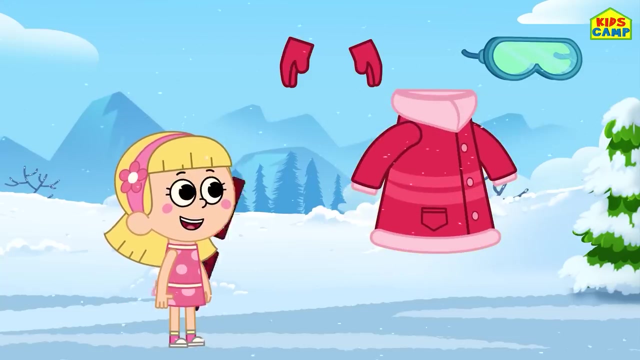 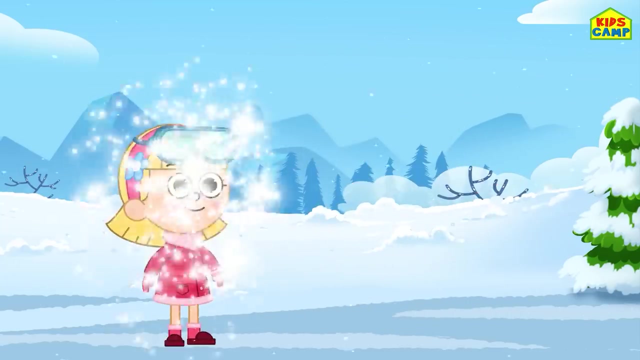 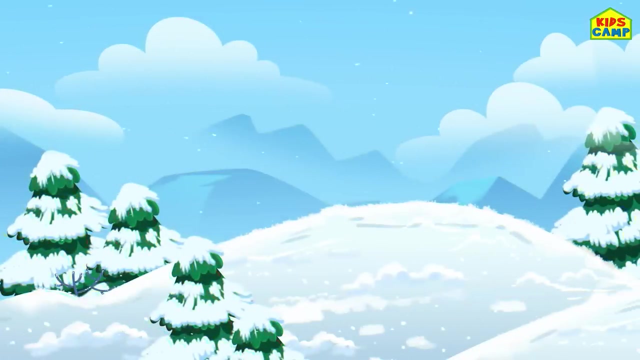 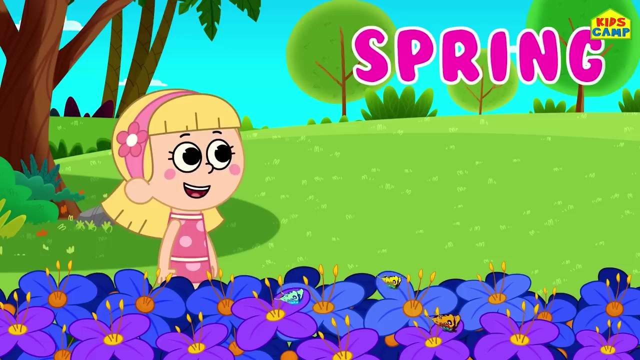 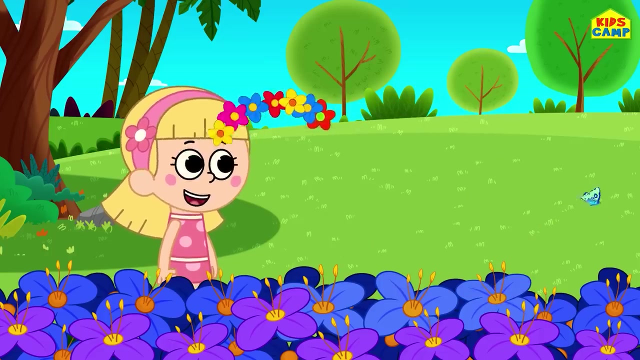 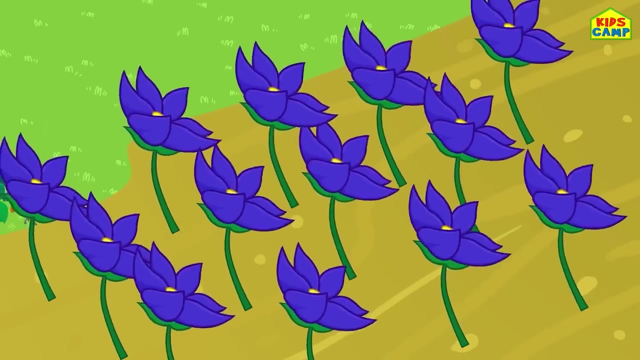 What season is this? Winter Gloves, Snow goggles, Coat, Boots, Yay, Wee, Woohoo. What season is this? It's spring. Flower headband. Wow, Look at the flowers bloom And the birds sing. 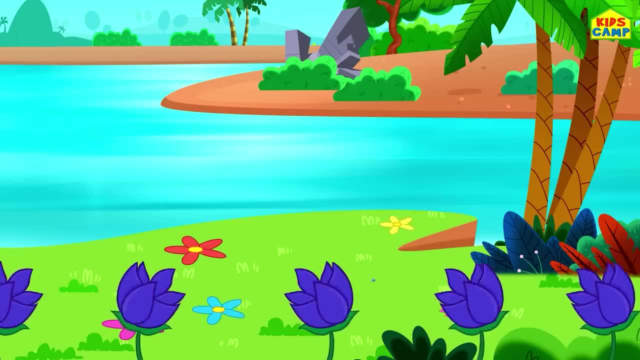 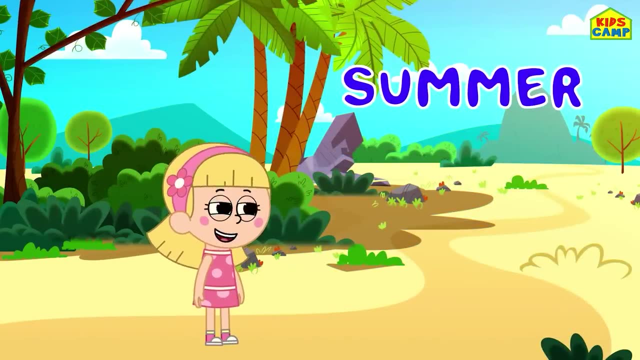 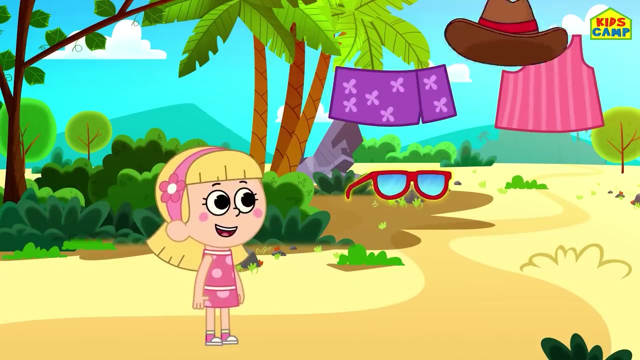 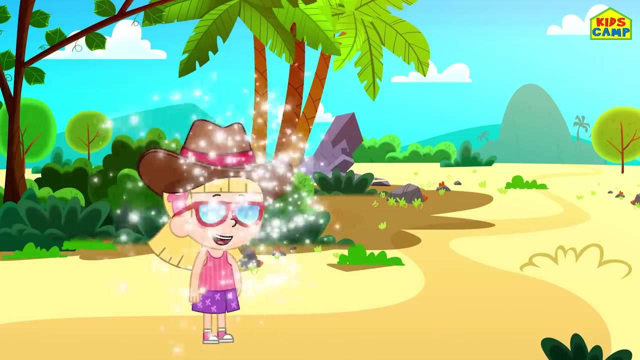 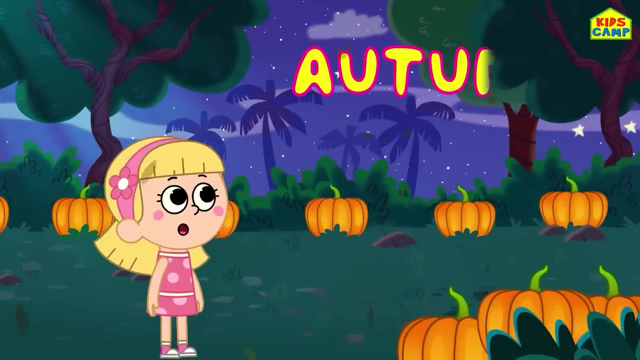 The bunnies have come out to play And the sun is shining bright. What season is this? It's summer. Swimsuit, Sarong, Sunglasses, Hat. Yay, We're ready to go to the beach. Oooh, It's nearly Halloween. 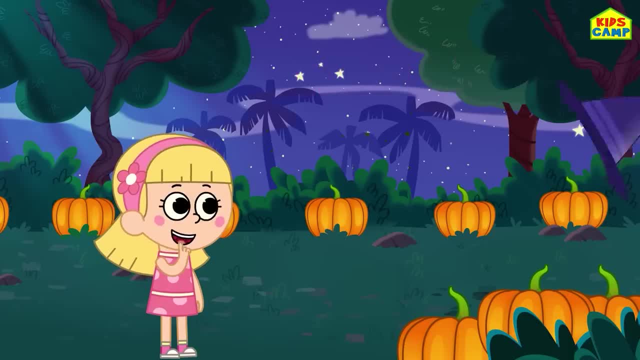 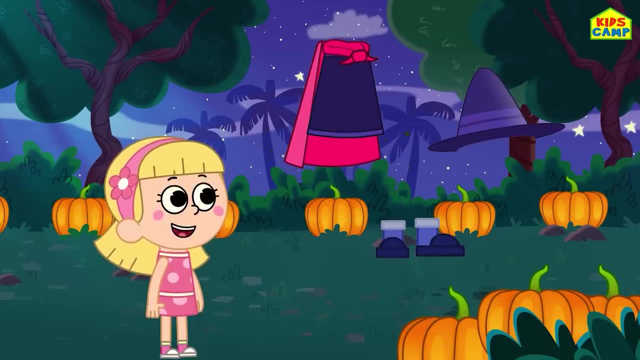 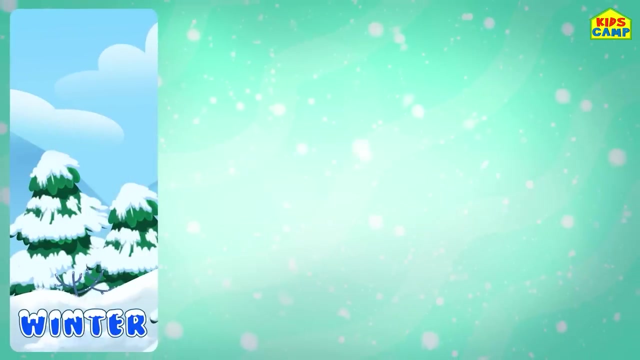 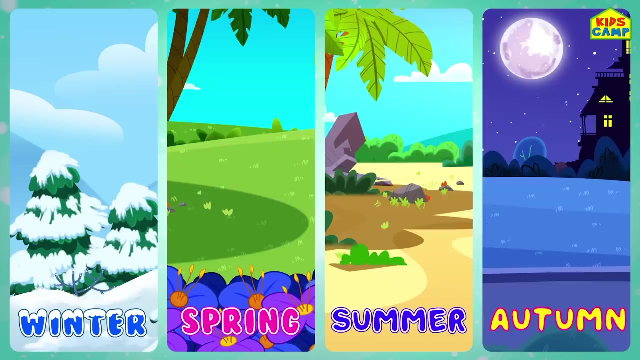 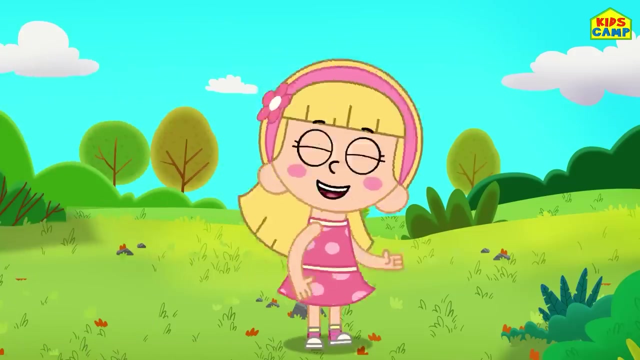 That means it's autumn. A witch's hat, A dress with a cloak And witch's shoes- Yay, I'm a witch. Today we learned our seasons: Winter, Spring, Summer And Autumn. Woohoo, Hi friends, I'm Elli. 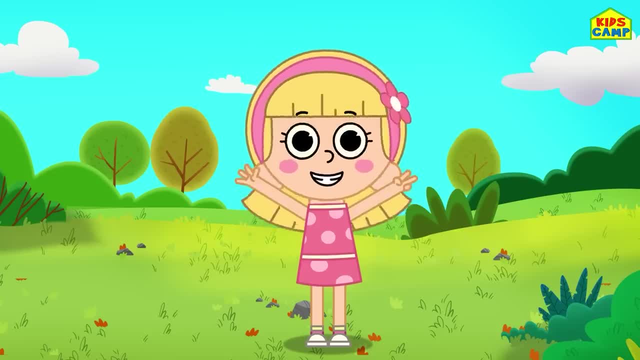 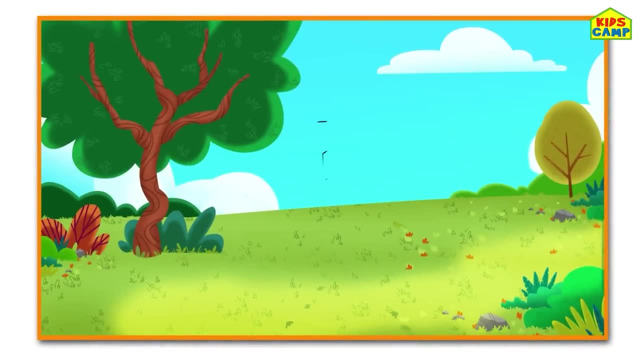 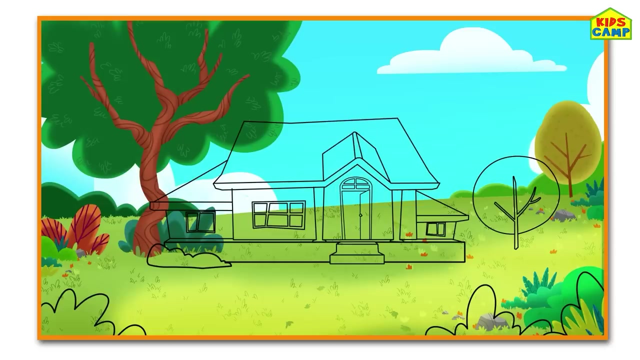 And today we're going to build a house. Excited So am I. Let's go. Oooh, That's the outline. Let's fit the different parts of the house right there. Let's figure out what goes where. First, the foundation. 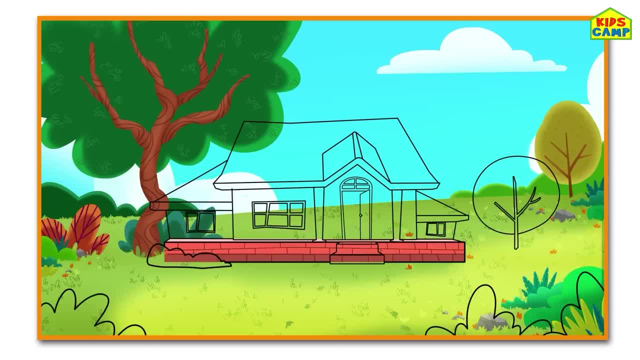 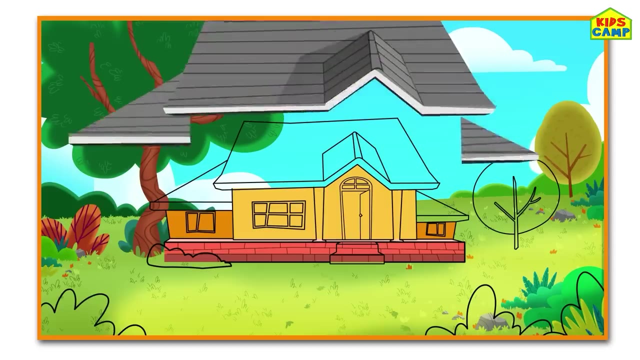 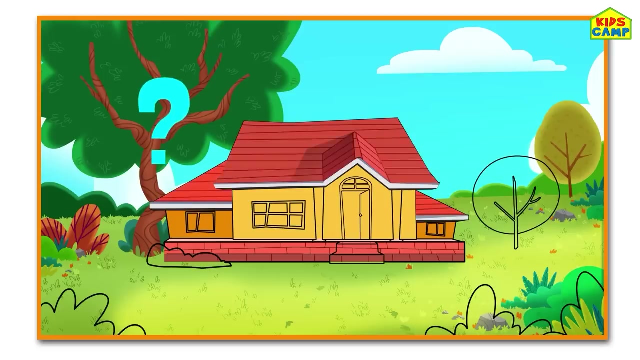 The base. Wow, That was easy. Now let's add the walls. I love yellow paint on my walls. This looks great. Next, let's add the roof. Perfect, It's starting to look like a house. What's missing, That's right, A door. 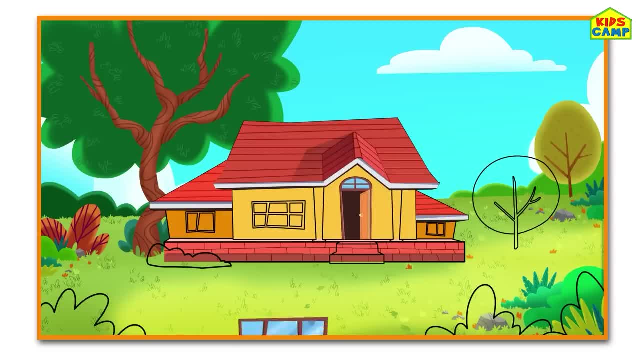 Yes, And lovely windows to look outside And for sunshine to come in. Next we need steps: Perfect, And now let's add the pillars. Going good, This is such a beautiful house, But what else is missing? Let's add color to my garden. 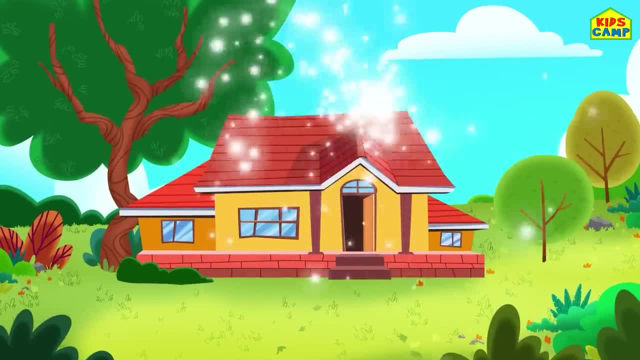 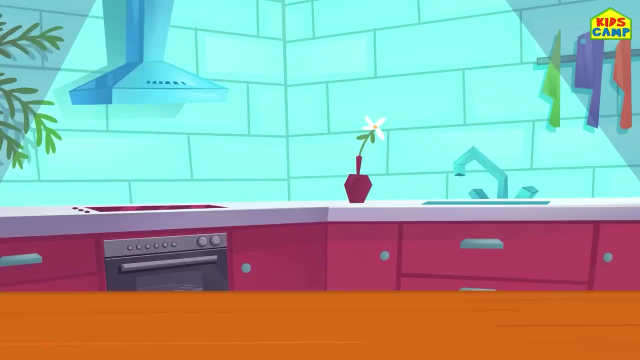 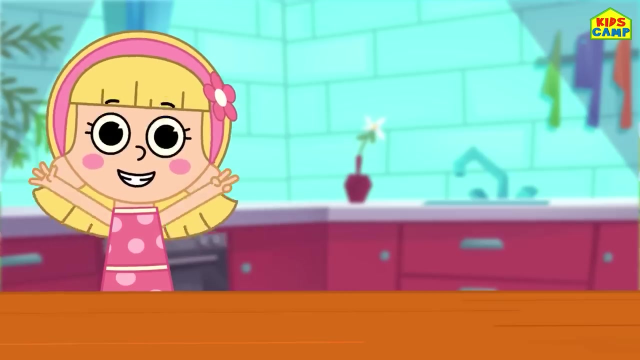 Wow, It looks beautiful. That's my house. Okay, friends, I'm going home. See you, Bye, Hi friends. I'm Elli And I love jelly beans, Don't you too? That's right, And this is Eva. 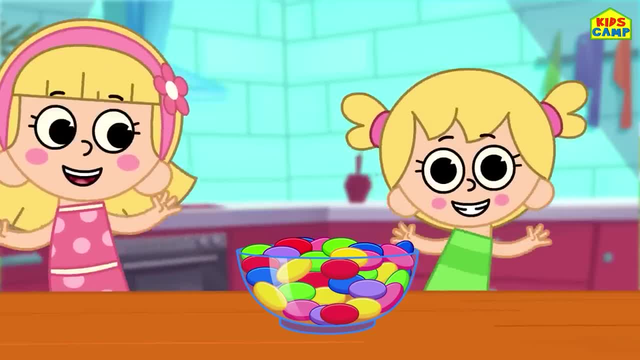 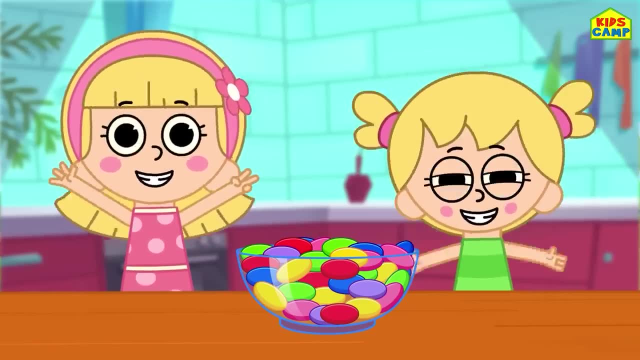 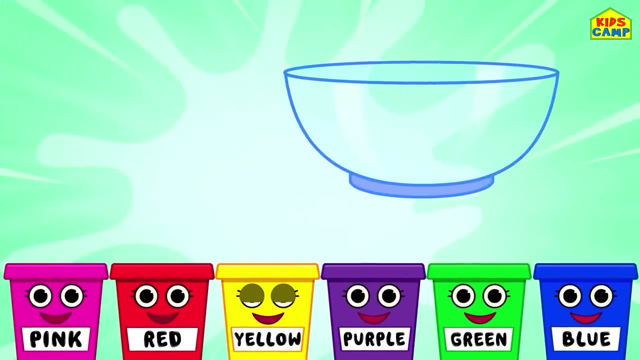 We have to sort the jelly beans by their color. That's easy. Yay, Will you help us? Let's get started. Yay, Yay, Yay, Ooh Jelly beans. Let's sort the pink jelly beans. 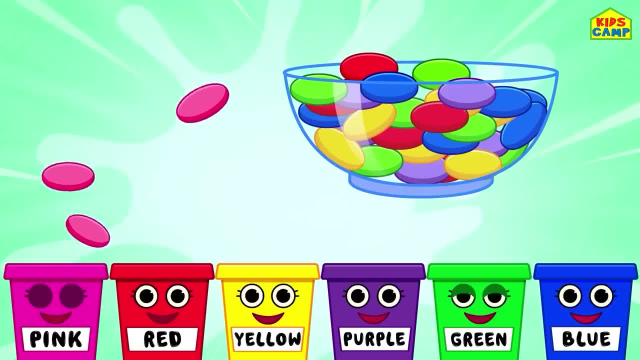 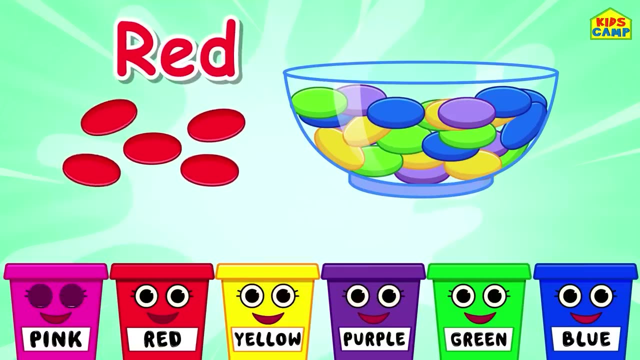 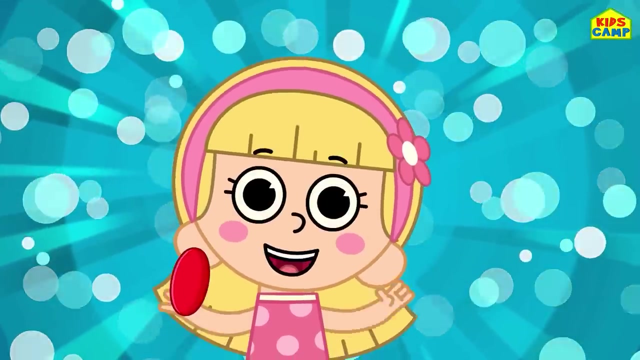 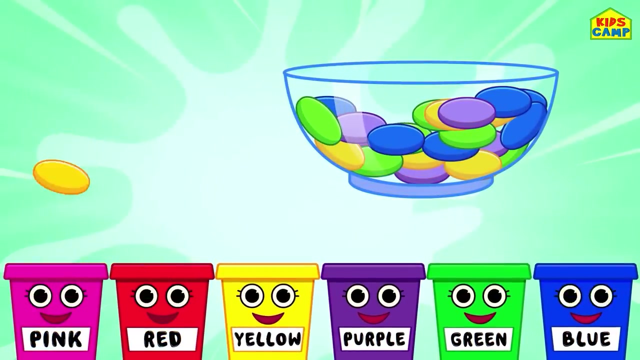 Yummy, Into the pink bucket, Wonderful, Yay. Next up is red. Let's sort the red jelly beans. Woohoo Into the bucket, Yummy. Next up is the color yellow. Yummy, Let's sort all the yellow jelly beans. 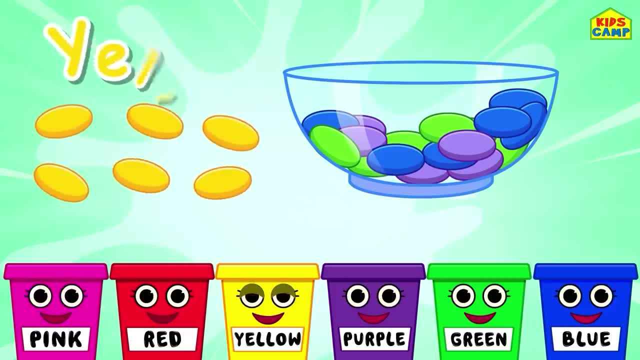 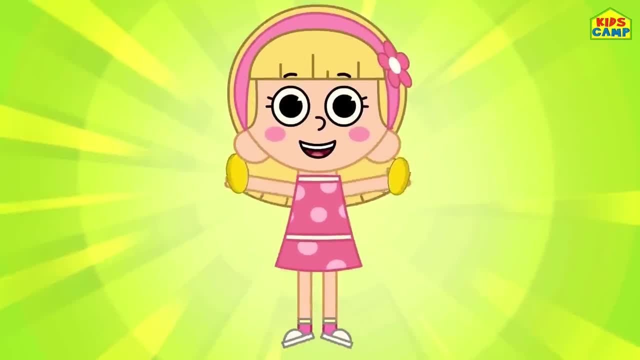 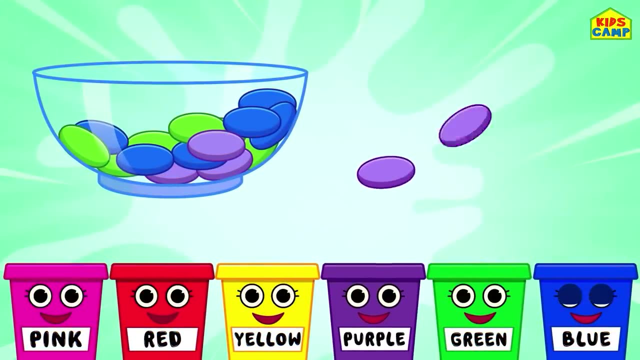 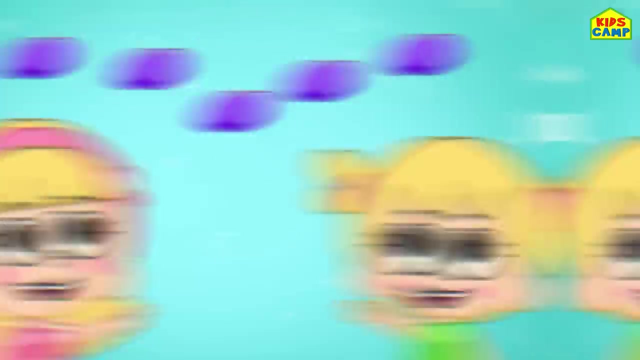 That's right Into the bucket. Wonderful, I love yellow. Next is purple. Look for all the purple jelly beans. Yes, That's right Into the bucket. Great job, friends. Wonderful. We all love jelly beans, don't we? 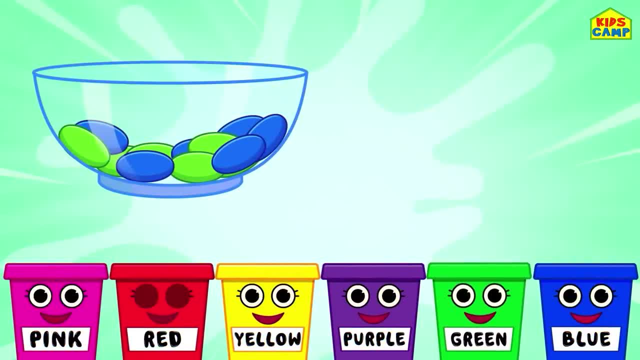 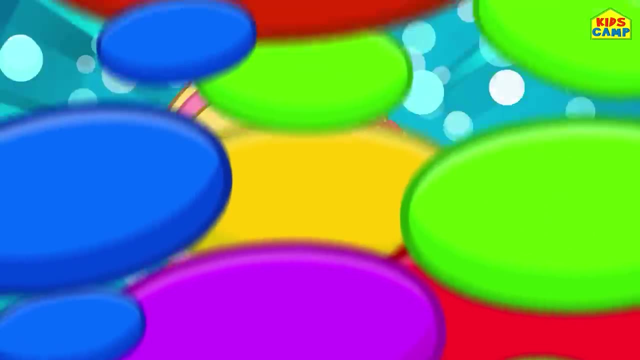 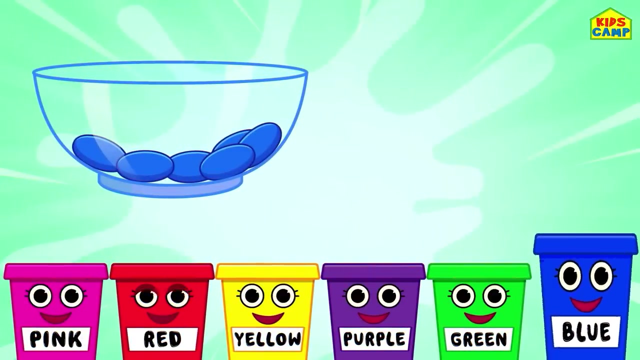 Next is green. Let's sort all the green jelly beans Yummy Into the bucket. Wonderful Yummy. And the last one is blue. That's right, We have only the blue jelly beans remaining. That's right Into the blue bucket. 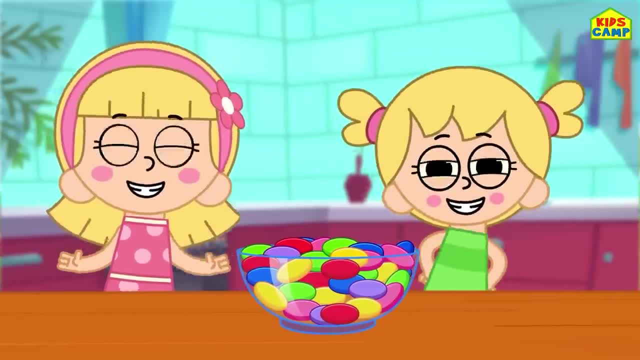 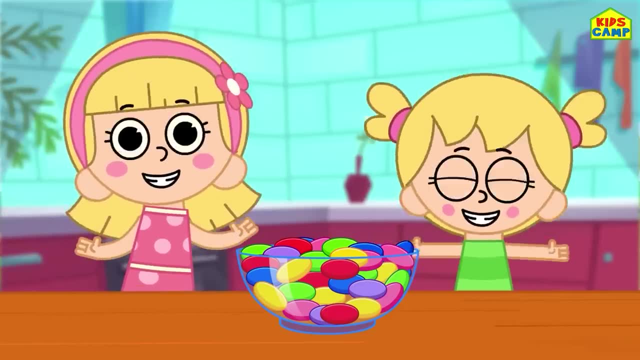 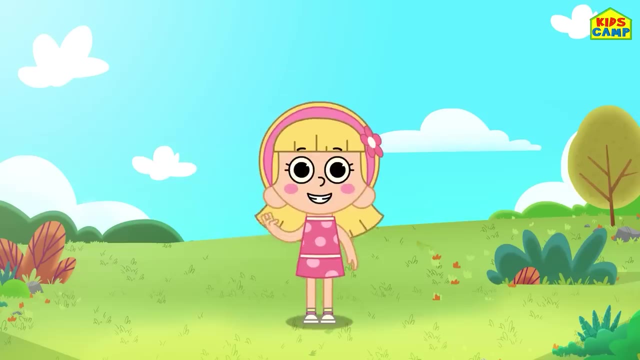 And we're done. Good job, friends. That was such a fun time sorting the jelly beans. Come back for more on Kids' GAM. See you soon. Bye-bye, Hi everyone, What a beautiful day. I'm Ellie And we are going to play a new game called Find the Matching Pear. 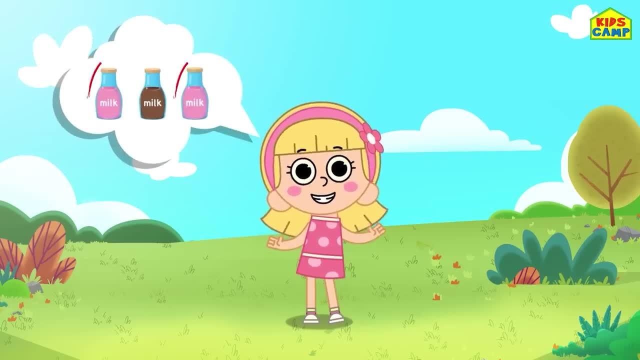 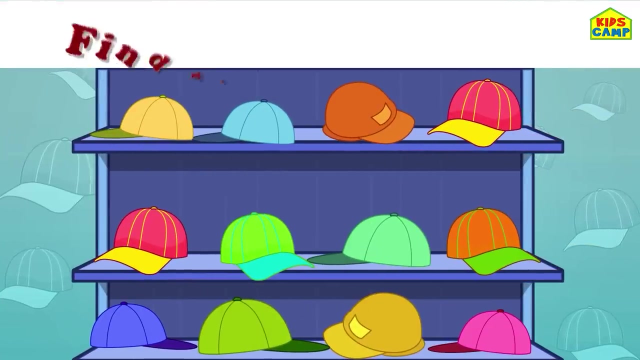 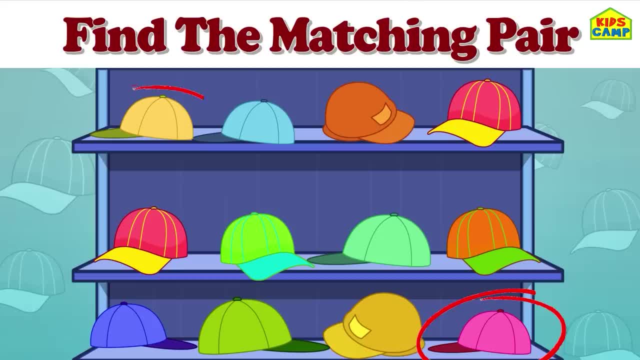 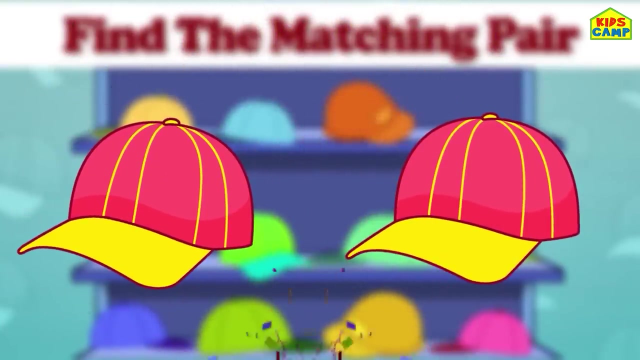 Can you spot two identical caps? No, They are not identical. No, Yes, Yay, We found them. They are two identical caps. Good job, Let's find another pair. Let's find another pair. Great, Find the matching rockets. 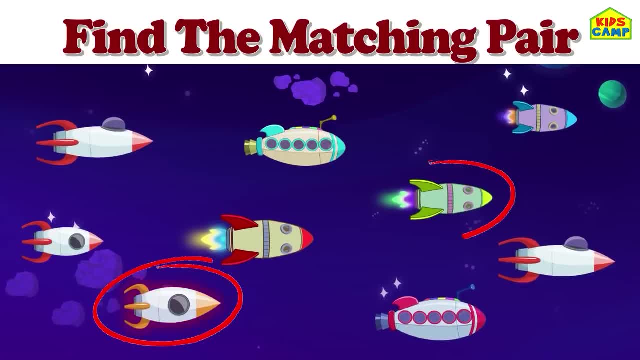 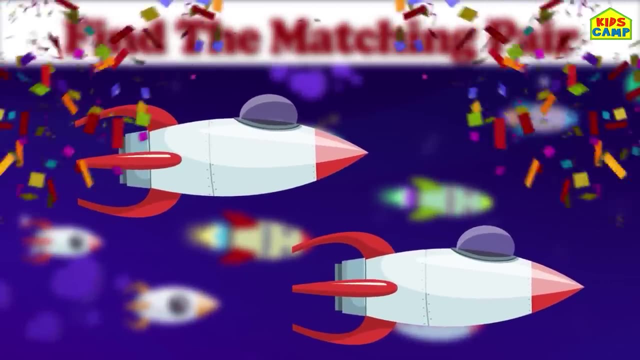 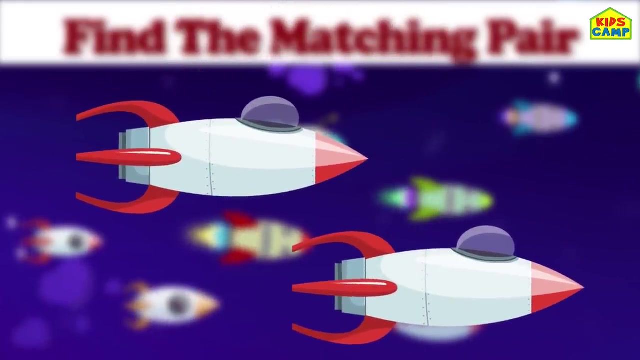 Can you? No, Not this one. No, Yes, That's right, They match. Perfect, We found them. This was easy. Let's go to the next one. Let's find the matching hats. Let's find the matching hats. 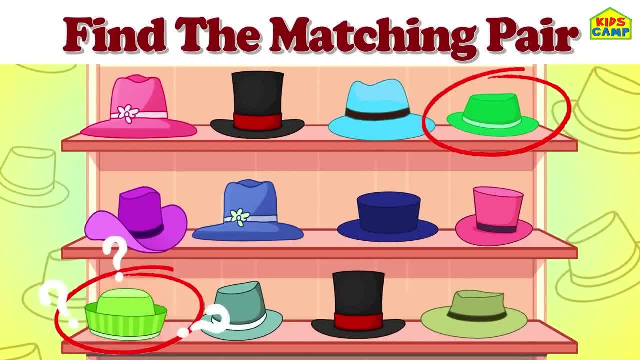 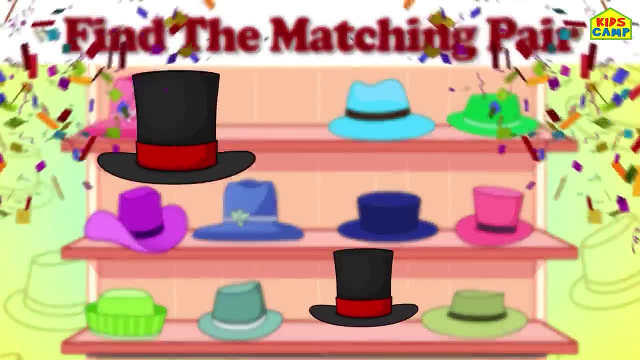 Find the matching hats. No, This ones are Reynolds. Nooo, We don't have this shape from school. Let's look for them in the landscape Now, we should have done this. Nooo, Yes, we found them Perfect. 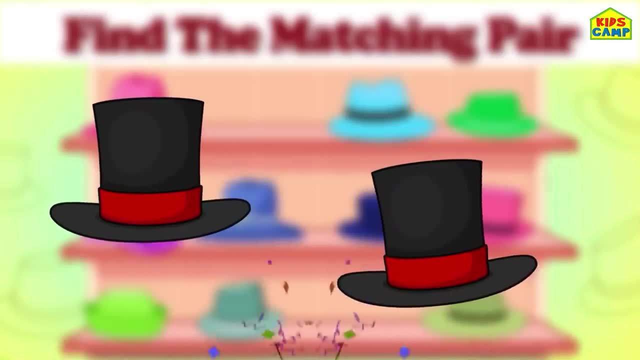 We have one pair, Perfect pair. Good job, friends. We have one pair of balloons. Two: tenemos dos almonds. Let's find the matching cheese. Can you find the matching cheese? We have one pair of balloons. Let's go to the next one. 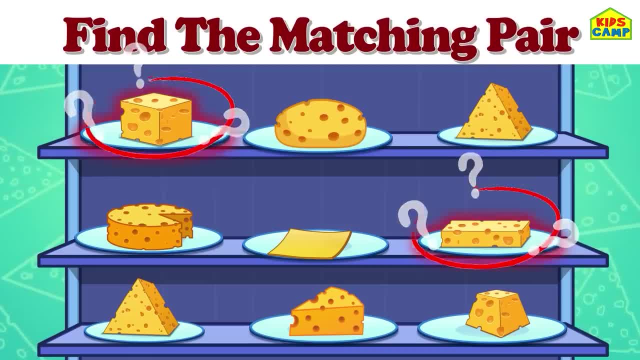 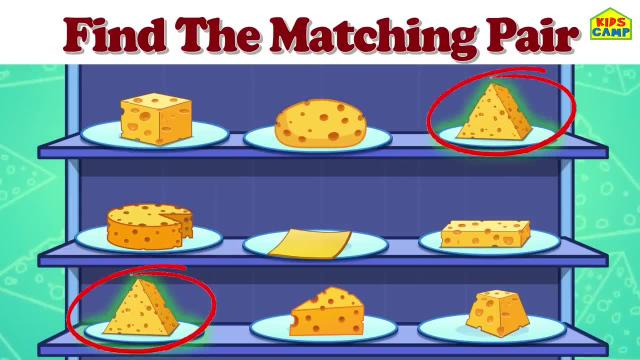 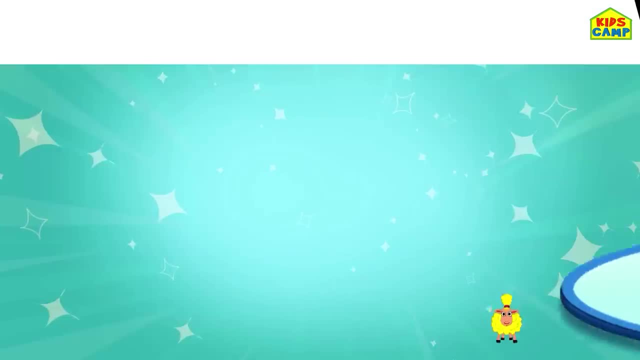 Can you find the matching cheese? Yes, That's right, These match. Perfect, Good job. Can you find the matching pair here? No, They are not identical. Yes, They match. No, No, No, No, No. 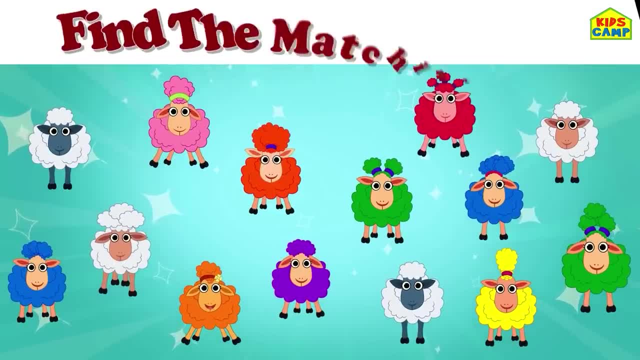 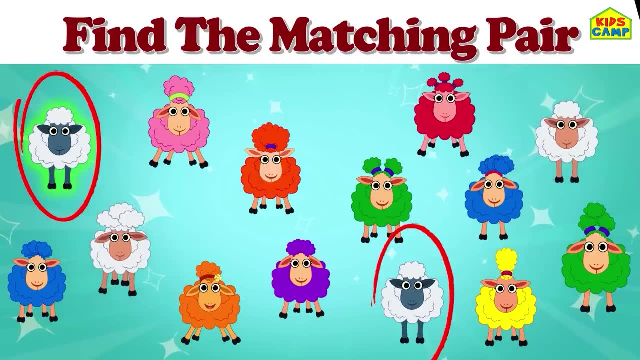 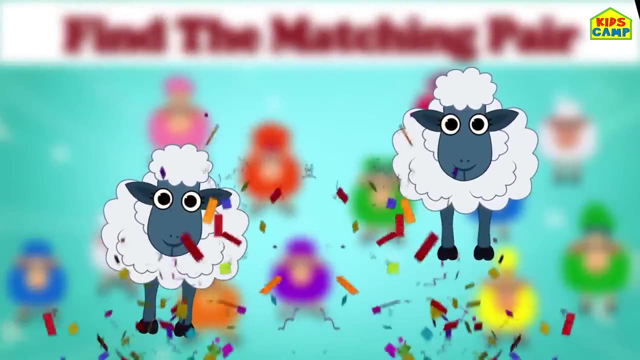 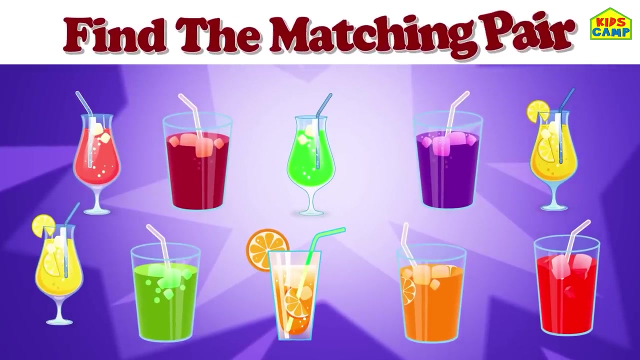 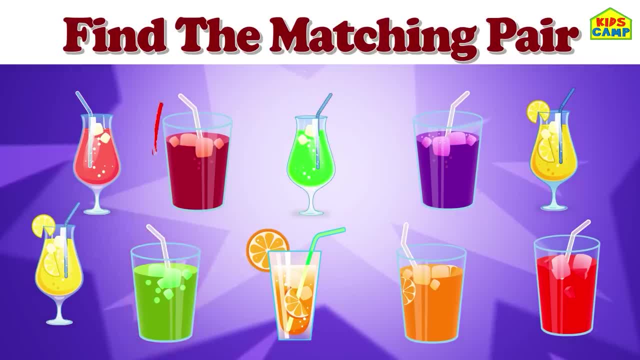 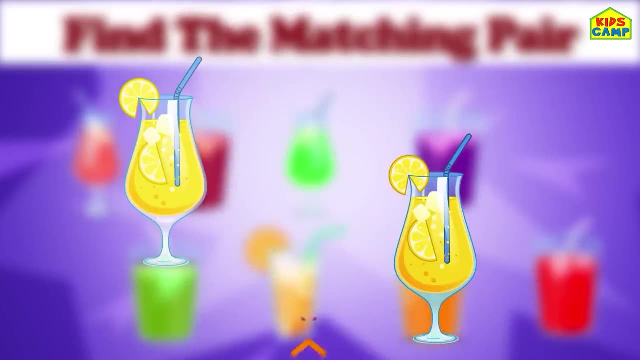 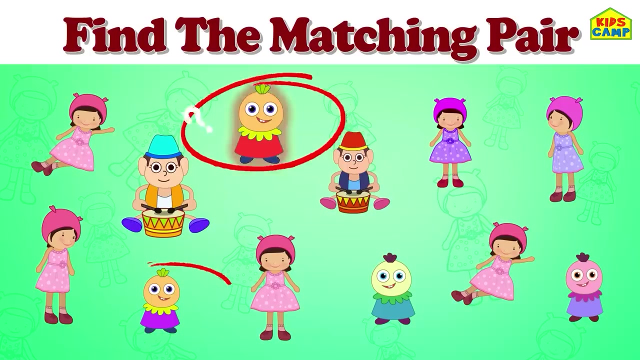 Yes, They match. That's right, These sheep match- Perfect. Find the matching coolers. Do these match? No, Do these match No. Yes, We've found the pair. Find the matching pair. Let's look for one. 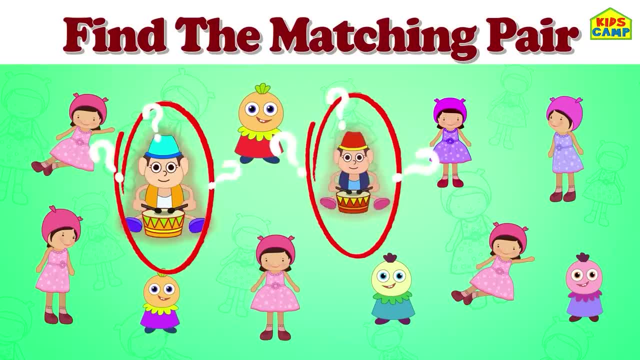 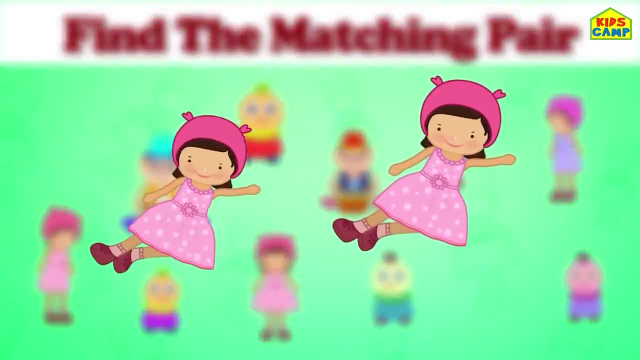 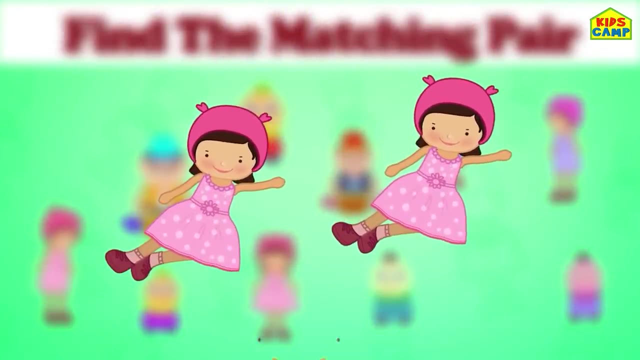 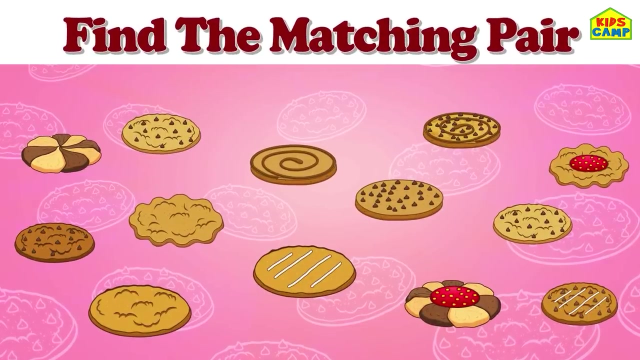 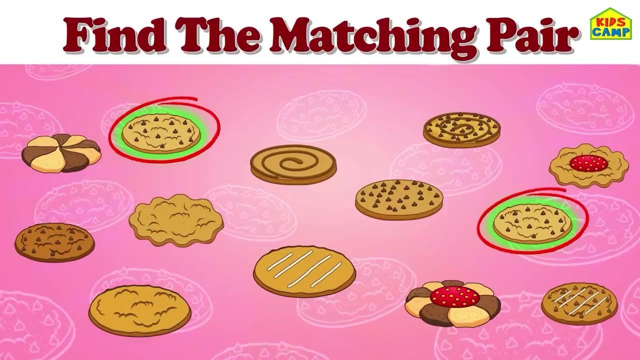 No, No way, That's right, We found the pair. Yay, Good job, friends, This game is so much fun. Ooh Cookies, Find the matching pair. No way, Yes, We found them. I love cookies. 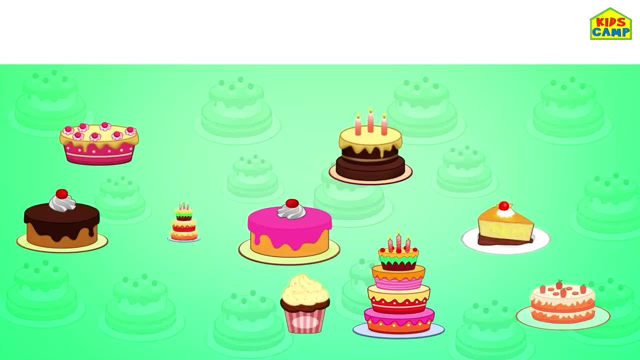 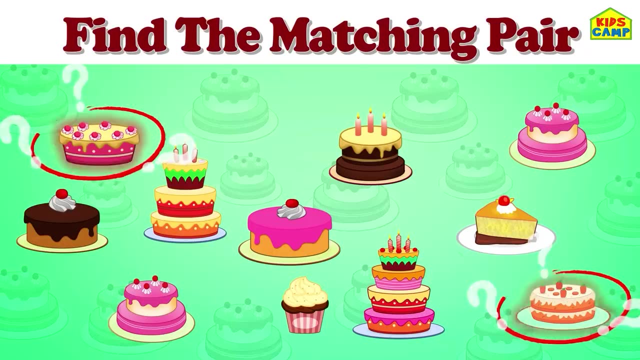 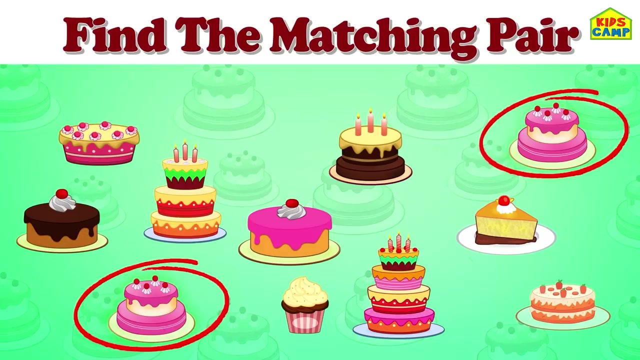 Yummy, Let's go to the next one. Hmm, Cakes. Find the matching pair. No, No, Yes, That's right, The matching pair of cakes. Yummy, Wonderful Ooh Donuts. Find the matching pair. 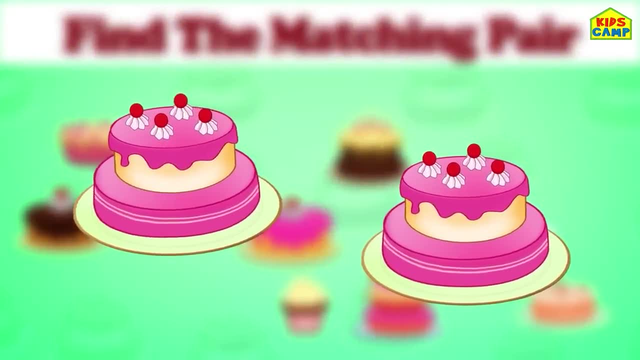 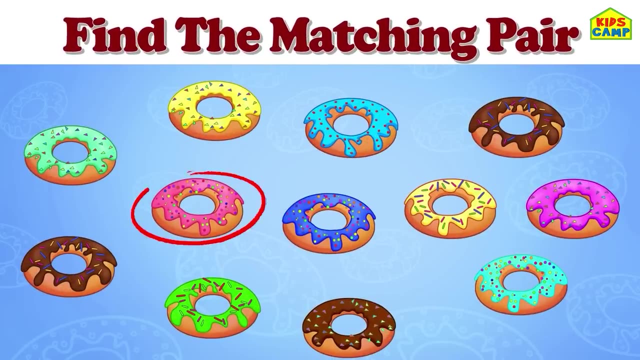 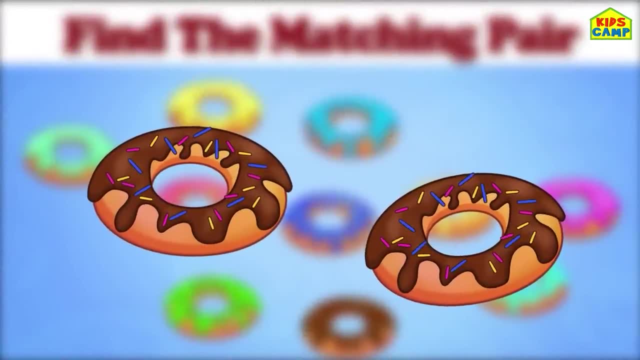 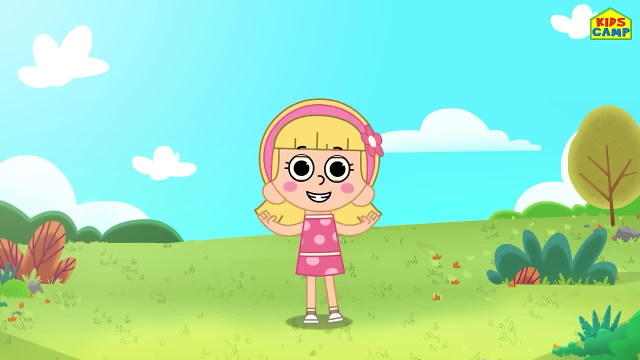 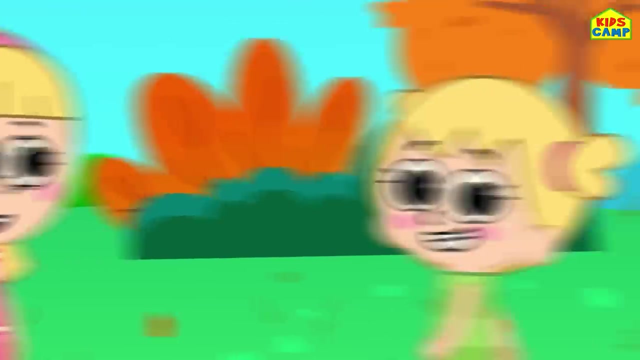 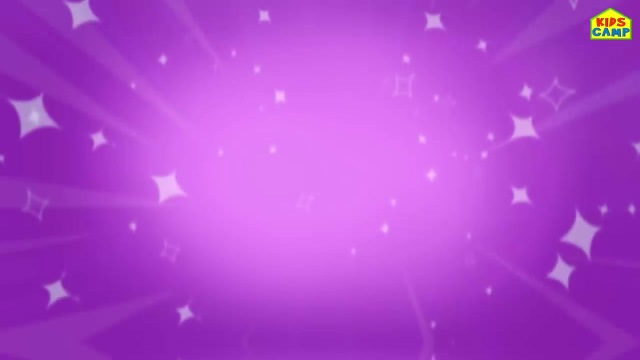 No, No match. this was such a fun game. friends, keep watching kids camp. bye, bye, hi friends, I'm Ellie and this is Eva. today we're going to play a fun game of hot and cold. that's right. we have to start according to what is hot and what is. 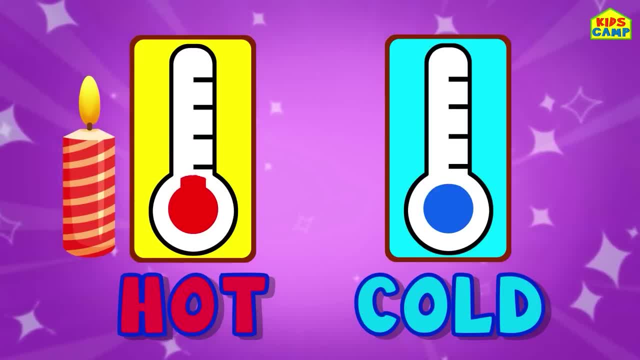 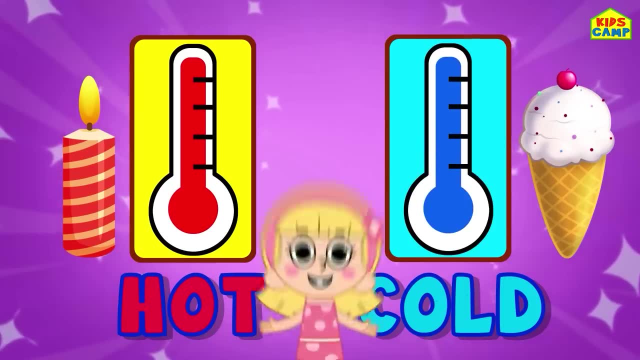 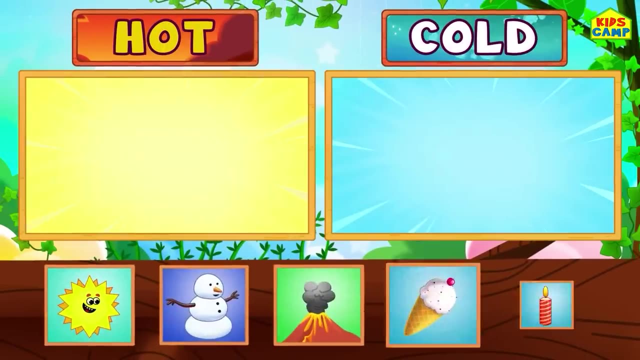 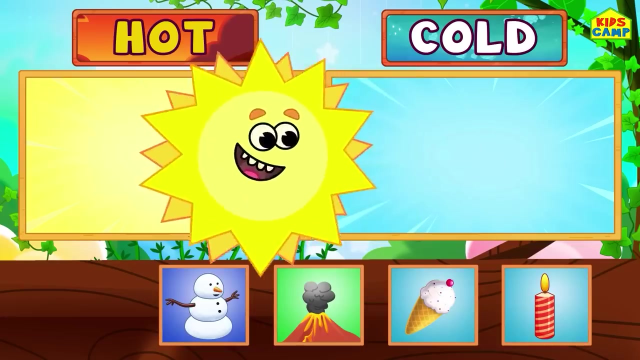 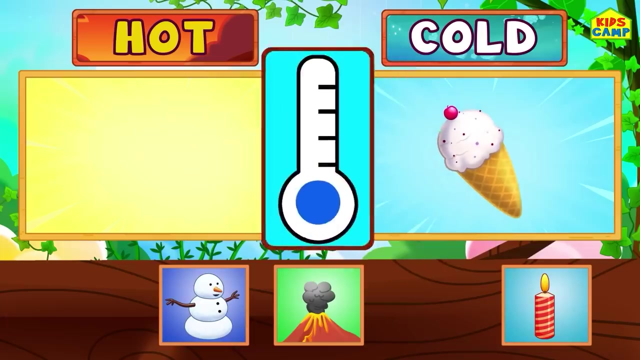 cold. for example, a candle is hot, that's right, and an ice cream is cold, that's right. wonderful, this is going to be easy. let's get started. is Sun hot or cold? that's right. Sun is hot, very, very hot, that's right. ice cream- yummy, a candle. 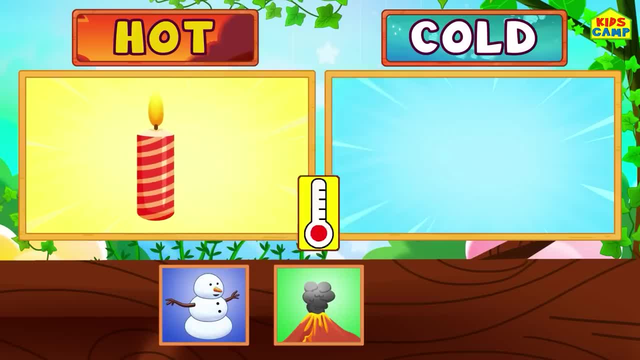 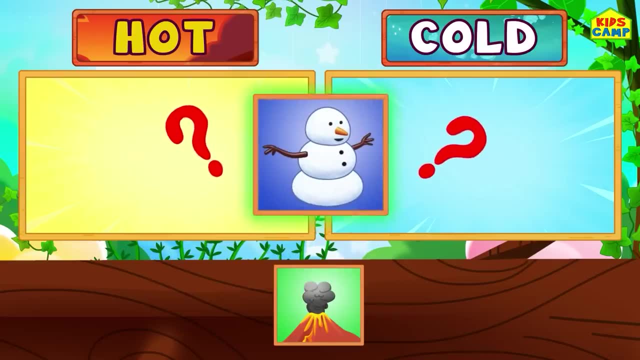 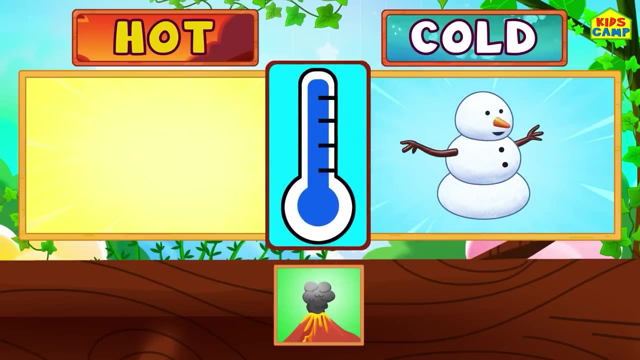 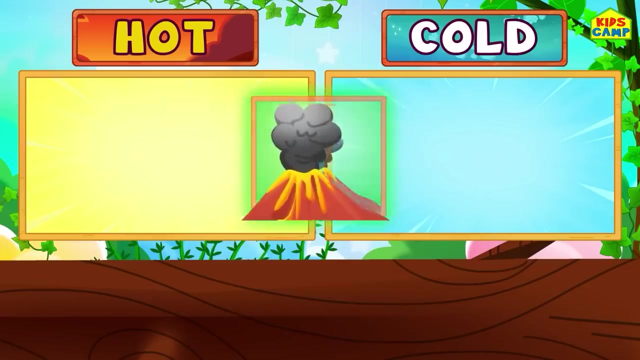 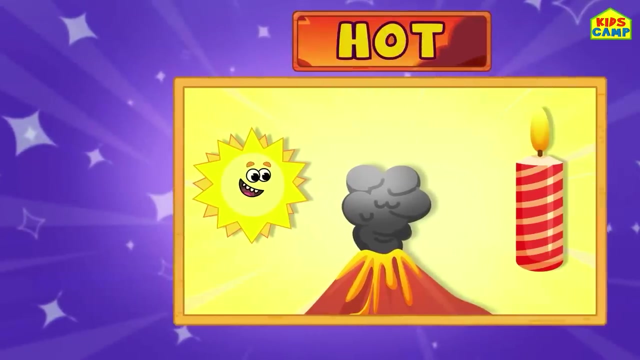 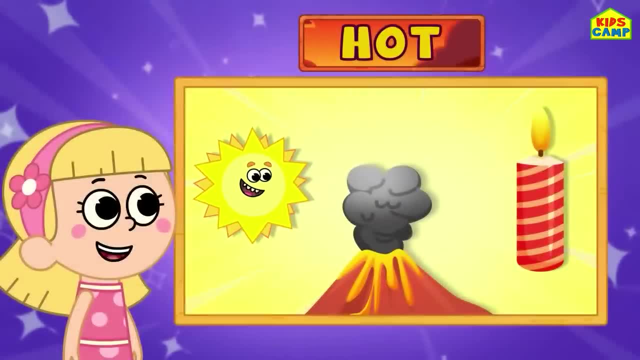 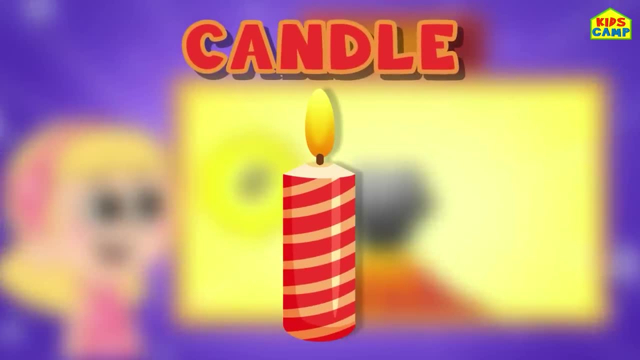 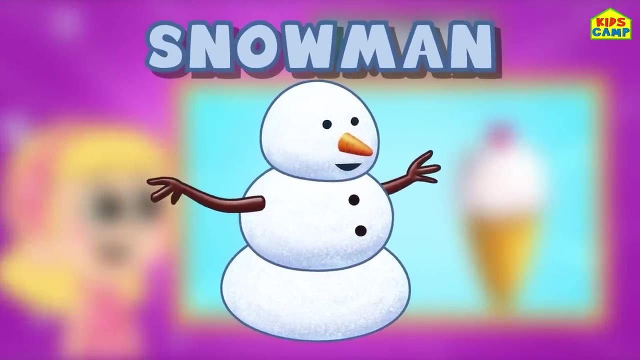 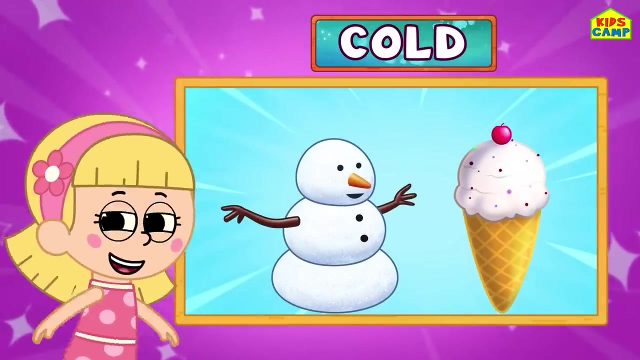 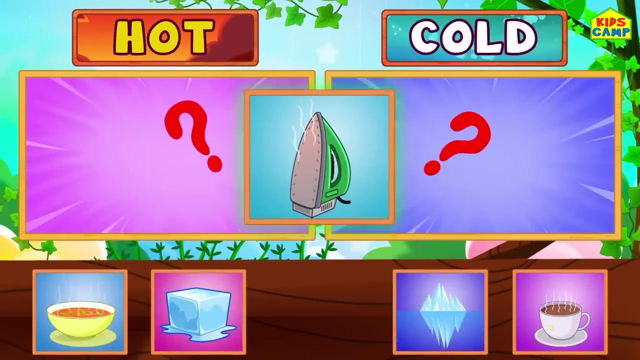 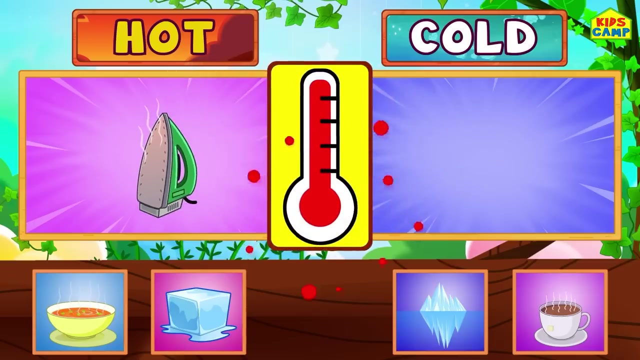 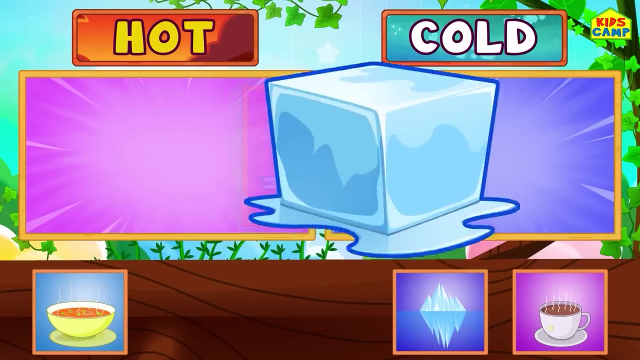 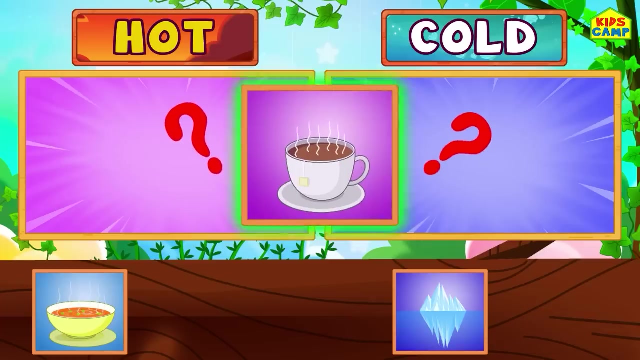 Sun, oh, volcano and the flicker cool, and we found the snowman and the ice cream all cold, be mine, yay. next is the easy game and iron, hot or cold, its suppose to be прямо azの. hot or cold, hot, that's right. an ice cube cold, very cold. a cup of coffee hot or 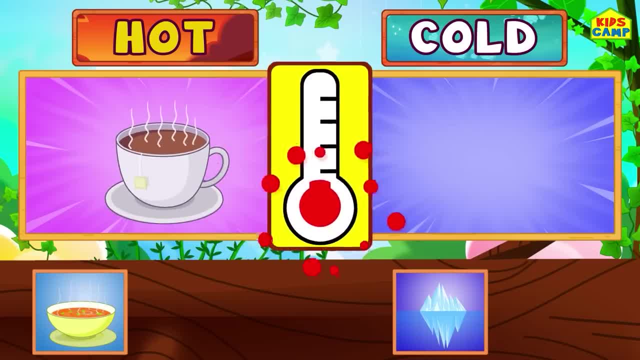 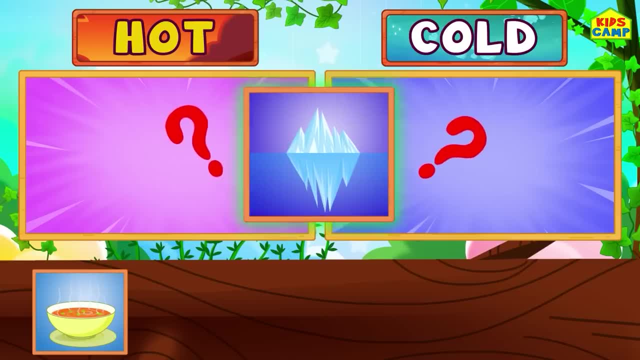 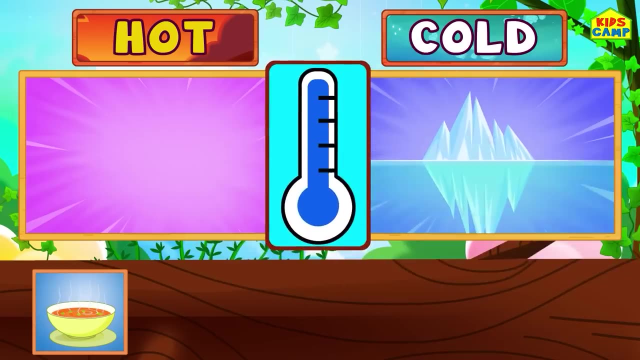 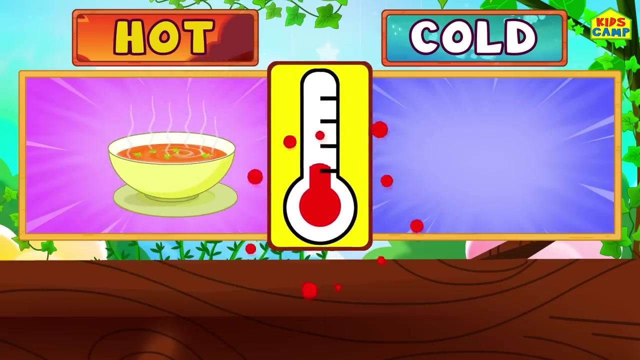 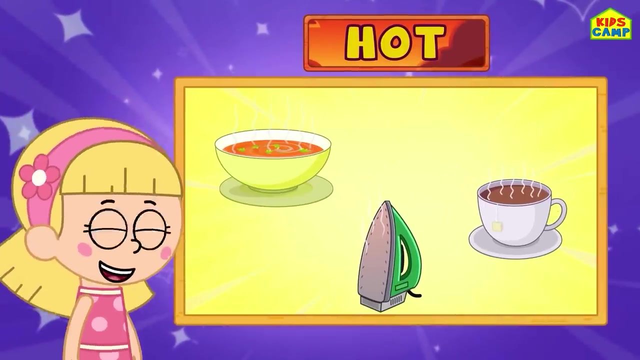 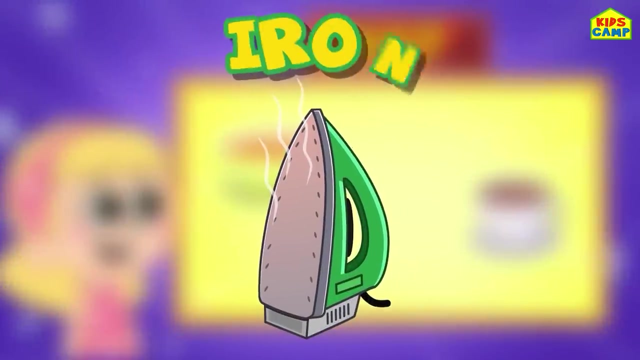 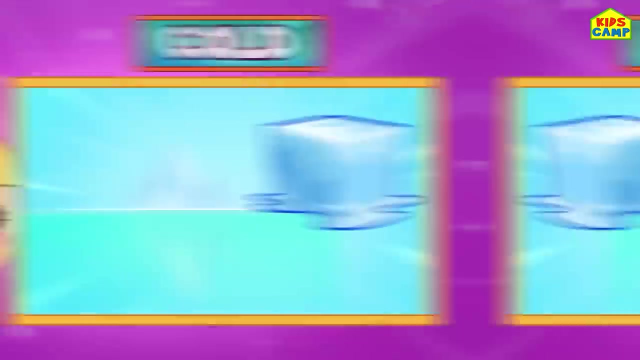 cold. hot, that's right. an iceberg: it's cold. good job. a bowl of soup, that's right. hot. wonderful. what did we learn? a bowl of soup is hot, an iron is hot and a cup of coffee is hot as well. an iceberg. 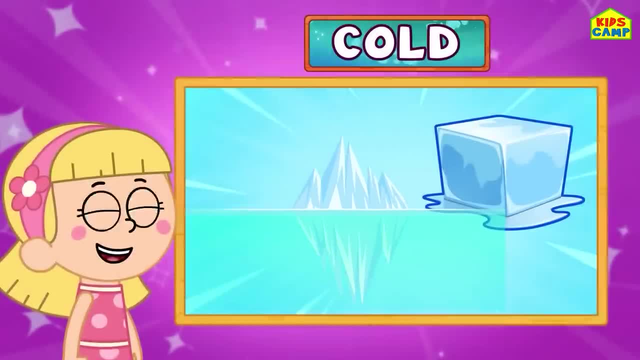 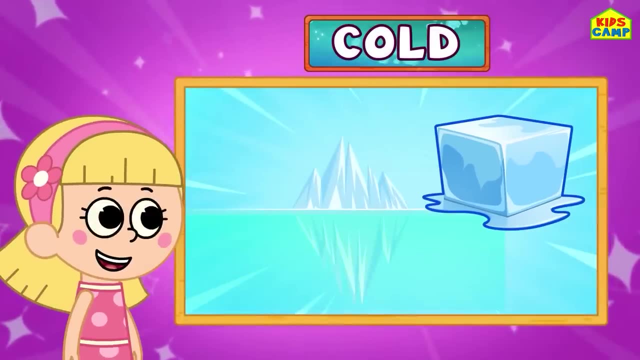 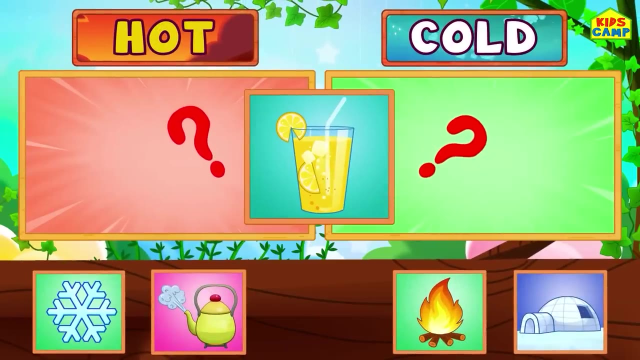 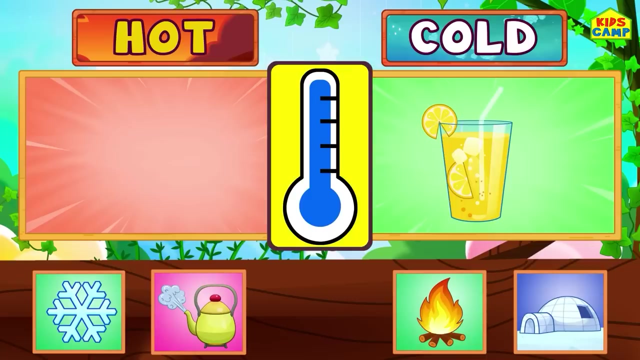 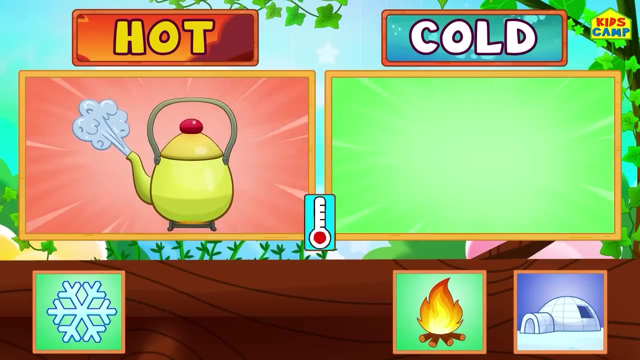 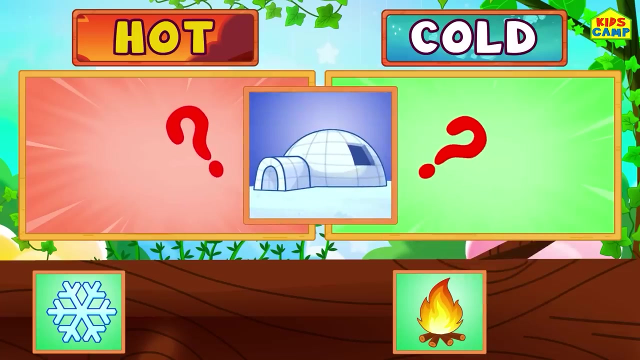 is cold. and an ice cube is cold too. that's right. yay, what's next? we're getting good at this game. a lemonade: it's cold, definitely cold. a kettle: it's hot, that's right, hot kettle. an igloo: that's right. an ice cube: that's. 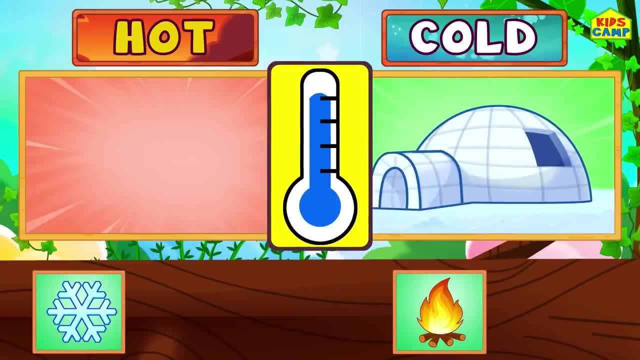 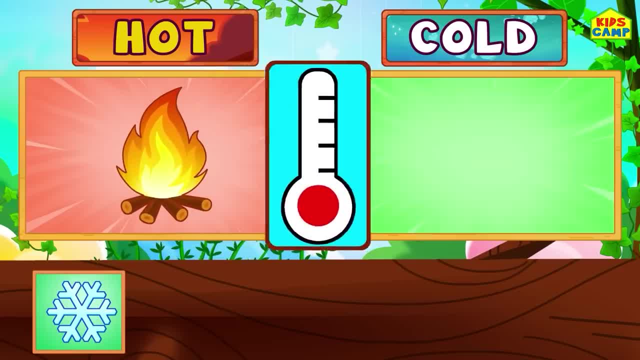 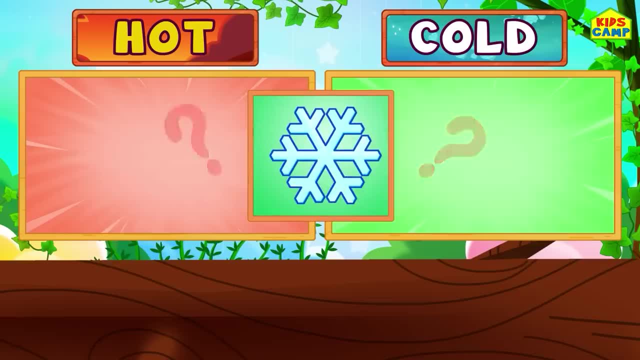 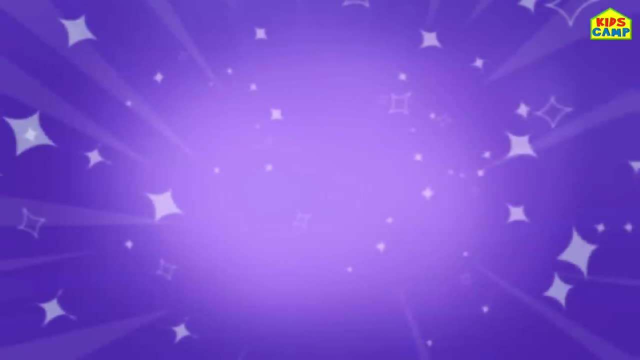 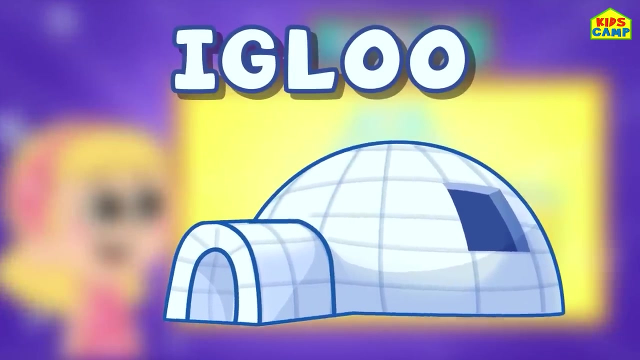 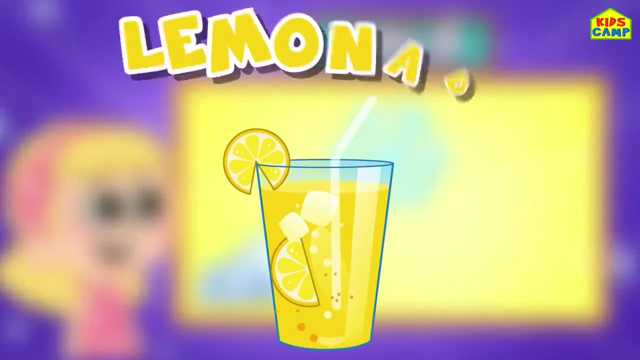 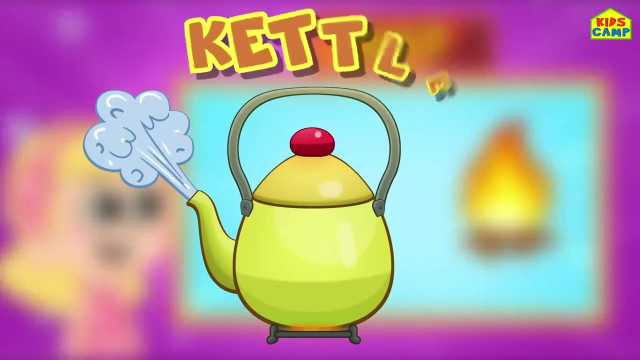 right, an ice cube definitely cold, cold, amazing. very good, I think I've got my strange confusion set. the ice cube is cold. fire, That's hot, definitely hot. An igloo is cold, A snowflake is cold And a glass of lemonade is definitely cold. A kettle is hot. 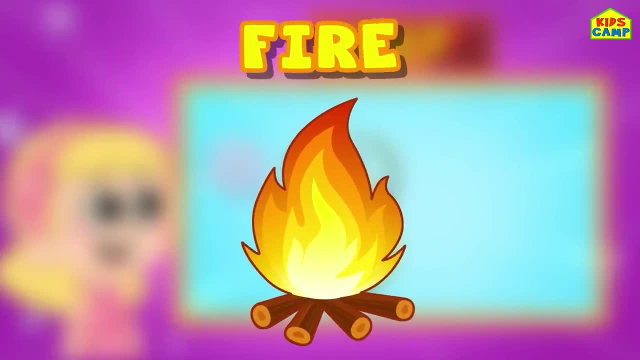 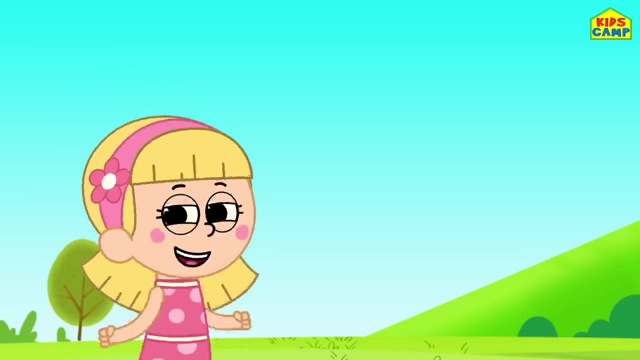 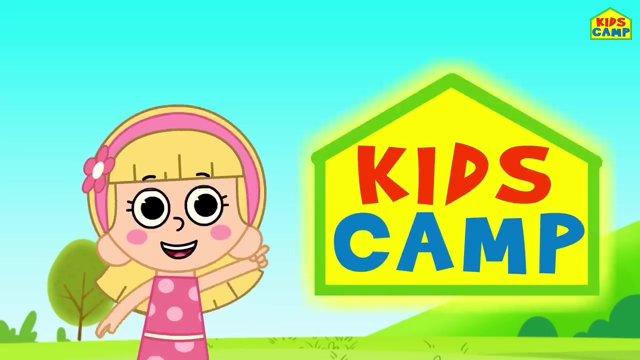 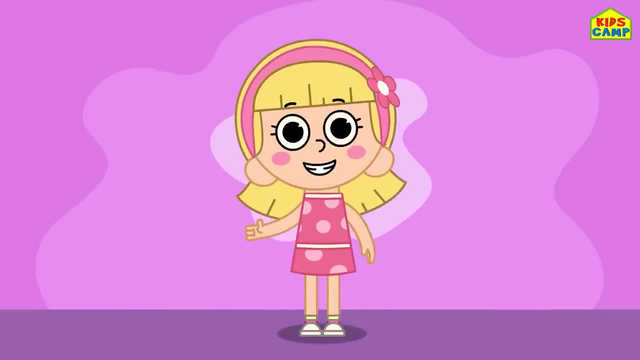 And fire is hot, Wonderful, Yay, This is so much fun learning. Come back for more. Until then, keep watching Kids Camp. Bye, Hi kids. I'm Ellie and today is Eva's birthday. Yay, Will you help me plan a birthday party for? 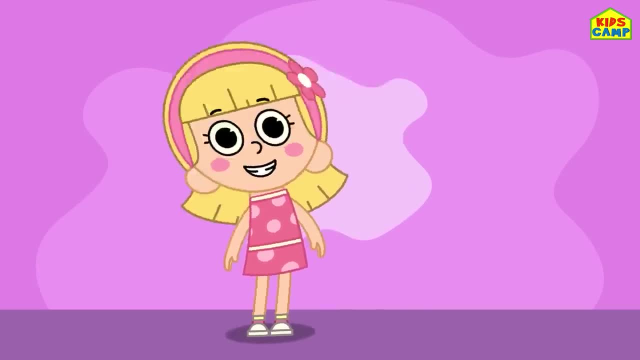 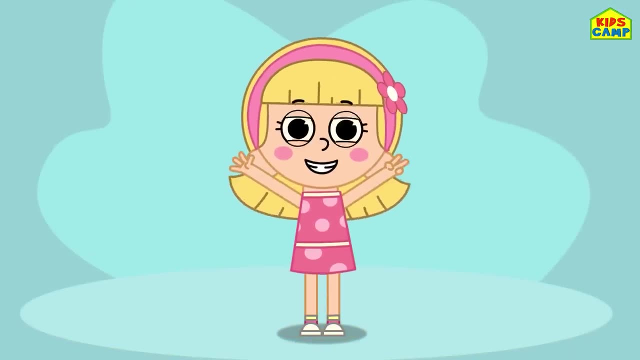 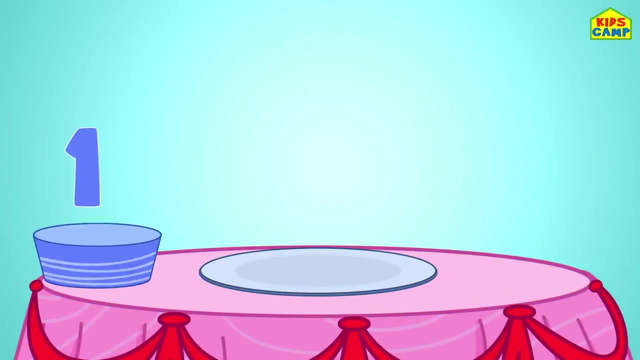 her. Yes, Let's go First. we'll need a blanket First. we'll need a birthday cake. Let's bake one. How many layers of sponge do we add to Eva's birthday cake? Let's count One, two, three, four, five. 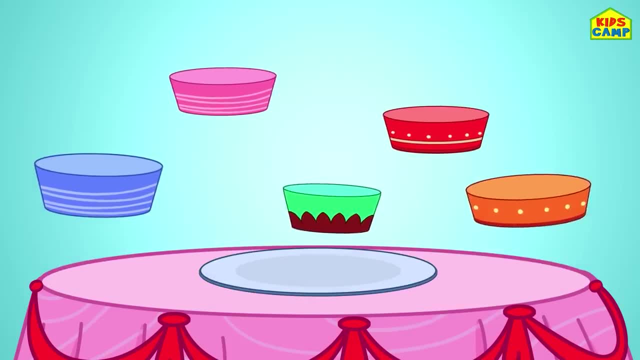 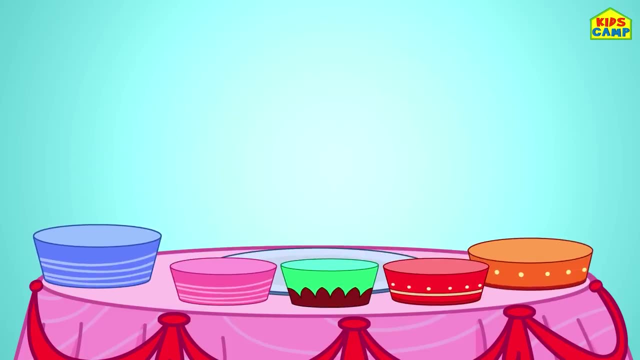 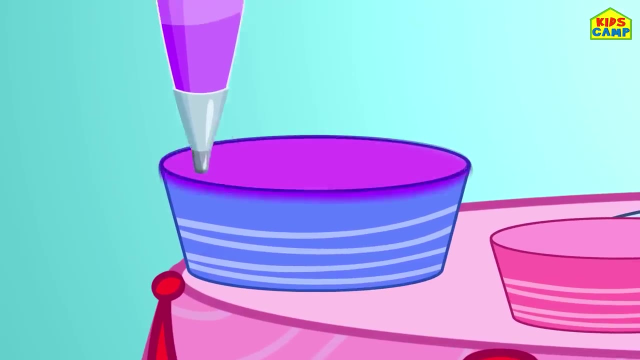 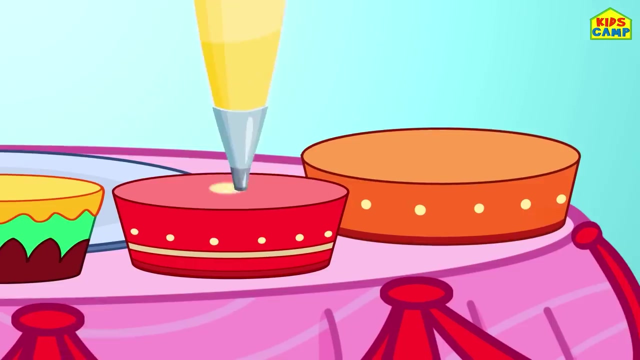 Five layers of cake. What else can we add on the cake? That's right, Ice. One, two, three, four, five. Let's add one layer of icing. Let's add… On the first layer, on the second, on the third, on the fourth and the fifth. 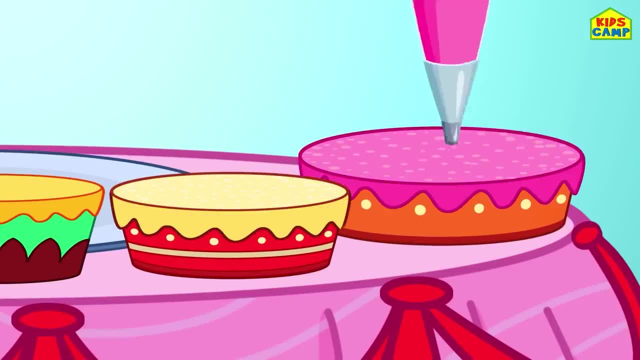 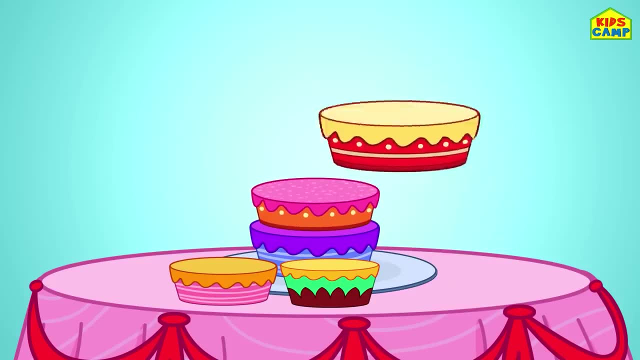 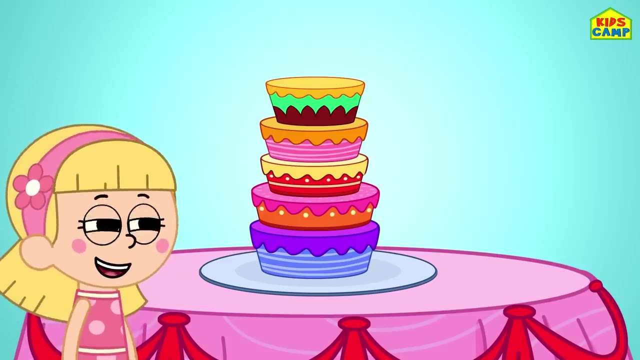 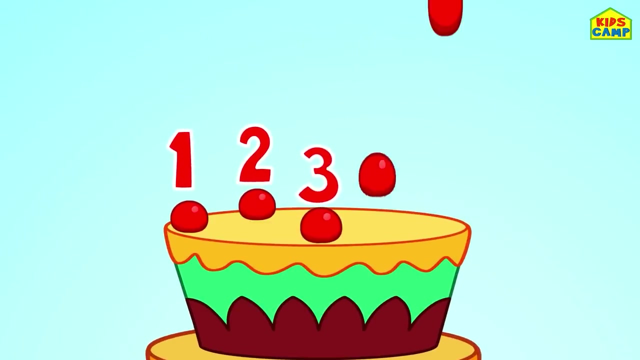 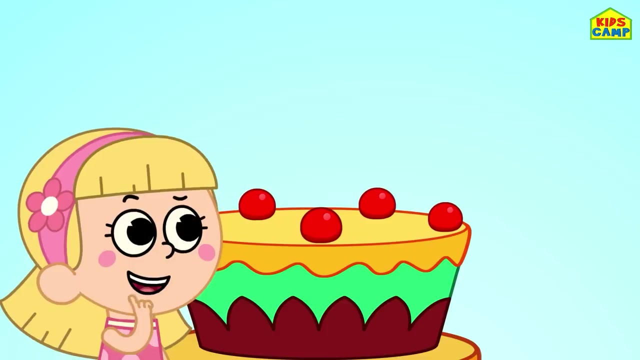 Woohoo, Five layers of icing. It looks yummy. Now let's add four layers of icing. toppings: let's add one cherry, two cherries, three cherries, four cherries, five cherries, yay, five cherries. hmm, what do you think is missing? candles, that's. 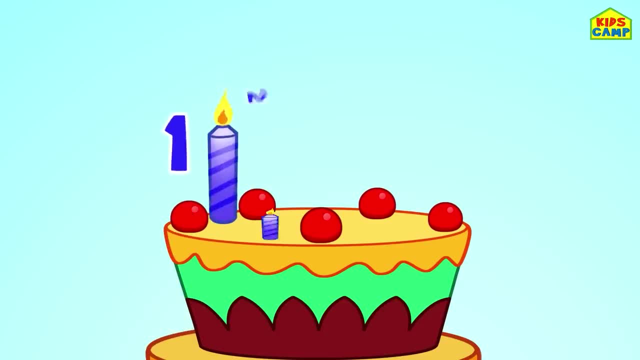 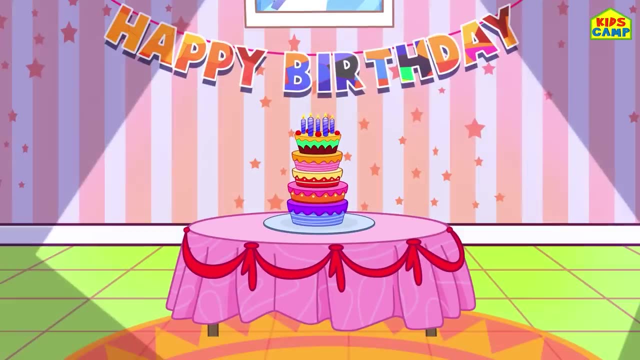 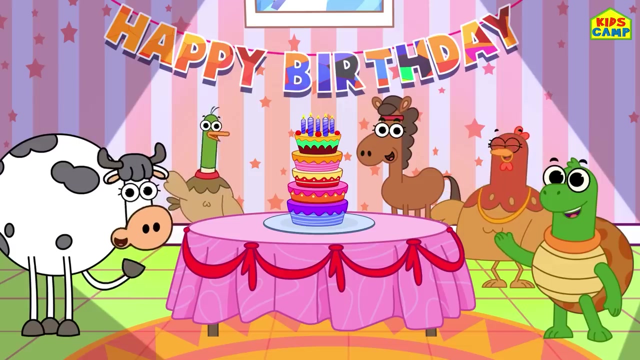 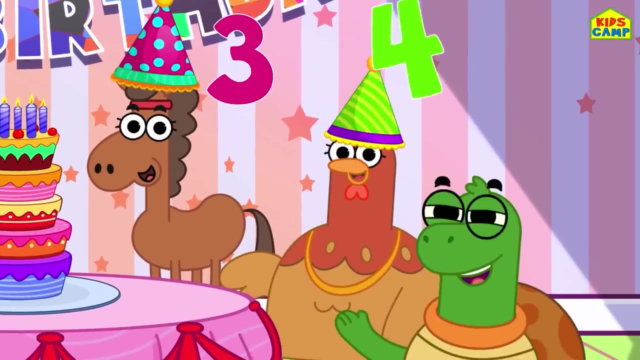 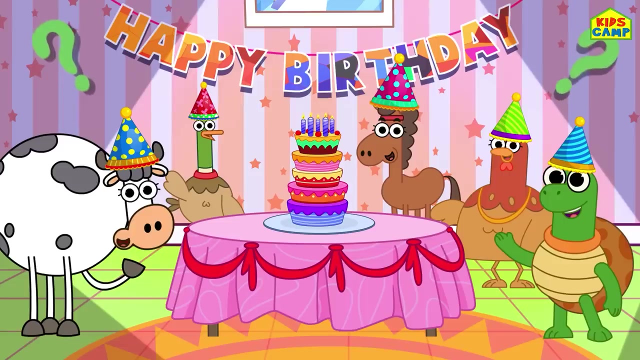 right, let's add candles: one candle, two candles, three candles, four candles, five candles. yay, Wow, everyone's here. hi, everyone. we need party hats. how many party hats do we need? one, two, three, four, five, five party hats? hmm, what else do we need? hmm, something's missing, that's right, we need balloons. 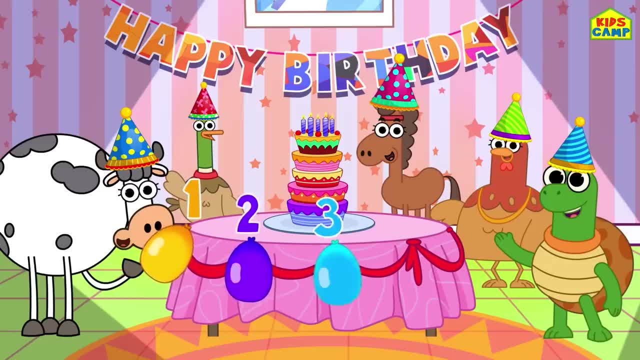 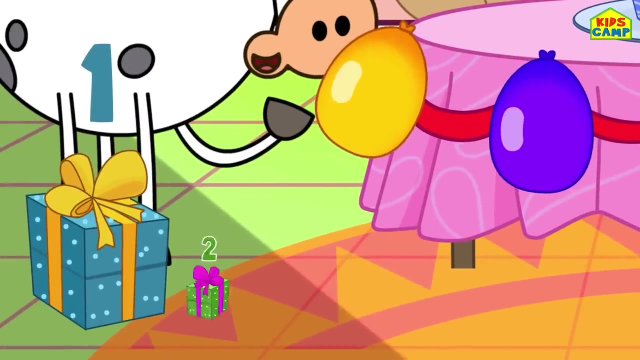 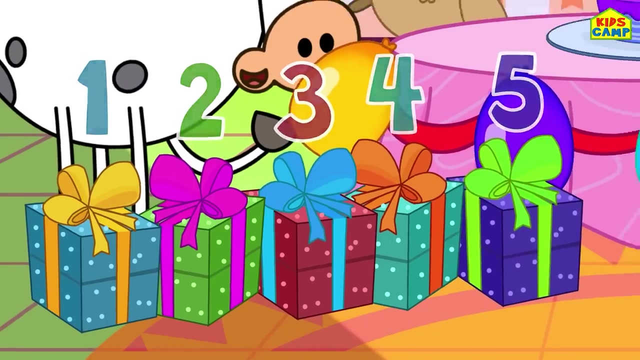 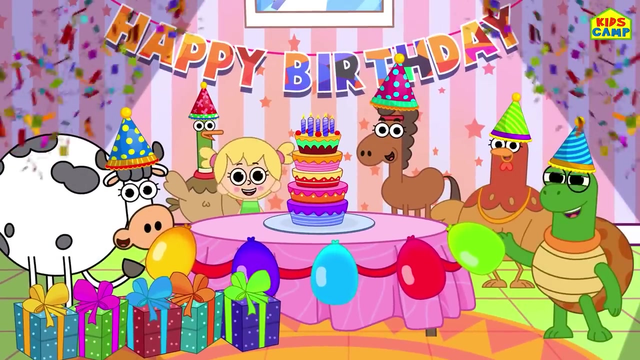 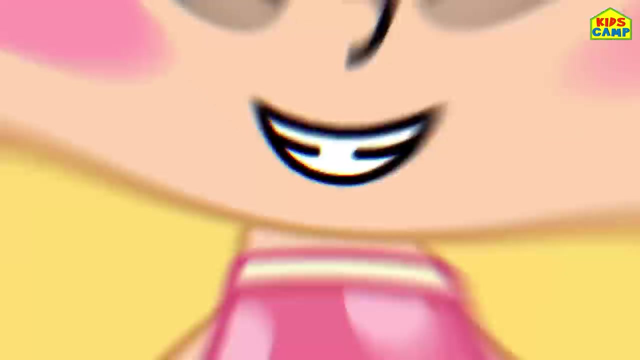 one, two, three, four, five, five balloons. oh, this is now starting to look like a birthday party. everyone's got presents for Eva. let's keep them here and count. here we go: one, two, three, four, five, five presents. let's get this party started. where's Eva? there? she is surprise. happy birthday, Eva. this is so much fun, and so is 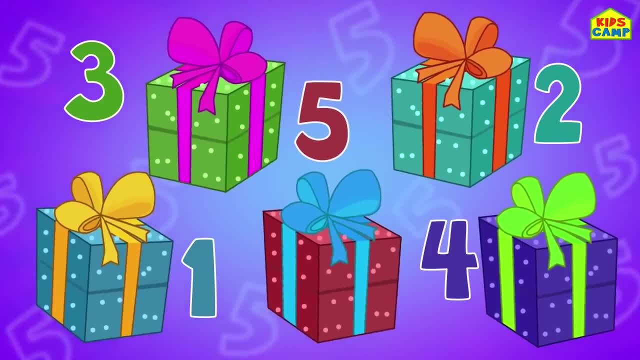 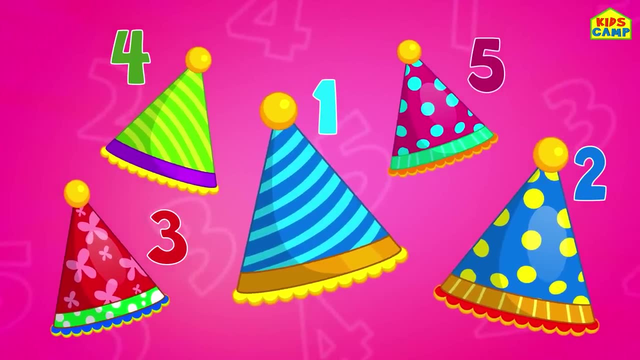 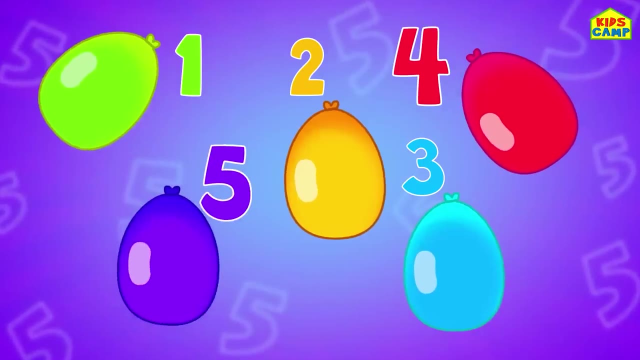 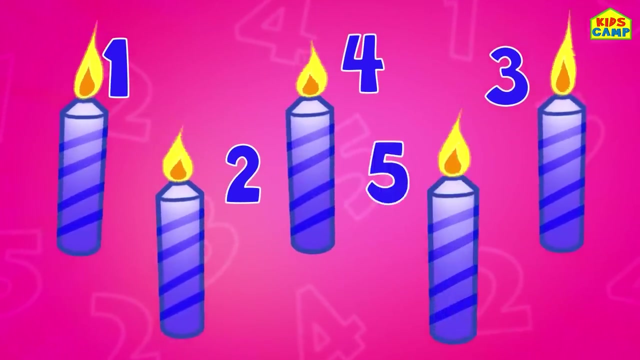 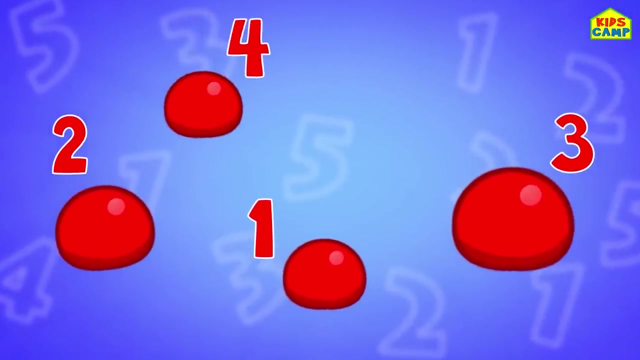 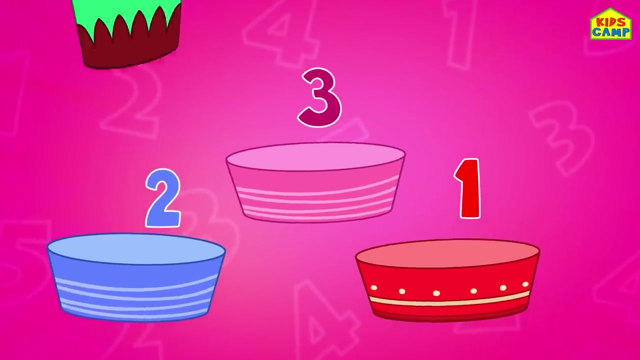 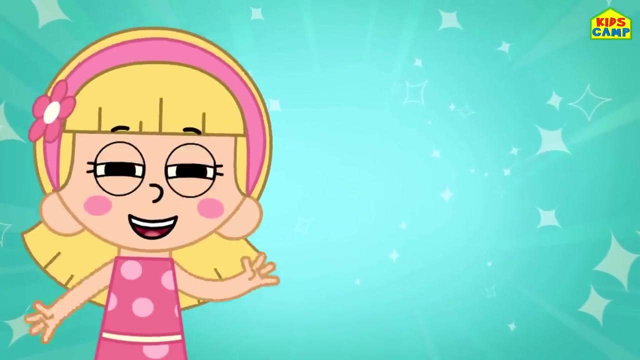 five, five presents: one, two, three, four, five, five. party hats: one, two, three, four, five five. balloons: one, two, three, four, five five. candles: one, two, three, four, five, five. cherries: one, two, three, four, five, five. layers of cake. this was so much fun. it was the best party ever. bye, bye. 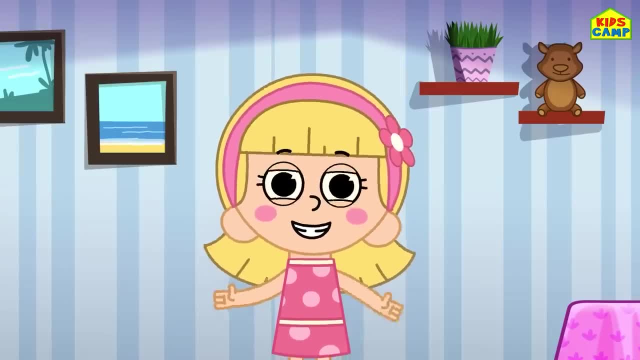 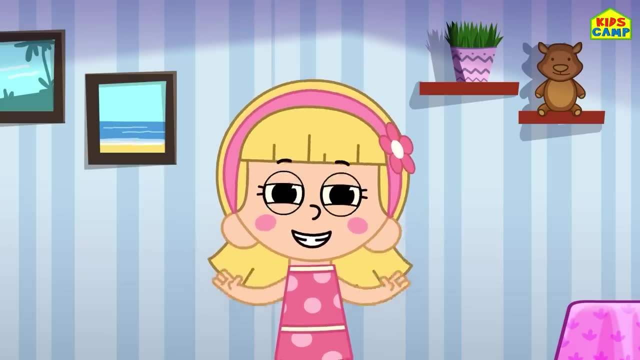 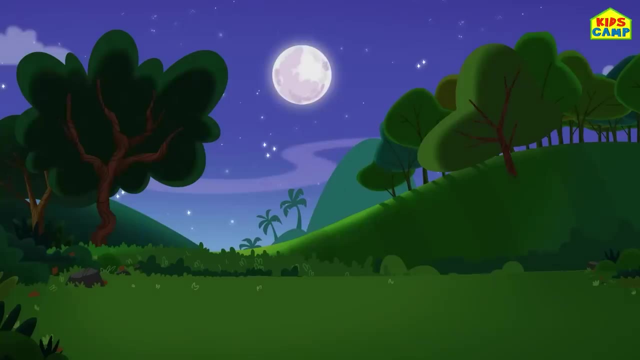 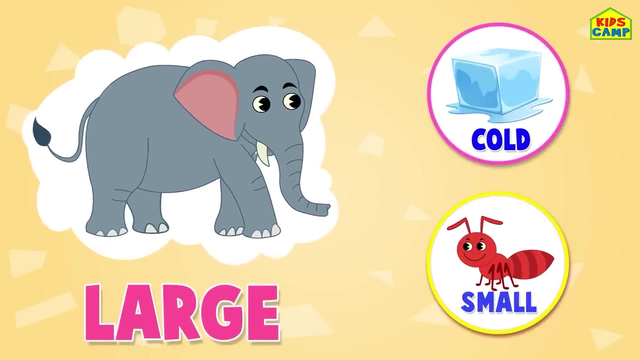 hi, I'm Ellie, and today we're going to learn opposites. what is an opposite? an opposite is when two words contradict each other. for example, if it's daytime, the opposite of day is night. right ready, here we go. what is the opposite of large? is it small or cold? it's small, that's right. 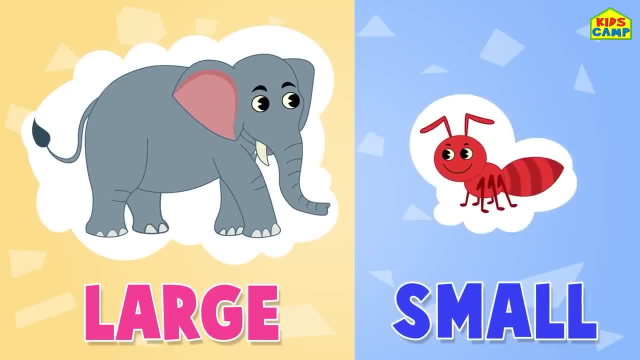 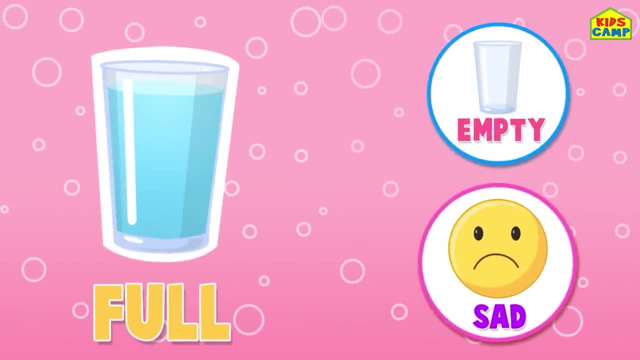 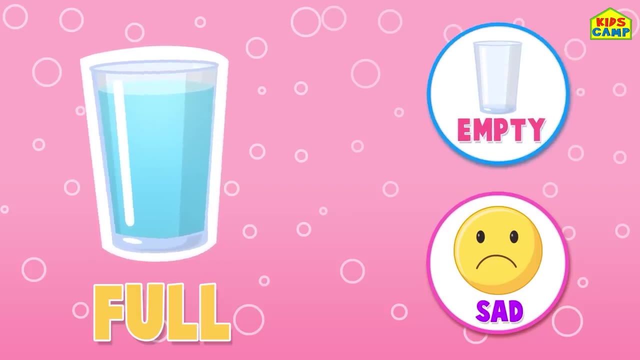 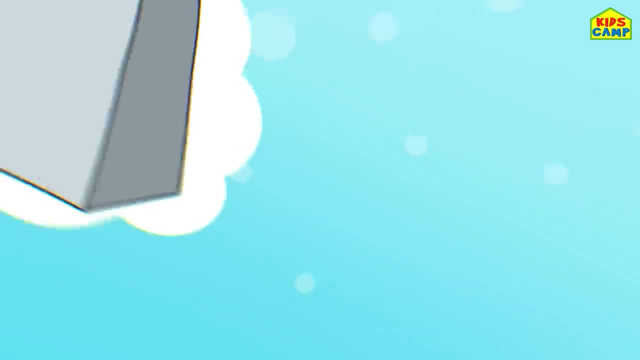 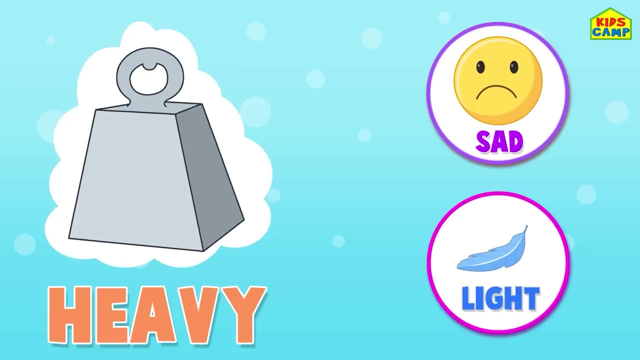 the opposite of large is small or cold. it's small. that's right. the opposite of large is small. what is the opposite of full? is it sad or is it empty? the opposite of full is empty. that's right. what is the opposite of heavy? is it light or sad? it's light, the. 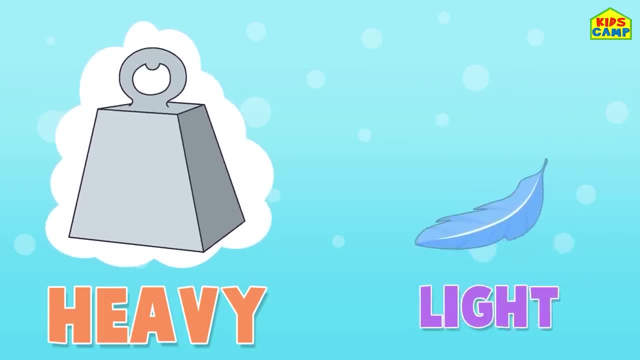 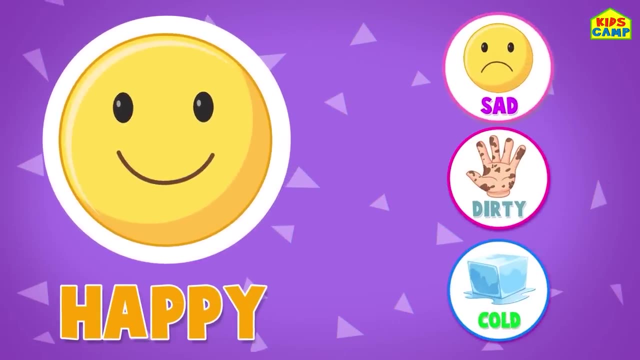 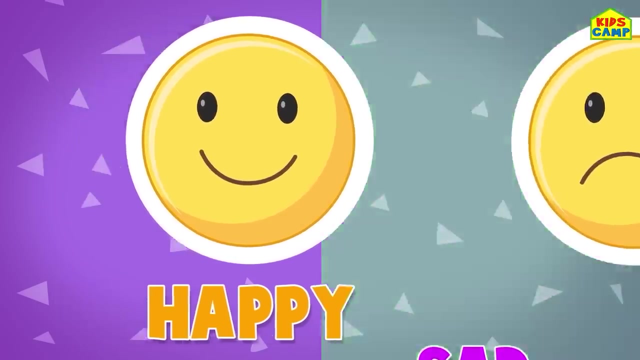 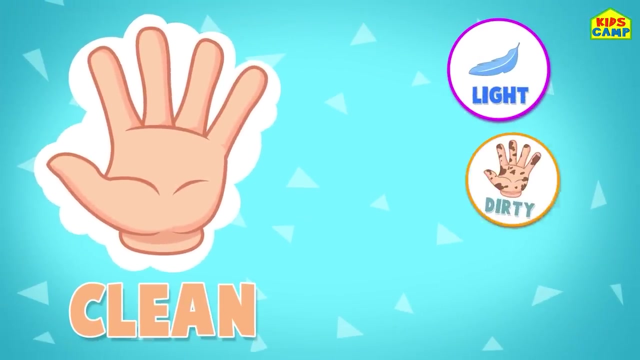 opposite of heavy is light. what is the opposite of full? is it empty or is it empty? what is the opposite of happy? is it sad? is it dirty or is it cold? it's sad, that's right. the opposite of happy is sad, and i feel happy right now, yay. what is the opposite of clean? 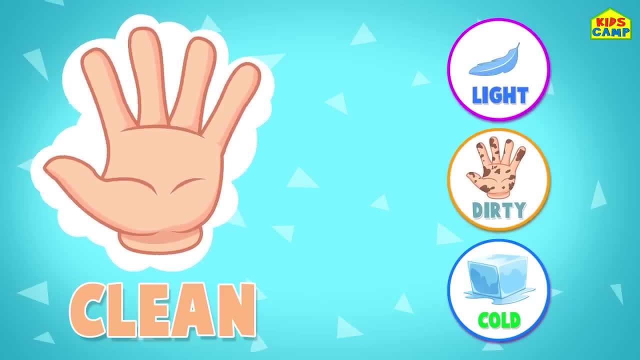 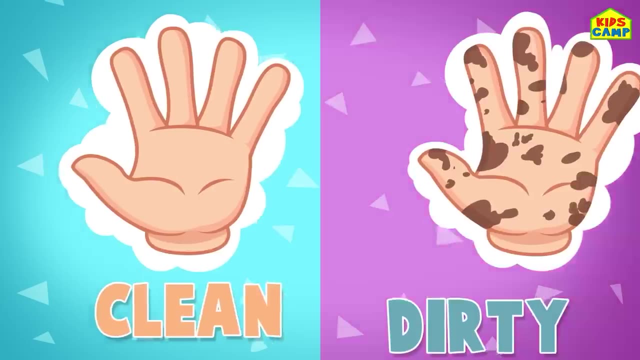 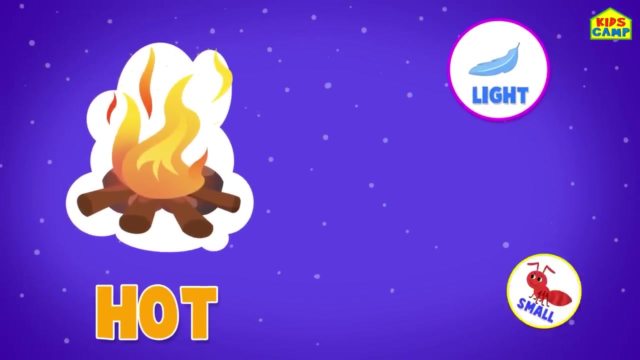 what is the opposite of dirty? is it dirty, is it light? is it hot or is it dirty? what is the opposite of dirty? is it hot or is it dirty? that's right, friends. it's their dirty. YOU SHOULD ALWAYS keep YOUR HANDS CLEAN AND NOT DIRTY. 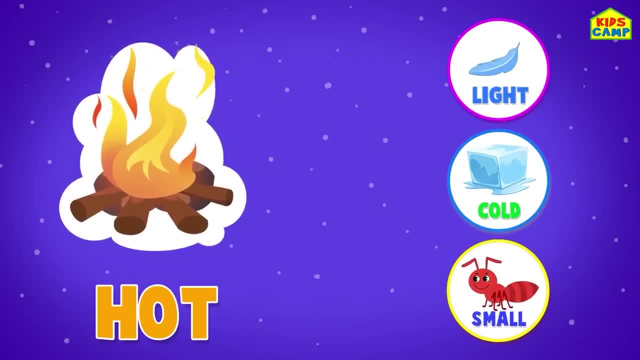 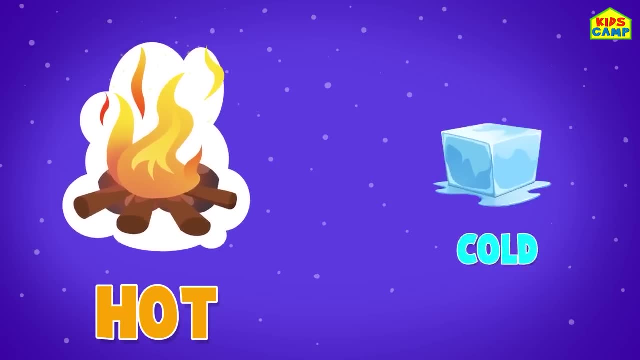 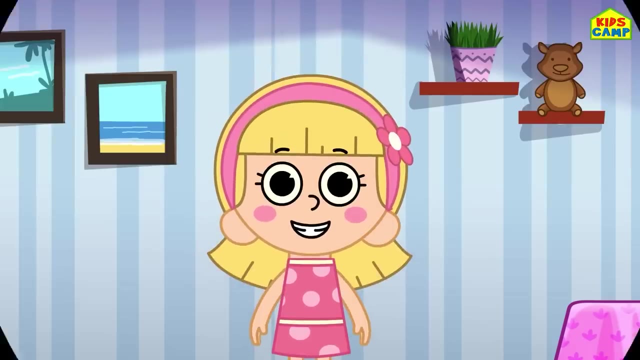 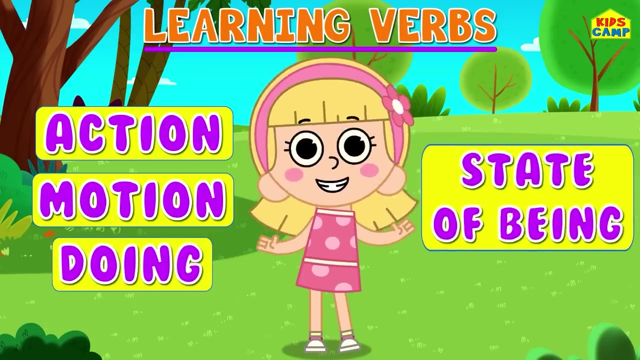 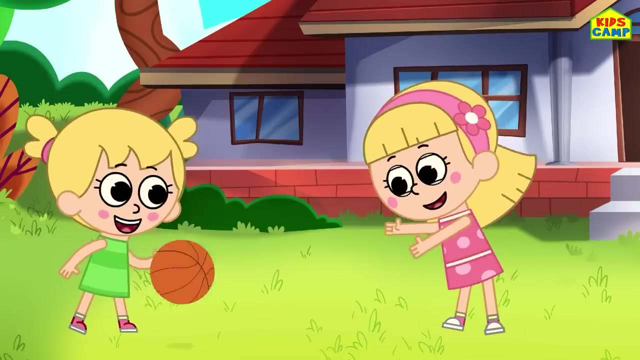 what is the opposite of hot? is it light, is it small or is it cold? it's cold. that's right of heart is cold. good job, friends, well done hi. verbs are words that show action, motion, doing or a state of being. and i am on a playground and i'm playing with eva. what we are going. 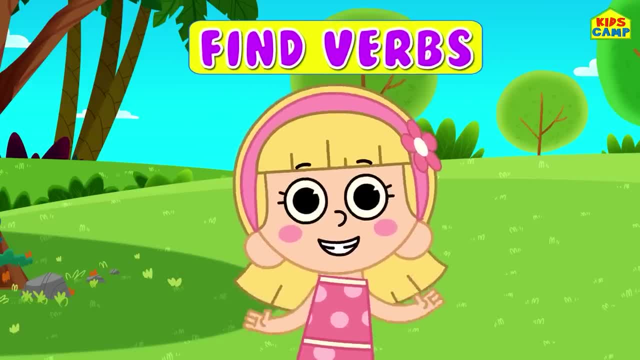 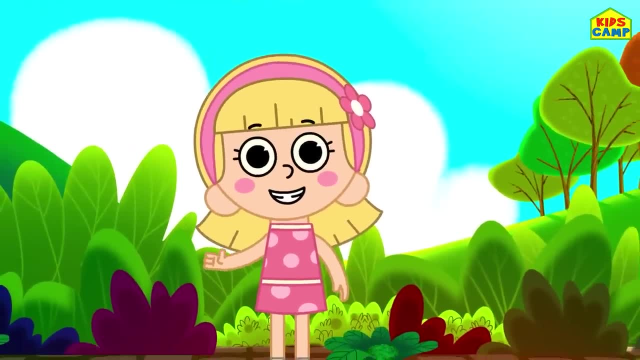 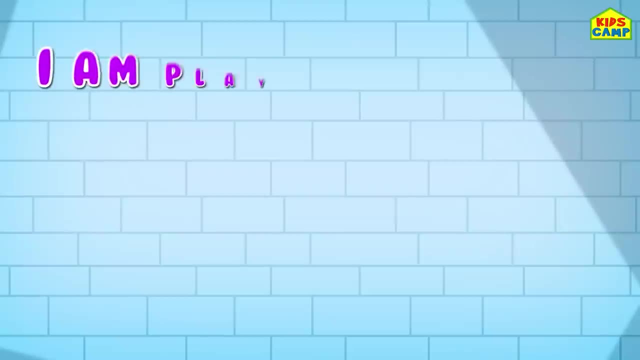 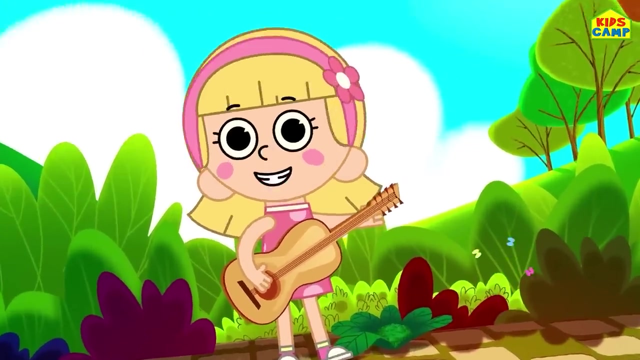 to do today is find verbs. are you ready? let's get started right away. we have to look for the verb. can you find what's the verb in the sentence i am playing the guitar? playing is the verb here? that's right. what's the activity i'm doing here? i am riding a bicycle. i'm going. 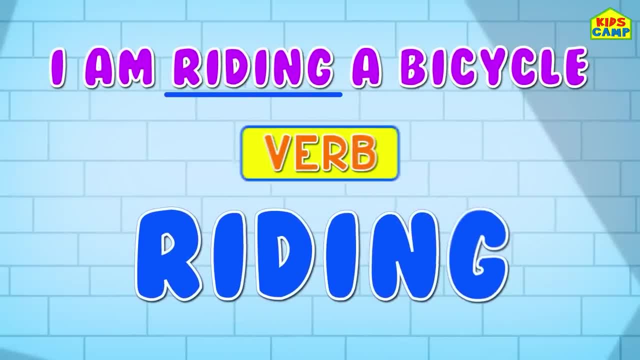 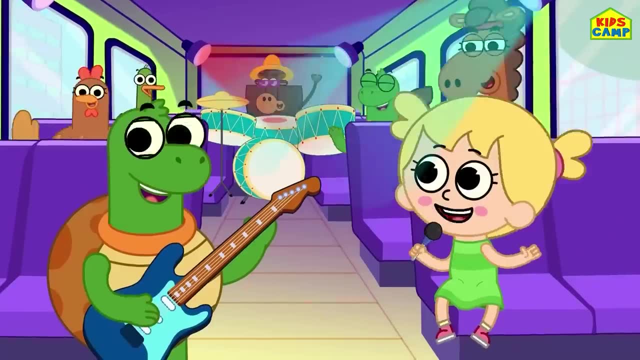 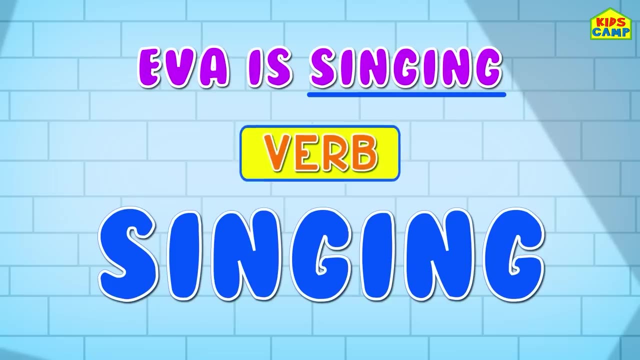 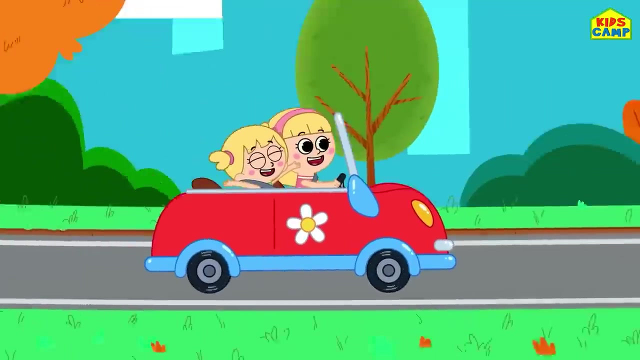 to ride a bicycle. that's right. writing is a verb. look at my little sister, eva. she loves to sing. that's right. eva is singing. singing is the word here. good job, friends. look at me, i am driving. yay, that's right. driving is the verb here. 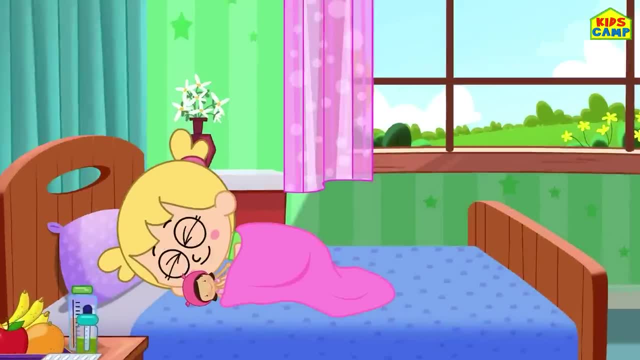 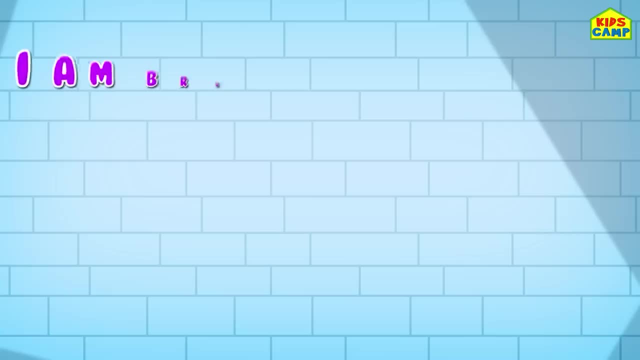 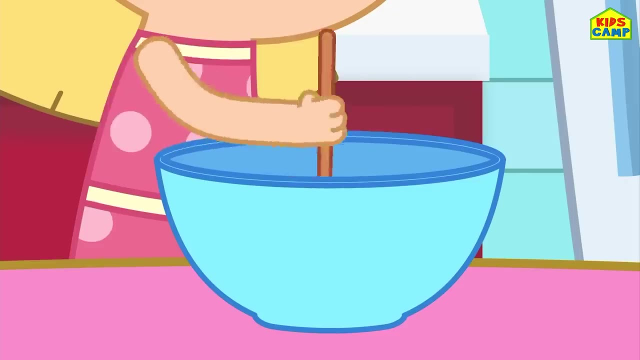 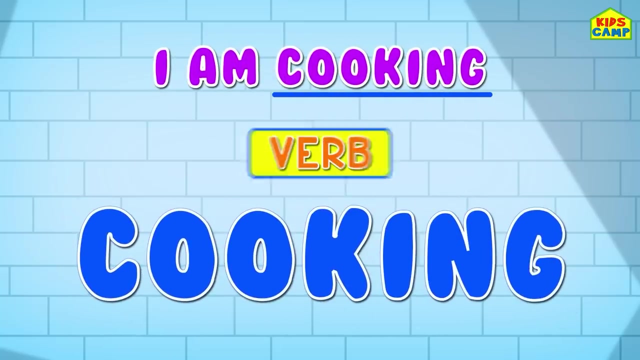 and what is it that we do the first thing when we get up in the morning, that's right. we brush our teeth. i am brushing my teeth- brushing is the verb here. evan, i love to cook, i am cooking- cooking is the verb here- and i've got a new box of. 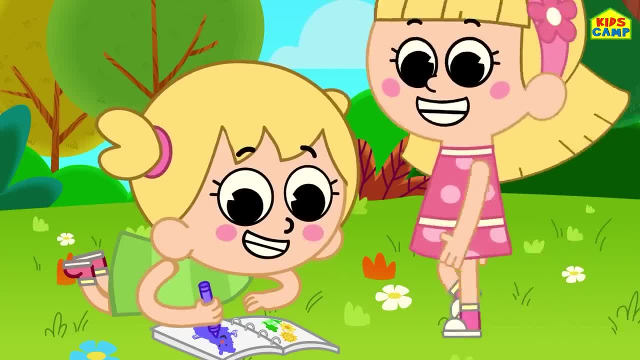 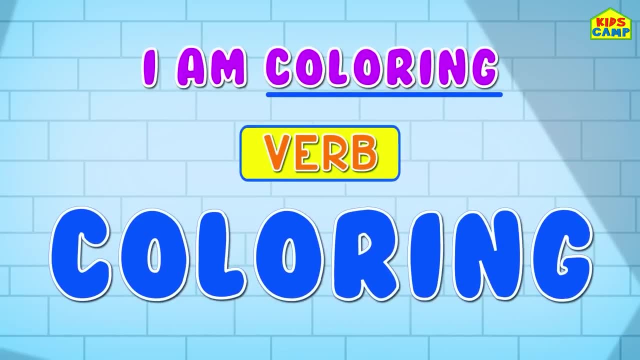 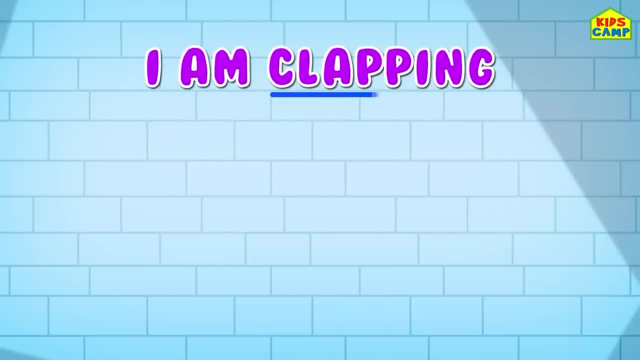 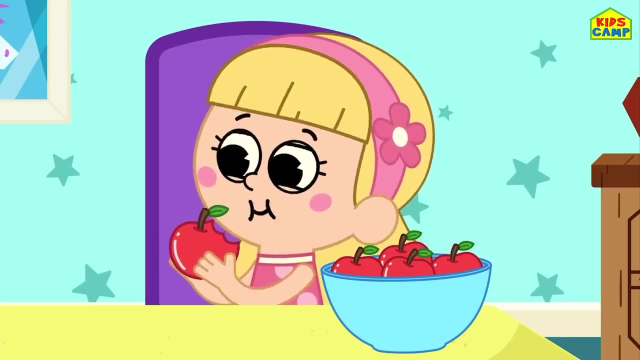 crayons. I love to use my crayons to draw and color. I am coloring. Coloring is the verb here. Woohoo, I am clapping. I am clapping. Clapping is the verb here. Woohoo, We are. 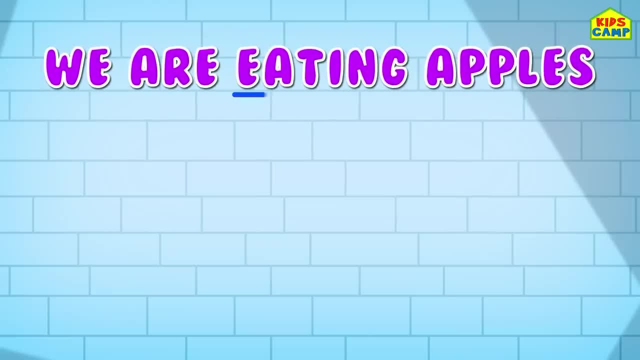 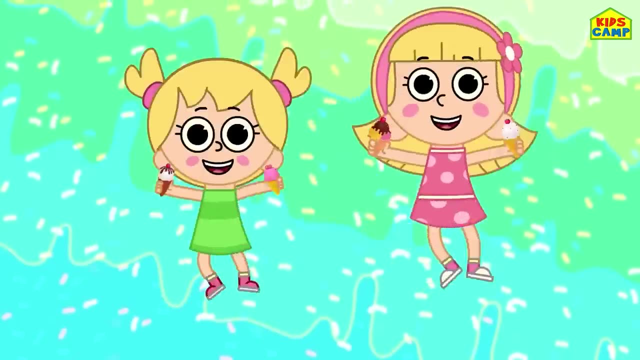 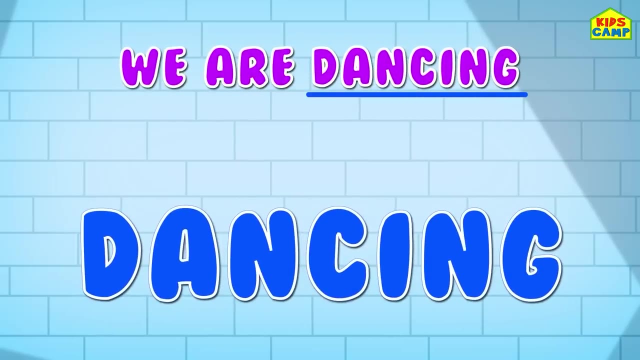 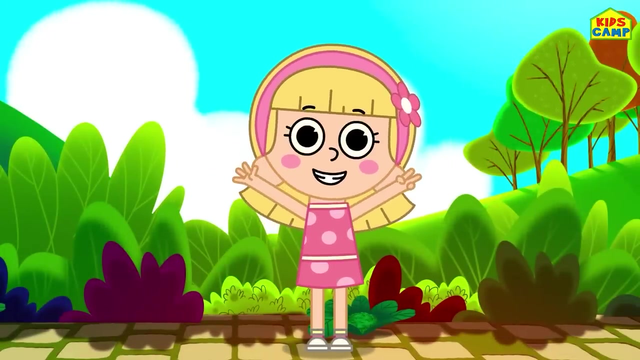 eating apples. We are eating apples. Eating is the verb here. Woohoo, That's right. We are dancing. We are dancing. Dancing is the verb here. Wow, This was so much fun. What do you like to do? Do you like to cook, play guitar, paint, sing? 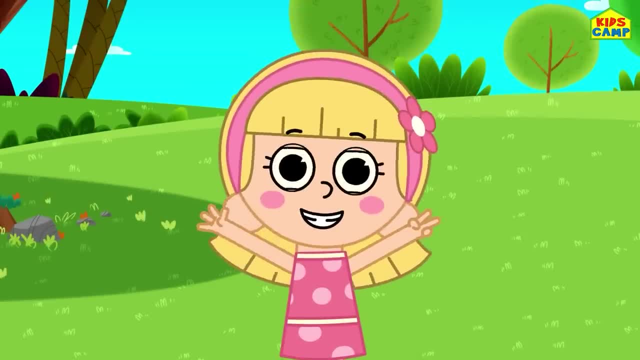 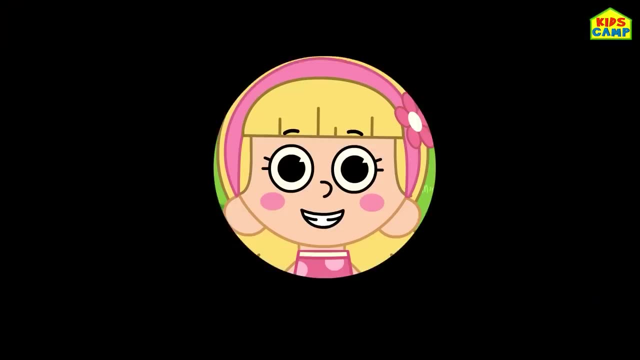 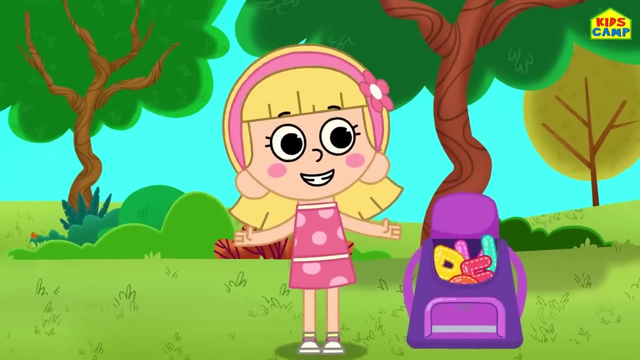 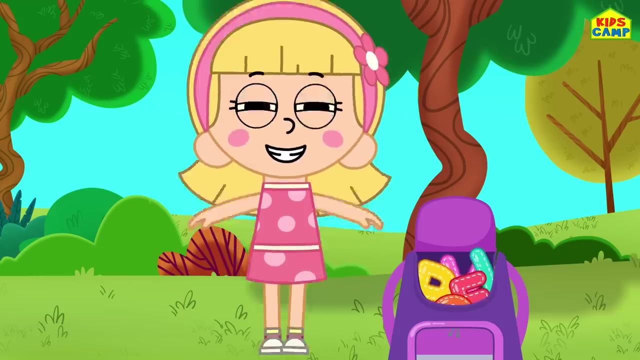 Or ride a bike. Let me know. Until then, keep watching Kids Camp. Bye-bye, Hi kids. I am Ellie and I have a bag of alphabets with lots of scrambled and jumbled letters. We have to unscramble them to find the correct word. Fun game, Let's start. 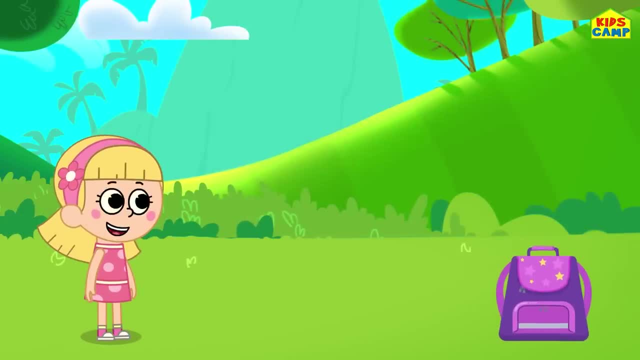 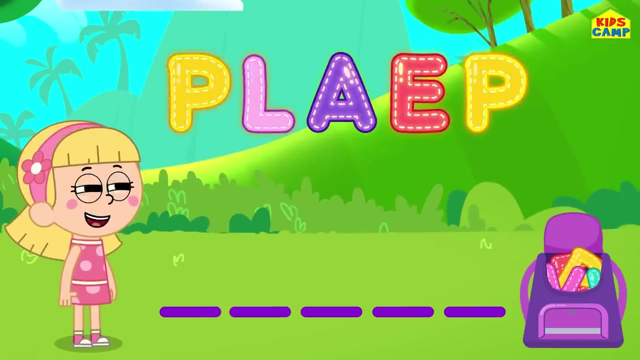 Alright, What is this? Hmm, I wonder what it is. Ah, P, L, A, E, P. Hmm, What word could this be? Oh, I know This is an apple. It starts with the letter A. 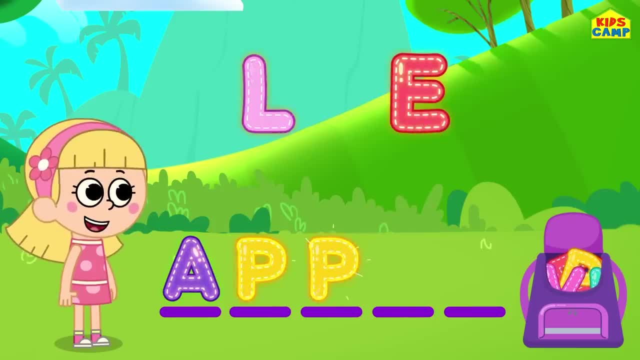 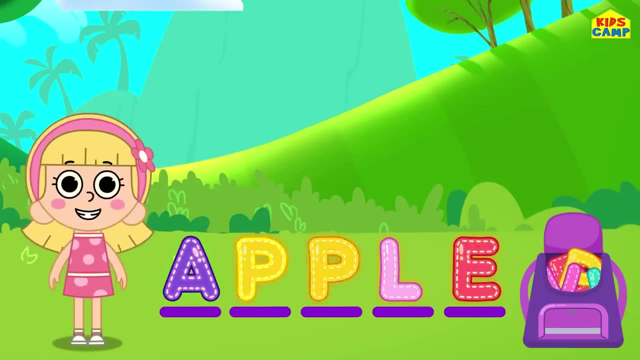 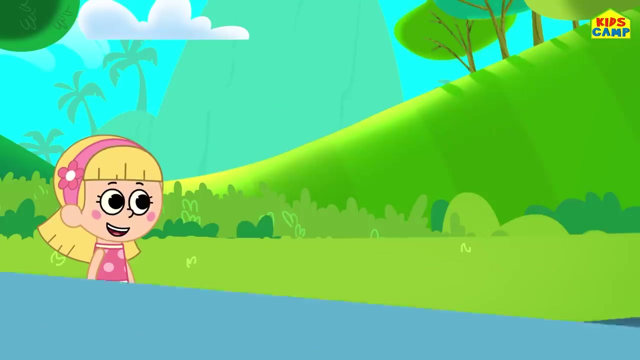 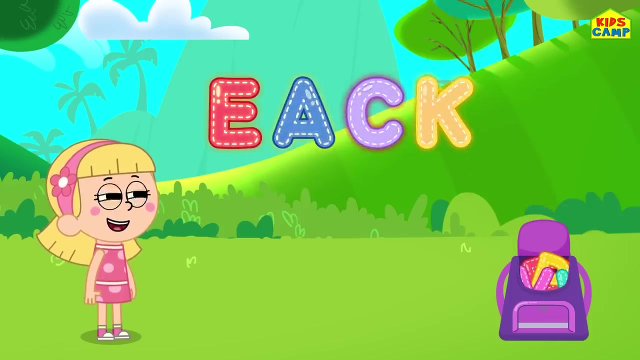 P, P, L and E. That's right, We got it right. kids, It's an apple. Woohoo, We got the first word correctly. What's next? Hmm, I wonder What could this be? The letter E, A, C and K? Hmm, This looks. 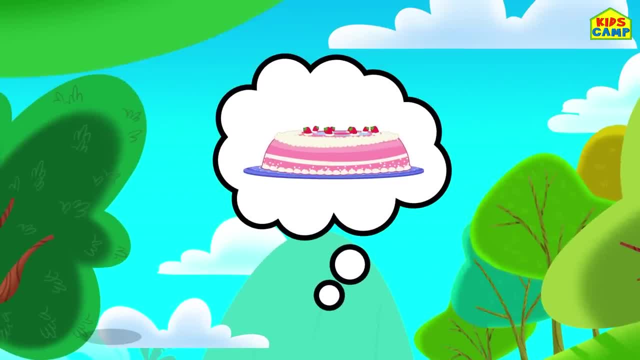 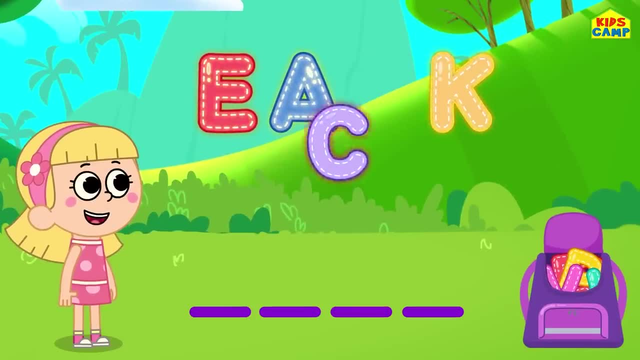 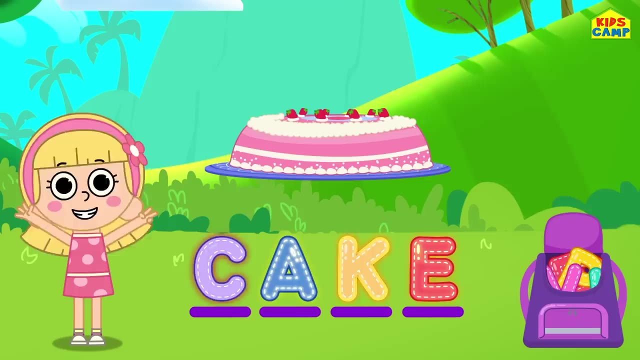 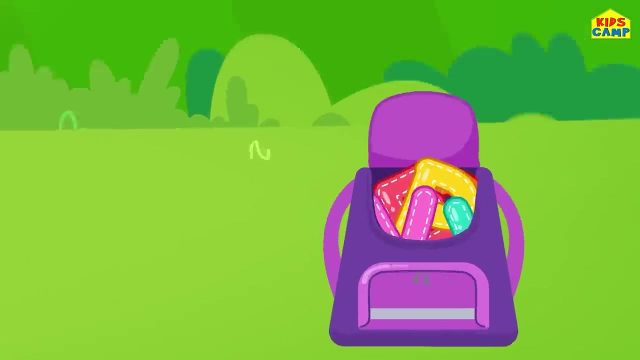 familiar. That's right, It's a cake. Yes, yes, I know this one. It starts with the letter C, A, K and E. Yay, We did it again. What's the next word? Any guesses? Hmm, We have the. 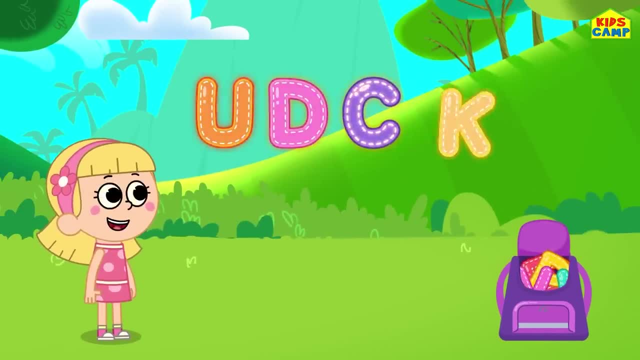 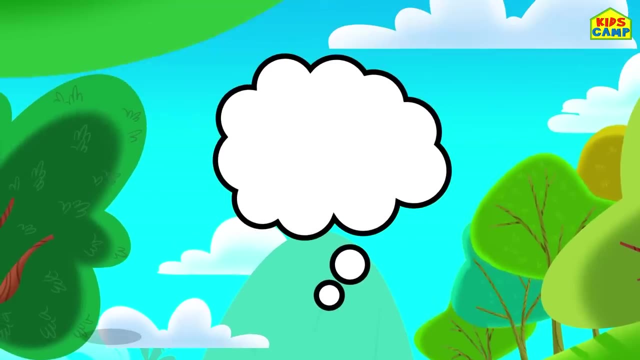 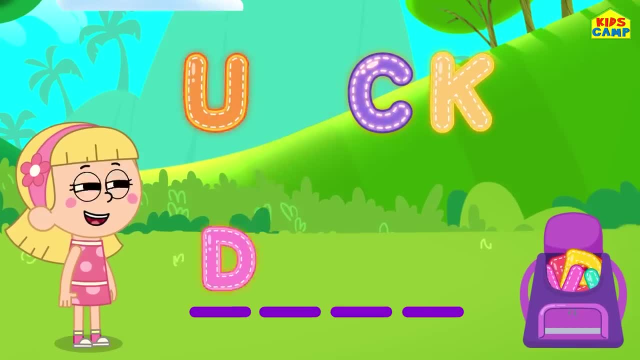 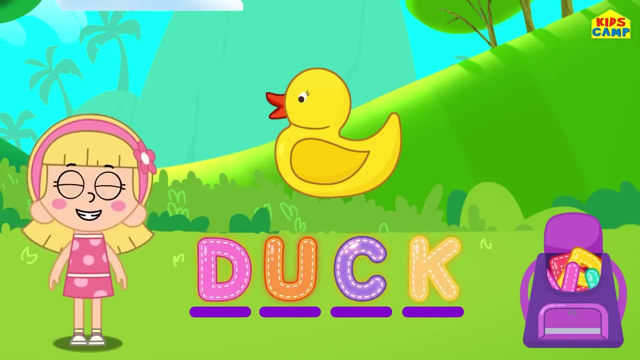 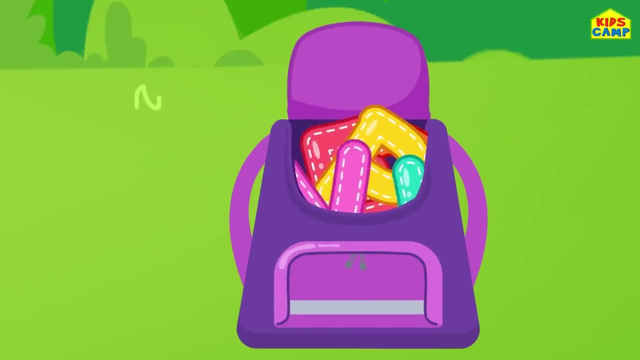 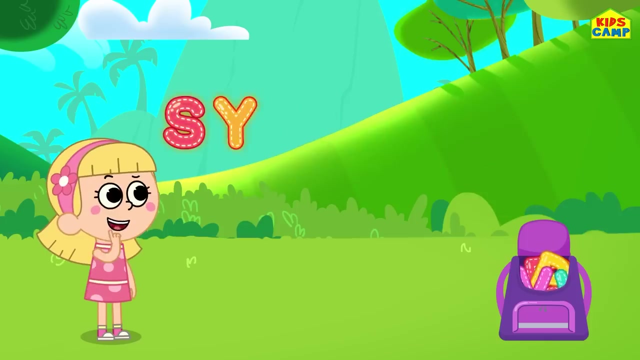 It starts with the letter D, U, C and K. Duck, Woohoo. Alright, let's go to the next one. What does my bag of letters have now? The letters S, Y, R, A, C, O and N. 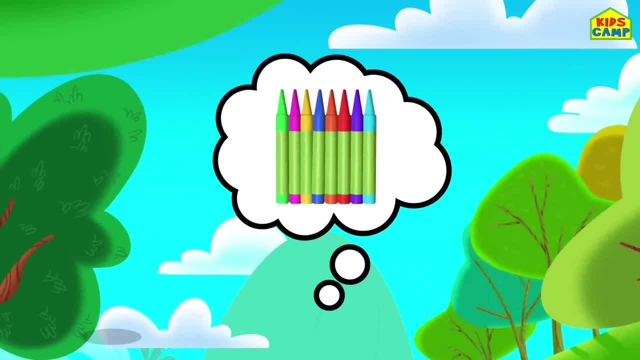 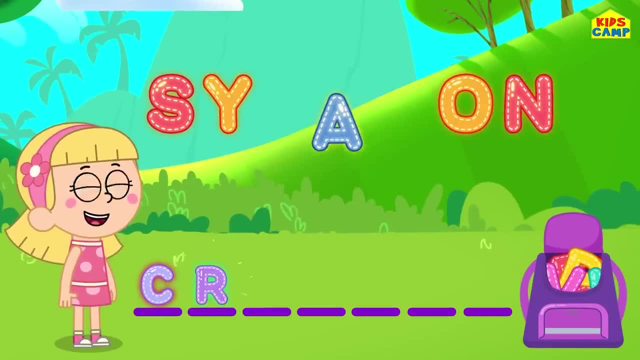 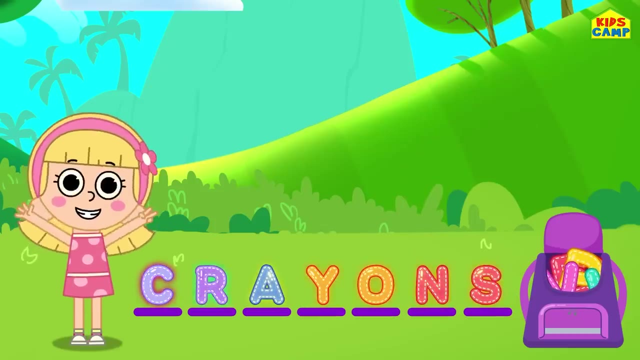 What could this be? These are crayons. That's right, kids, I love crayons. It starts with the letter C: R A Y O N S Crayons. That's right, Woohoo. 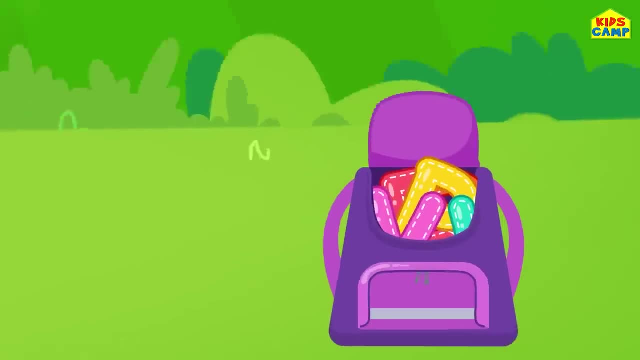 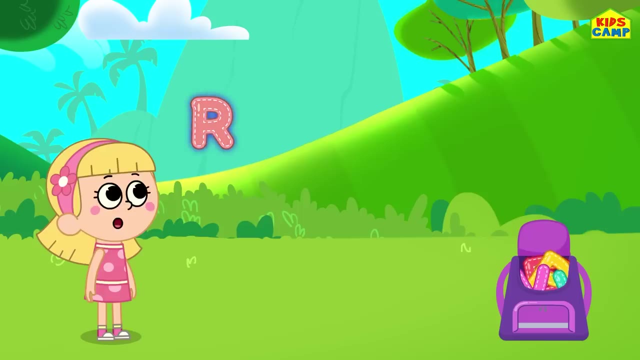 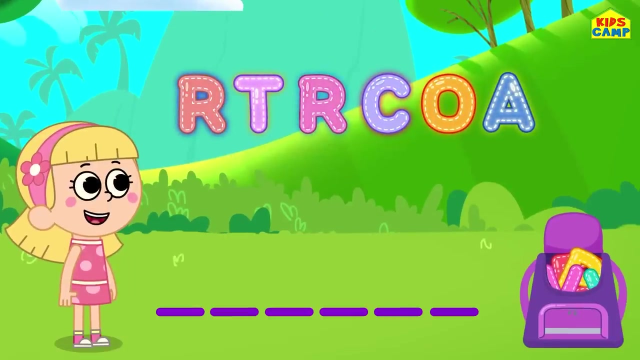 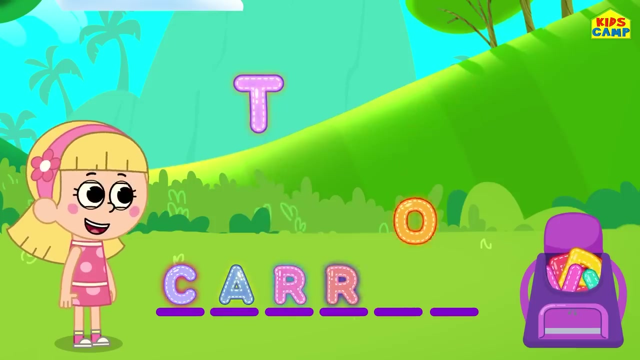 One more. What will come out of the bag of letters? What letters? R, T, R, C, O, A? Hmm, what could this be? It's a carrot, That's right. That starts with the letters C, A, R, R, O and T. 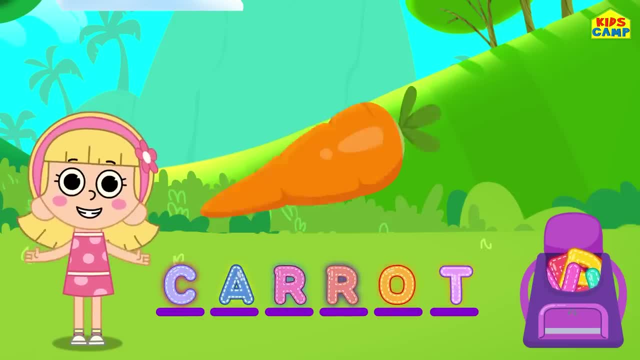 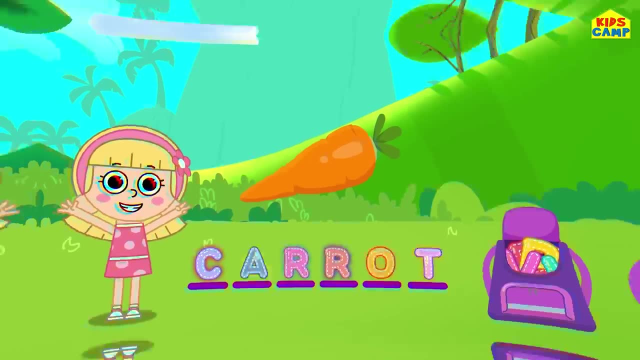 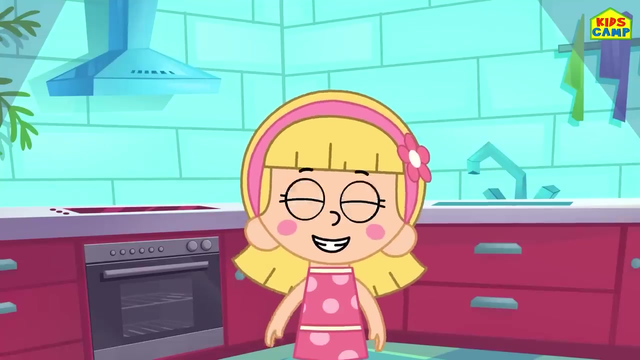 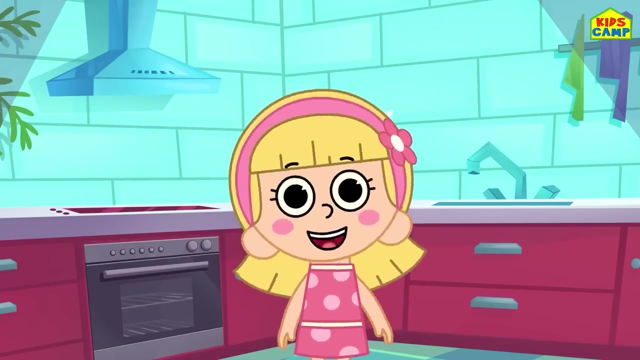 That's right, Carrot. Woohoo. Good job, kids. Well done. This was so much fun. Bye-bye, Hi friends, I'm Ellie And I'm making some yummy treats for Eva. Okay, But first we have to sort them according to their sizes. 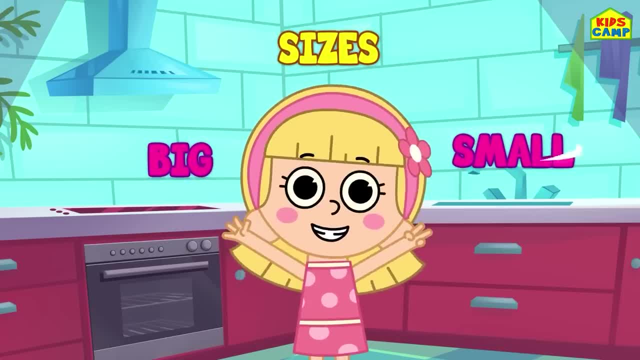 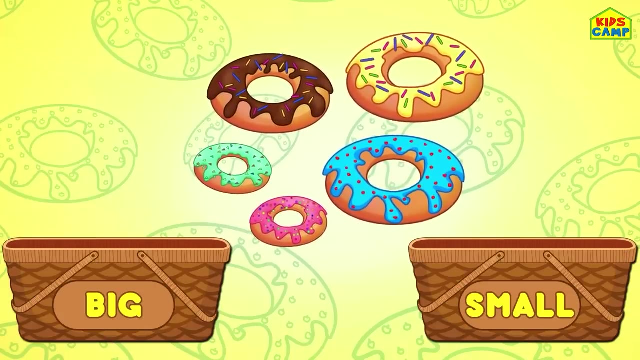 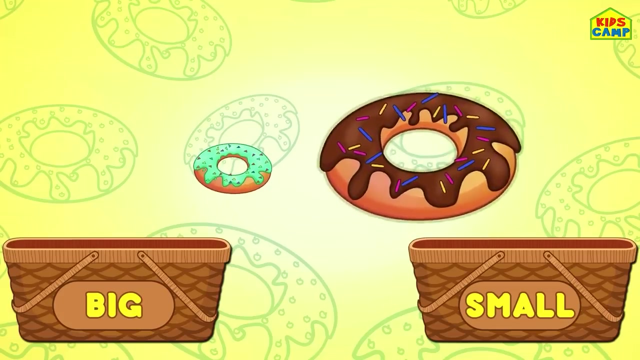 Ready, Big or small? Will you help me, friends? Yes, Then let's get started Right away. Wow Donuts- Yummy, I love them. Let's sort them according to their sizes. This chocolate donut looks bigger than this one. 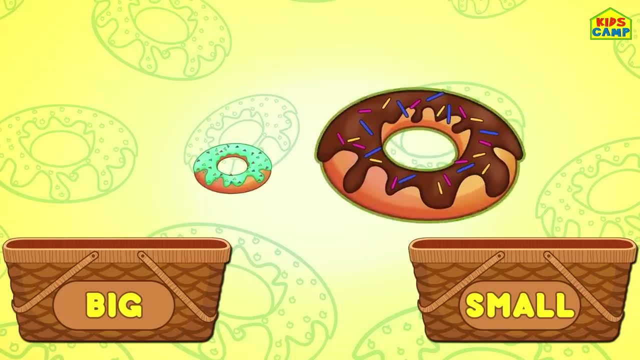 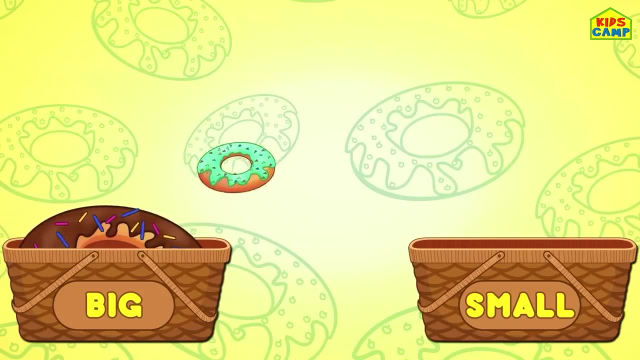 That's right. The bigger donut goes into the basket labeled big, That's right. And the small donut goes into the basket labeled small. Yay, Hmm, let's compare these two. The pink donut is smaller than the yellow donut. 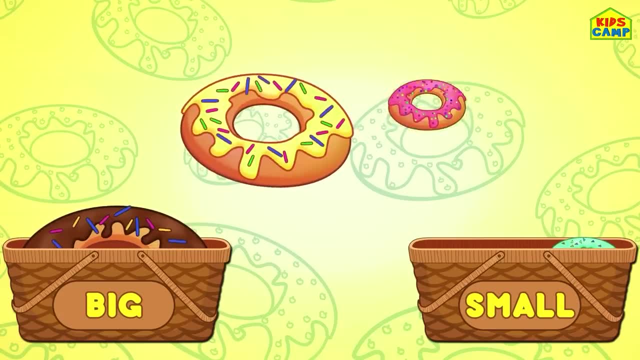 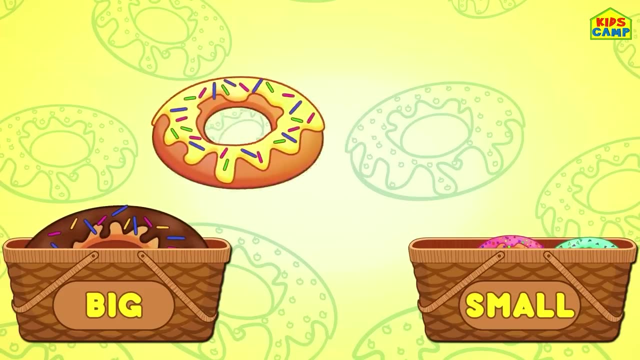 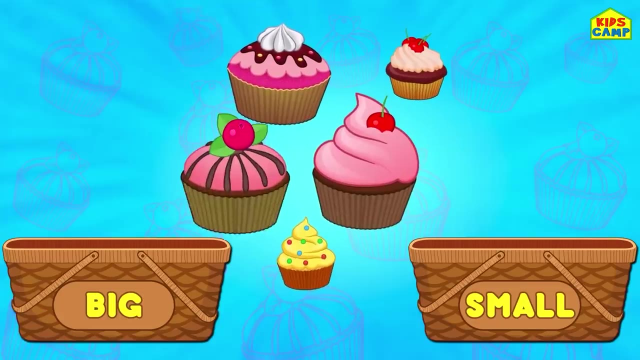 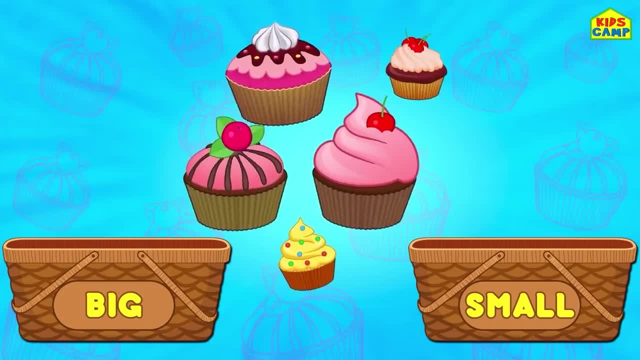 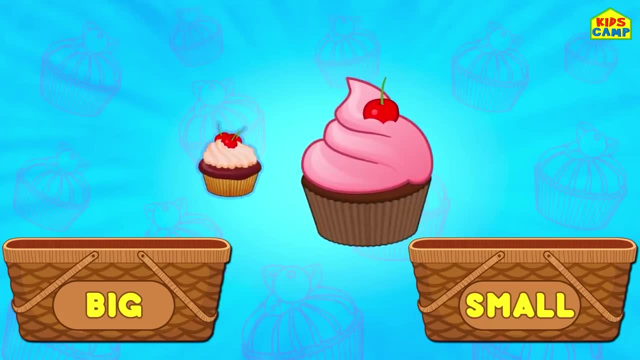 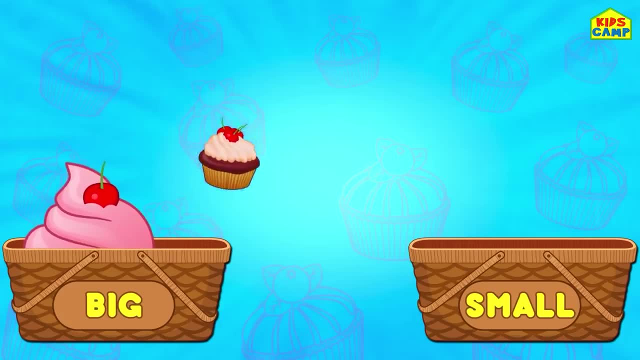 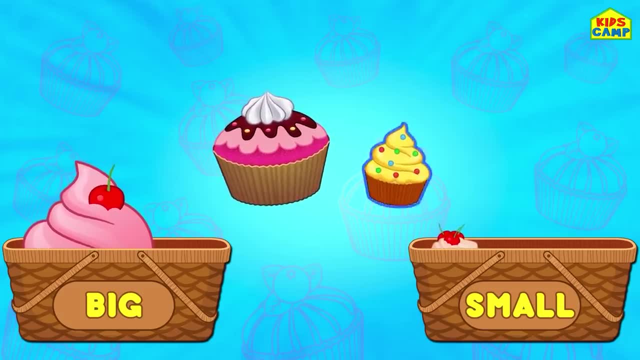 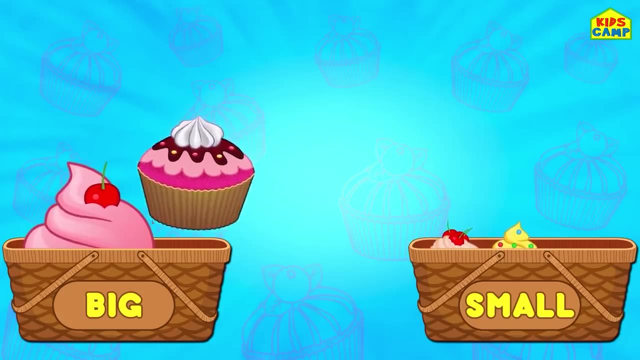 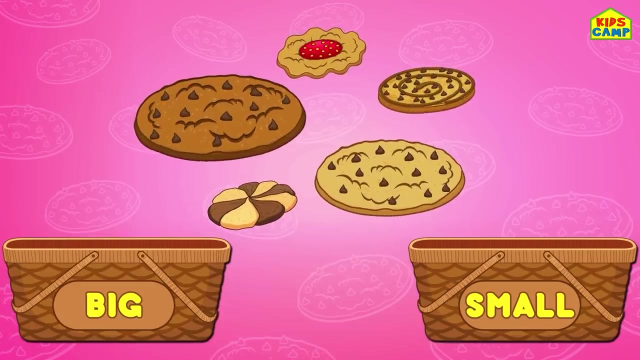 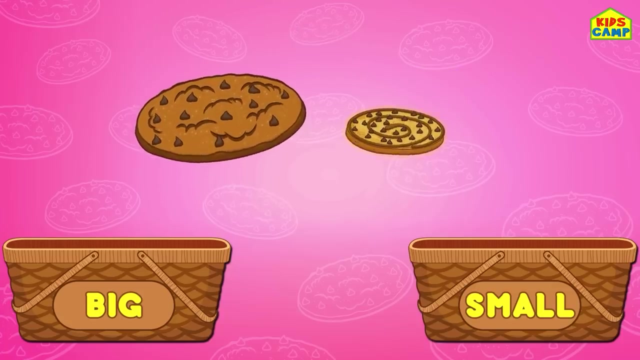 Yay, Wow, Ooh, More cupcakes. Let's compare these: The big goes into the small basket and the big one goes into the big basket. Yay, What's next? Cookies- Wow, Let's sort the bigger cookies from the smaller ones. 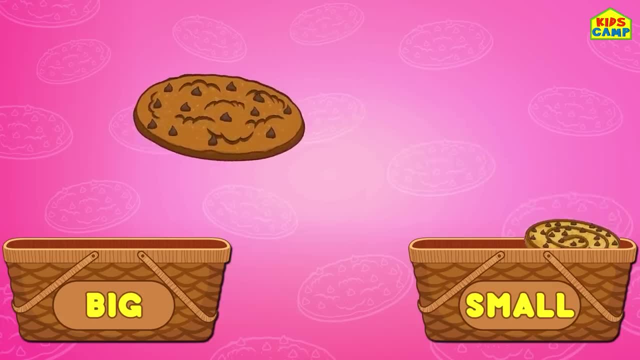 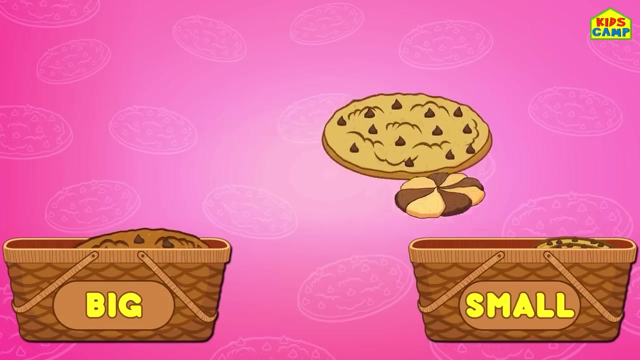 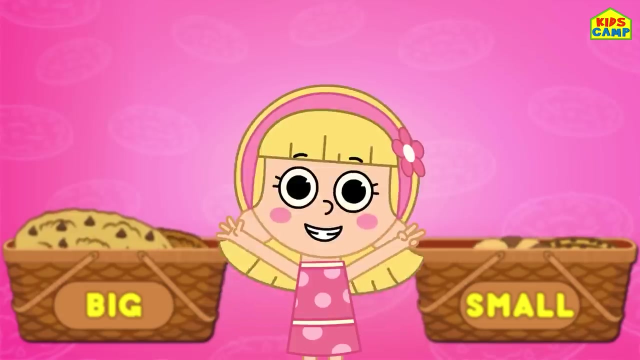 The smaller cookie goes into the small basket and the bigger cookie goes into the big basket. That's right. Yay, This smaller cookie goes into the small basket and this big one goes into the big basket. Wow, We sorted all these treats according to their sizes. 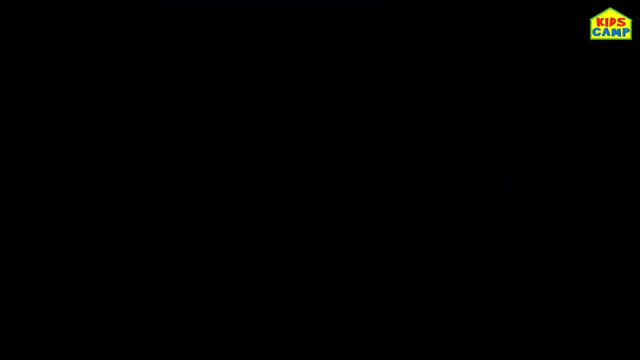 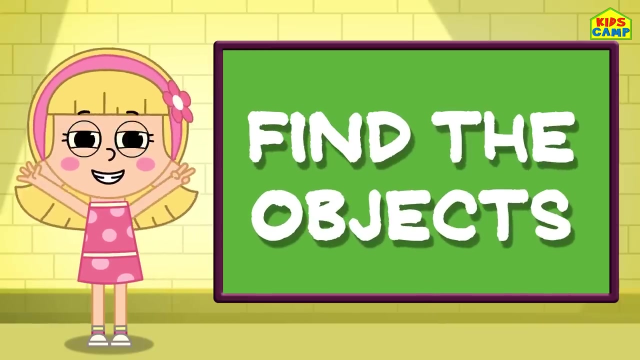 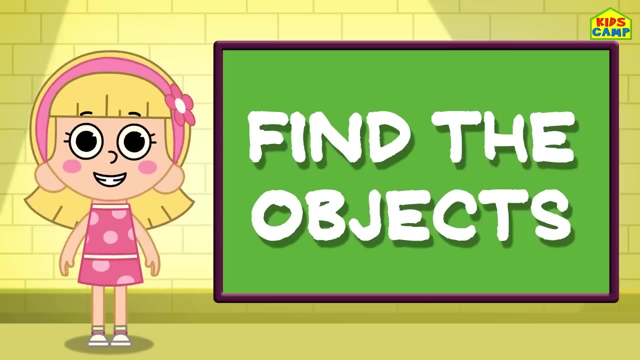 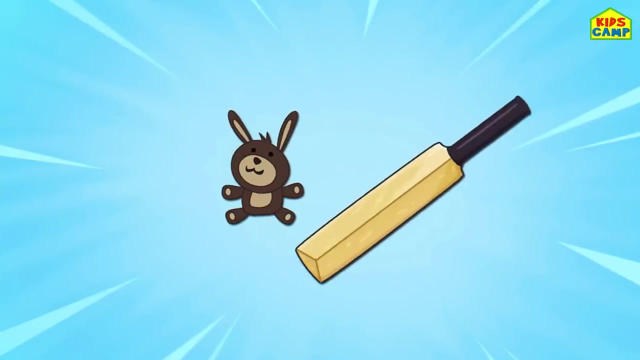 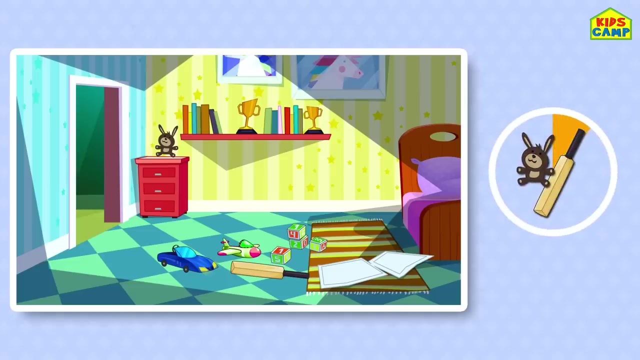 Good job, everyone. Let's find the objects. Yay, That's right, Let's get started. Woohoo, Let's find the bat and the teddy. Ready, Here we go. Can you find the bat and the teddy? 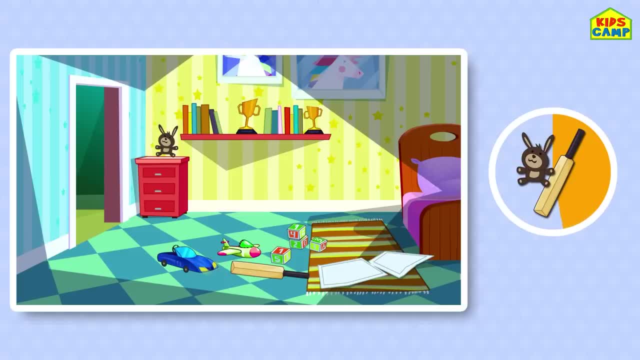 Where could it be? Can you see the bat and the teddy anywhere? Keep looking Time's up. Aha, There it is. Yay, We found the bat and the teddy. Find the flowers and the book. Let's look for it. 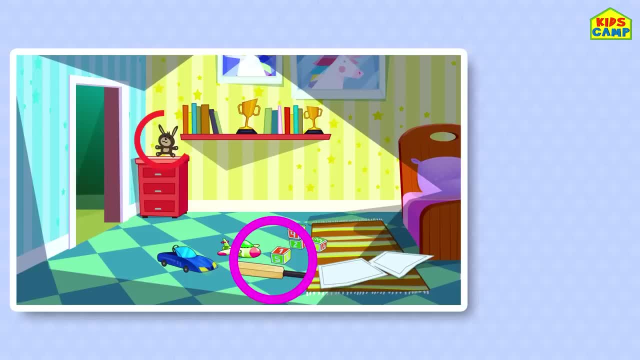 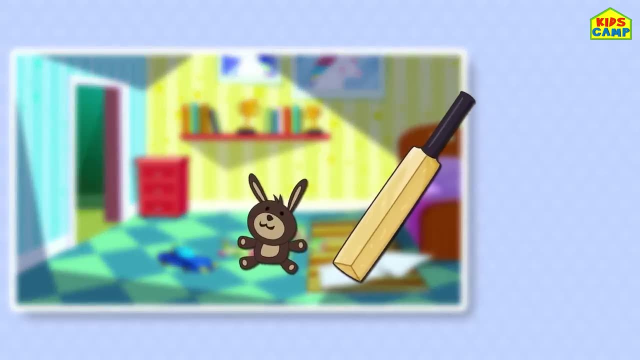 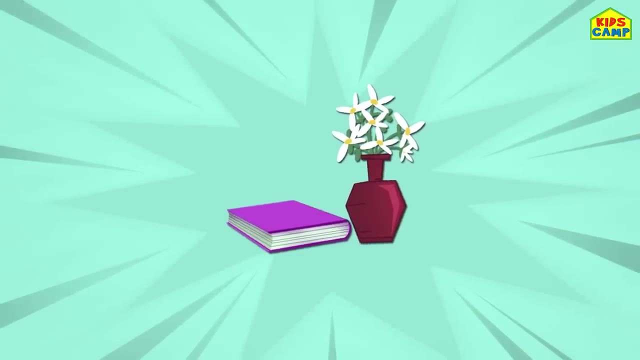 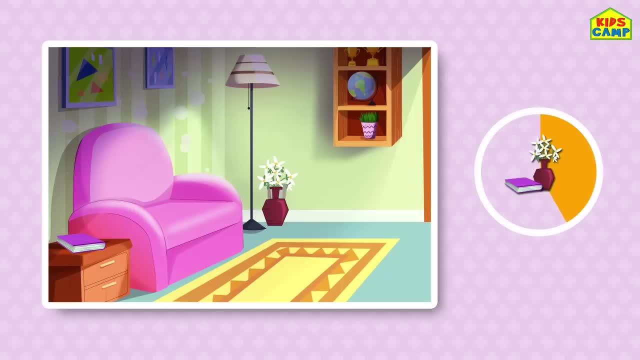 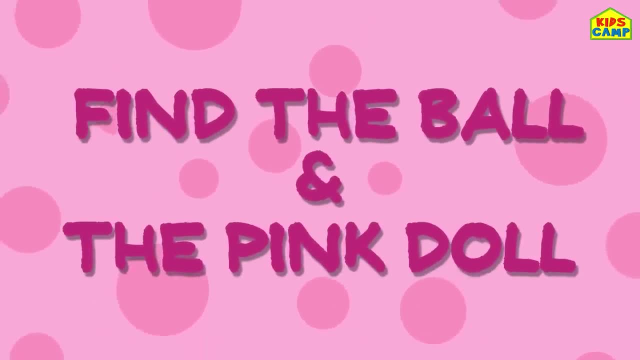 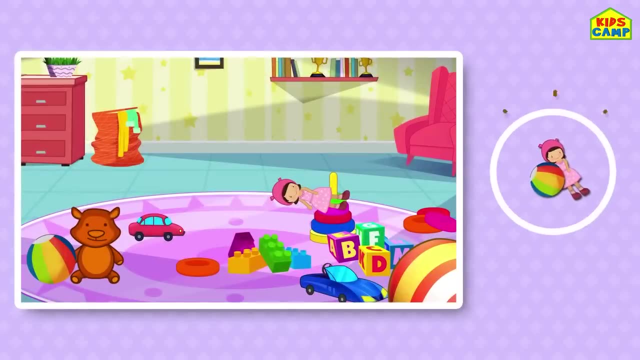 Yes, This is a gorgeous flower, Ready. Can you spot the doll and the ball? Where could it be? Where could it be? Keep looking Our time's almost up, Time's up. Did you find it? Yes, There it is. 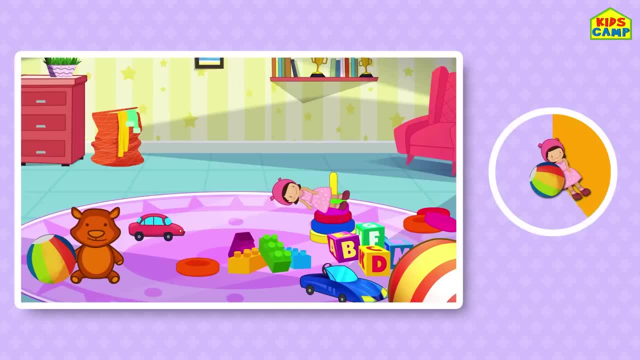 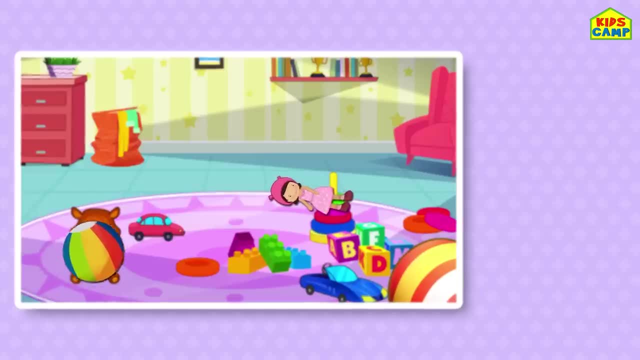 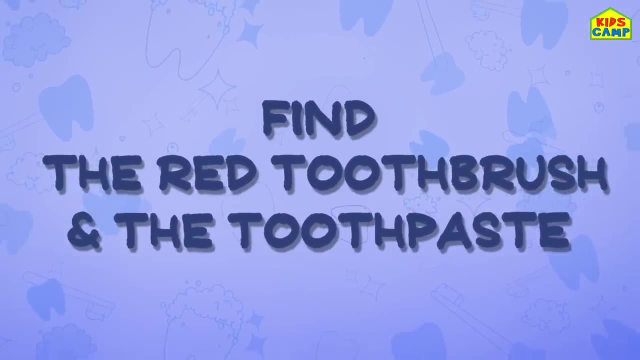 Yay, Yay, Yay, Yay. We found the ball and the pink doll. Yay, Find the red toothbrush and the toothpaste. Ready kids Look for it. Can you spot the red toothbrush and the toothpaste? 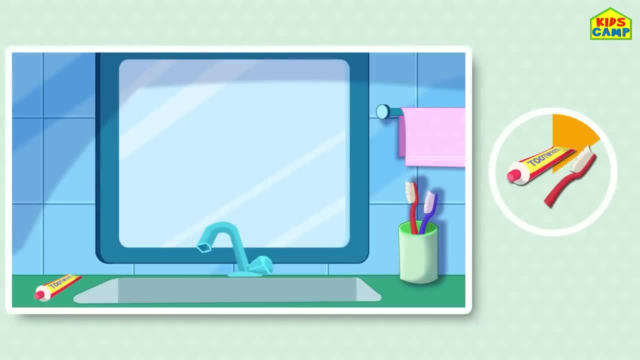 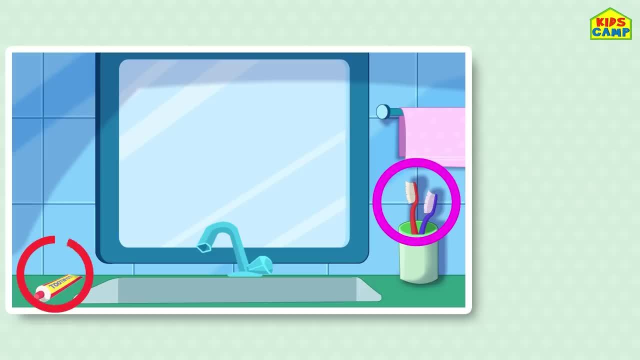 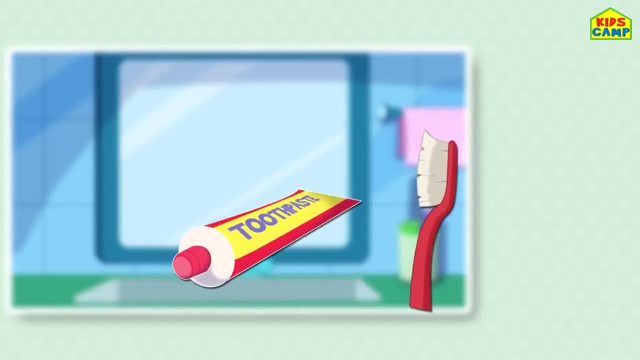 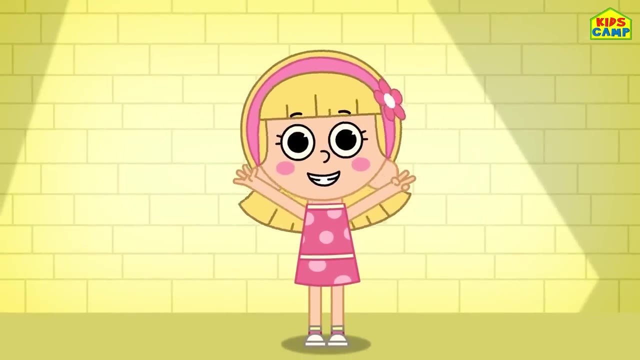 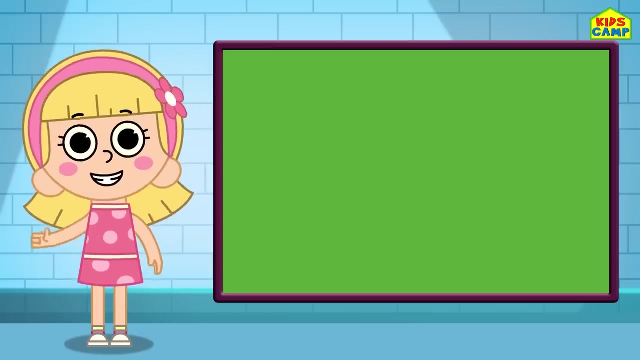 Time's up. REAM Of LOVE. You did find it There. it is The red toothbrush and the toothpaste. This was so much fun, kids. We found all the objects. See you soon, Hi kids, I am elly. 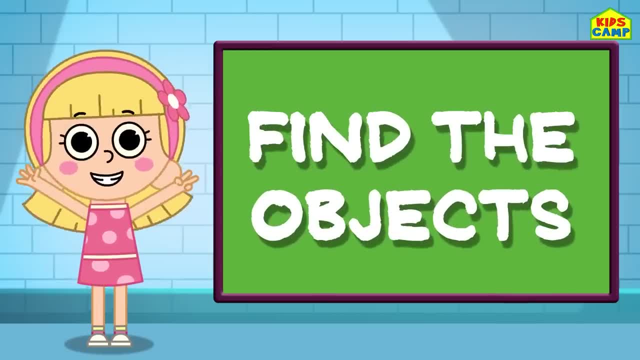 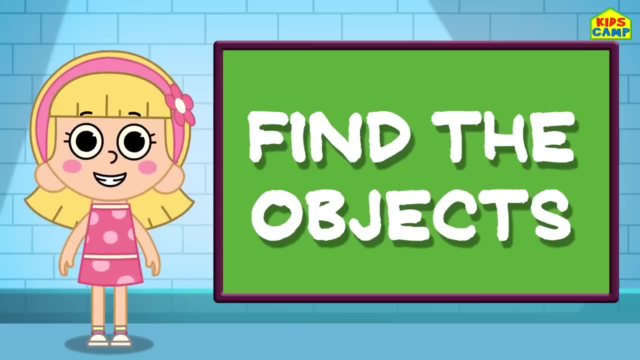 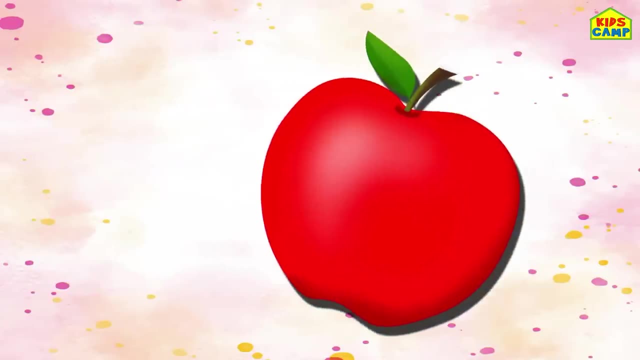 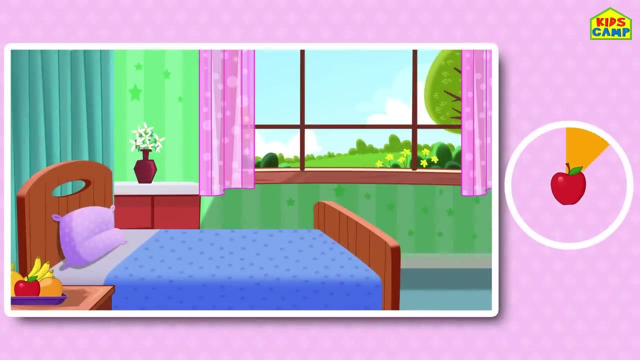 And today we are going to play Find the Objects. Yay, Ready, Let's get started. Find the apple. Hmm, that's easy, Let's look for the apple. Where's the apple? Is it on the bed? No, 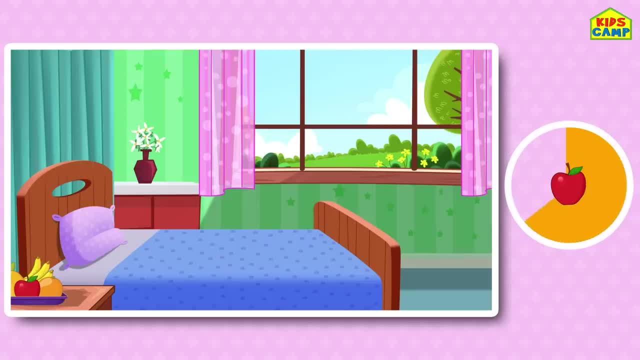 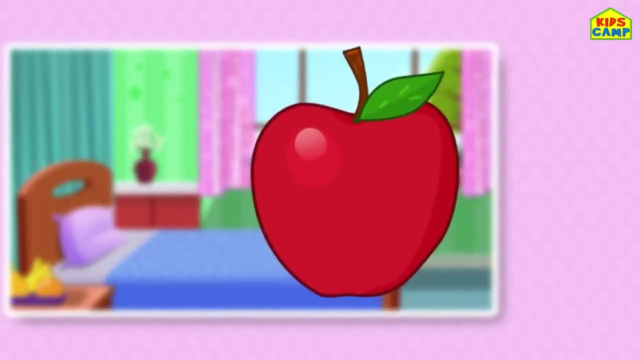 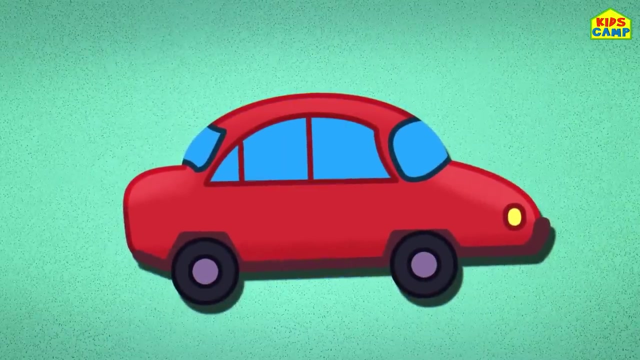 Where is it? Keep looking Time's up. Did you spot the apple? Yes, there it is. Good job, kids. We found it. Find my car. We have to look for my red car. Can you spot it? Hmm, where is it? 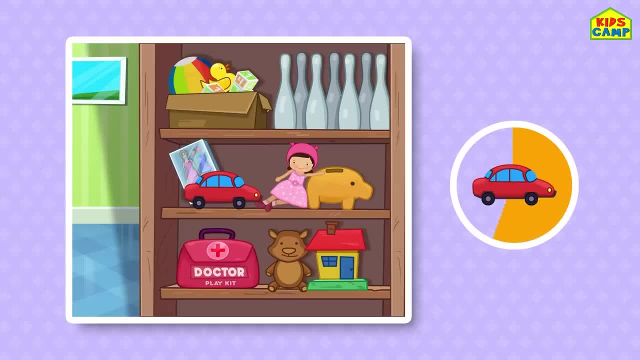 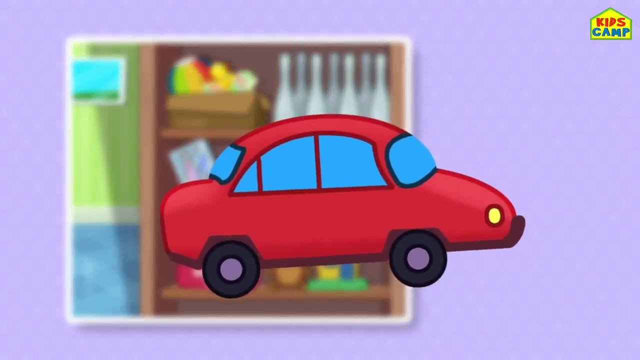 There's so many toys. There's so many toys on the shelf. Uh-oh, time's up. Did you spot it? Yes, that's right, That's where it is. That's my red car Vroom vroom. 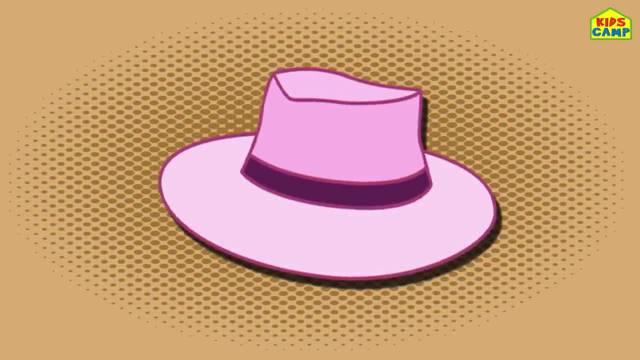 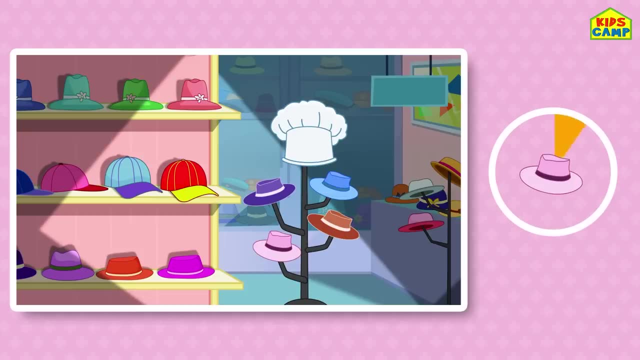 Find my hat, My pink-colored hat. Can you look for my hat? Oh my, there are so many hats. Can you spot the right one? Come on, Time's up? Yes, that's the one. Good job, kids. 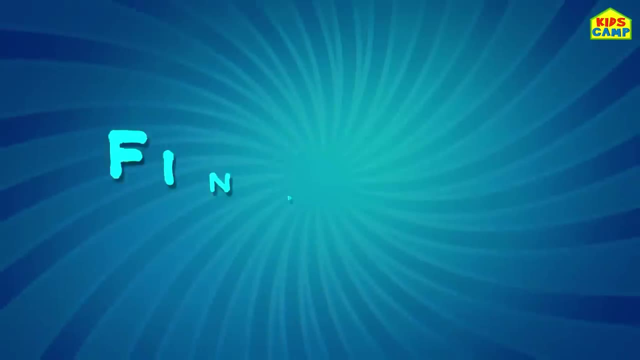 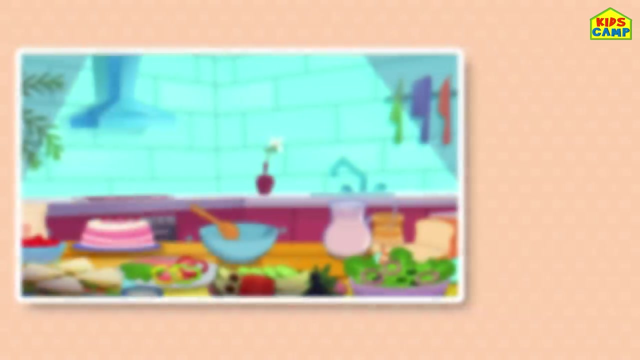 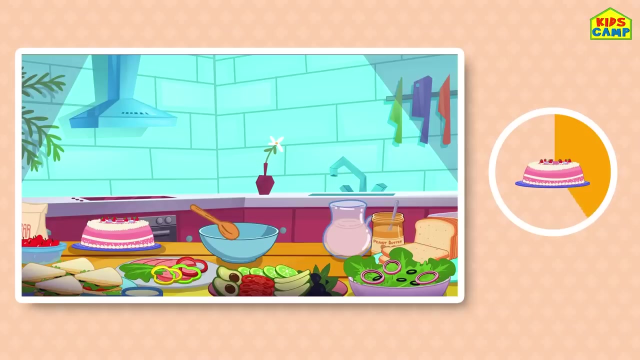 You found it. Woohoo, Find the cake. Hmm, delicious, Hmm delicious, Hmm delicious. Let's look for the cake. Wow, there is so much food on the table. Can you look for the cake? Where's the cake? 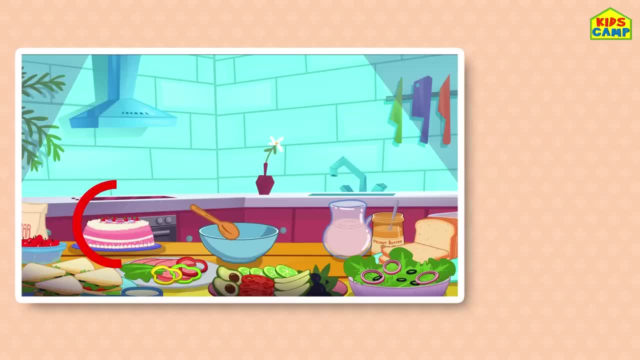 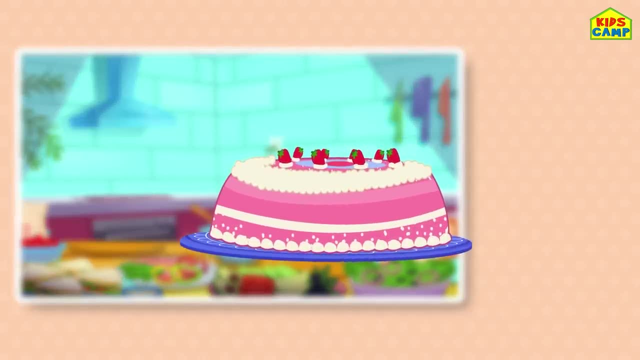 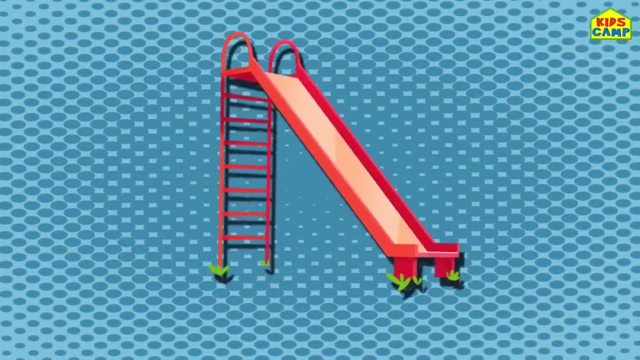 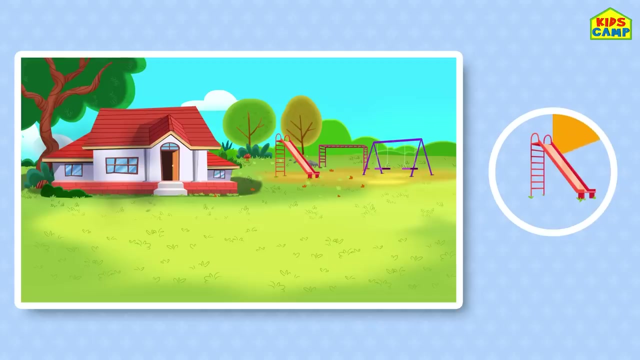 Time's up. That's right, There it is. You found the cake Looks delicious. Find the slide. Wow, I love the slides. Where's the slide? Can you spot it? Keep looking. Time's almost up. Uh oh, time's up. 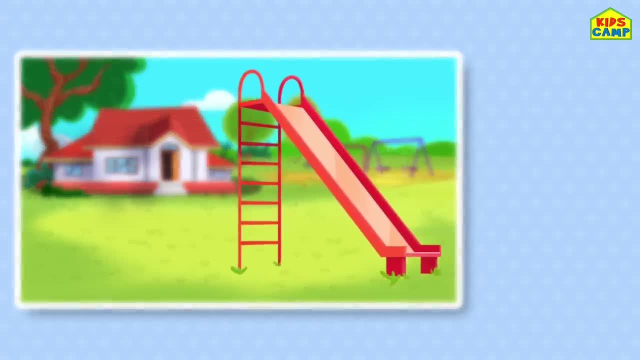 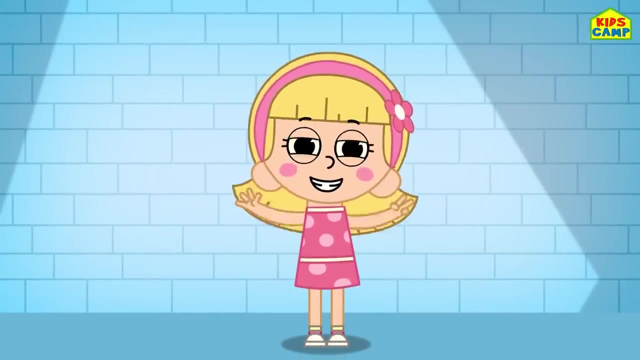 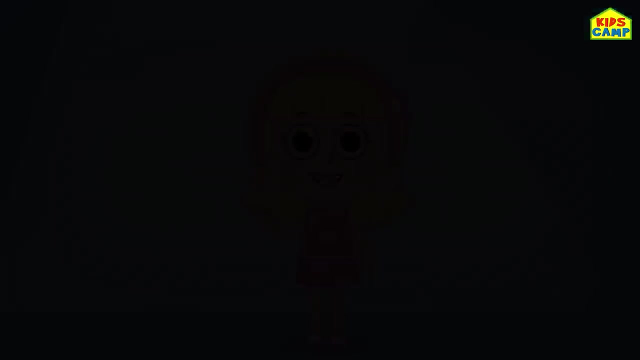 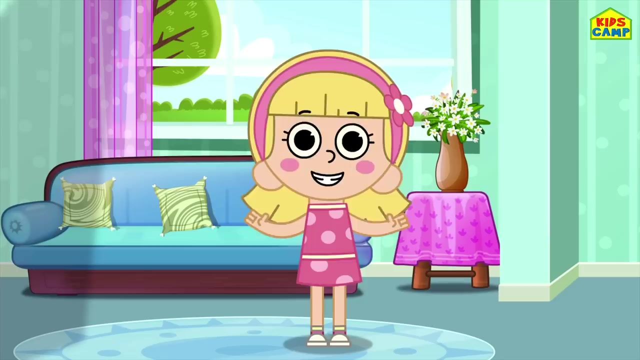 Yes, that's right, We found the slide. the slide. Woohoo. Good job. We had so much fun finding the objects. See you soon. Bye-bye, Hi kids, I'm Ellie And today we are going to play with puzzles. Don't we all love puzzles? 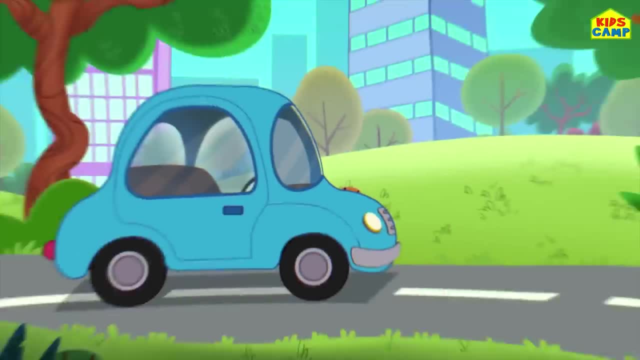 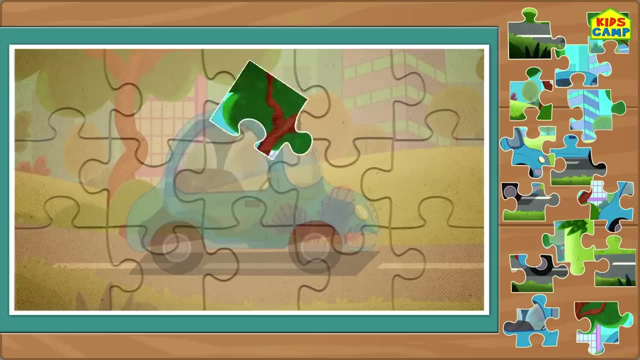 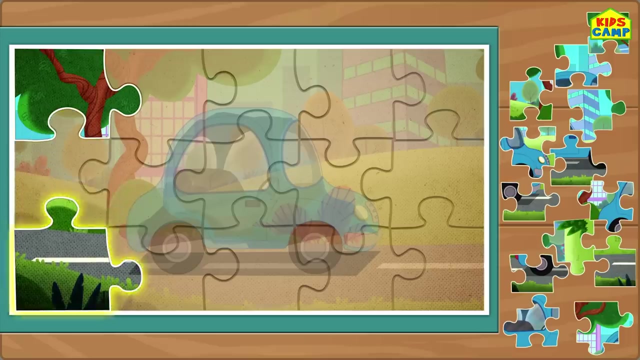 That's right, Let's start. Oh, that's a car. Let's put all the pieces together. Let's start with the corners. That's right, It goes right there. That's right. Perfect, We got all the four corners. 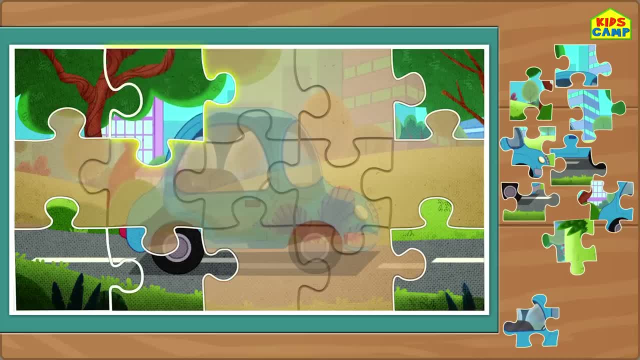 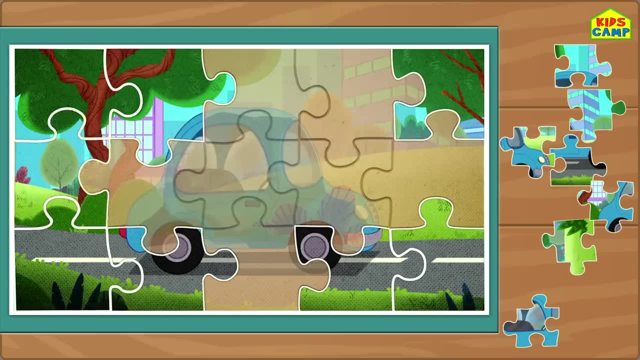 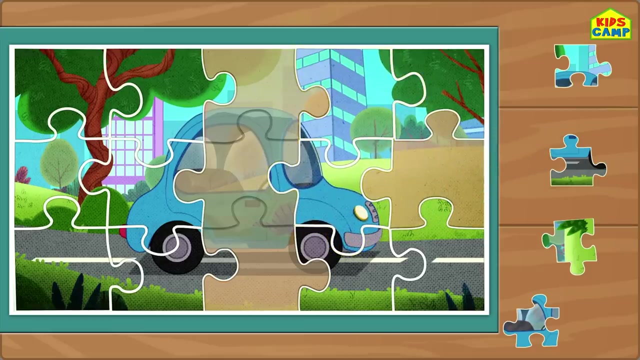 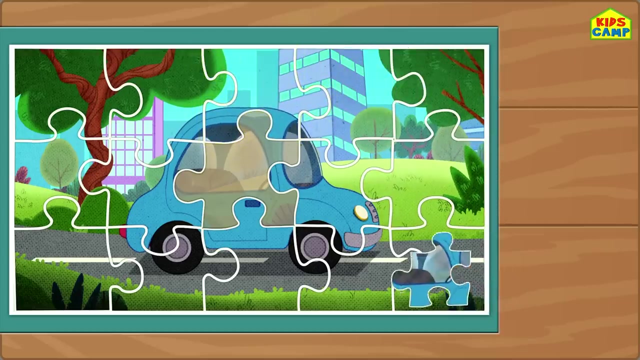 No, that goes up there, That's right. Another wheel, Perfect. Great, Uh-oh, That's right. Wow, This is so much fun. I like puzzles, Don't you? No? no, That doesn't seem right Now. it is Perfect. And the last piece? Woohoo, We did. 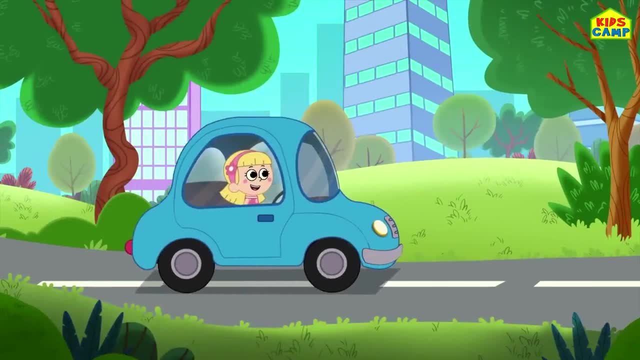 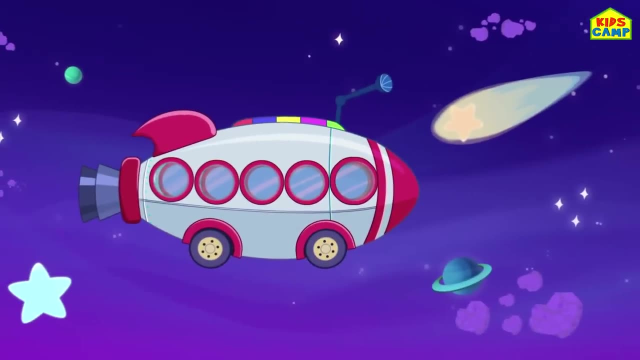 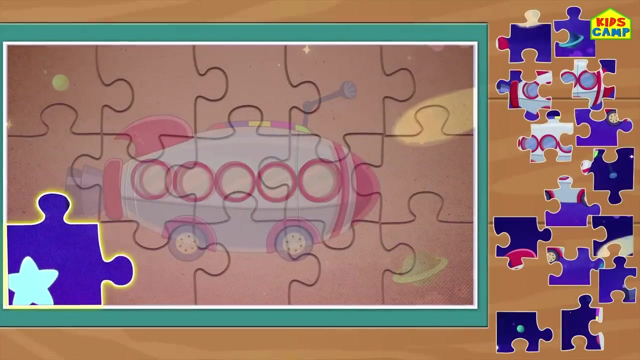 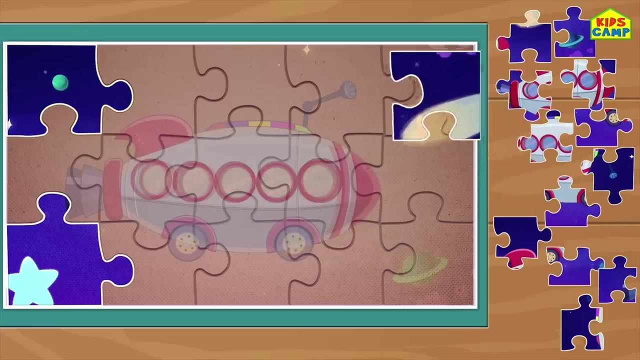 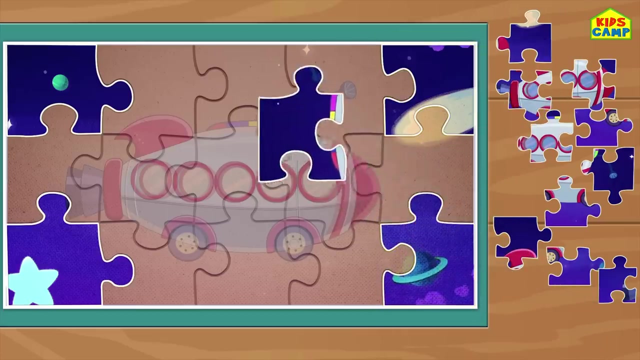 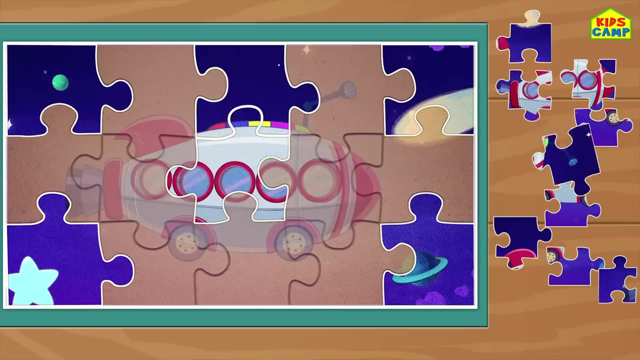 it, kids. There goes my car Vroom, vroom, And now we have a spaceship. Let's start with the corners. That's right, Yay, We got all the four corners. Uh-oh, Yes, Wow, The windows. Perfect, Woohoo. 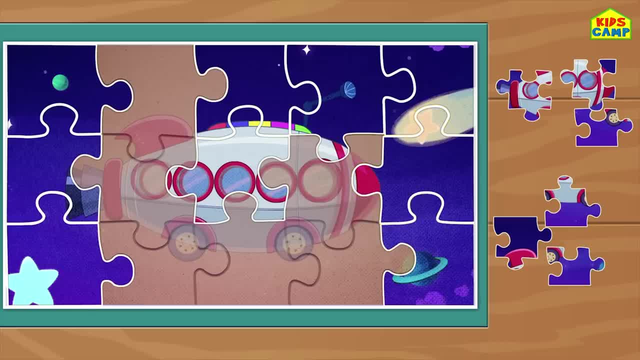 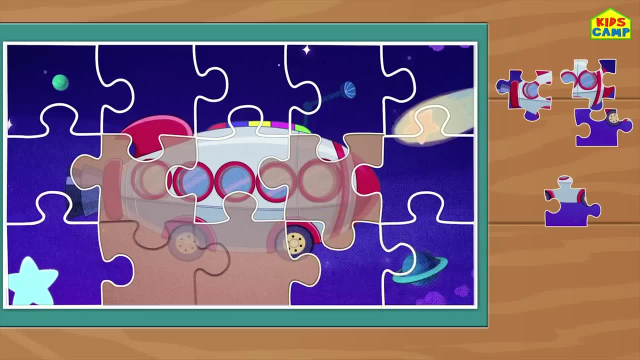 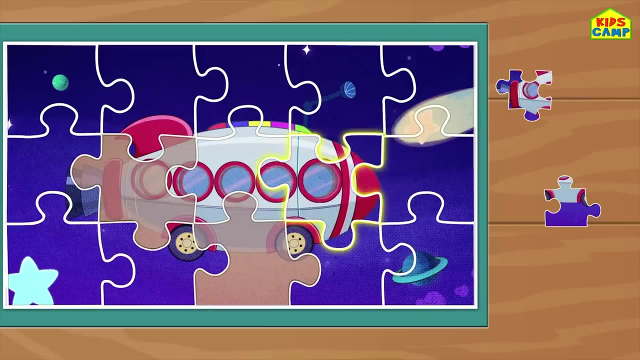 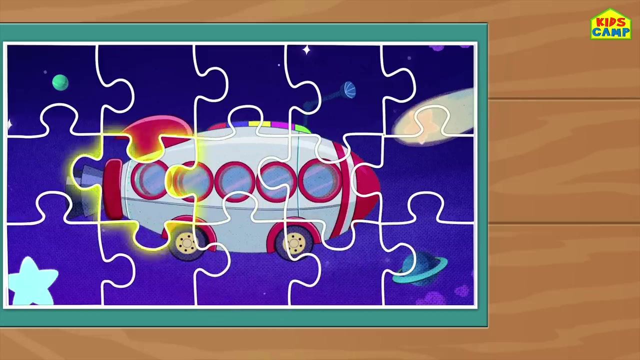 That's right, We got all the four corners. Uh-oh, Yes, Wow, The windows Perfect. Woohoo, that's right, we're almost done. just a few more to go perfect. a few more pieces, wow, this looks so good. and the last piece: our spaceship is completed and 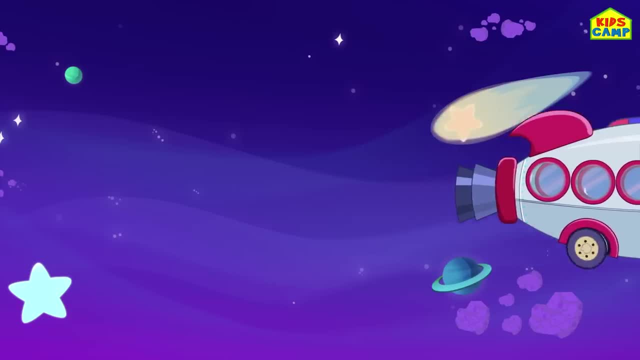 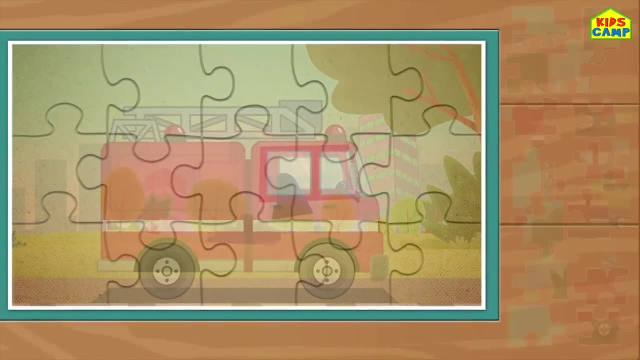 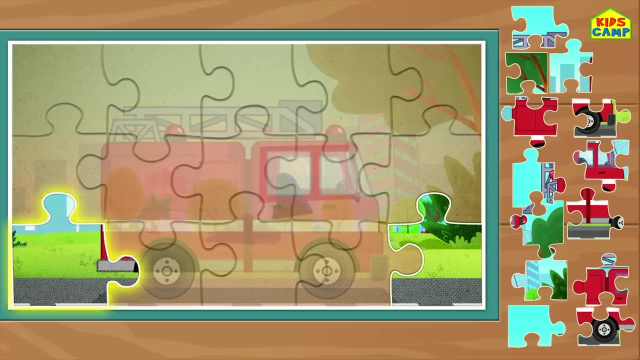 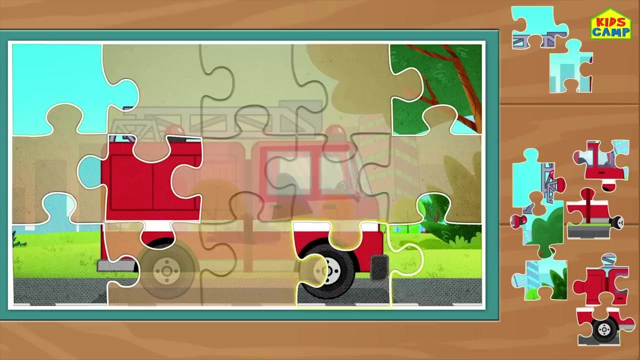 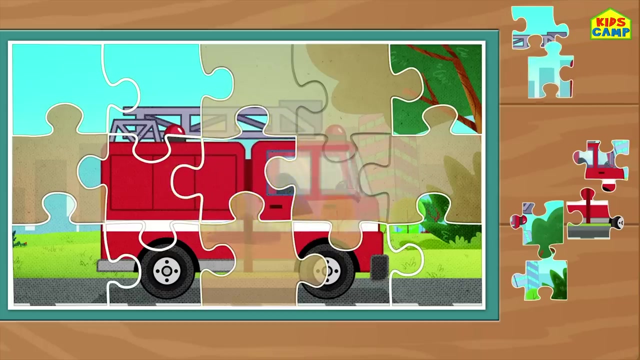 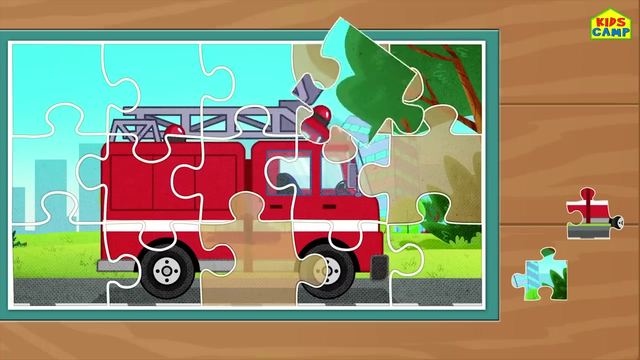 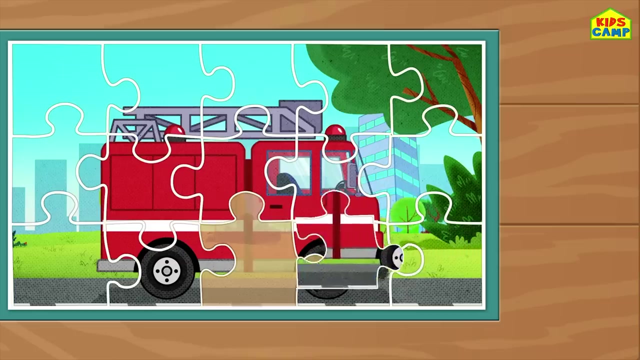 here I go, a fire truck once again. let's start with the four corners. good job, kids, we're learning. Oh, the wheels and the second wheel. Oh, the centerpiece. Wow, we almost got it. a few more pieces that fits correctly. oh, we gotta spin that around. perfect, and the last piece. we did it. 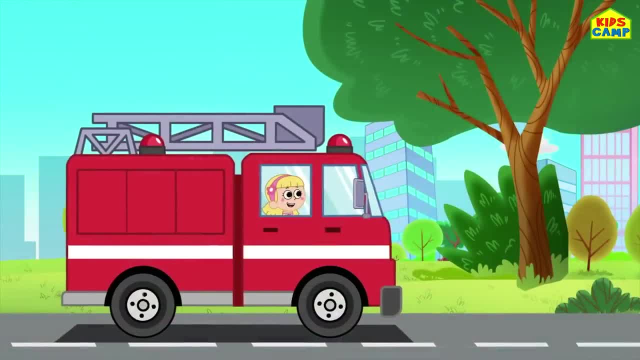 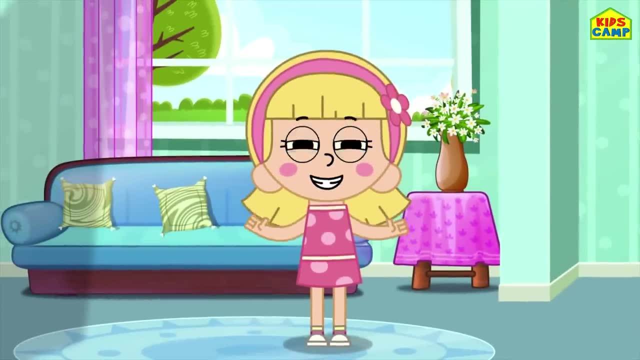 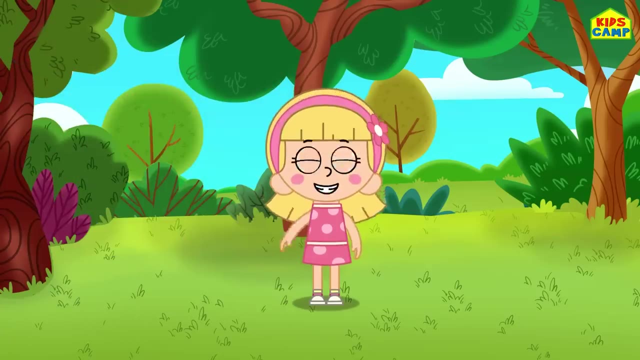 Our fire truck is ready to go. wow, yay, this was so much fun solving puzzles. see you soon. hi, I'm Ellie and we're going to play a fun game. we have to spot the tобр 북한 tent to find a car misses. oh yeah, then go. I want to am all I know. I wanted to take you to j estos. 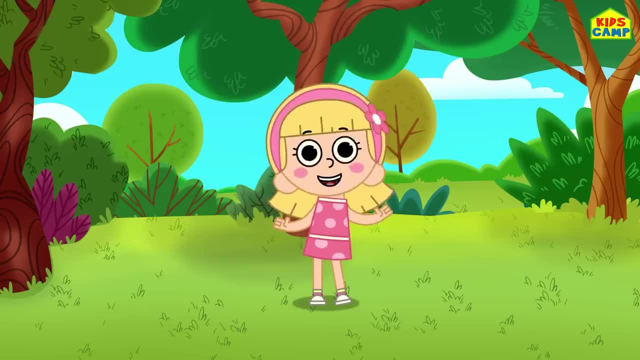 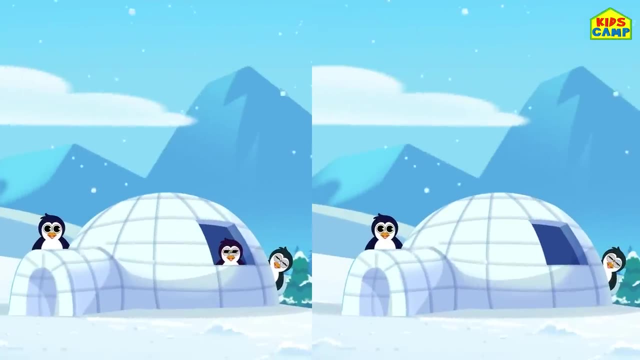 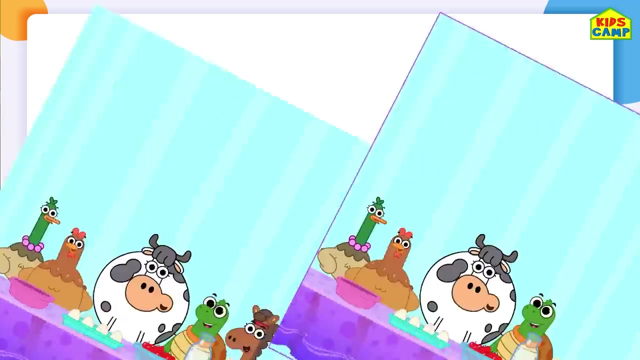 fun game and I just want to remember to do more things. over and over and over it again. We have to spot the differences and this is going to be such a fun game. ready, Let's start. Can you spot the difference? That's right, Can you spot the difference? 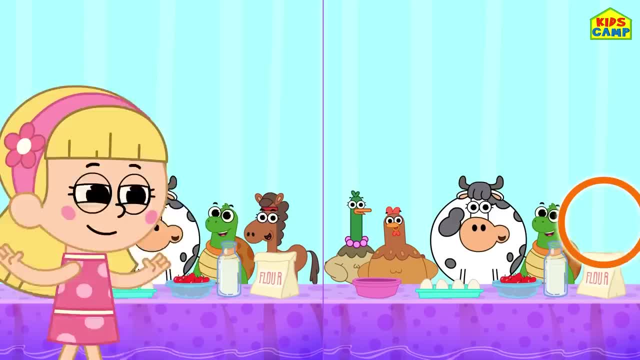 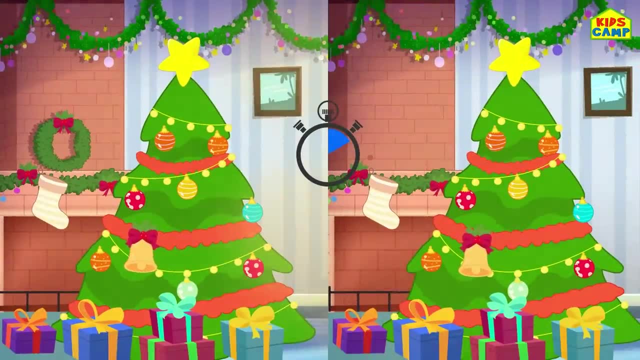 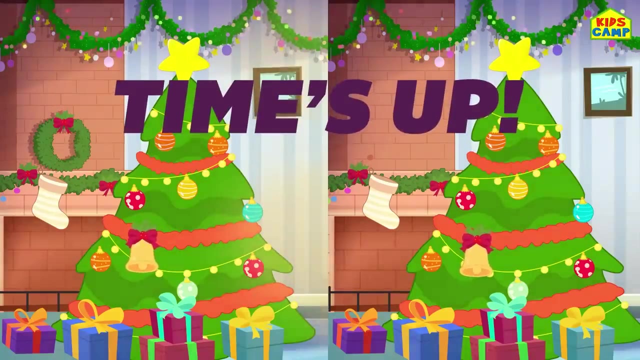 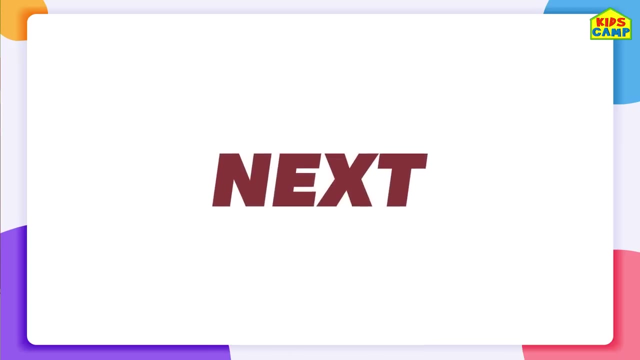 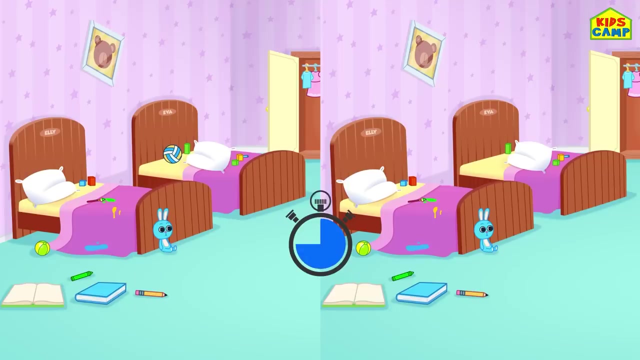 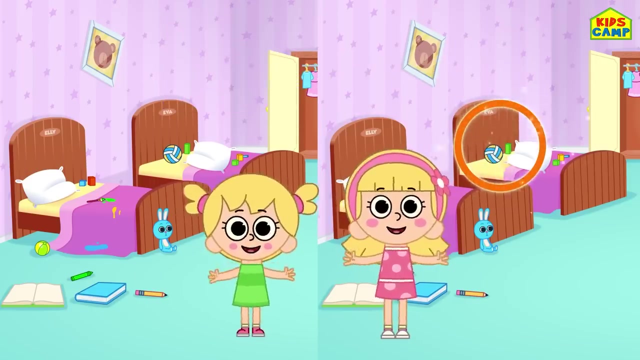 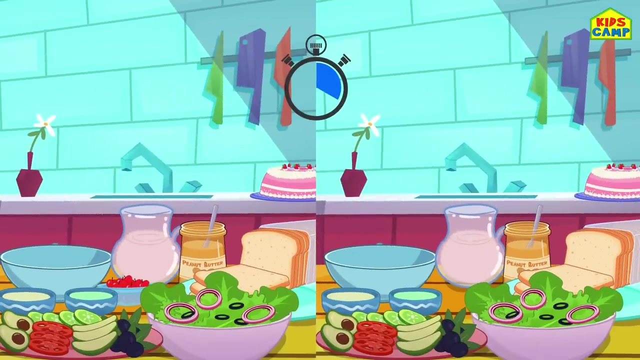 Time's up, That's right. Can you spot the difference? Keep looking Time's up, That's right. Next one: Can you spot the difference? Can you spot the difference? Keep trying Time's up, That's right. Next one: Can you spot the difference? Can you spot the difference? 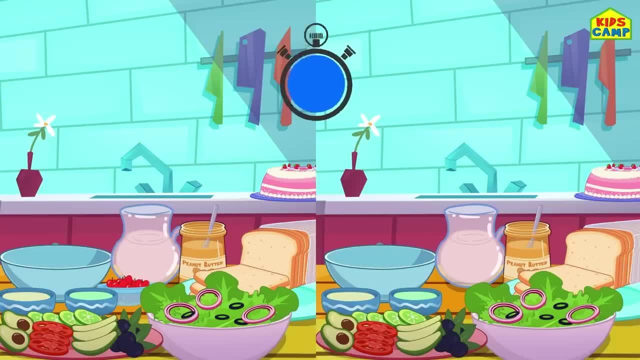 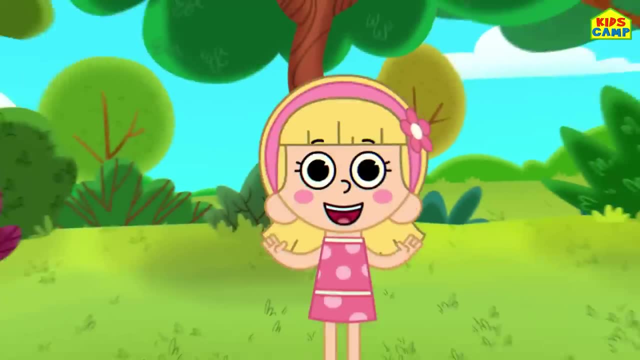 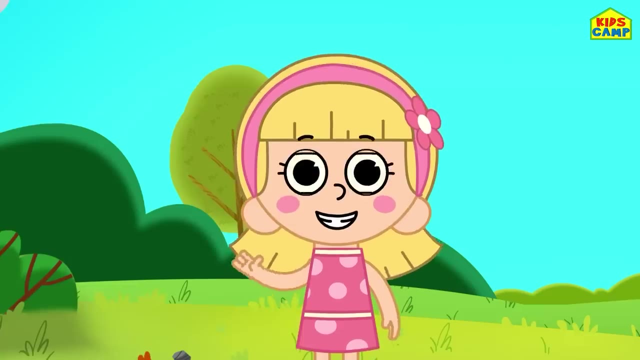 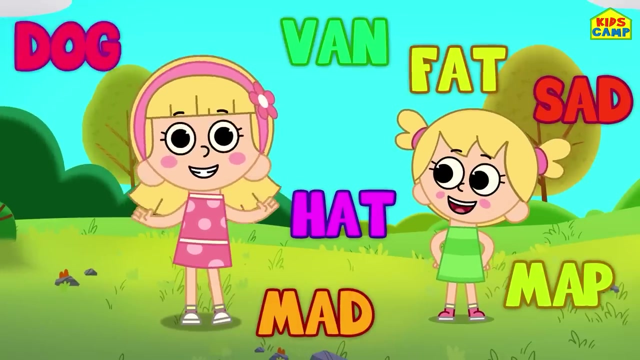 Keep trying Time's up. Woohoo, You guys did it. Yay, This was so much fun. Bye, Bye, Hi friends, I'm Ellie and I've learnt some new words. That's right. Do you also want to learn with me? Yes, Let's get started. 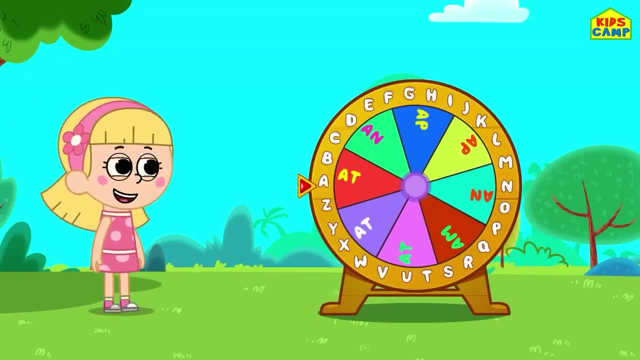 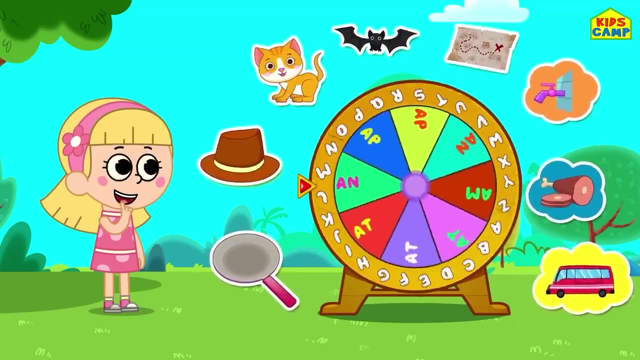 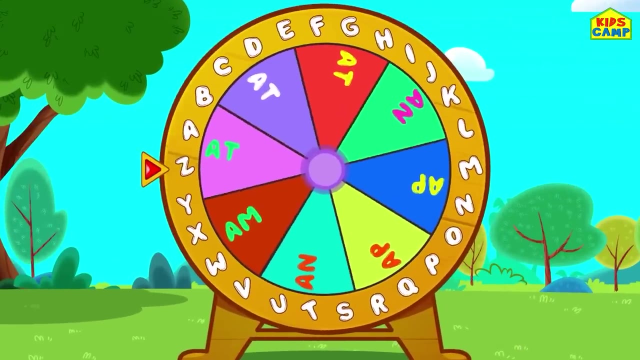 This is the word wheel. We have to spin the wheel and match the letter to make the correct word, And we also have clues. This is going to be so much fun. Let's get started. Let's spin the wheel. Let's spin the wheel. Woohoo, Is that a word? 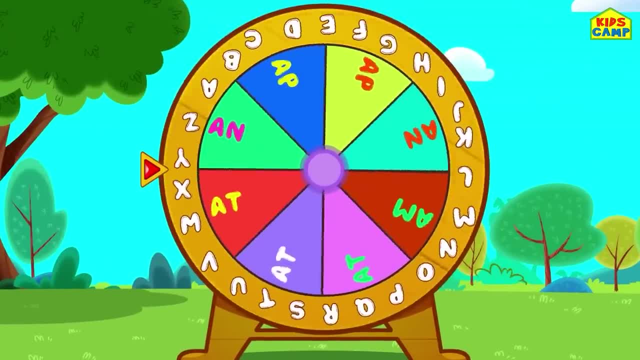 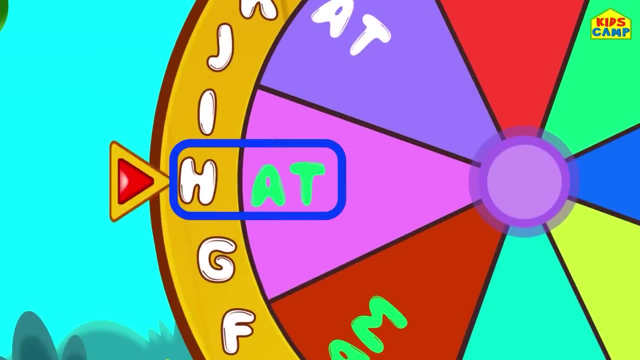 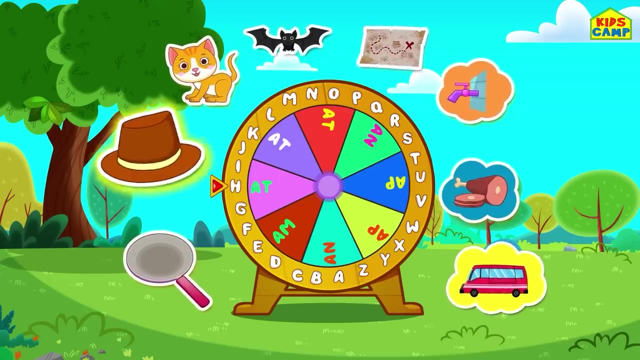 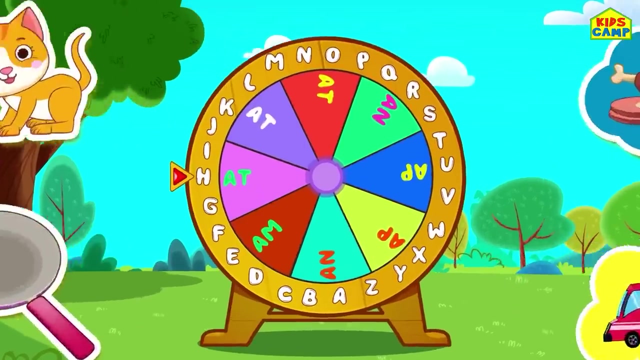 No, Let's keep spinning. Is that a word? Is that a word? H-A-T Hat. That's right, That's how you spell a hat. We found the first word. Let's look for more. Let's spin the wheel. Let's spin the wheel. Let's spin the wheel. 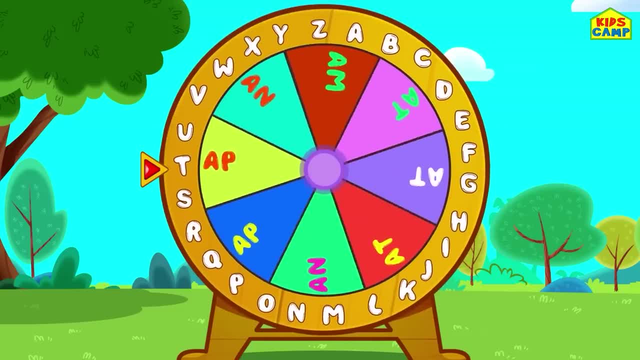 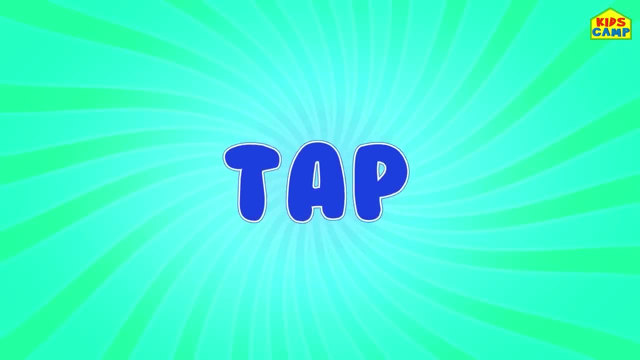 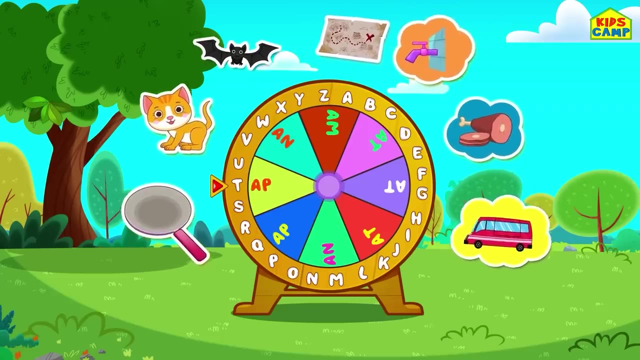 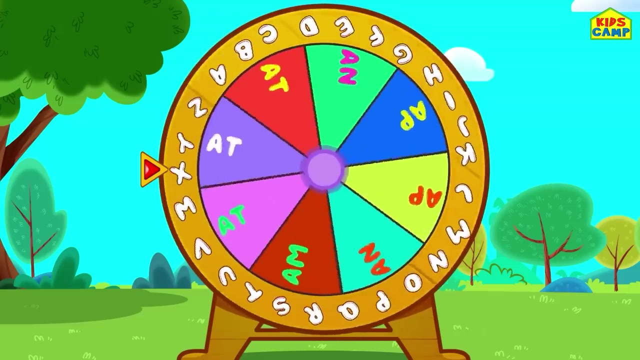 Woohoo, Is that a word? T-A-P-Tap, T-A-P-Tap, That's right, That's a word, A tap, Wonderful, We found one more. Let's look for some more. Keep spinning, Keep spinning, Keep spinning. Woohoo, Is that a word? 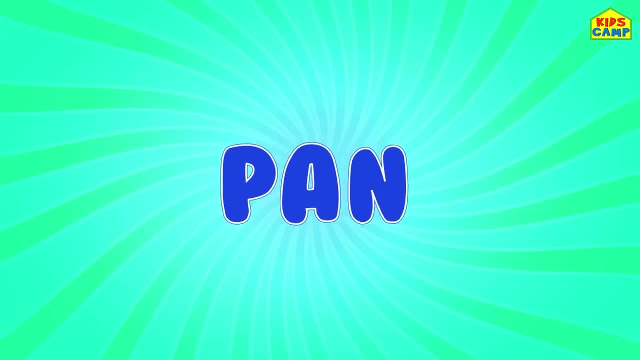 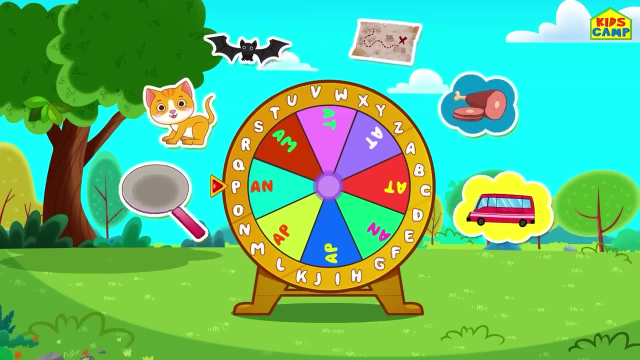 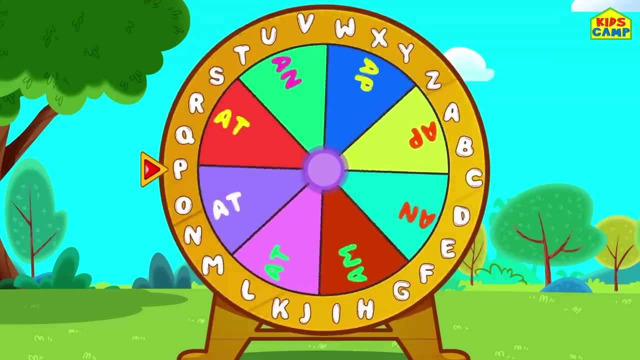 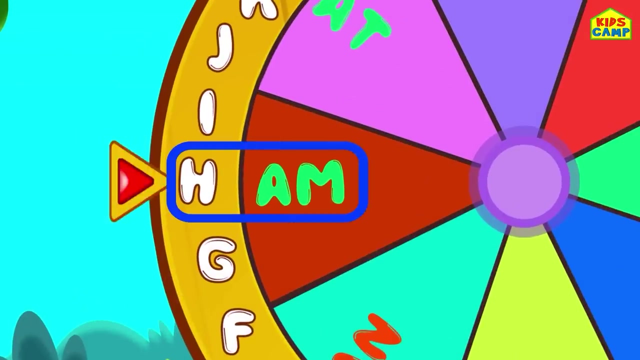 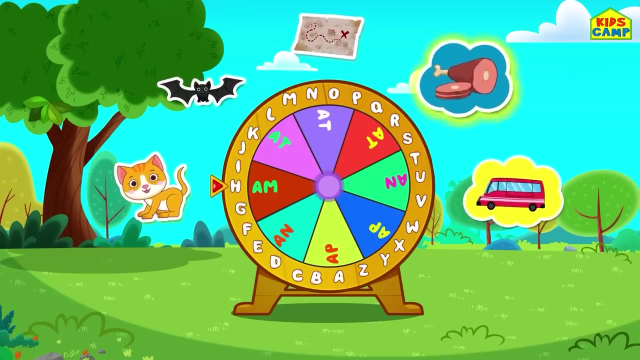 P-A-N Pan- Yes, that's a word. Wow, We found another one. What's next? Let's keep spinning. Let's keep spinning. Yay, Is that a word? Is that a word? H-A-M Ham- That's right, That's a word. Yummy. 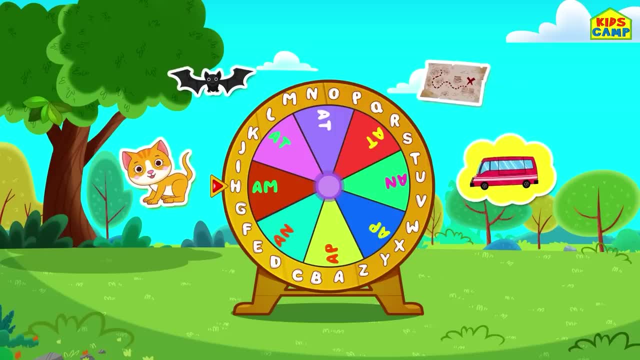 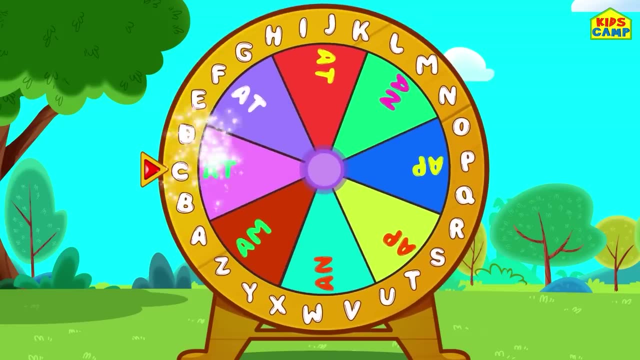 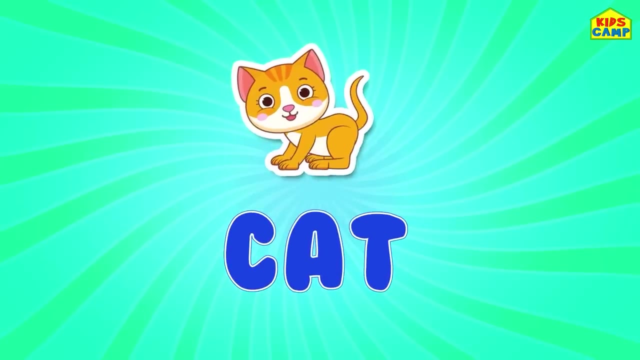 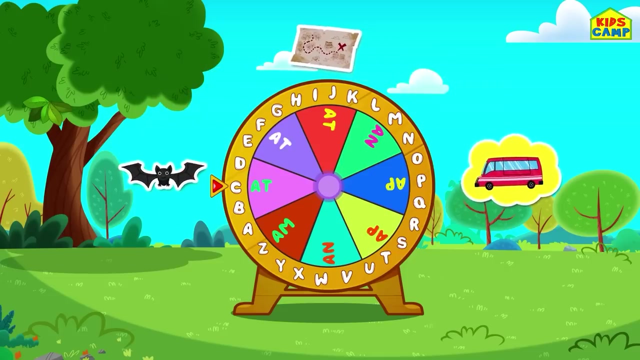 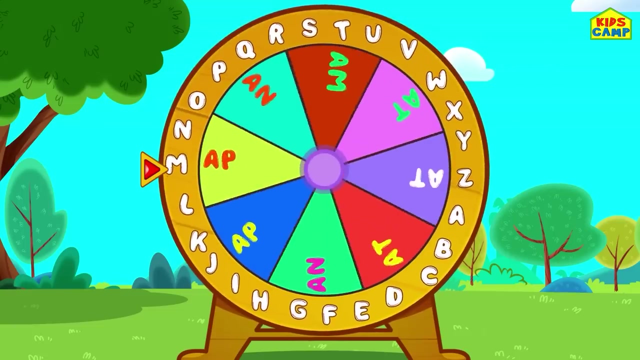 We found another one. Let's find some more friends. Let's spin the wheel. Let's spin the wheel C-A-T. That's a word. Cat Woohoo, Yay, What's next? Let's spin the wheel again. Word wheel: Keep spinning. Uh-huh, We found another word. 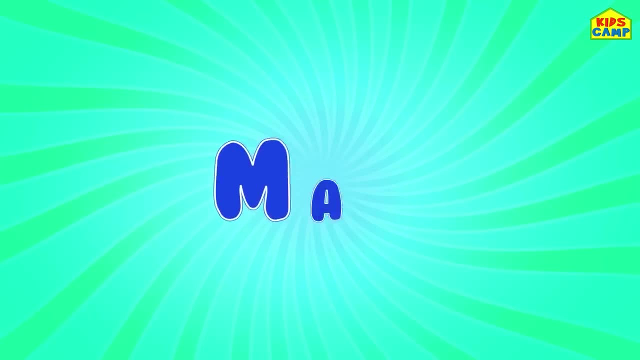 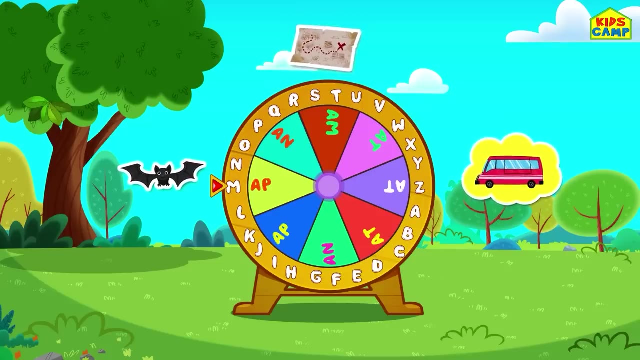 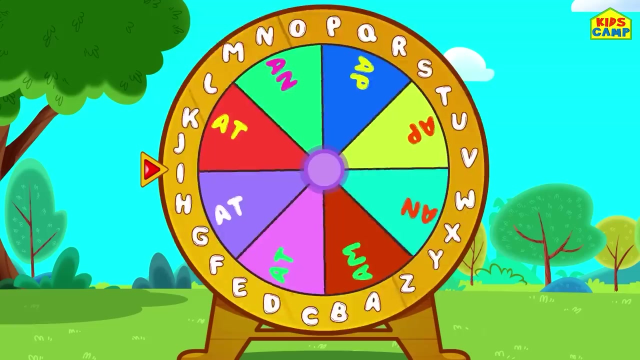 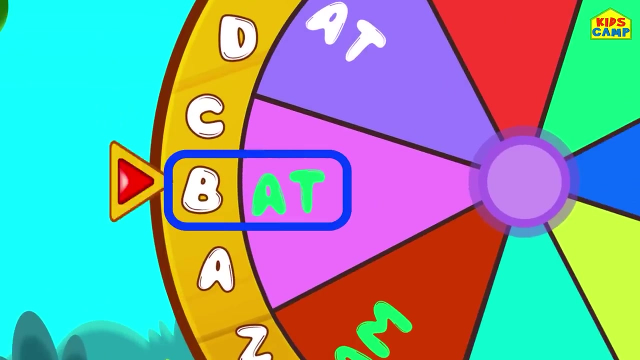 M-A-P Map. That's right. Map is a word. We found the word map. Good job, friends. Let's keep spinning the wheel. Let's keep spinning the wheel. What's next? That's a bat. That's a bat. B-A-T bat. That's right. We found another word. 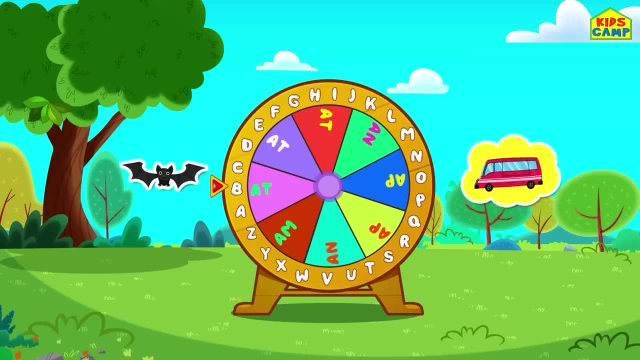 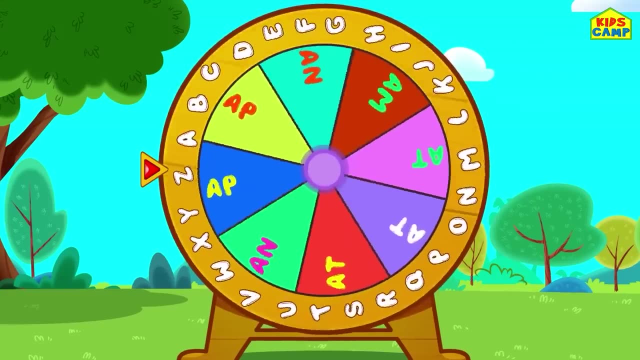 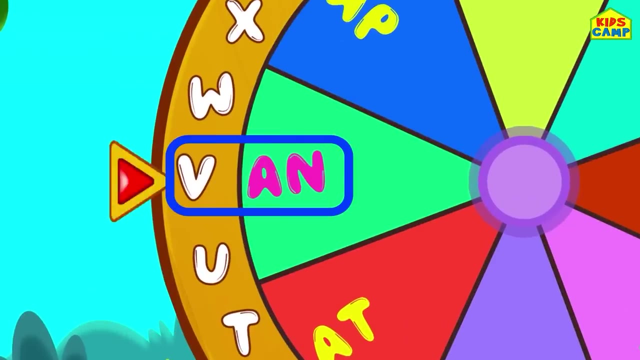 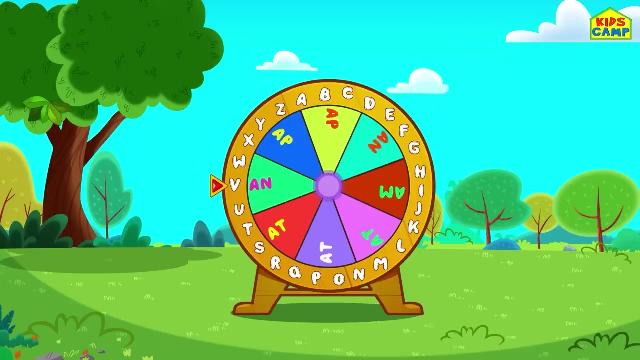 A bat Good job. What's the last word? Let's keep spinning the wheel. Let's keep spinning the wheel. It is A van B-A-N Van. That's right, Yay, Woohoo, We got all the words. We had lots of fun today, Yay. 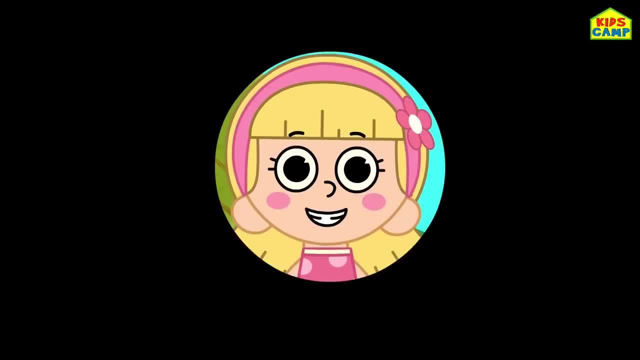 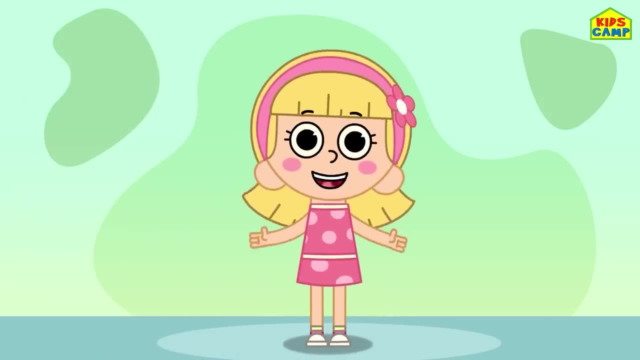 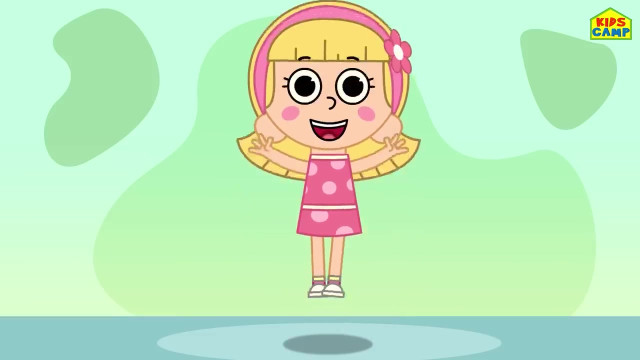 We learned some new words today. Bye, Hi kids. I am Ellie And I am going to put up some pictures In Eva's bedroom. But there is just one tiny problem. There seems to be a missing piece In each picture. Can you help me find it? Woohoo. 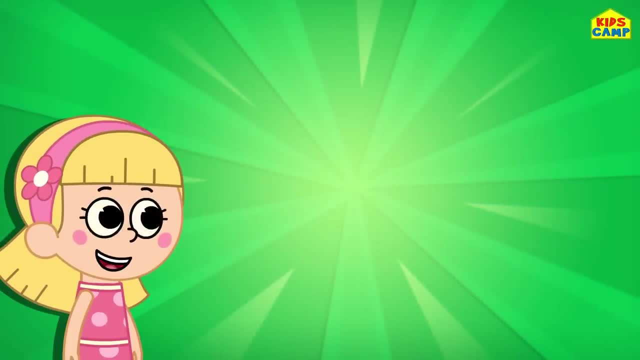 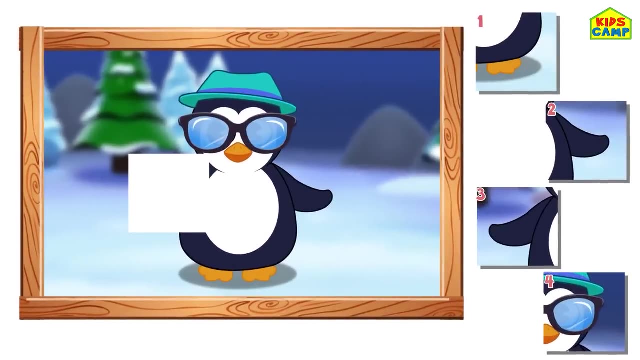 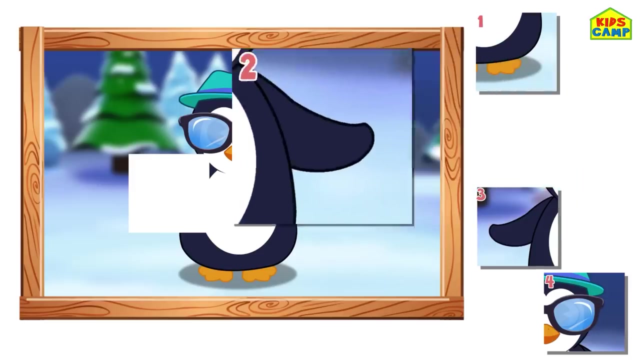 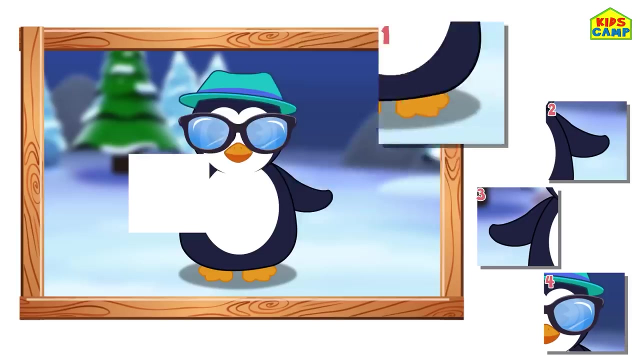 Let's get started. This is going to be a fun game. Let's find the missing piece. Hmm, Do you know which one is the right piece? Let's try. Is number two the right piece? No, It isn't. Is number one the right piece? No. 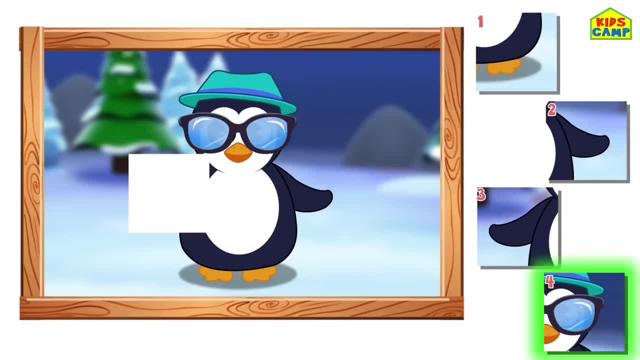 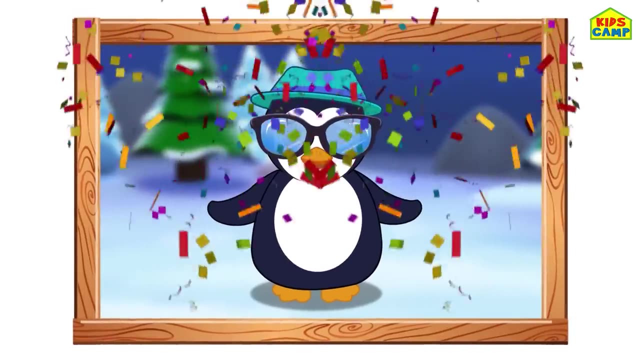 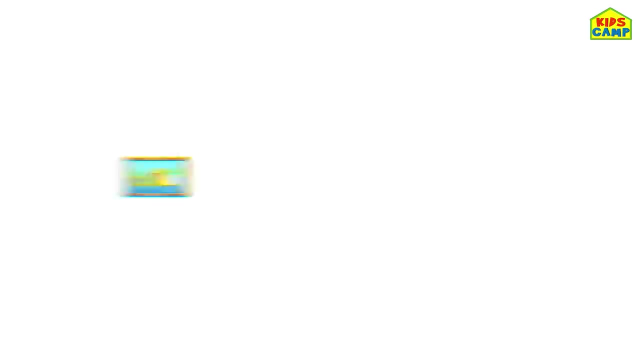 Uh oh, It isn't. Is number four the right piece? No, No, Hmm, Let's try number three. Yes, We got the right one. Woohoo. Good job, kids. Let's move to the next one. What is missing from here? What is missing from here. 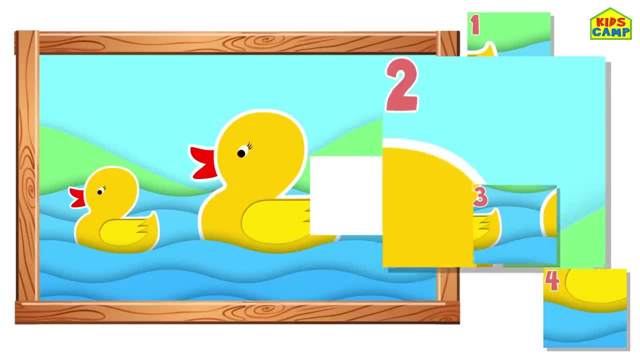 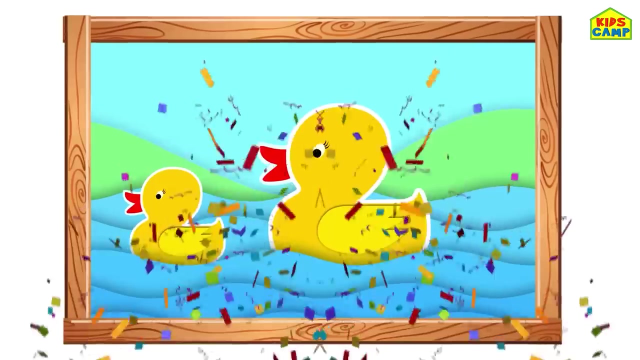 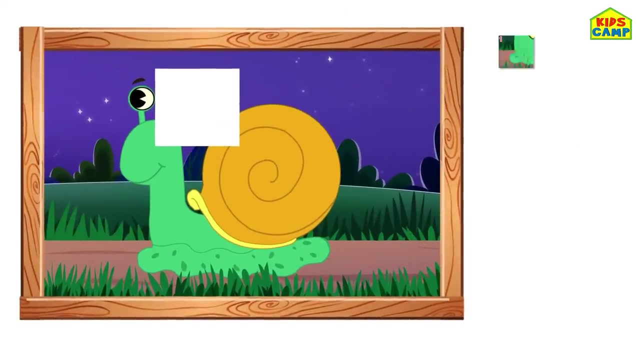 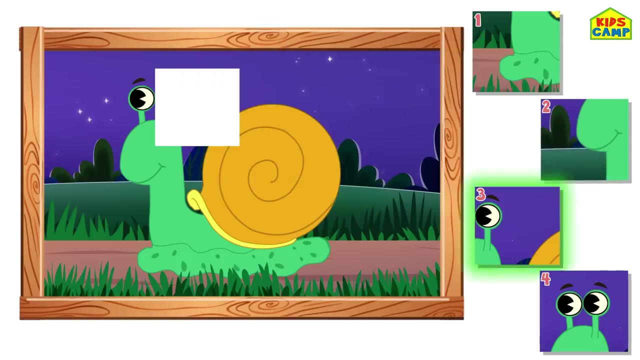 Let's try number two: No, No. Let's try number four. No, No, No, No. Let's try number one. Yay, That fits right, We got it. Woohoo, Moving on. Hmm, What's missing here? Let's find out. Let's try number two. No, That doesn't fit right. 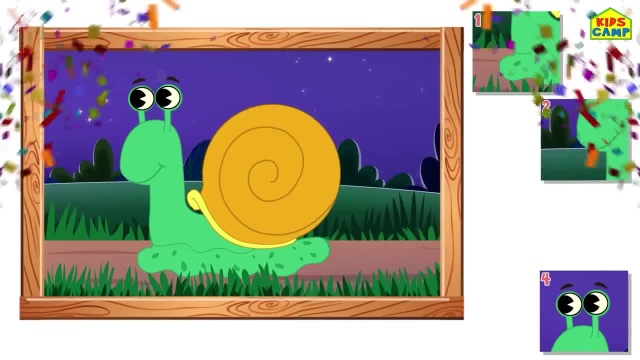 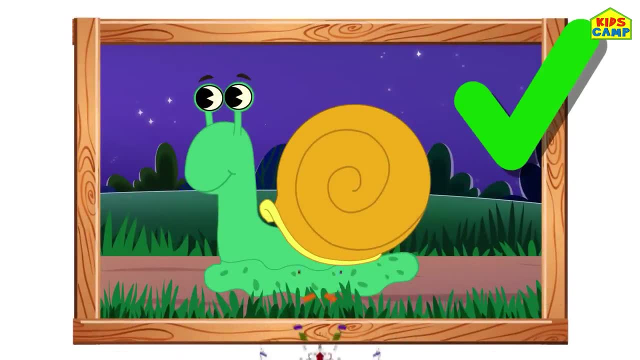 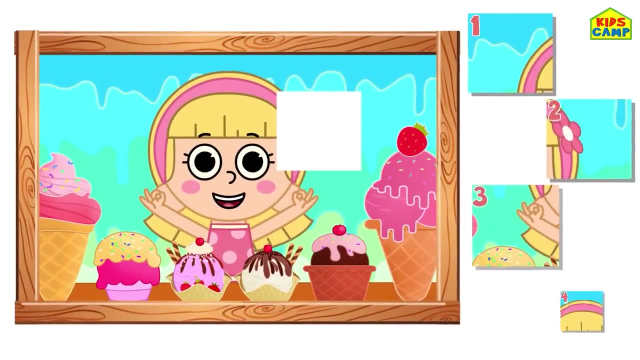 Let's try number three. Wow, We did it. We got that one right, Ready to go. Let's go up on the wall Moving on. Hmm, What's missing here? Let's try number one. No, That doesn't seem right. Let's try number four. No, No, Let's try number three. 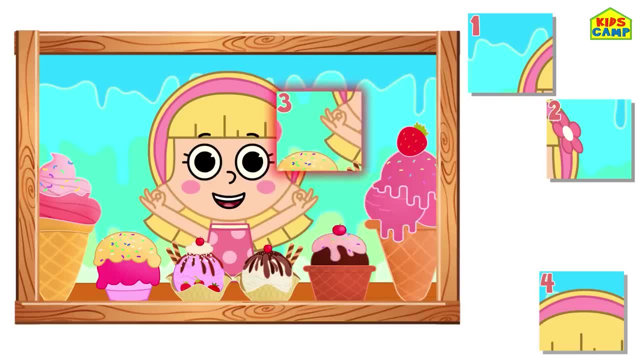 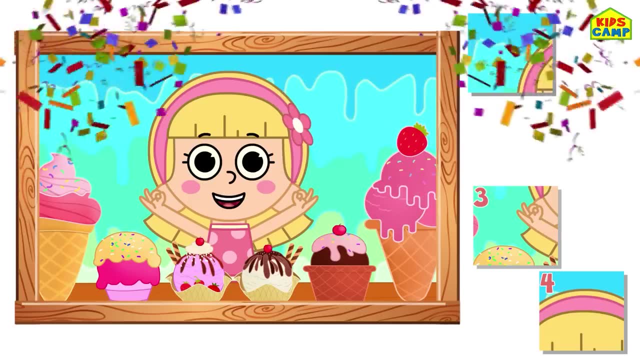 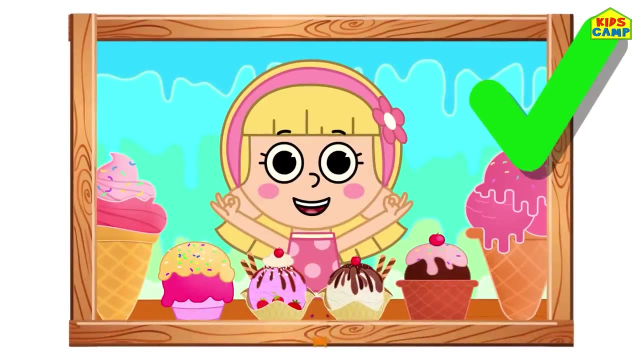 No, No way. Let's try number two. No way, No way. Yes, this fits right. Woohoo, we did it again. Good job, kids. Yay, They already look so good up on the wall. They already look so good up on the wall. Eva's gonna love this. 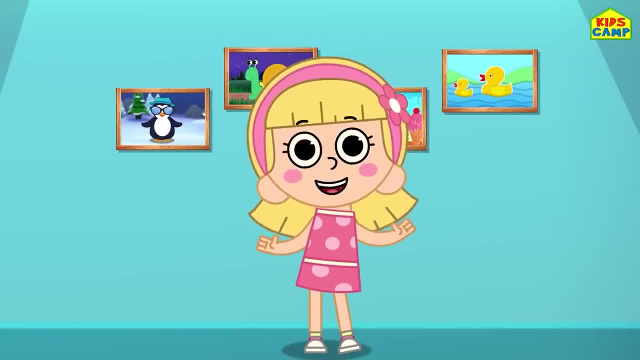 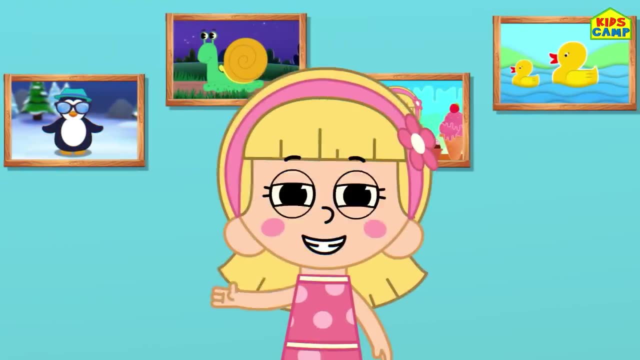 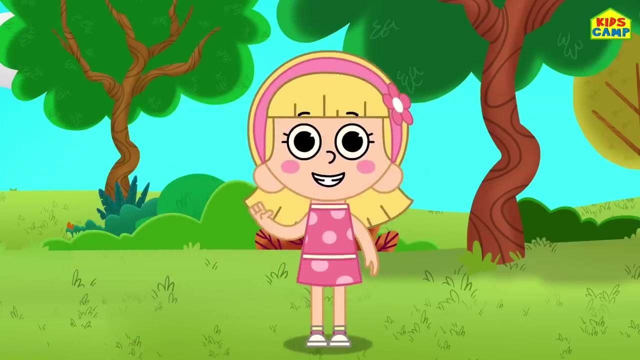 Eva's gonna love this. Thank you so much for helping me out. Thank you so much for helping me out. This was a fun game And I hope you guys will come back for more learning videos. Until then, Bye bye, Bye, bye. Hi, I'm Ellie And we are going to play. spot the difference. 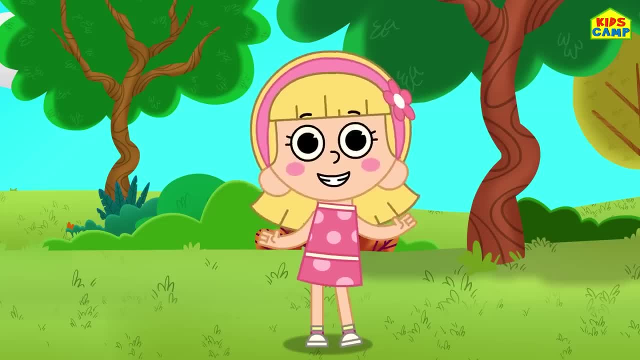 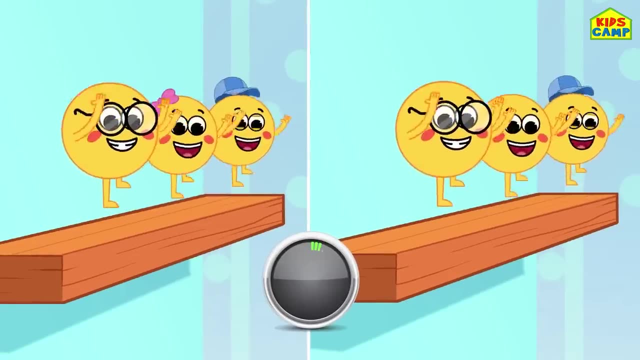 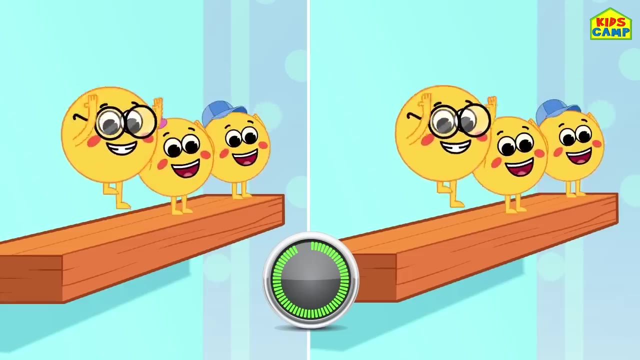 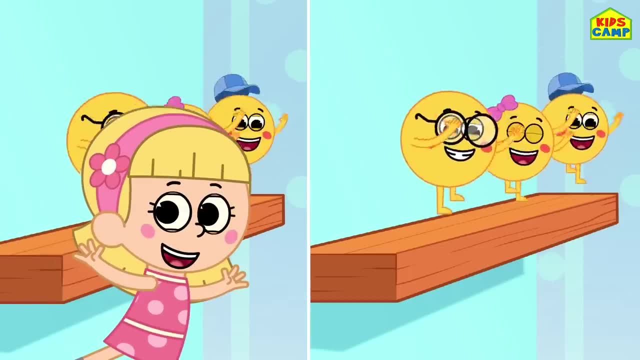 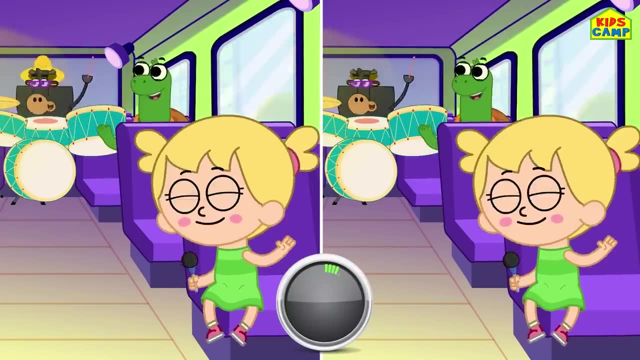 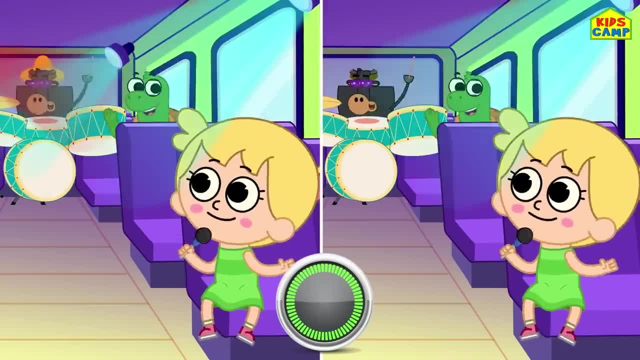 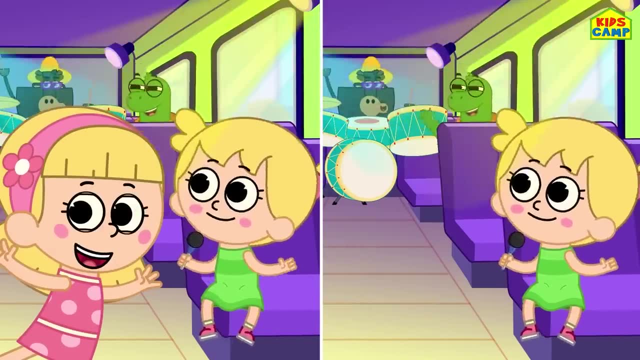 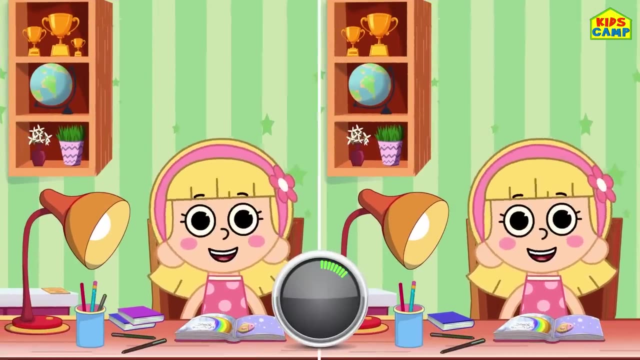 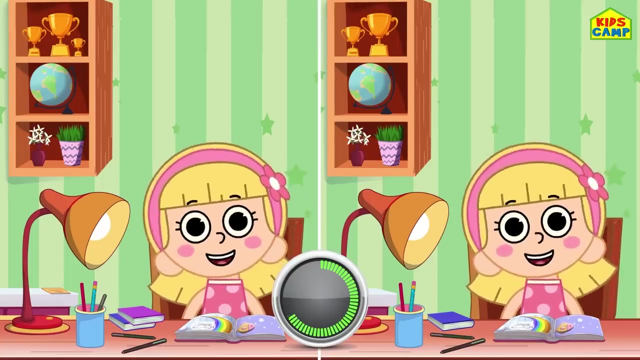 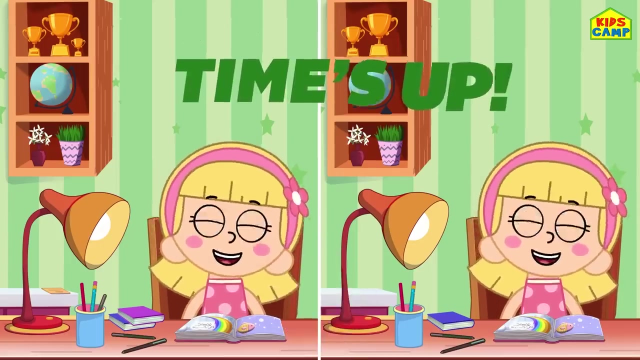 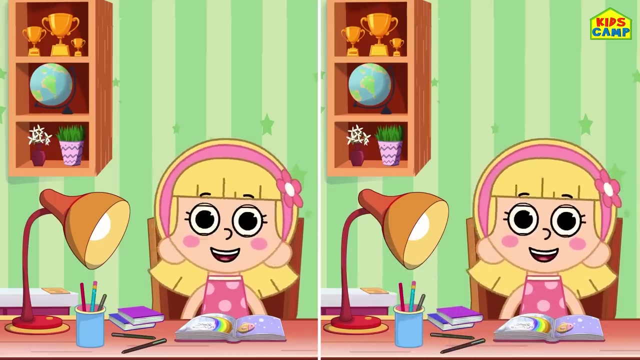 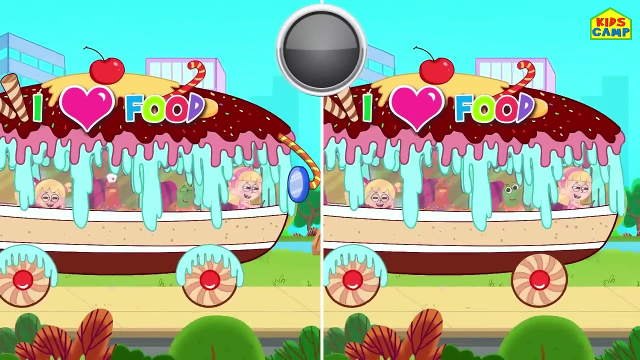 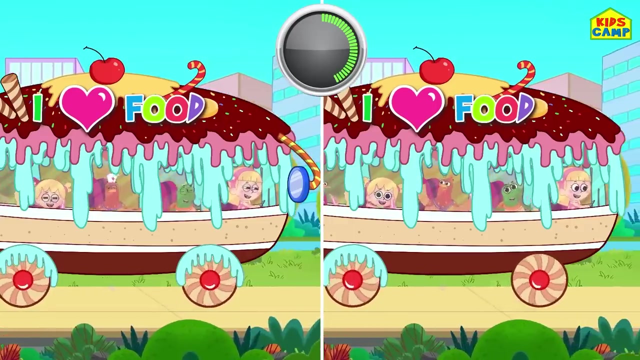 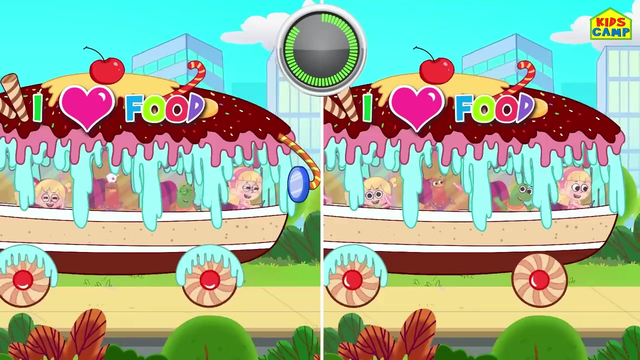 Can you spot the difference? Let's do the next one. Can you spot the differences? That's right, You got it. Next one: Can you spot the differences? Keep trying. Next one: Can you spot the differences? Can you spot the differences? 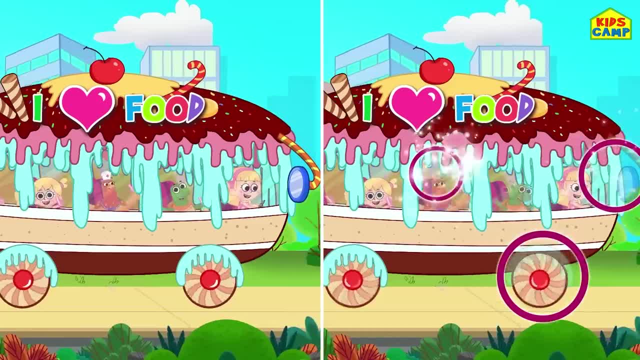 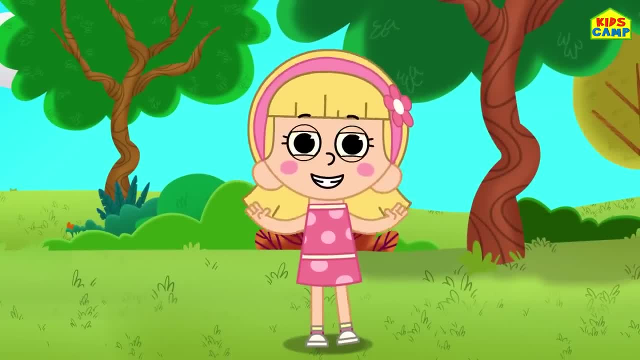 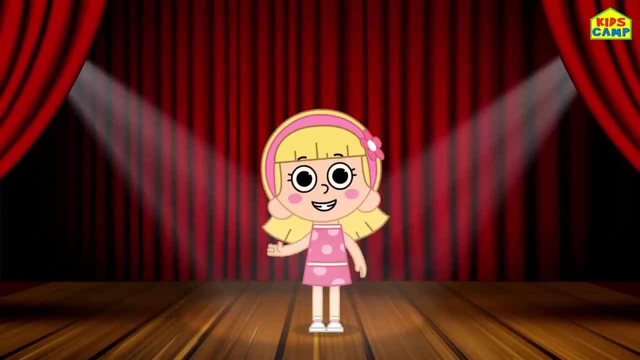 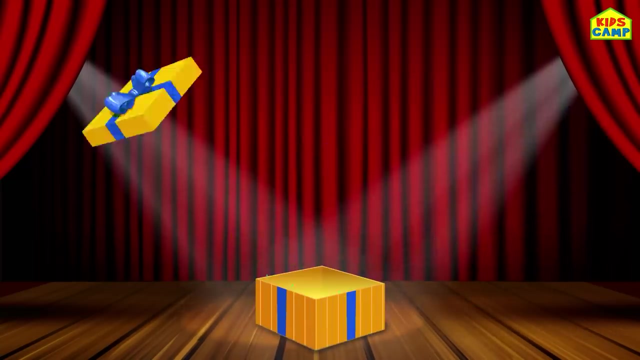 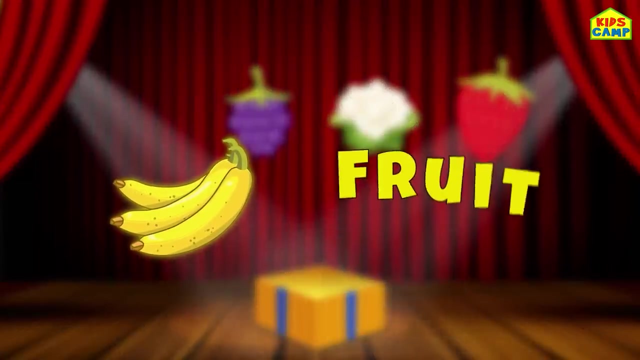 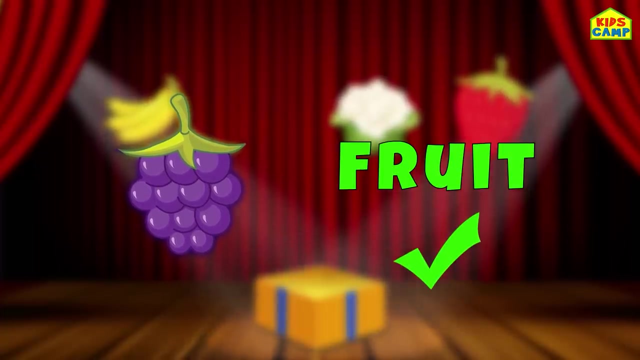 Time's up. You got it. Good job, kids. This was so much fun. Keep watching Kids Camp. Bye-bye, Let's go Spot the odd one out. Is this a fruit? Yes. Is this a fruit? Yes. 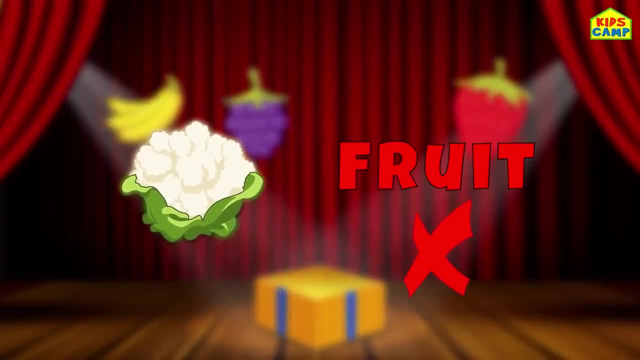 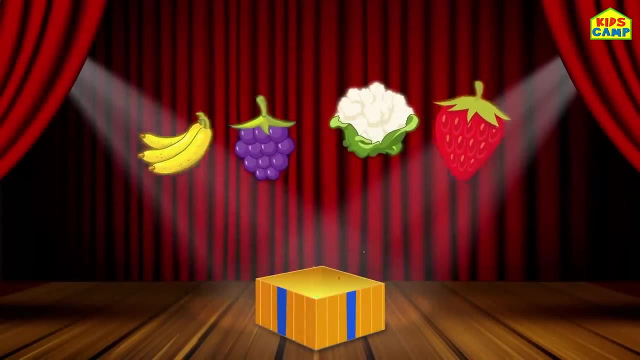 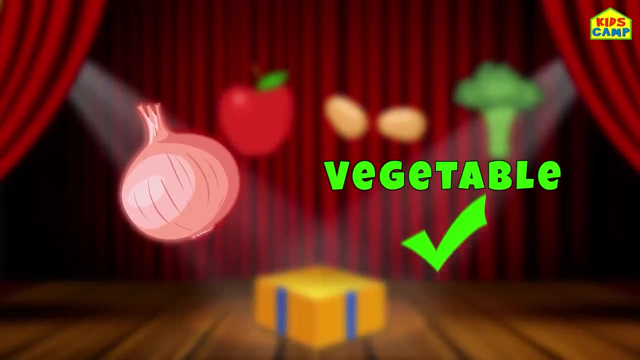 Is this a fruit? No, Is this a fruit? Yes, Here we go. This is the odd one out. Spot the odd one out. Hey kids, can you spot the differences? This is the vegetable. Yes, Is this a vegetable? 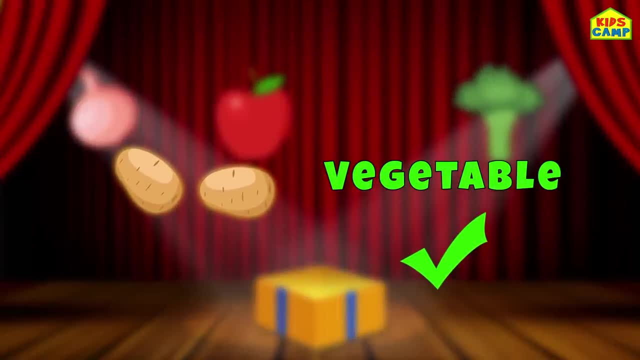 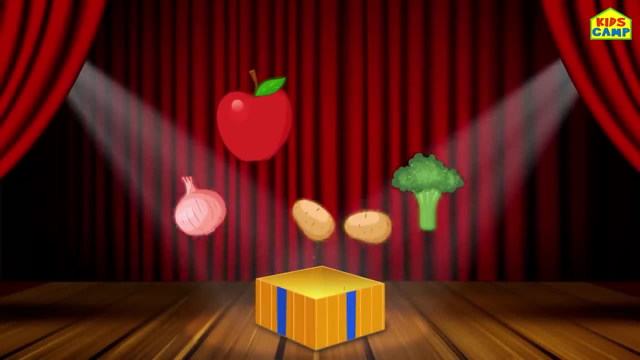 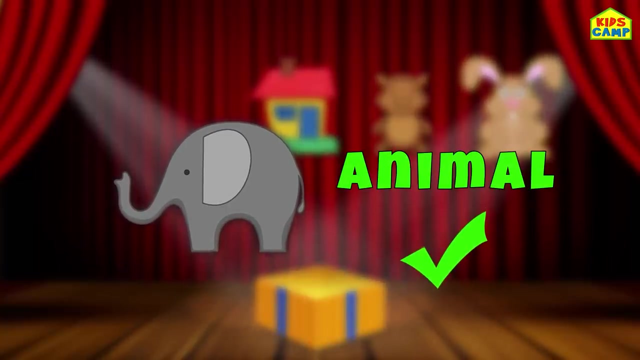 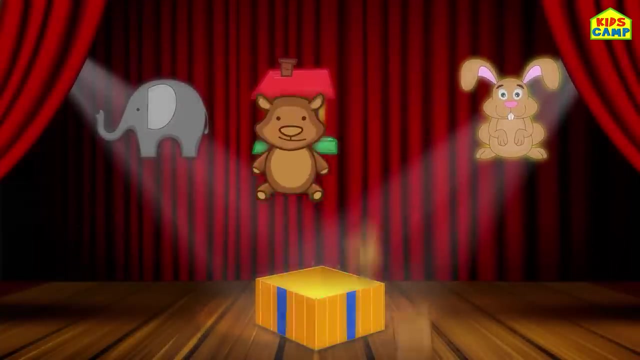 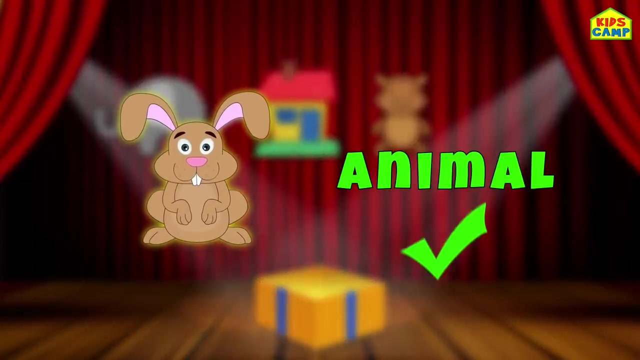 Yes, Is this a vegetable? No, Is this a vegetable? Yes, Is this a vegetable? odd one out. What next? Is this an animal? Yes, it is. Is this an animal? No, Is this an animal? Yes, yes, Is this an animal? Yes, it is. We spotted the odd one out there as 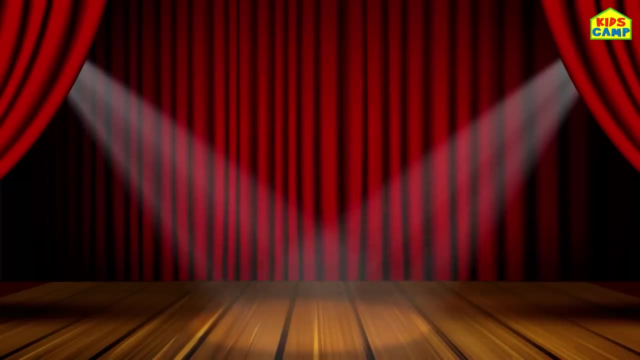 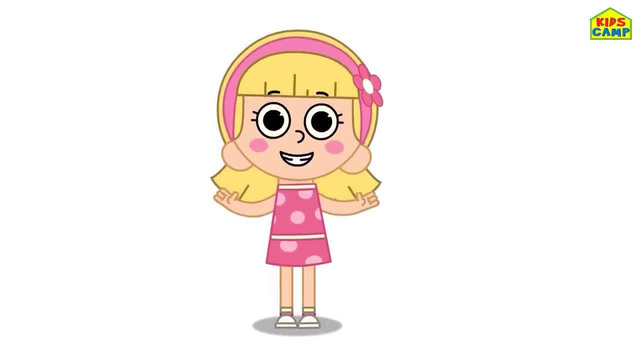 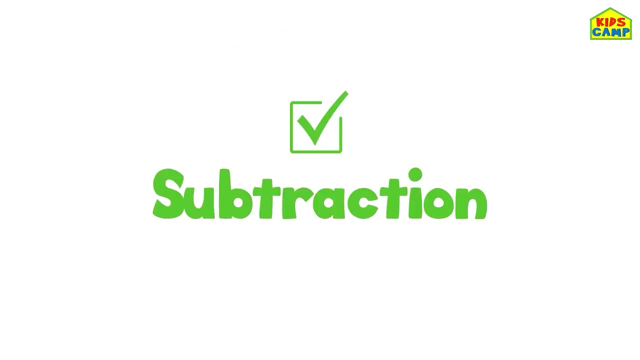 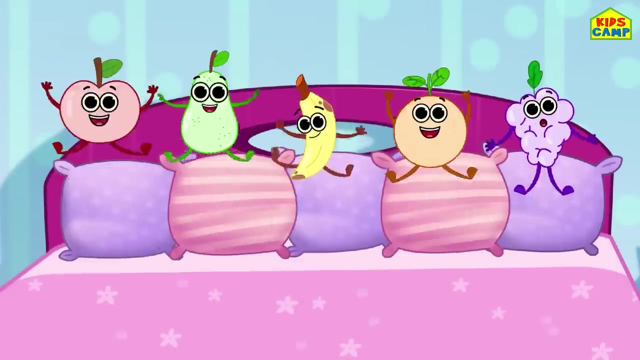 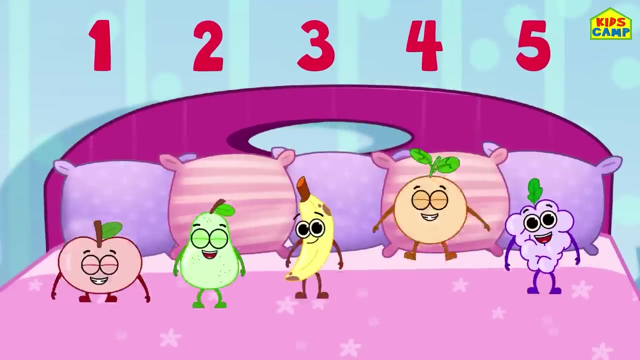 well, Good job kids. Hi, I'm Ellie. Well, hello boys and girls. Today we are going to learn how to do simple math Subtraction. That's right, We have five fruits. Look at them jumping on the bed, So cute. One, two, three, four, five, Wow. 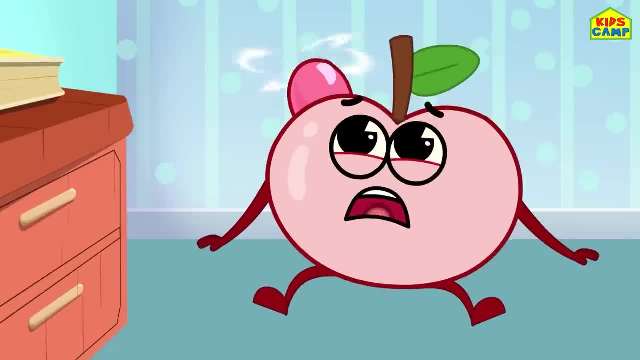 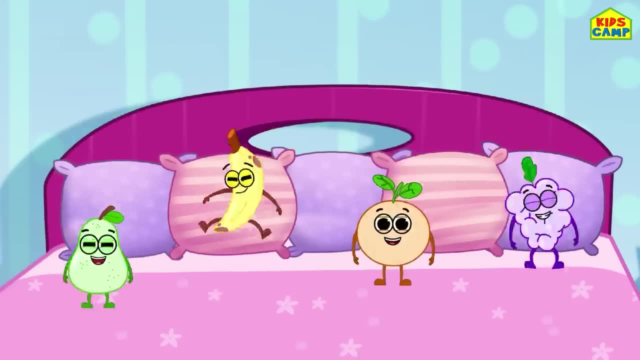 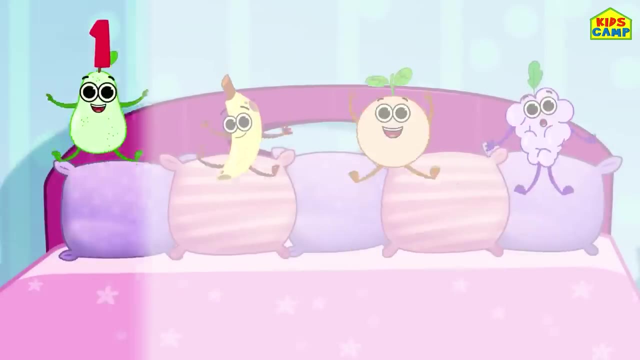 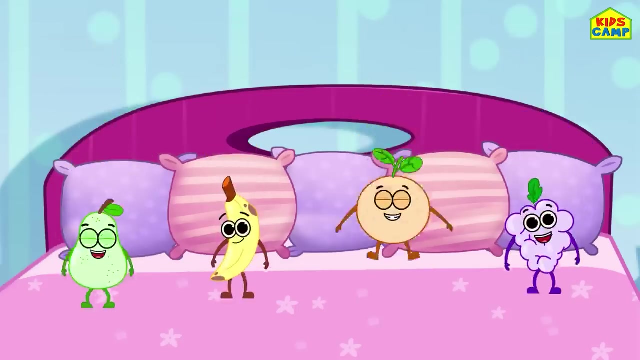 Five fruits. Oops, one of them fell down. How many fruits do we have on the bed now? Five minus one is We have one, two, three, four. We have four fruits jumping on the bed. That's right, Five. 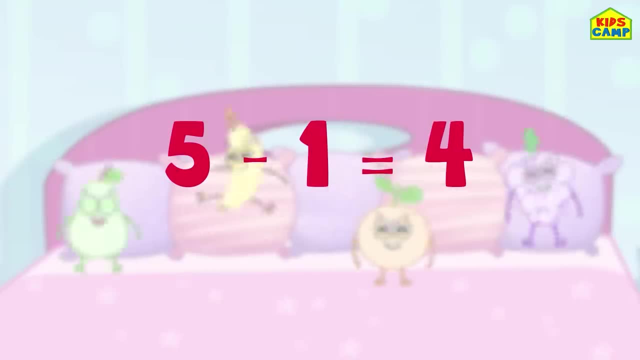 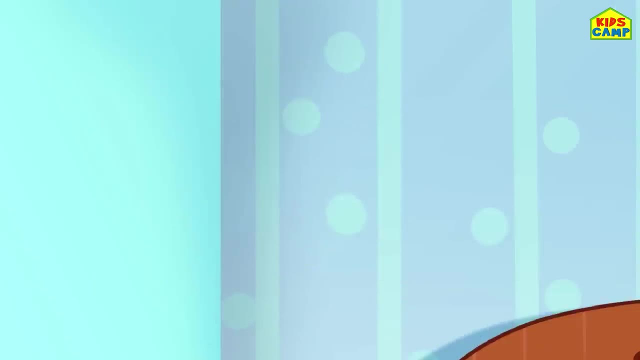 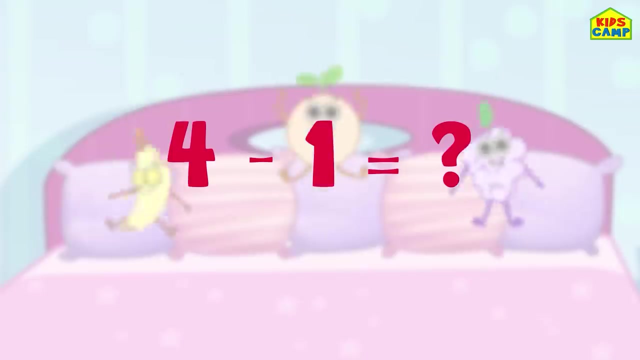 minus one is four. We have four fruits jumping on the bed. Oops, one fell off. Oh, How many fruits do we have jumping on the bed now? Kinda easy, Four minus one is: Is it four, Is it two, Is it one, Is it three? Let's. 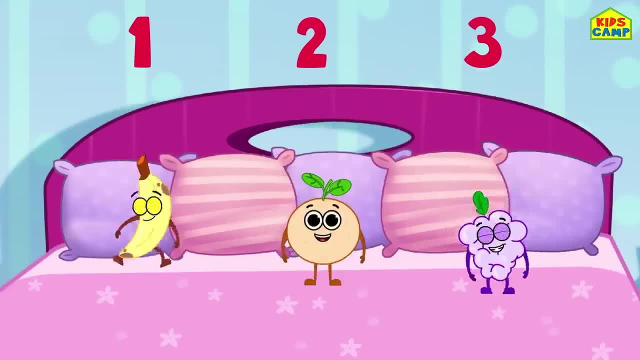 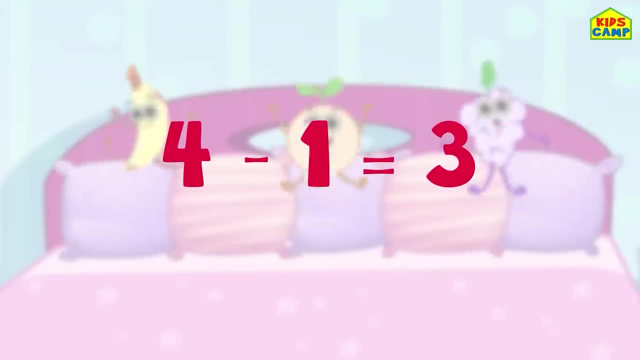 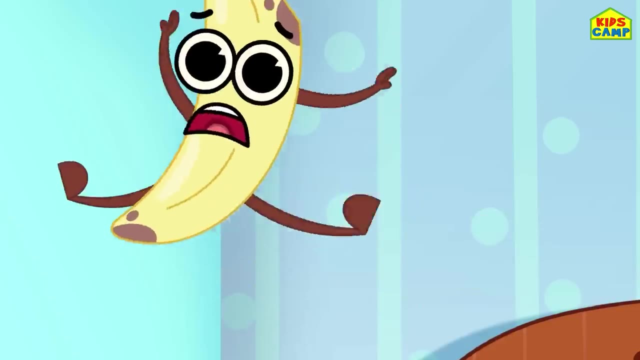 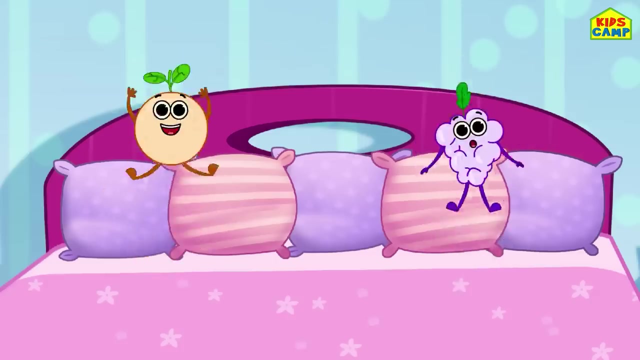 count One, two, three. We have three fruits jumping on the bed. Four minus one is three. Yay, So hey, big Oops, One more fell off. Oh, Three minus one is Is it one, Is it two? 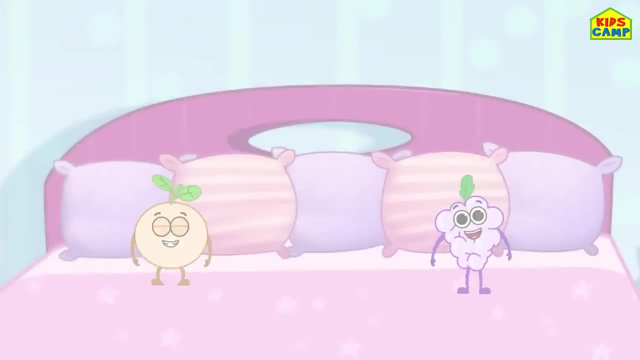 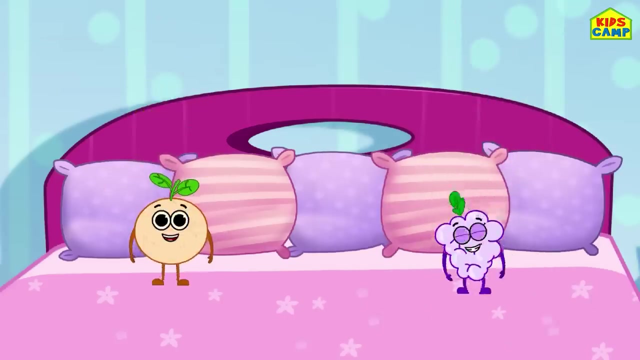 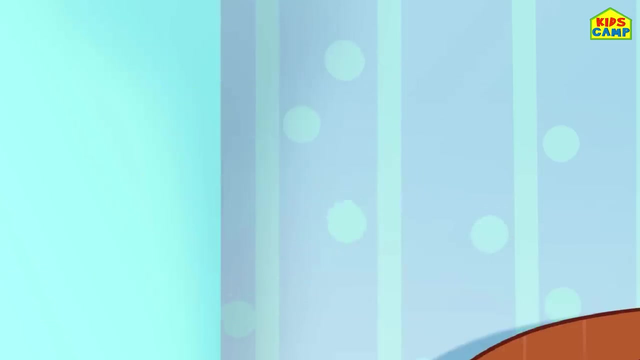 Or is it three, One, two. We have two fruits jumping on the bed. Three minus one is two. Woo-hoo, Wow, One more fell off. Ouch, Hmm, How many left on the bed? Two minus one is. 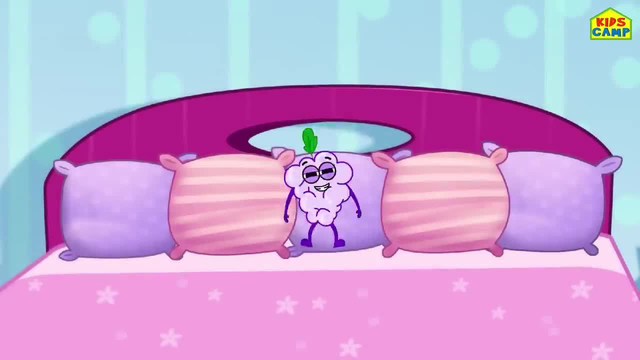 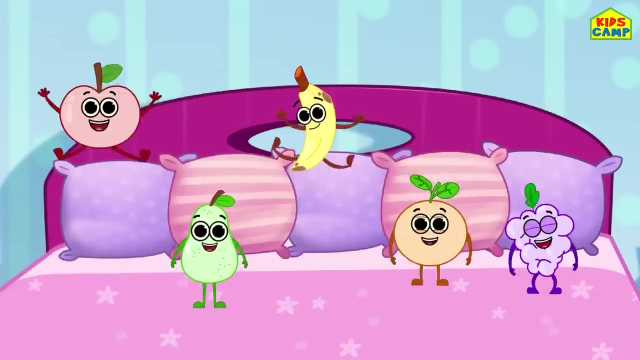 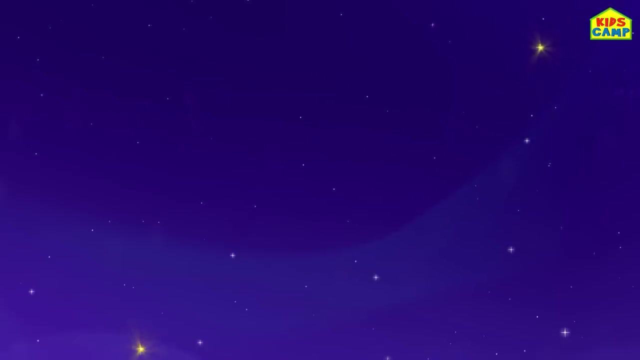 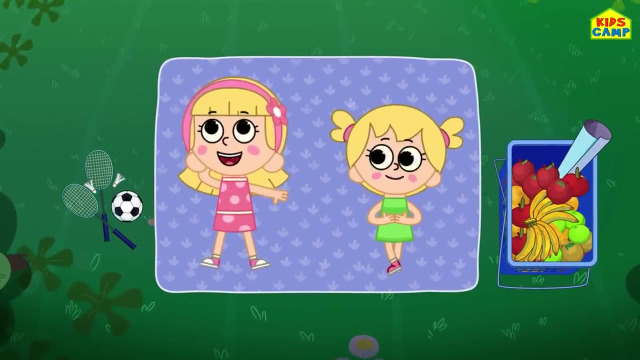 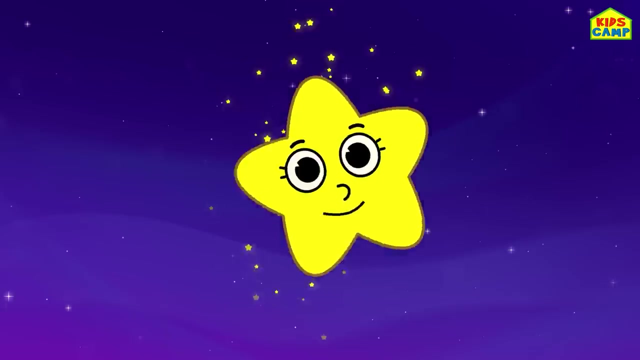 One. Let's put all the fruits back on the bed. Yay, We did it. Good job, kids. Bye-bye, Look, Eva. Twinkle twinkle little star. Twinkle twinkle little star. Tell me what vehicle you are. 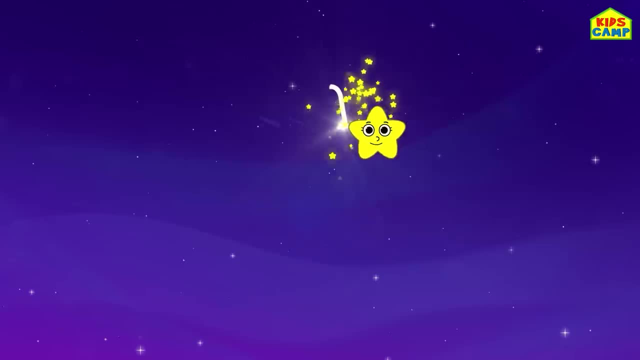 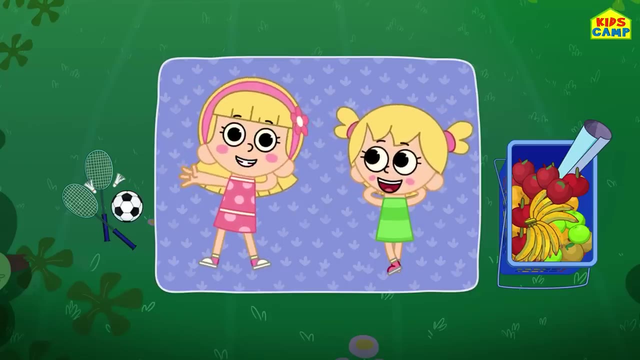 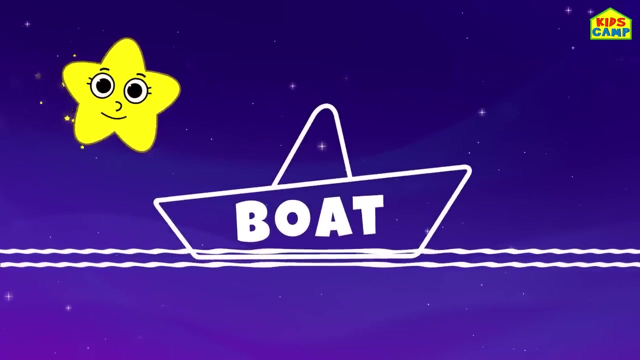 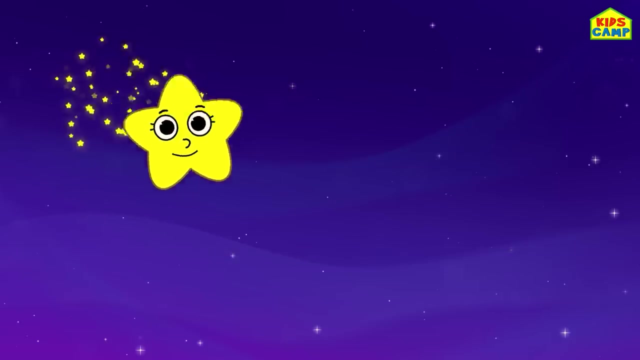 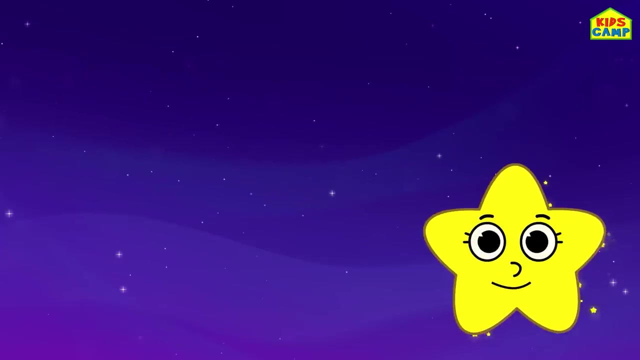 Tell me what vehicle you are. Wow, This is so exciting. Woohoo, What is that? I think it's a boat. The boat sails in the vast ocean. Twinkle twinkle little star, Twinkle twinkle little star, Twinkle, twinkle, twinkle little star. Tell me what vehicle you are. 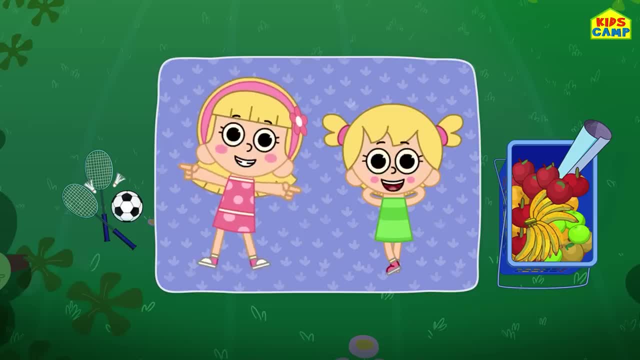 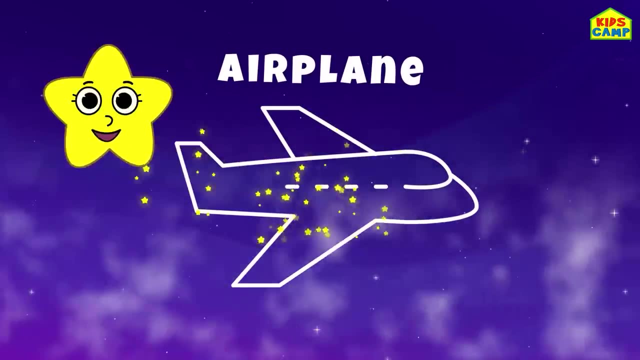 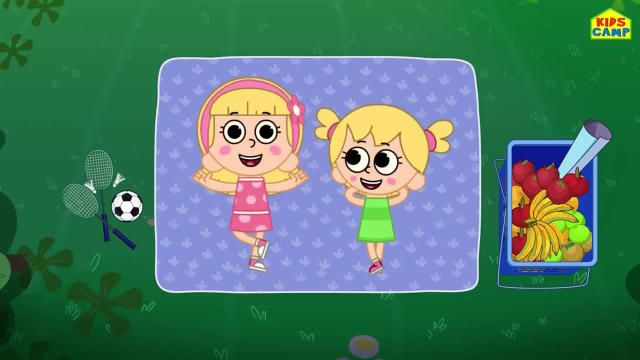 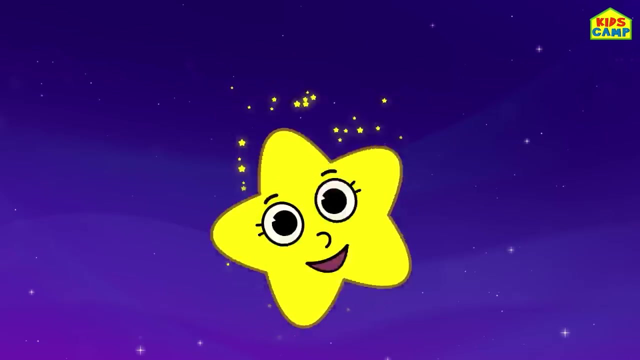 Here comes another one. Wow, Look, It's an airplane. An airplane flies high in the sky and can take us anywhere in the world. Wow, We're getting good at this. Twinkle, twinkle, twinkle, little star. Tell me what vehicle you are. 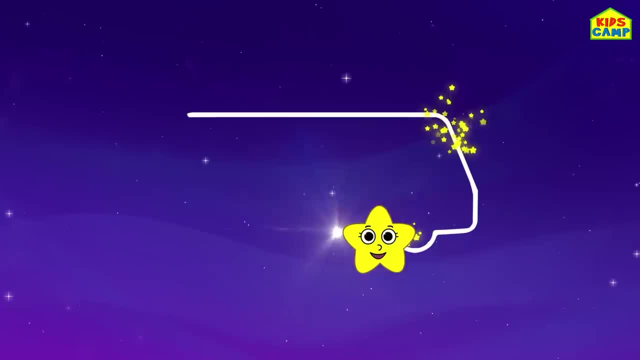 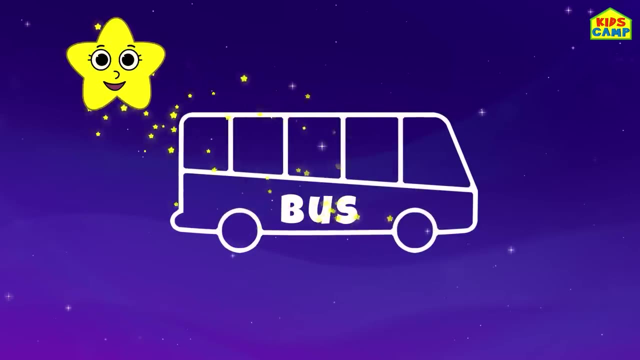 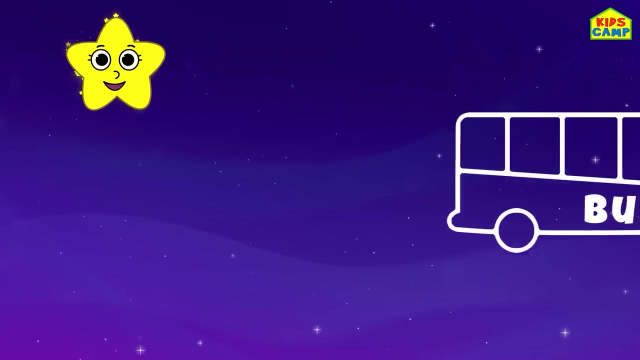 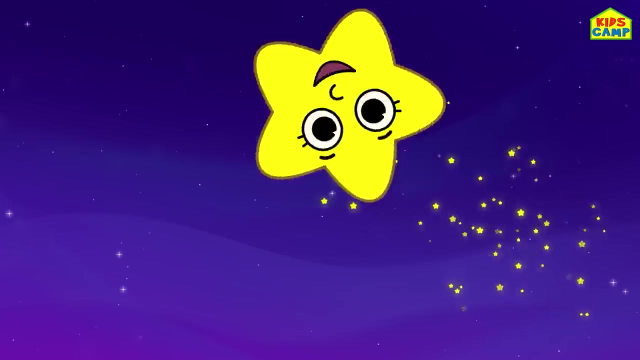 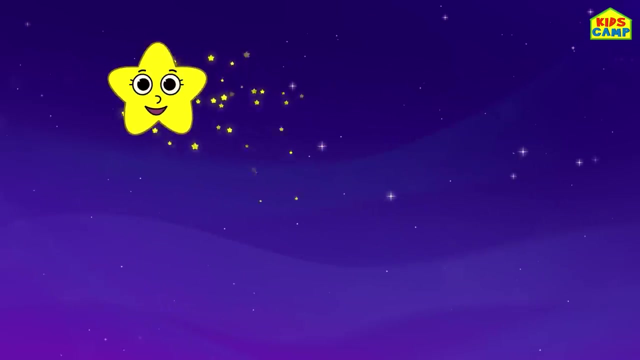 Look. Look One more. It's a bus. You're right, Ellie, We go to school in the bus. It's so much fun. Yay, Twinkle, twinkle little star. Tell me what vehicle you are. Hey, Look. 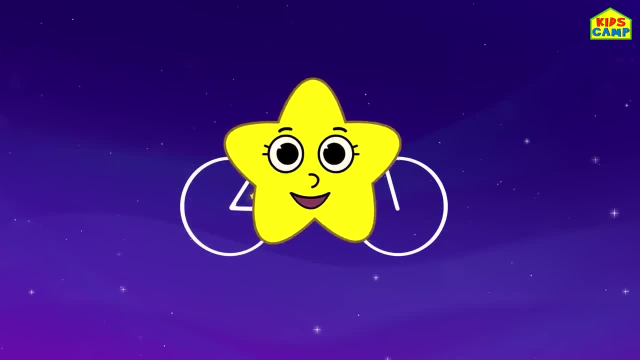 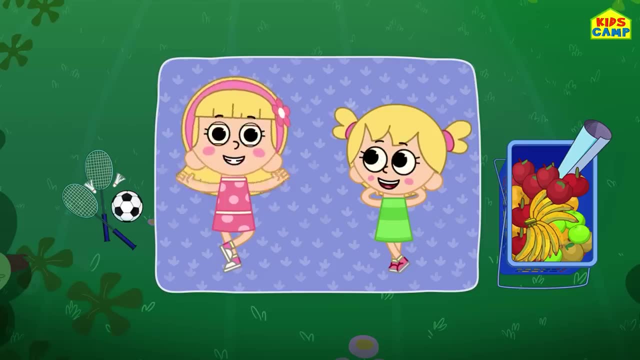 One more: Is that a bicycle? Yes, yes, I love cycling. It also keeps us fit and healthy. Yay, We did it. We had so much fun learning vehicles. Bye, Woohoo, Hi friends, I'm Ellie. 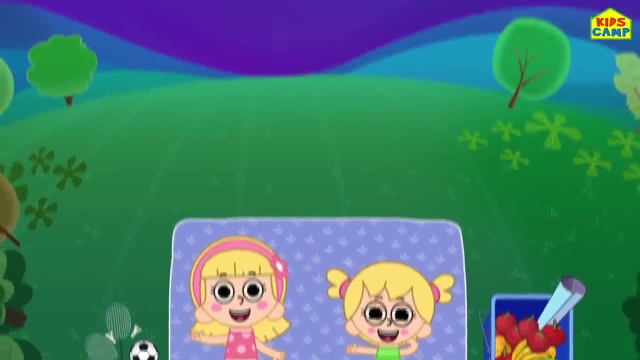 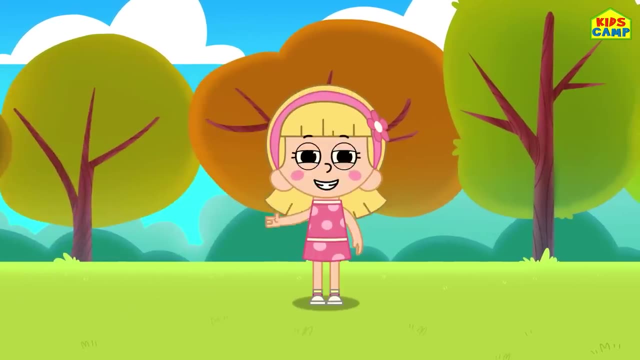 Let's play a fun card game. We have six colorful cards. Let's flip them over and start the game. Yay, Let's go, Let's go, Let's go. Yay, Woohoo, Yay, Yay. 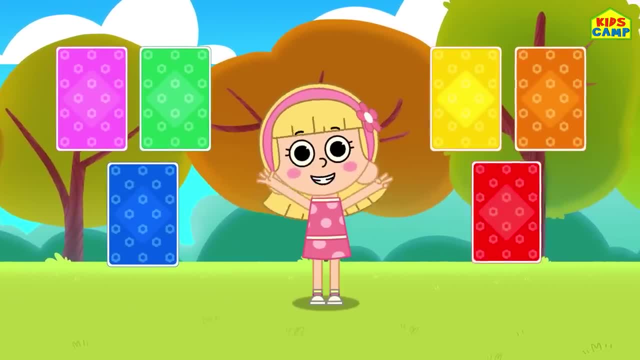 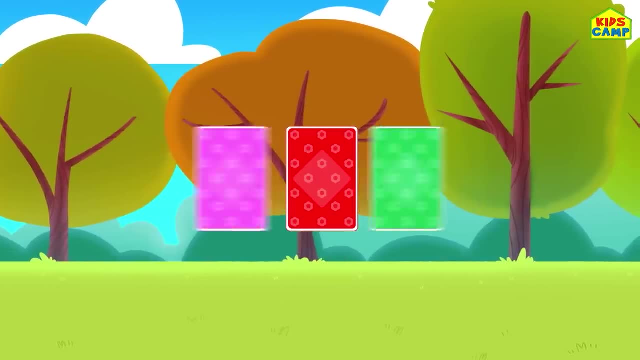 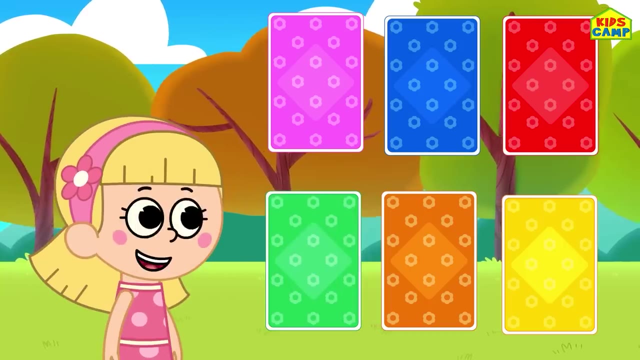 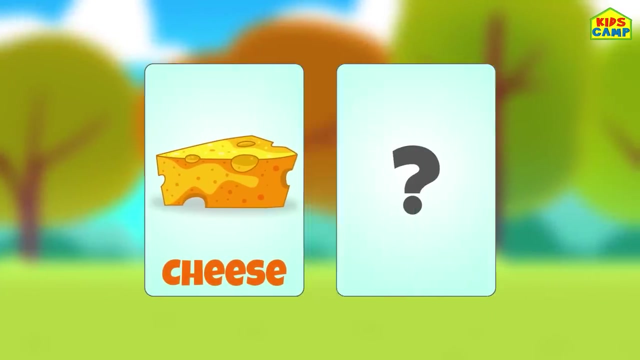 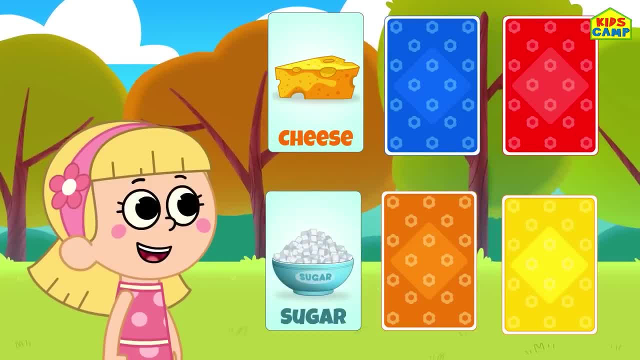 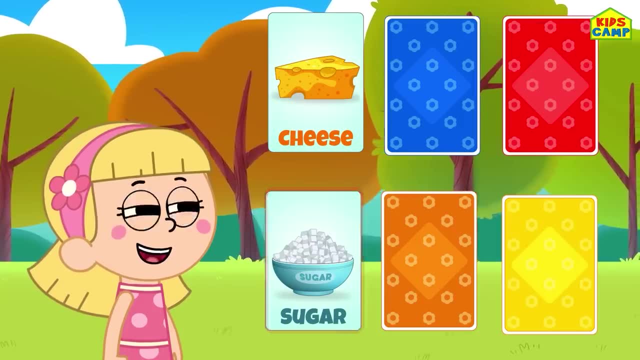 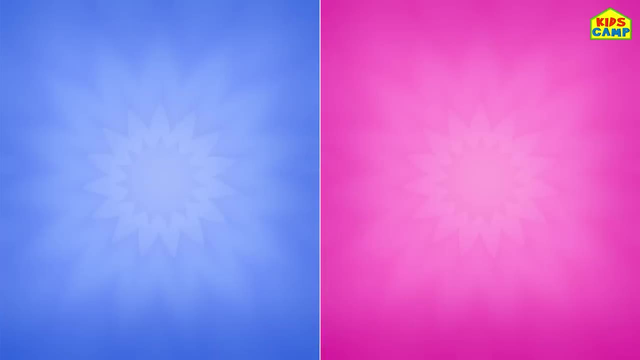 Oh, what is this? It's sugar. Is cheese made from sugar? No, I don't think so. Let's flip another card. Hmm, it's milk. Yes, we got that right: Cheese is made from milk. Yay. 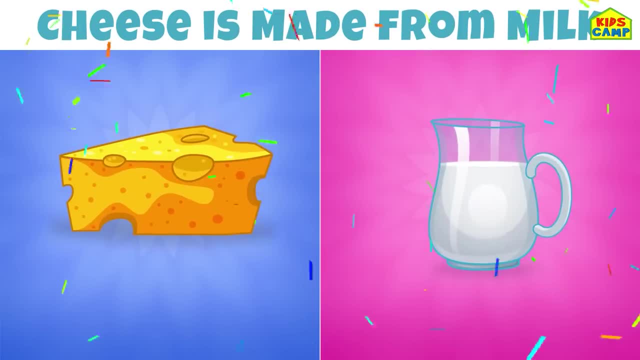 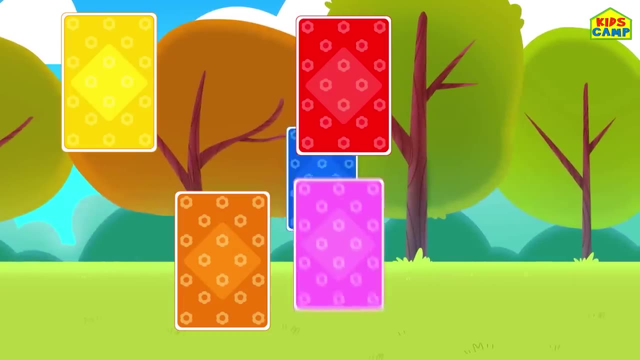 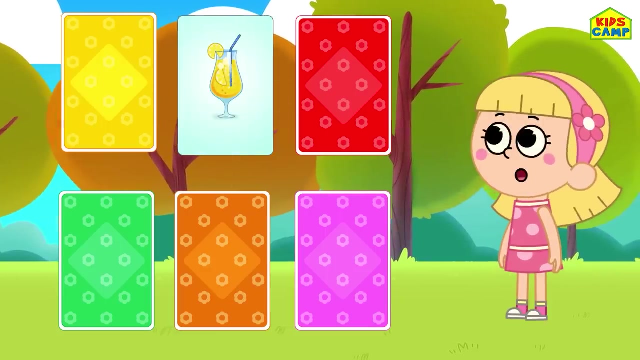 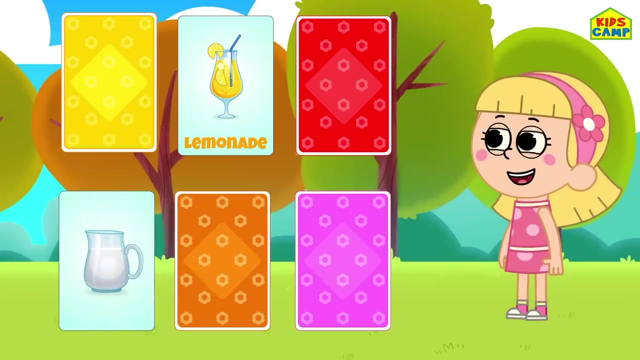 We got that right, kids. Yummy. Let's find out what's next. Let's flip the blue card. Oh, what's that Lemonade? What is lemonade made of? Let's flip this card. Oh, what is this? 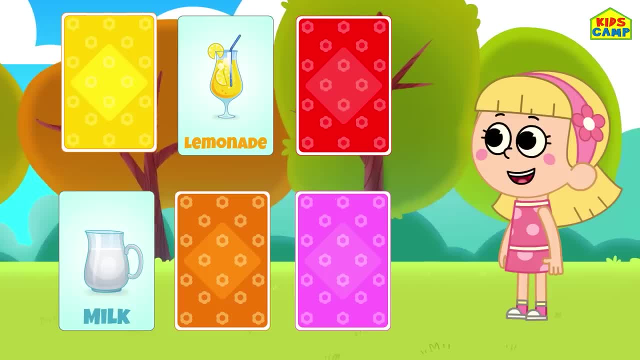 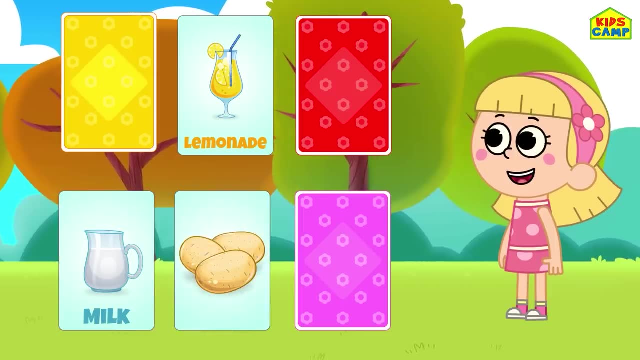 It's milk. Is lemonade made from milk? No, I don't think so. Let's flip another card. Oh, what's this? Potatoes. Is lemonade made from potatoes? No, I don't think so. Let's flip the pink card. 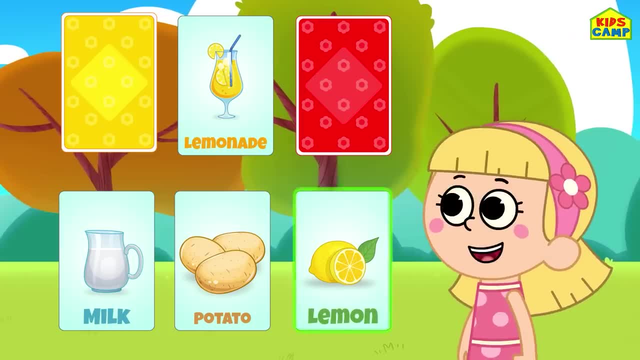 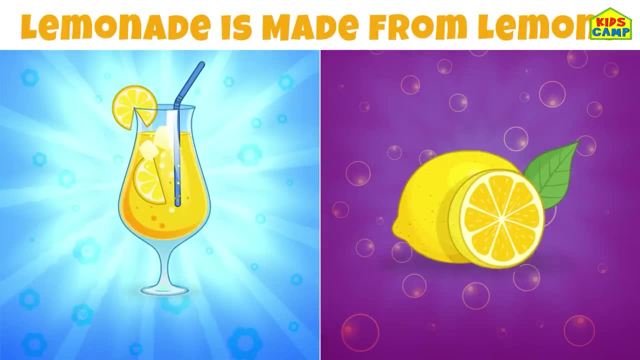 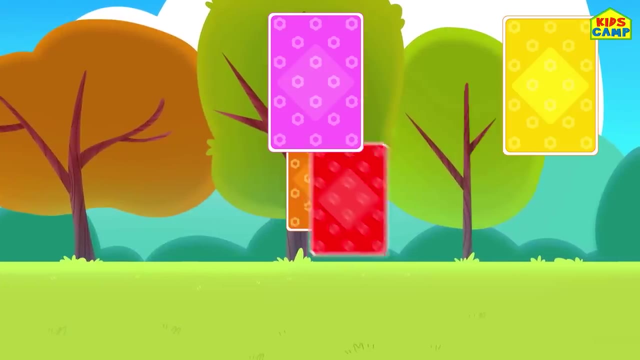 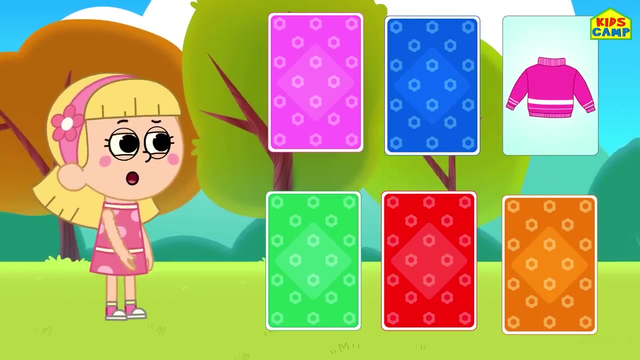 Let's flip the yellow card. Wow, Lemons. Is lemonade made from lemons? Yes, we got that right: Lemonade is made from lemons. I like this game. Let's flip the yellow card. Hmm, what's this? 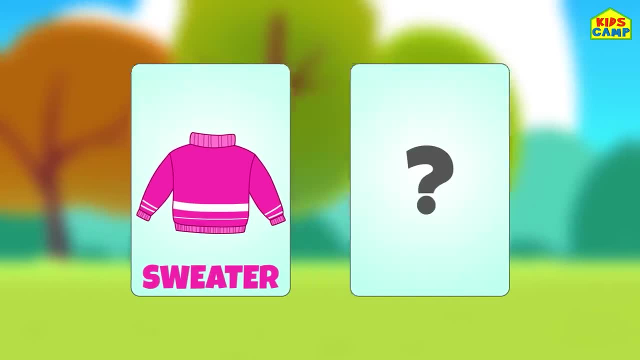 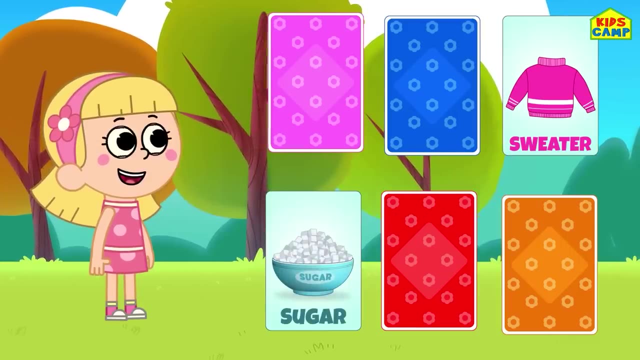 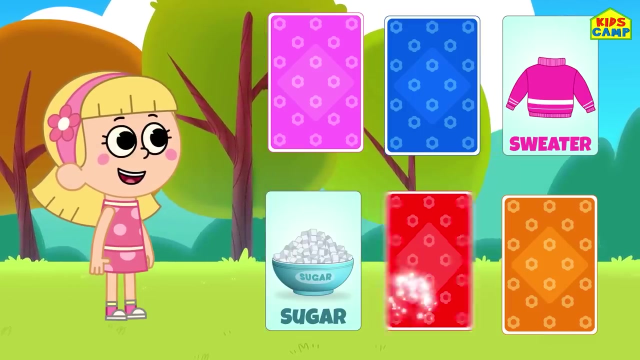 It's a sweater. What is a sweater made of? Let's flip a card: Wow, What's this Sugar? Are sweaters made from sugar? No, definitely not. Let's flip the red card: It's wool. Do we make sweaters from wool? 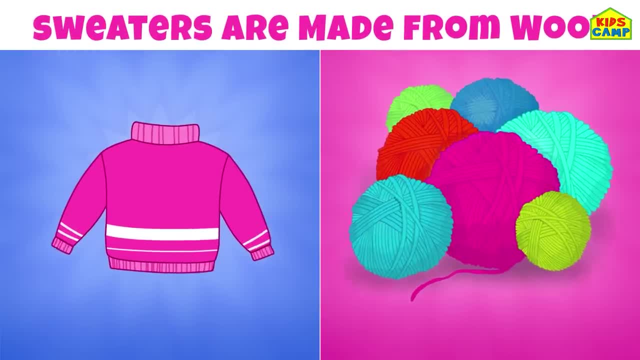 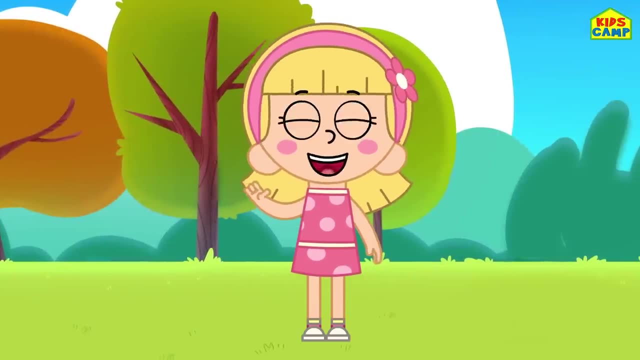 Yes, we do. Sweaters are made from wool. Good job, Yay, We did it. Bye-bye. 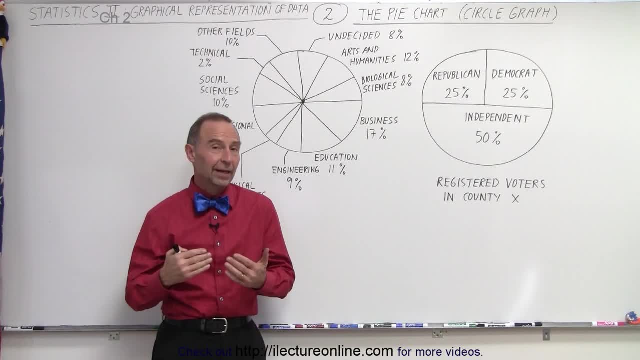 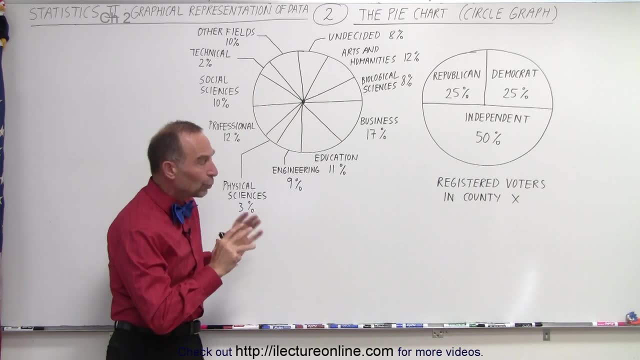 Welcome to iLecture Online. One of the most useful and most common graphs is the circle graph, also called the pie chart, And the reason why it seems so popular is because it gives us a really visual representation of what's going on, especially if the number of data types there are. 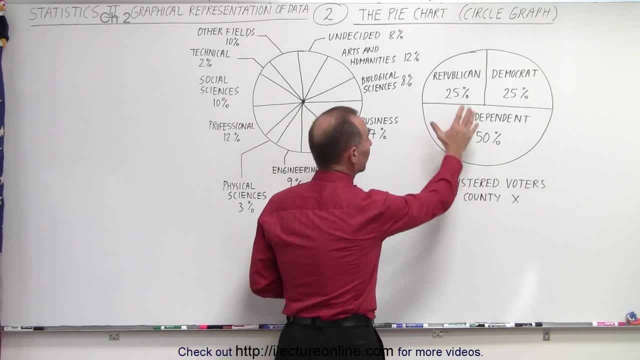 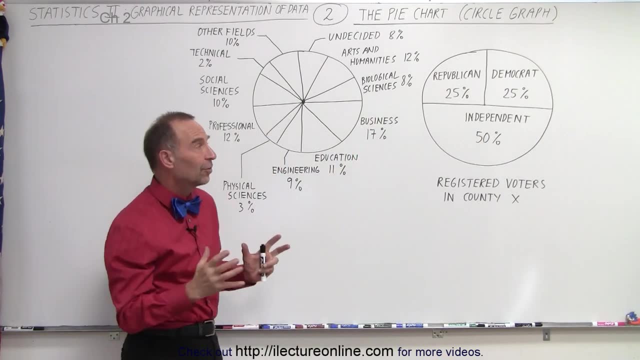 is relatively few. For example, here we only have Republicans, Democrats or Independents registered as voters in a particular county. Since there's only three data types, it gives you a very nice representative view of which one is the most common and which ones are less common, Kind of. 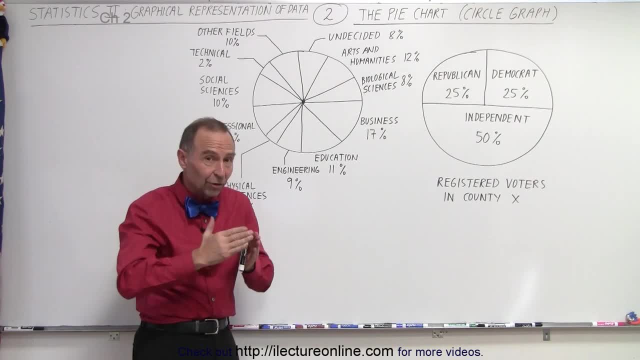 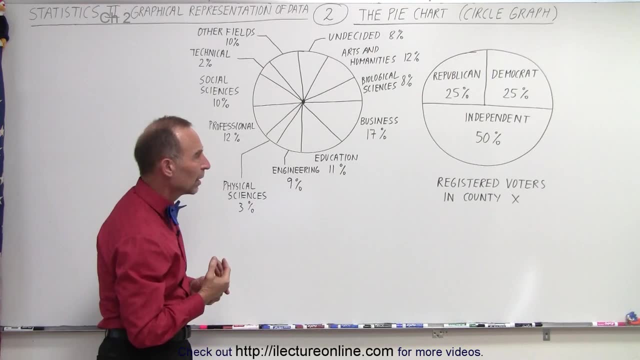 like when you grab a pie and you want a piece of it. you can take a small piece or a large piece If you like the pie, of course, And so you get that same kind of feeling with a pie chart, but it becomes less effective when the data types become large, For example. here may be a 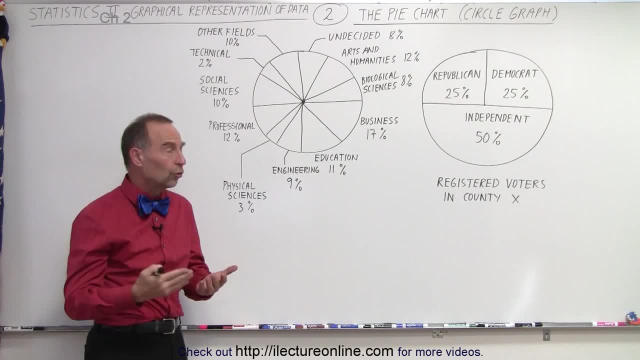 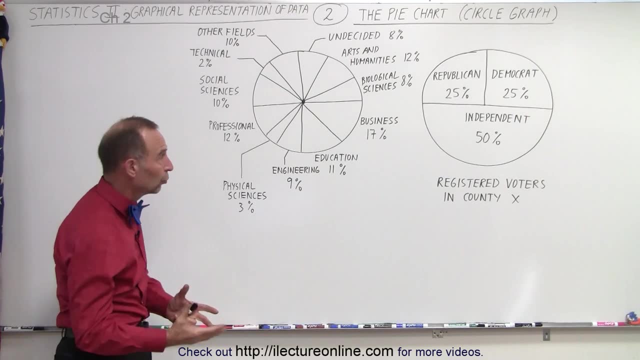 smartphone. This is a smartphone that I use to communicate, for I want to communicate between my survey that was done to find out what the students would like to graduate as, or with one, with what kind of degree they would like to graduate with, or perhaps it's the totality of all the students in the college, and so, as a